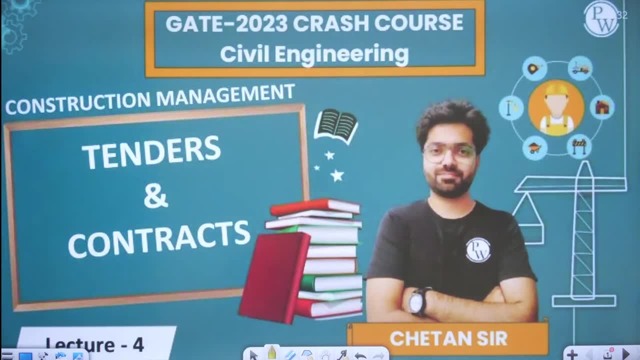 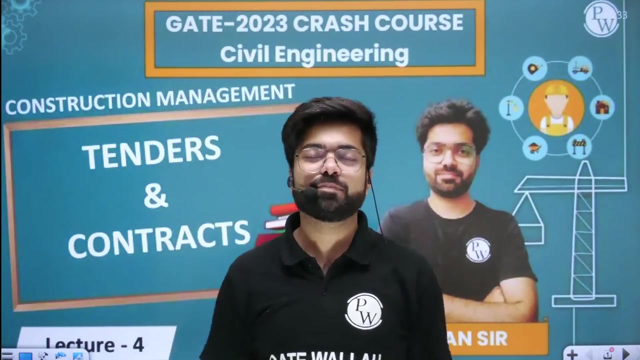 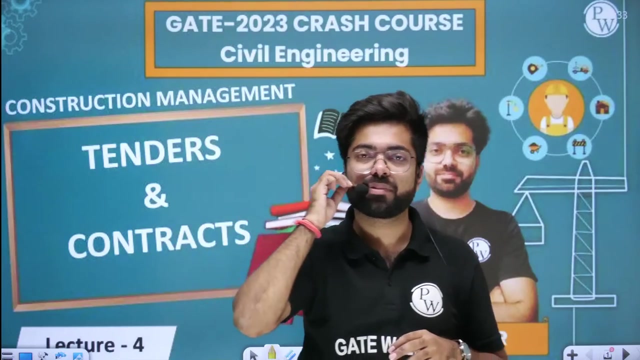 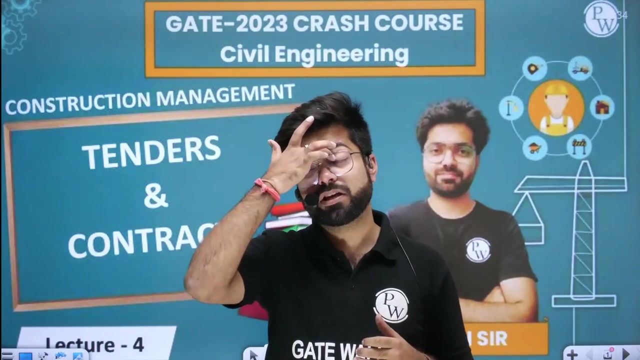 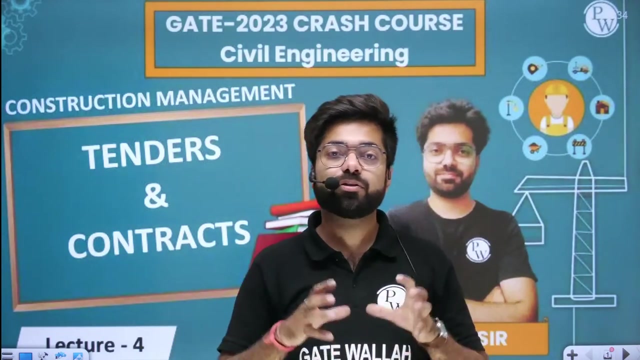 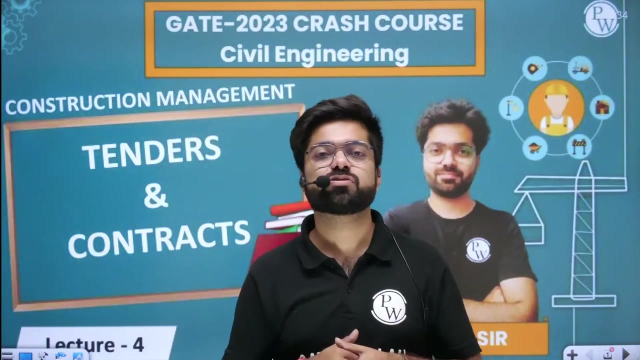 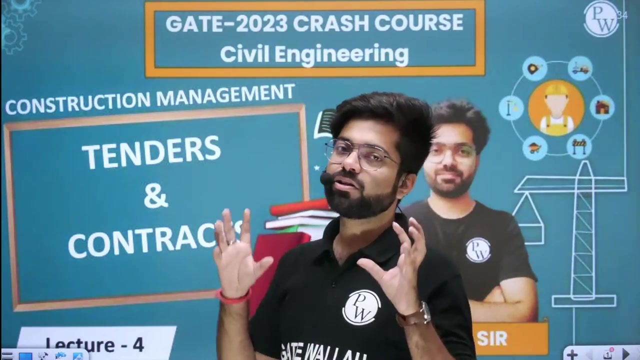 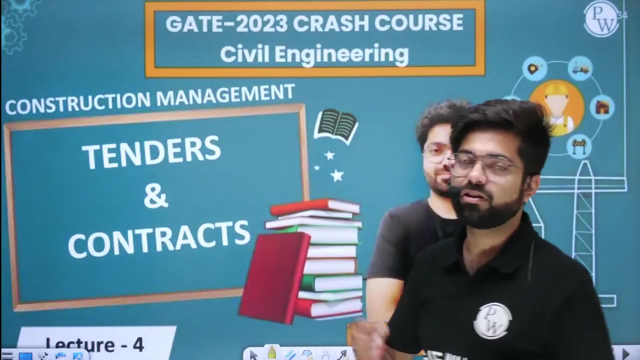 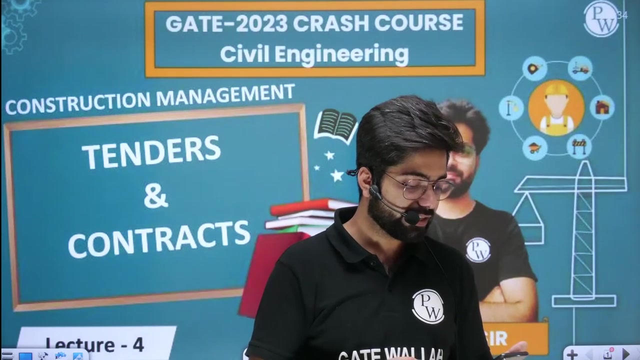 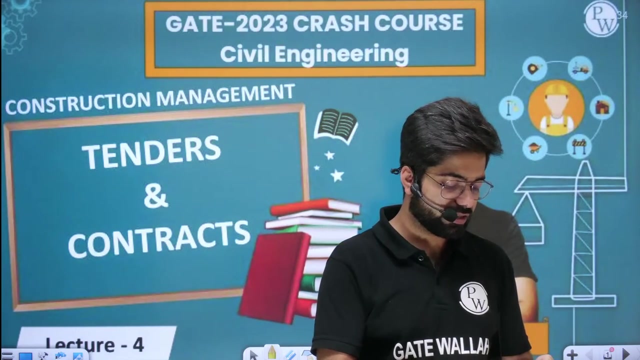 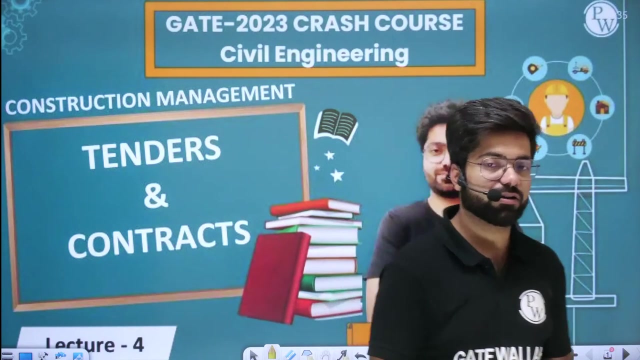 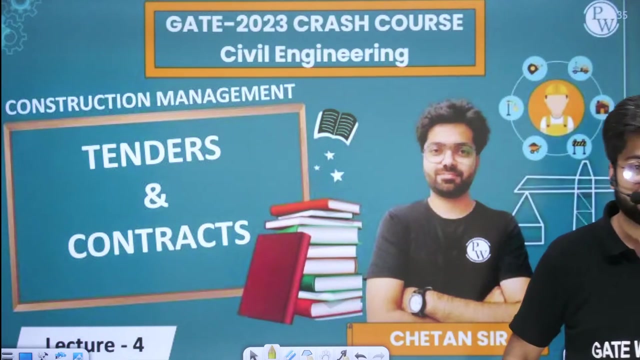 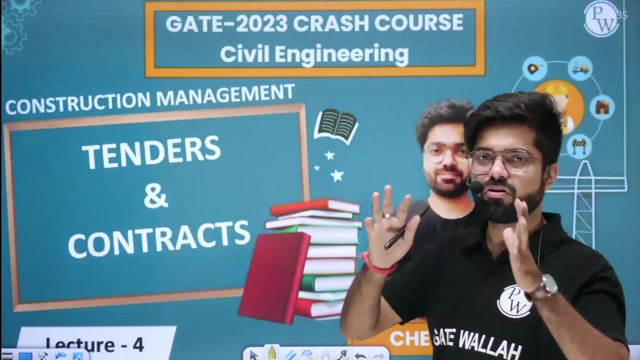 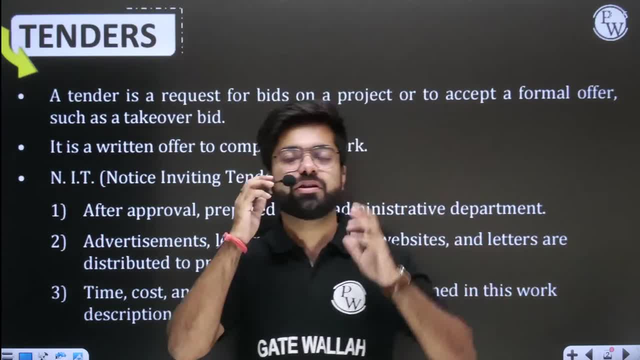 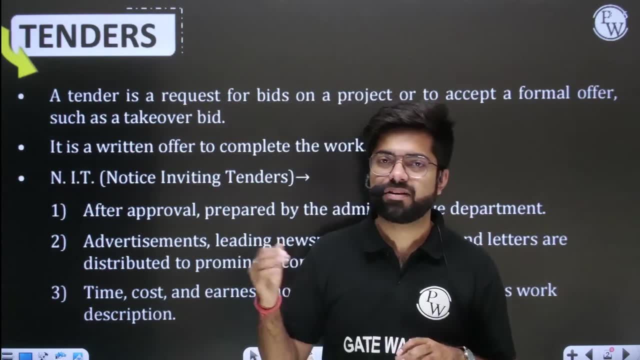 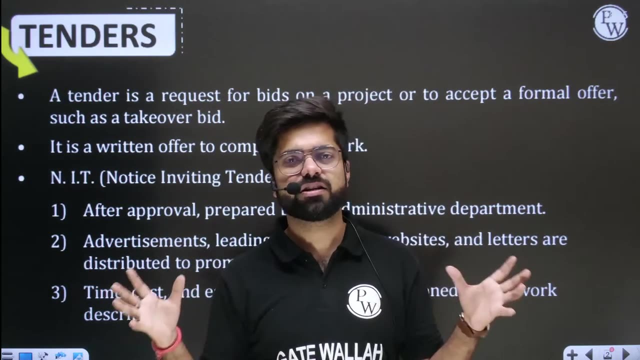 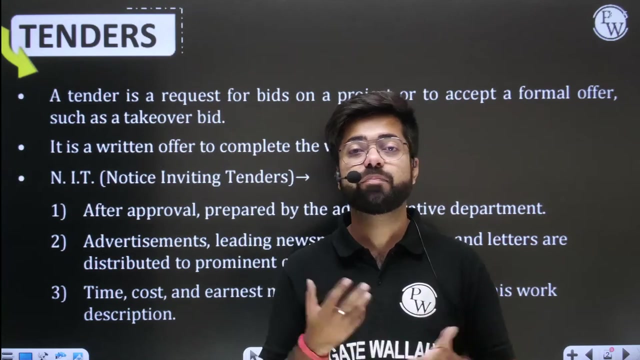 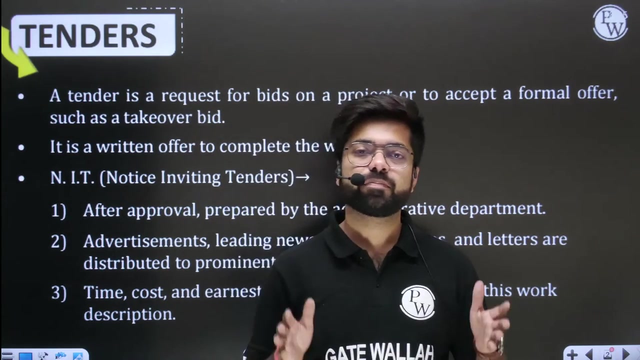 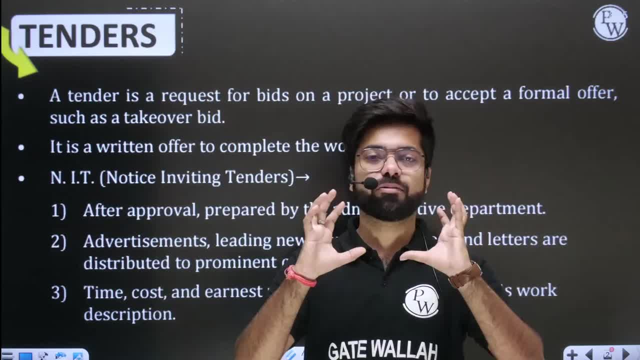 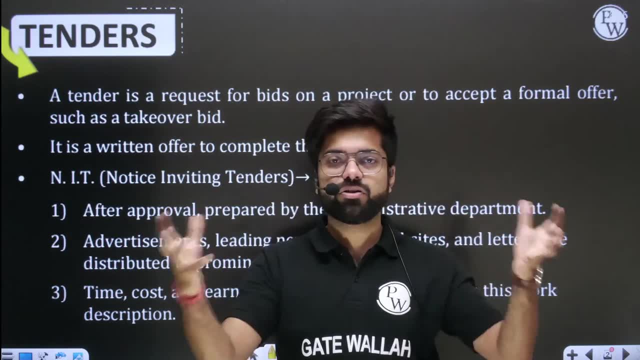 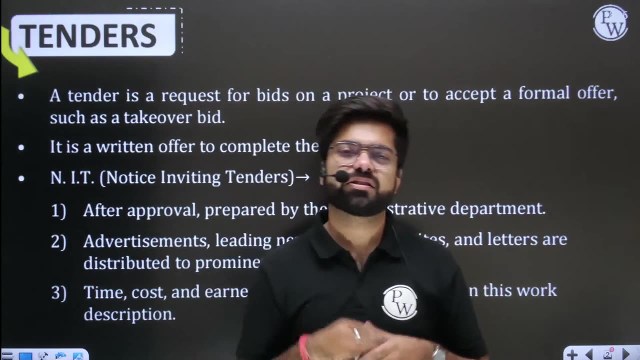 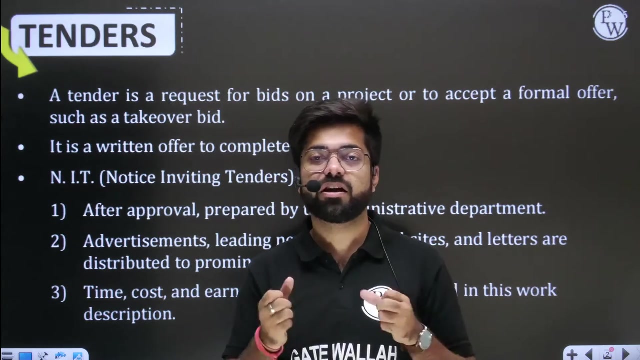 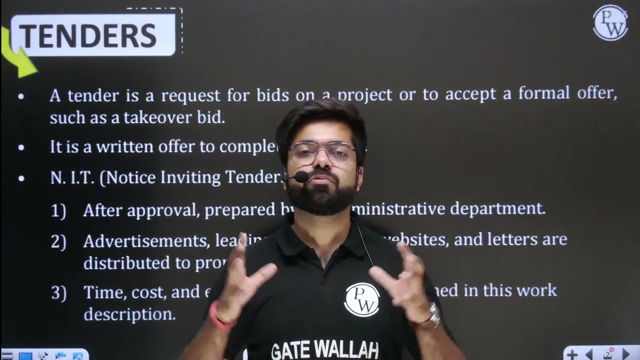 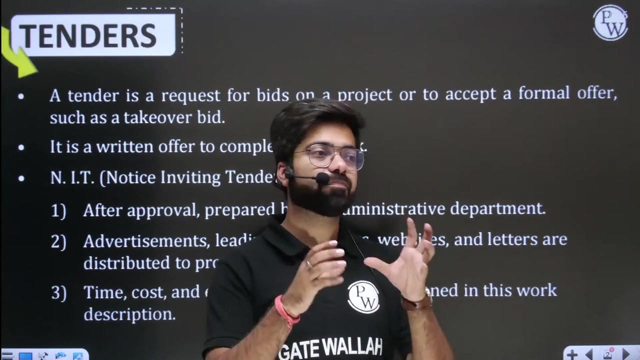 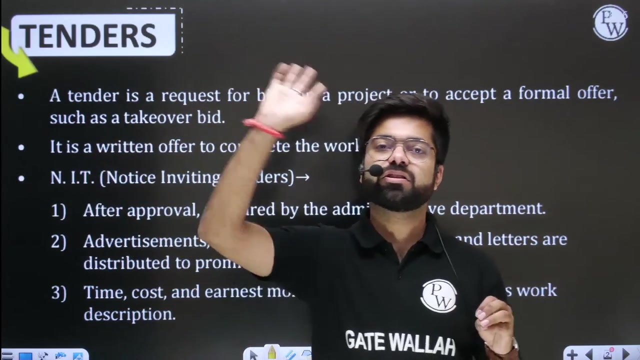 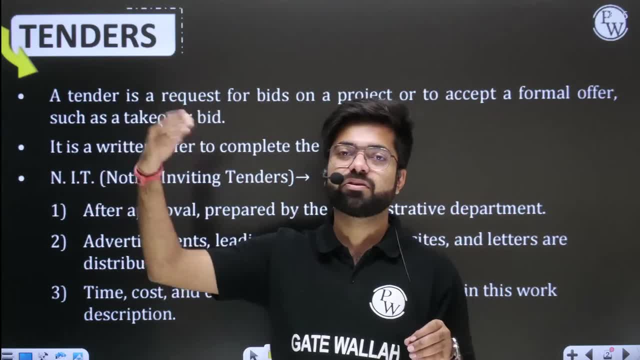 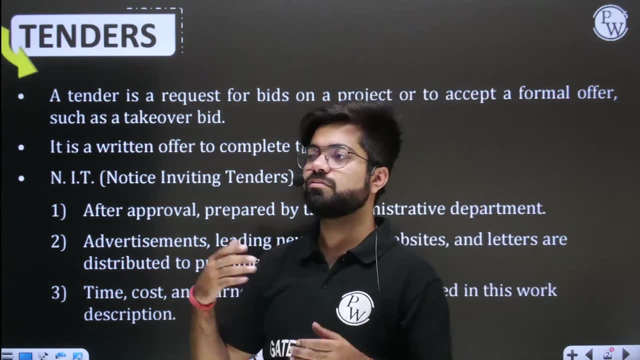 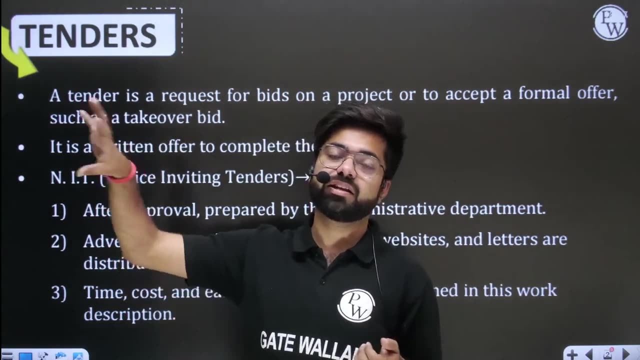 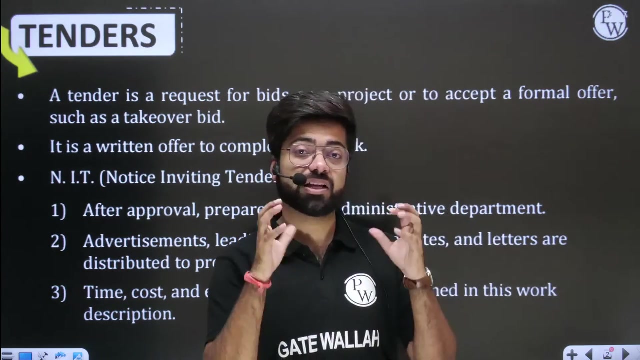 ok, they will manage their farming well, Jaivik. Jaivik means organic farming. that is, every department gets some money, what the state collects, and from that fund obviously improvement comes. you see that development is being done, roads are being made, you will see that dam, weir, pierage, canal, this is being done. irrigation department: ok. such schemes are implemented in different departments: ok. but now it comes to how works work in actual, so that we have to understand today, ok, now, because you are an engineer, when you go further in departments, 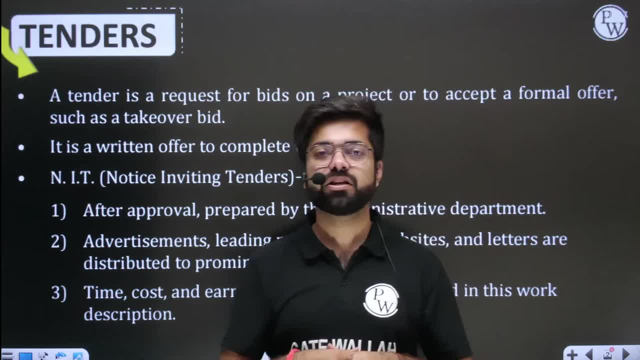 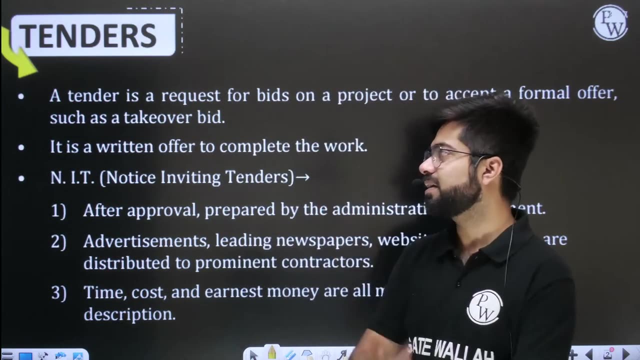 see in as an officer or whatever your post will be. there are also junior engineers, assistant engineers, executive engineers- there are many types of engineers. so at a different level, you will have to deal with all these things. so how the work is done, we are going to talk about that today. so first of all, let's understand what is tender. 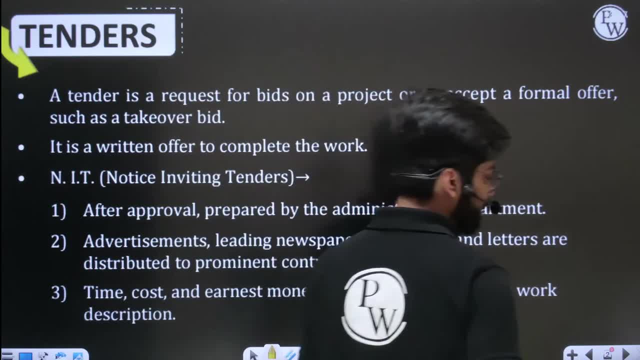 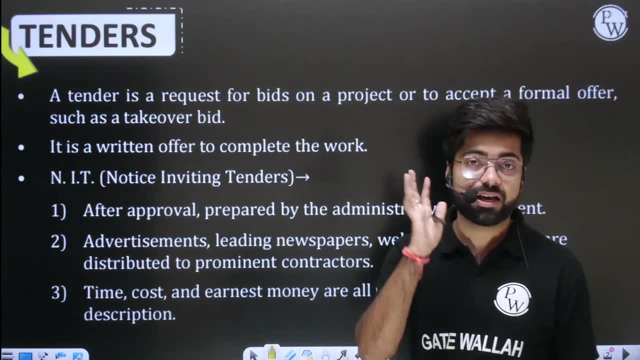 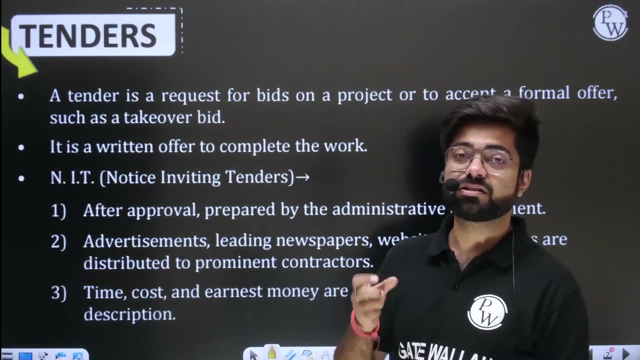 before knowing the tender, let's understand a basic procedure. it is very important. it is absolutely a very good story today. today's story is very good because this real story- that means real. this is a practical story because you will know many things within it: How you give. 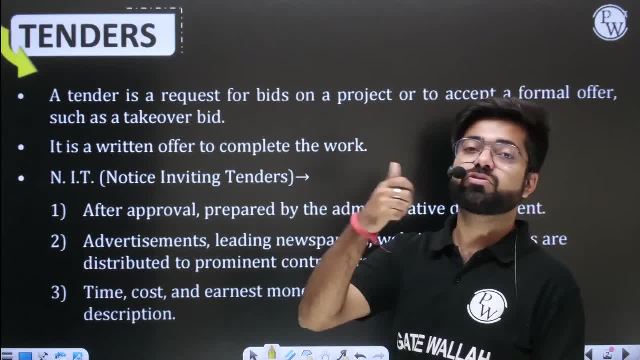 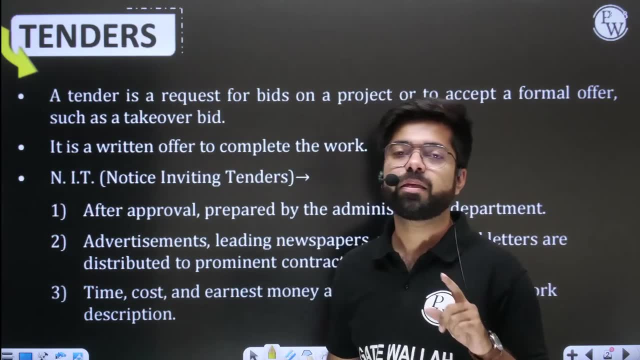 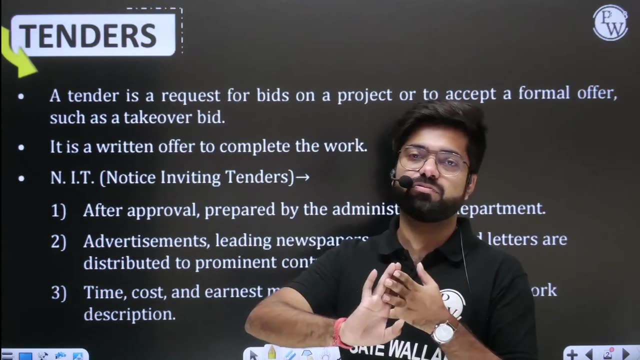 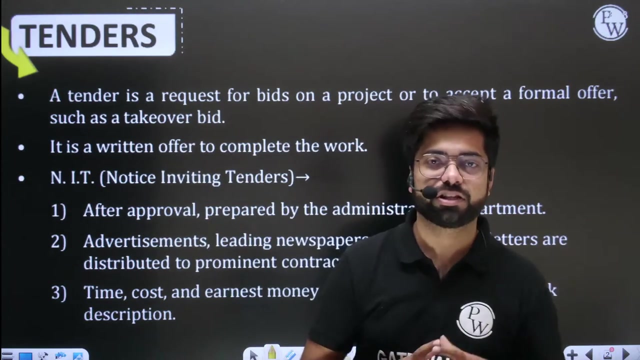 directions and what is tender. what will come in your mind? what is the agreement? then snap here tender. then snap here contract, agreement and different types of tender, different types of contract. we will try to understand this today and we generally like you in any. 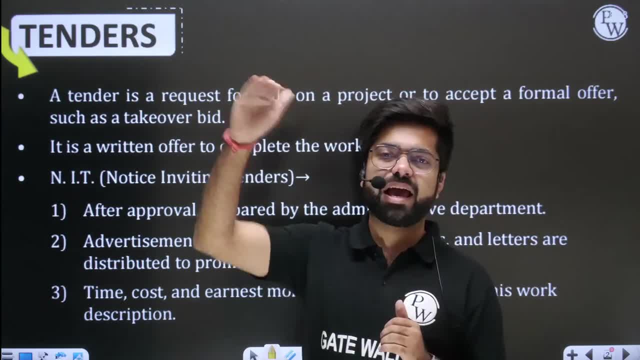 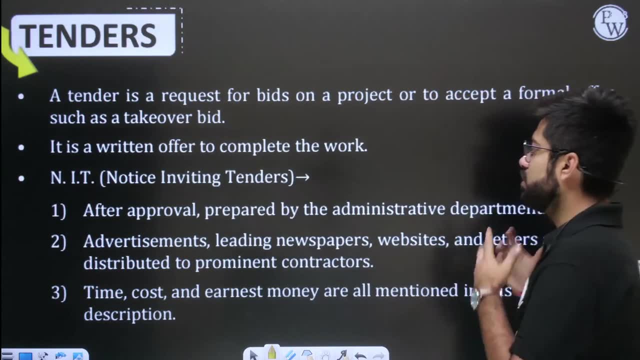 state or any central organization. when you will go then, what is a hierarchy, that? who is above, then, who is below? what is the work of all? so we will try to explain you that. so let's start the story. see, this is any work has to happen, like, for example- we take an example- a canal. 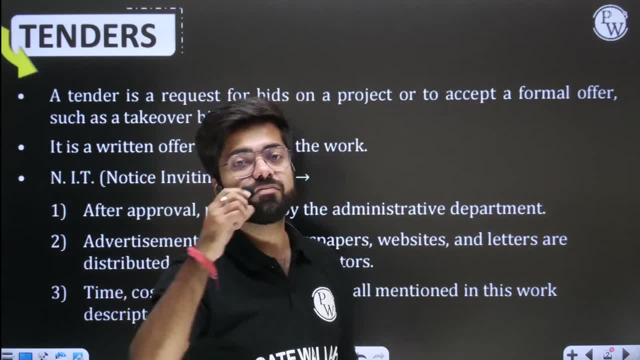 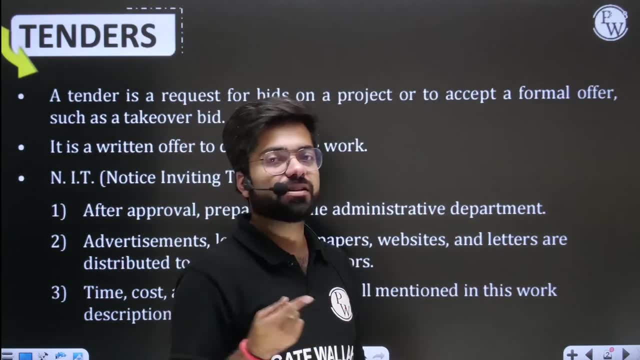 has to be constructed. so this work will come in which department? this will come in the water resource and in the irrigation department. why is the canal made? to do irrigation? why is the canal made so that irrigation can be done? everyone knows this thing. so now suppose this work is happening. 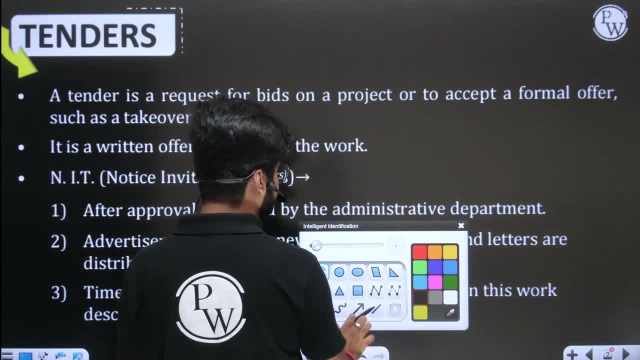 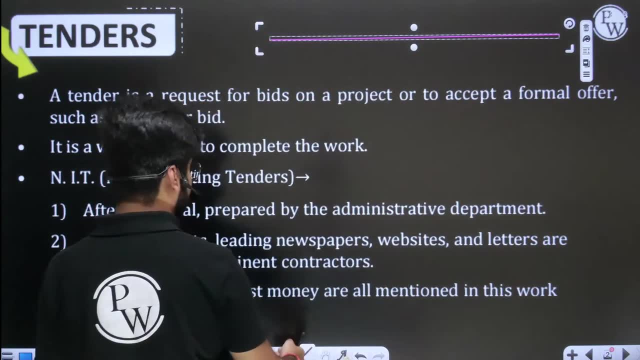 so let's make a timeline here. see, here we will make a good timeline. see, the process should be read with fun. then things come to a good understanding. so suppose this is our timeline. now, in this timeline, what happens in the beginning? that suppose in the irrigation department, whatever the irrigation department will be. 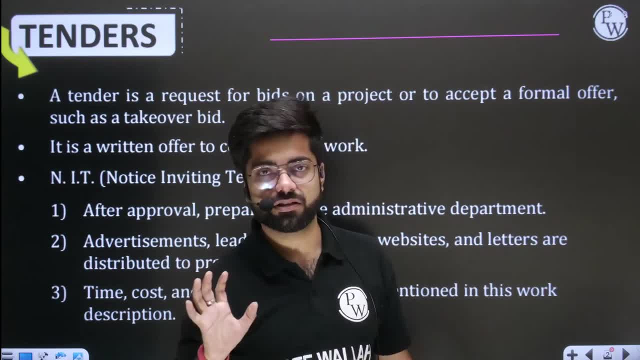 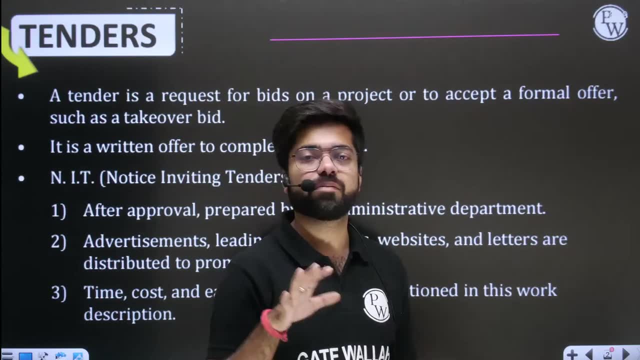 there is a tendency to work itself in. it can work fine, but tell you the truth, nothing like this happens. all the work is done by third party, from outside contractors. third party is done. third party brother is like this: you will make it, yes, you will make it. you will make it. 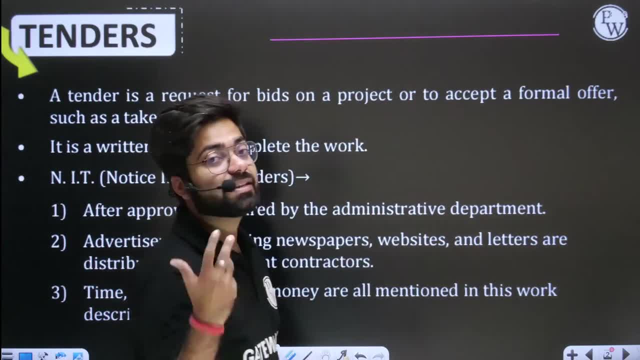 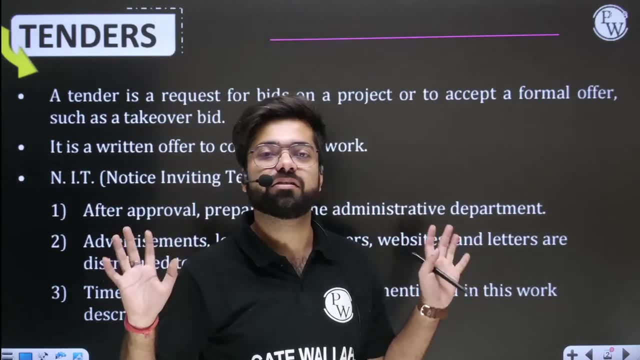 talk to a lot of people. so how can we talk like this? how can we reach a competent person or qualified person who will make a good path for us? department is happy, department is money. who is giving money? state government or central government? any central level work can be done and state level work can be done. 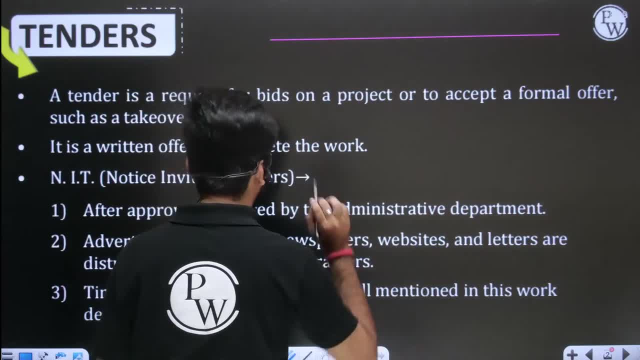 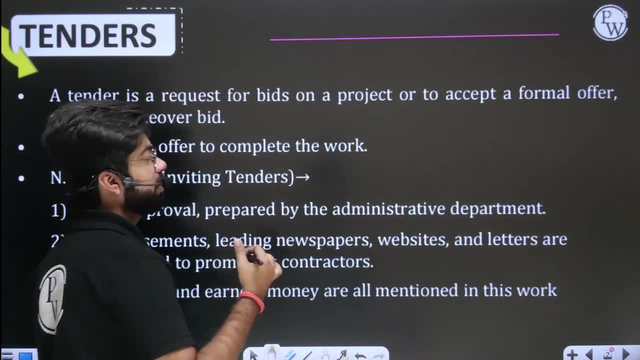 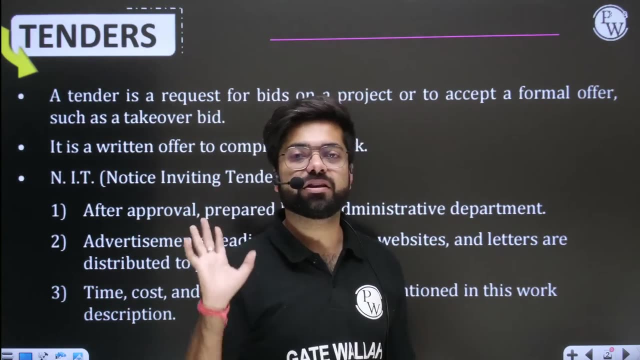 work can work. so see, here started time, now the time starts. so first of all, here is tender float. tender float means ad is given, are given. advertisement department has made in mind that the 80 km canal has to be made from here. it will go here. it should be so wide, it should be so deep, it should be like this it should be. 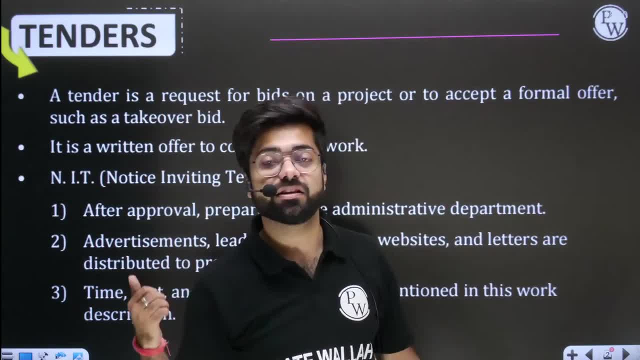 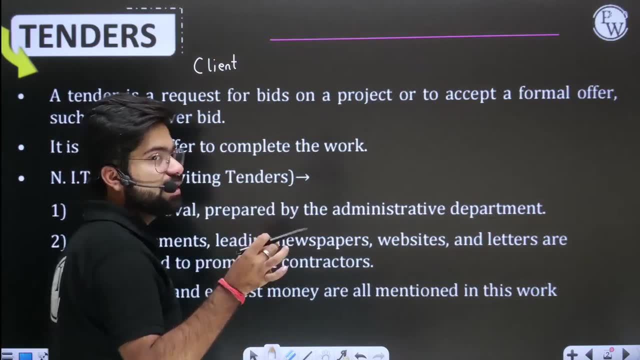 like this. you think it all. who thought it was the client, what is called a client? so, first of all, the client can say anything to that. What is that client? I see the archives. The client has cleared all the pictures in his mind that I have to do this and that. 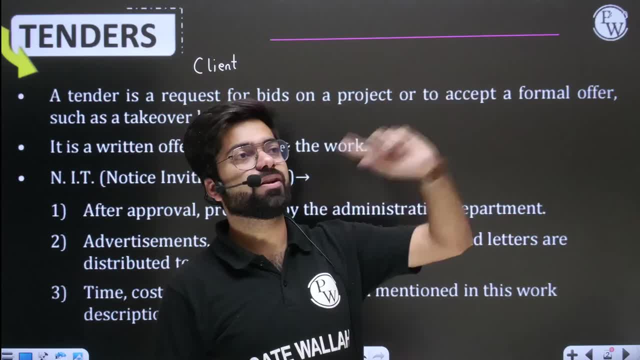 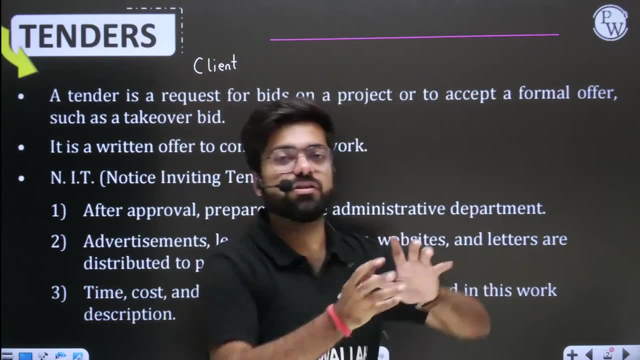 Now, if there is a PWD, then let's say that the PWD wants a metro line to go from here, or the PWD wants a road to be made from here. It should be of this much kilometer, it should be of this thickness, it should be like this, it should be like this, it should be like this, it should be like that. 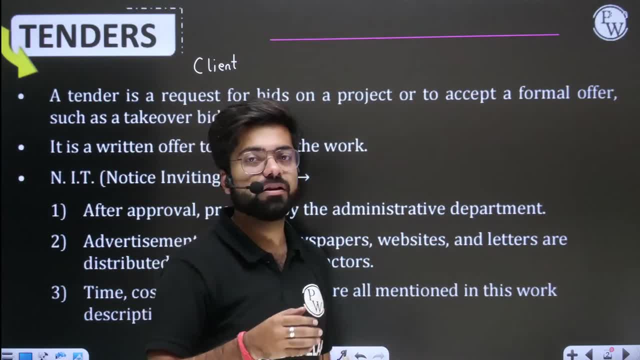 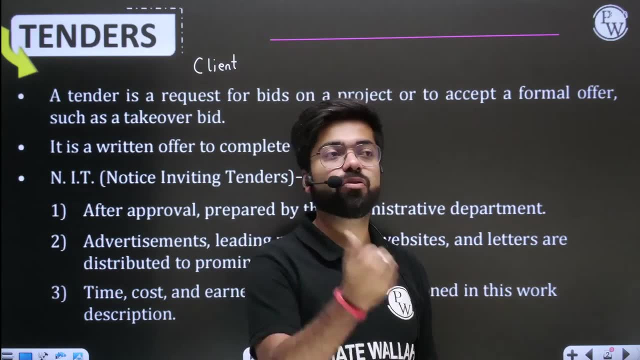 All this is kept in mind by the client. Let's say: you will become a client in the future. You are a private client and he is a government client. There is only this much difference. Client means the one who needs something. Now let's say that our house should be made. 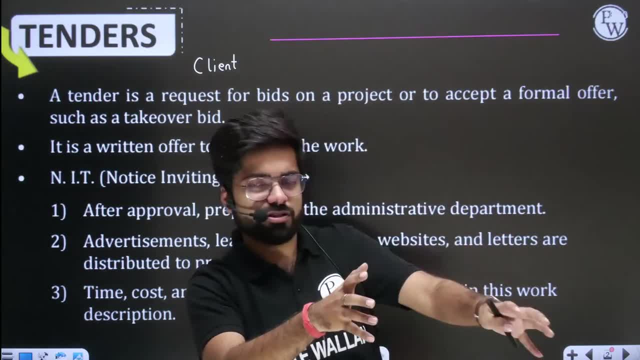 It should be of three floors. It also needs a swimming pool. It also needs this. It also needs that There should be a movie hall in the back. There should be a garden in the front. So these are the specifications of the client. 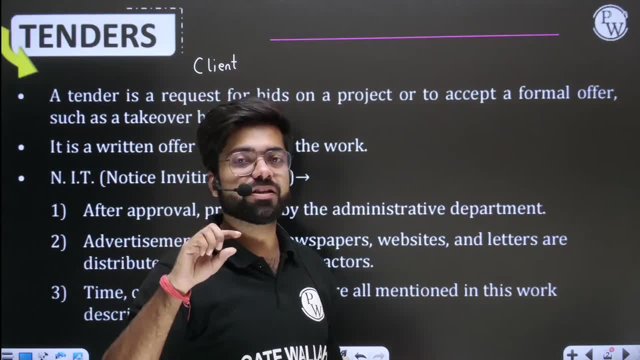 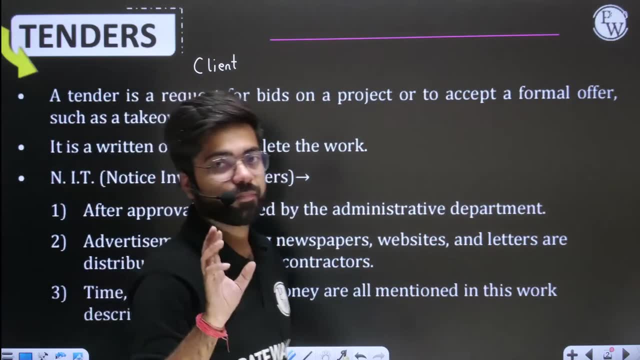 What are the specifications? In this whole lecture we will say spec again and again. Spec means specification. So the client has thought of his specification. Whatever work he has to do Now, he needs a good man who works well. So to find him he takes out a form. 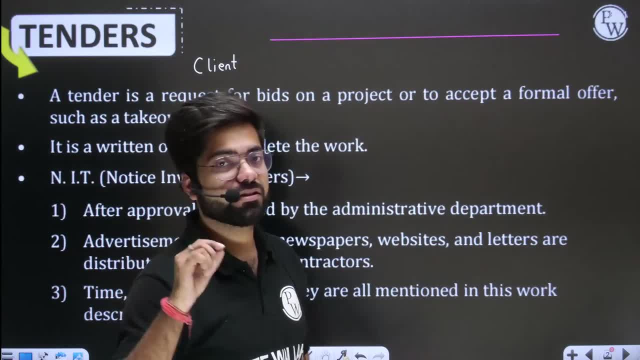 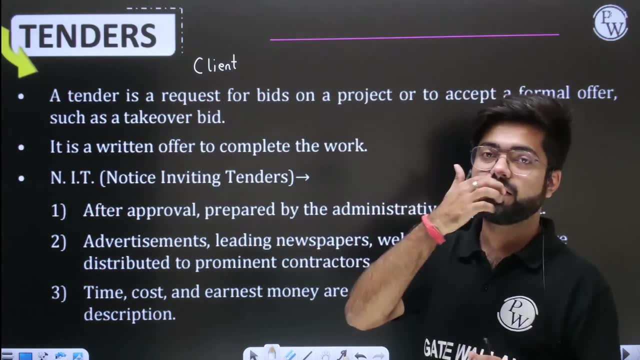 Which we call tender form. Let's talk about tender form. First will be NIT. What will come first, You will understand carefully. First will be NIT Notice Inviting Tender. A notice will come out. You must have seen in the paper. 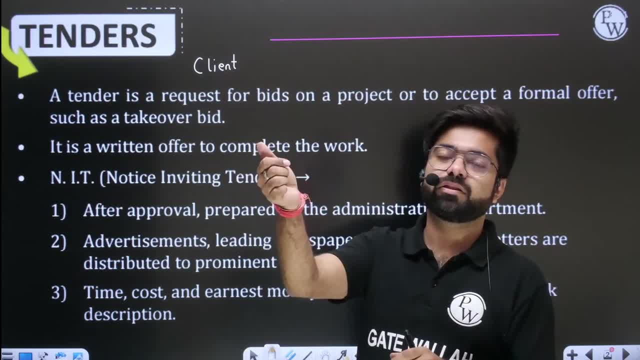 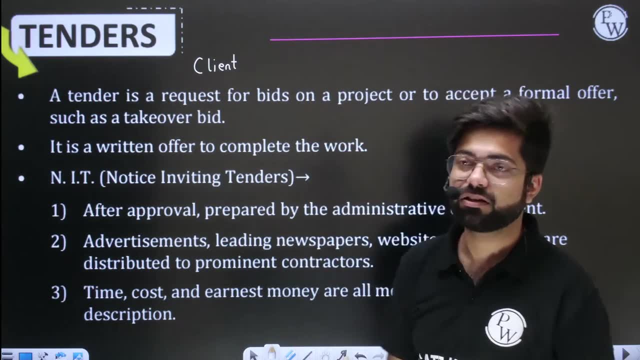 Hindi newspaper comes. It is written as Vigyapti. It is written as Vigyapti. It is written that this is some work, This is such and such. These things have to happen. That is the date of its publishing comes. 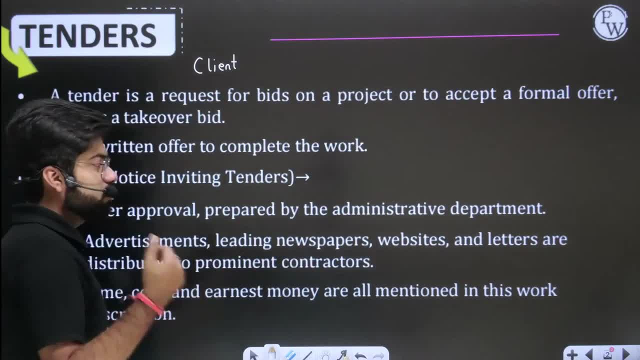 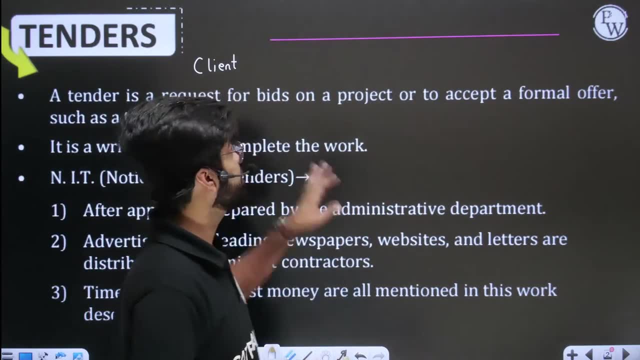 So at least these things should come out in some newspapers Now notice: inviting tender means Simply: we gave this notice that we need such and such work. Who is it? Come to us, Meet us, Talk to us, We will give money Work. 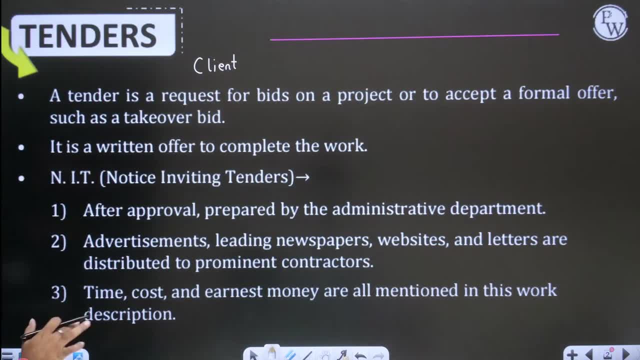 So we make an NIT. There is a whole document. There is a document- This is our notice. inviting tender- Okay Means what is written in it: Approximately how much time we have, How much money is our budget Okay, How much time we have. 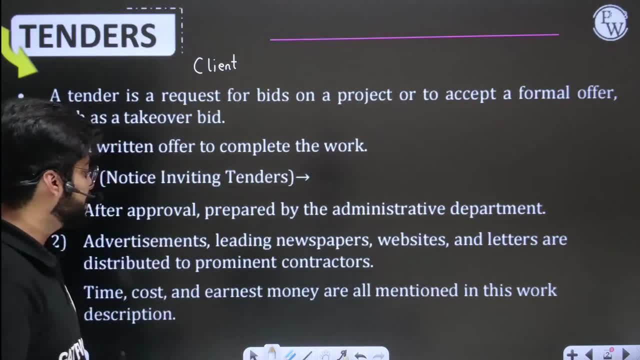 How long should the canal be made? How much money should we invest? Okay, There is earnest money. Okay, We will tell you about earnest money later. So all these things are written in your NIT. NIT means notice, inviting tender. 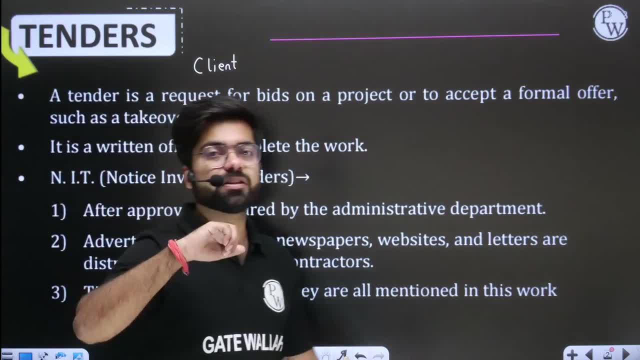 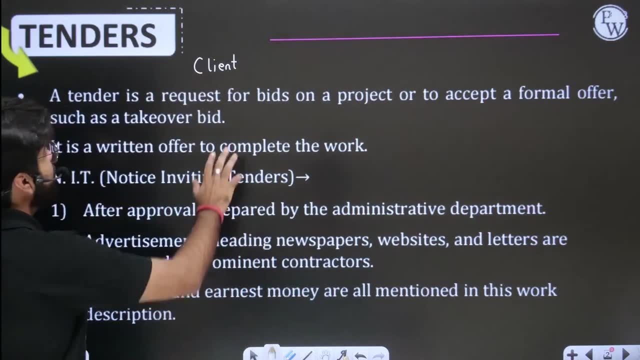 There is a notice. So many people see this notice in the newspaper And the one who knows how to make a canal, He will come and apply his tender. Okay, So if someone asks you what is tender, So tender? you can say this simply: 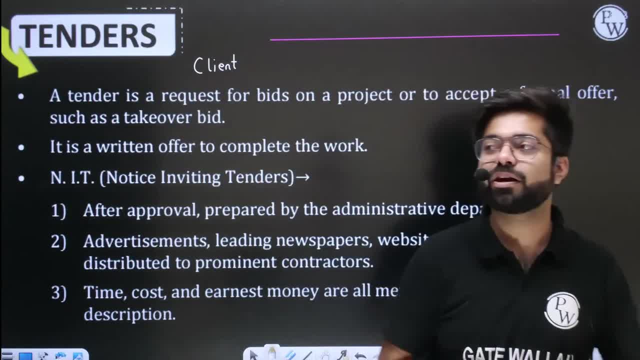 There is a bid. Do you understand what a bid means? Bid? If you are not able to understand the bid, Let me explain it to you in a better way. There is a bid. Okay, Should I take this example or not? 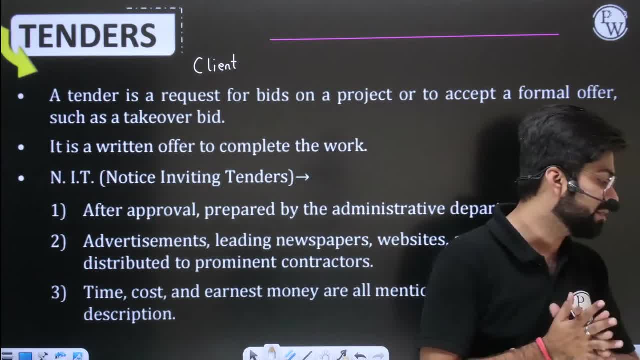 Let's take it. Okay, Let's take the example. Like what happens nowadays, There is a lot of wedding atmosphere going on. You know that all these people have a wedding atmosphere. So what happens in that? The boy who is there, 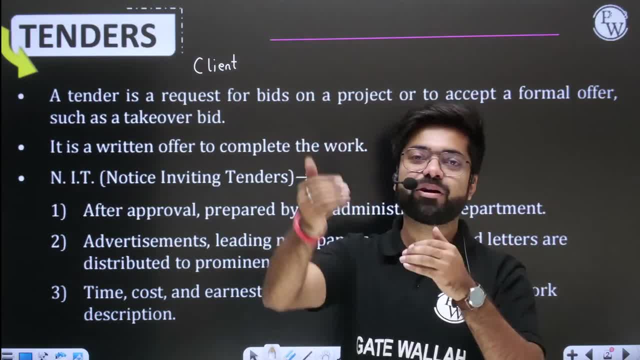 There are a lot of bio data coming from him. Okay, Bid is coming. You are not able to understand. Hey, marriage is also a project. Marriage is also a work. It is a project. Now, what happens in marriage? That a lot of bids come. 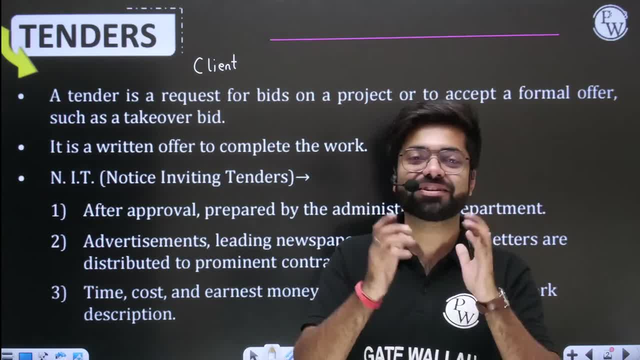 Yes, brother, This face. There are a lot of filters. It should be like this. It should be like this: The same work is also done, The same program is the same. So a lot of people have tendered Yes. 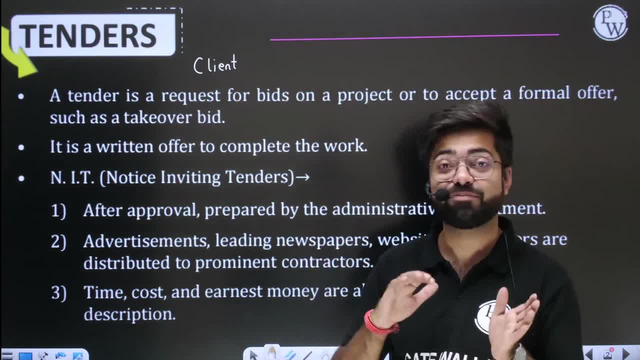 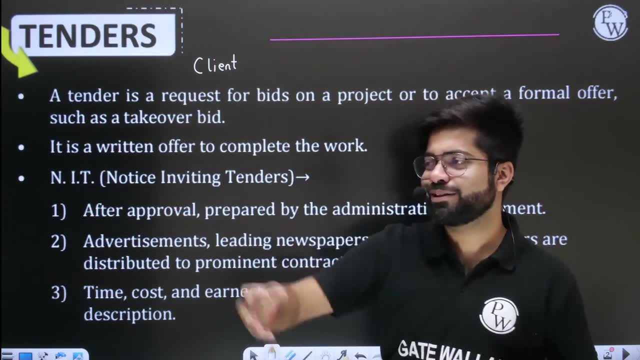 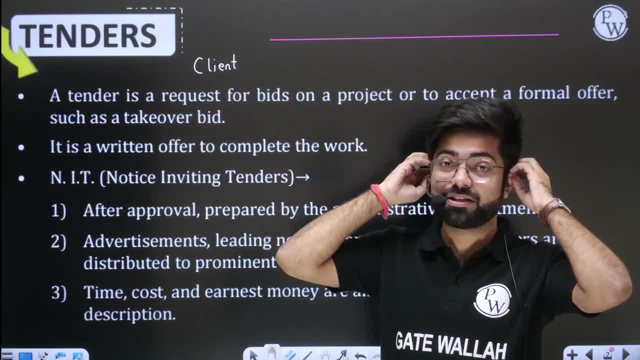 Many people bid In. our program is. We are there. We have some we look like. By the way, I saw there It is not. Look, everyone wants to get it. What is it, brother, If you are a government employee? 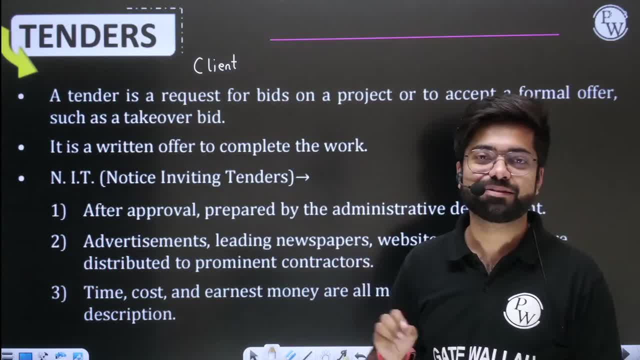 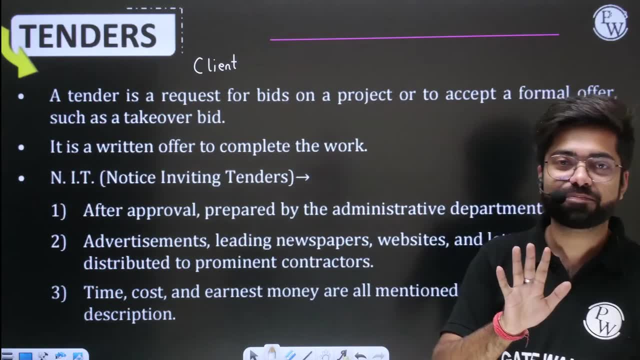 Good will be. So good work. You can say that. The placement: Yes, It is a very good guy. You can say that. So a lot of people microphones and fill, But aich not fill. Everybody forms. Look, we look like this. 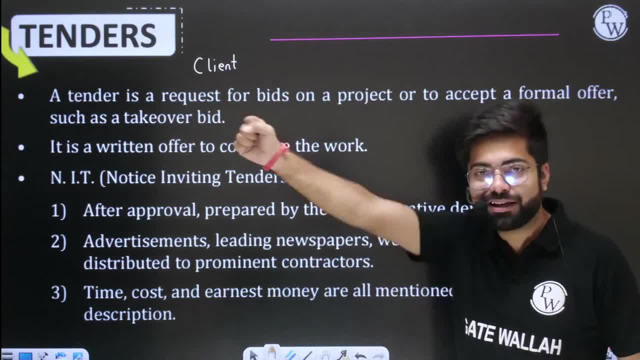 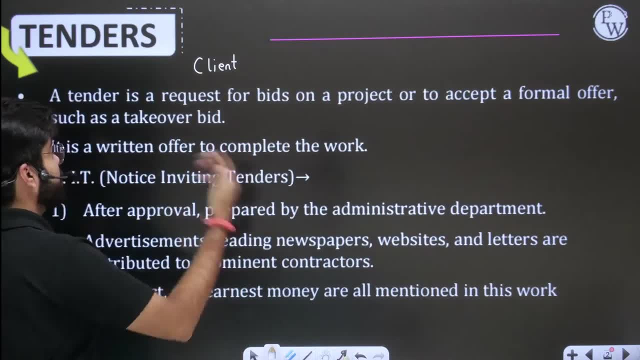 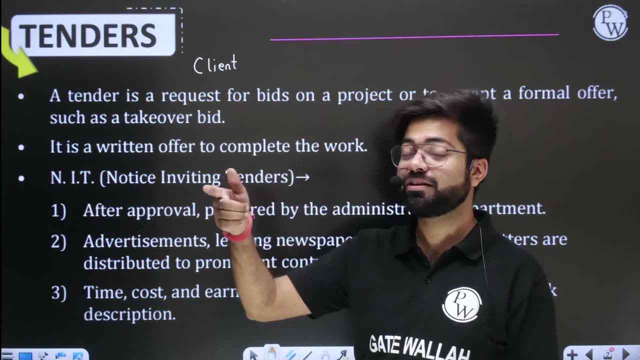 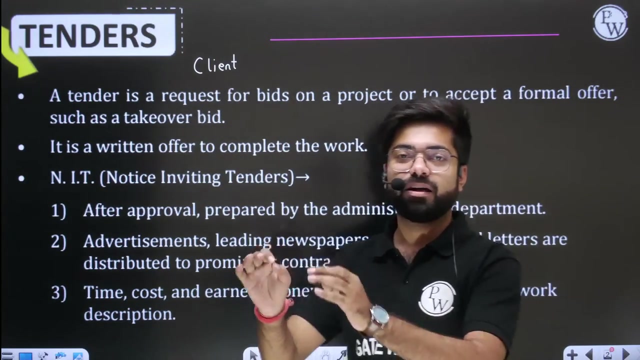 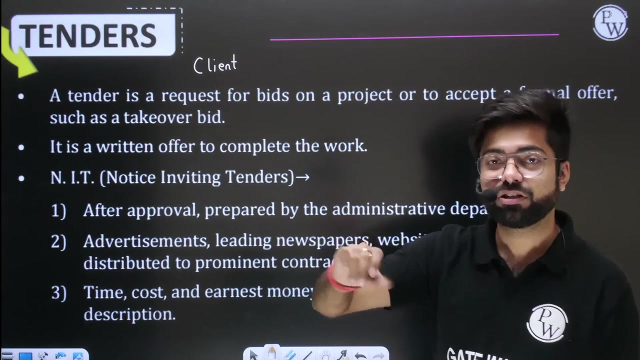 We look like this. We are this, We are. We want to make a channel. we want to marry him. we want to marry him. this is a bid. okay, so we understood it as a bid. we understood it as a proposal. so what is the symbol of the tender? what is the symbol of the tender? we are simply requesting that we get married to us. that is, we will not get married to us. what to do with us? we will make a good one. okay, we are simply requesting here that we are good. we are very capable. try it once. we will make such a channel and give it to you. you will enjoy such a channel. okay, so this is a bid. 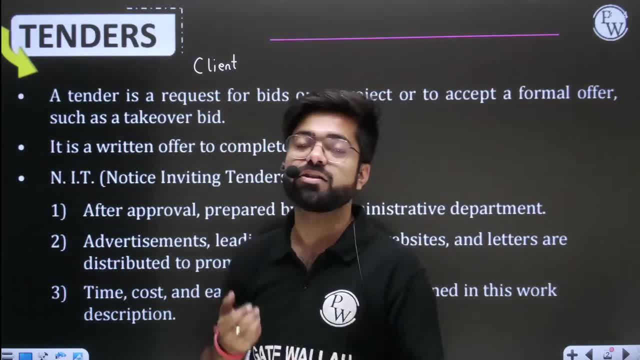 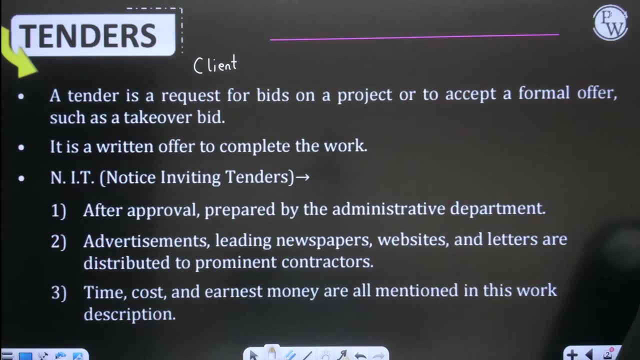 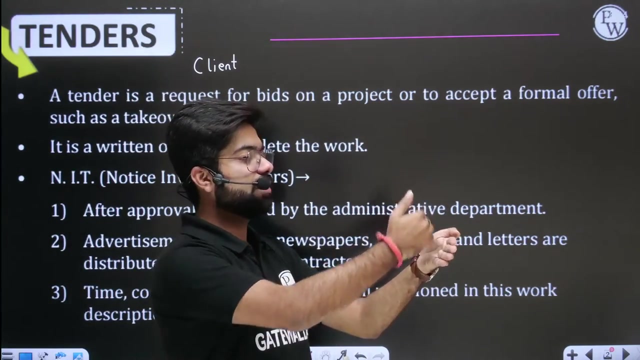 Now everyone has put a request here. many people try: brother, there is a lot of government money, a lot of money is earned, people do it a little high. so all this lecture has just started. okay, come on. there is a lot of laughter going on in this time, no one. so here the request starts coming for some project. that is, it is a formal offer. okay, now, as soon as the wedding event comes, then a picture comes in the bio data and below 50 things are written that this is done in this way. so many things will come. 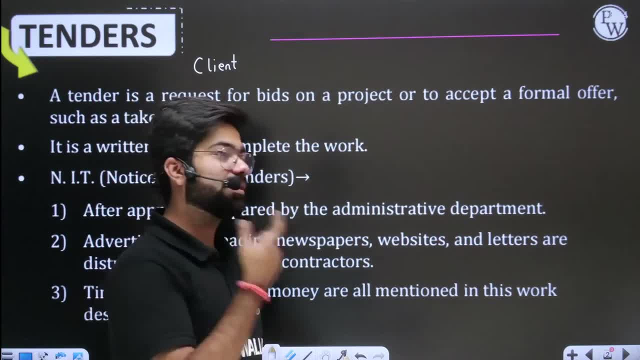 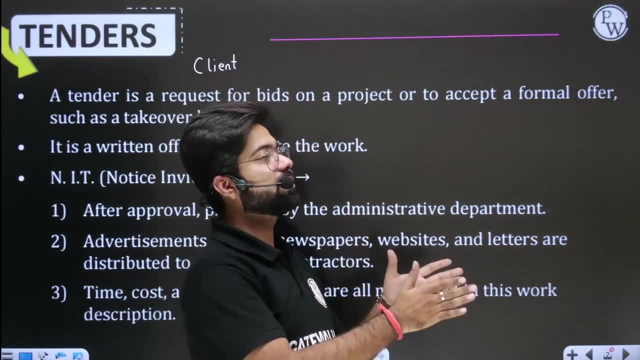 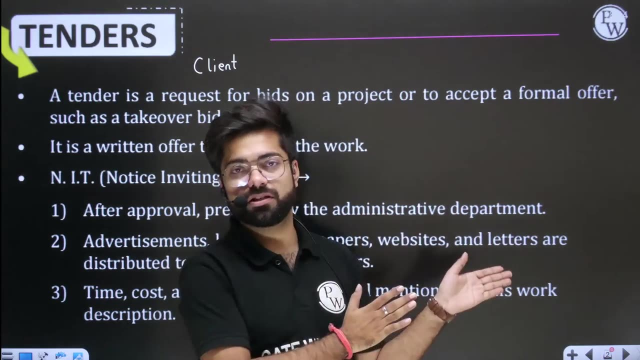 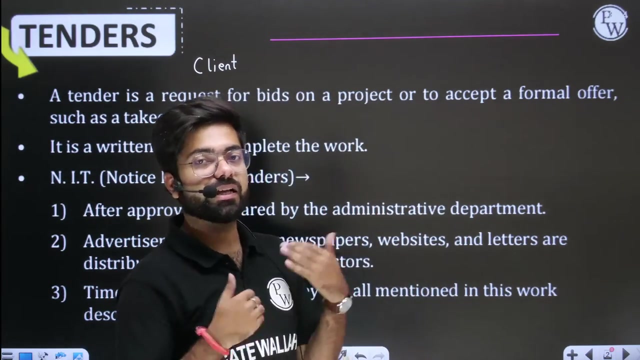 Now when you have to select. you are a client, you will have to select who to do the work from. so what will you see? obviously, you will see a lot of things in its form, right. you will see from it in the form that brother. you will ask him how you have worked in the last five years. you have never made a channel, or not. how good is your company working behind? it will be seen to the past experience. which successful projects have you done? then his technical qualification will be checked right that when people get married they see the entire history of life in it. 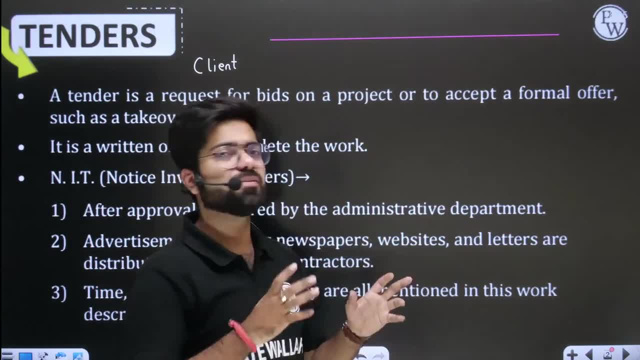 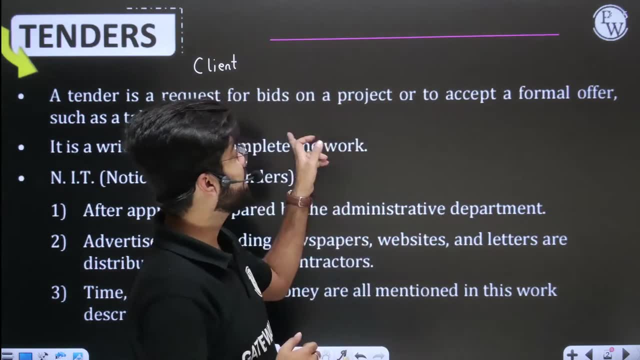 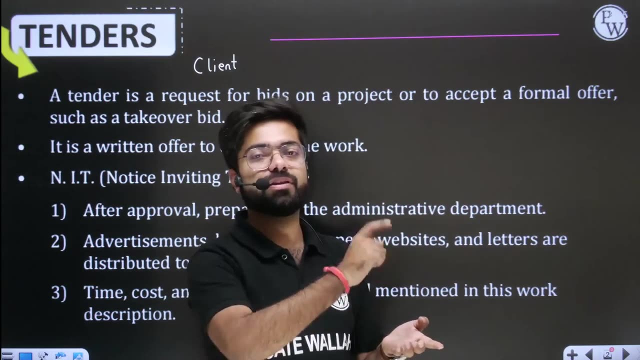 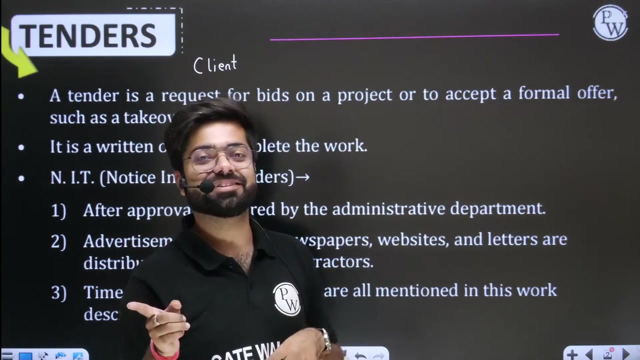 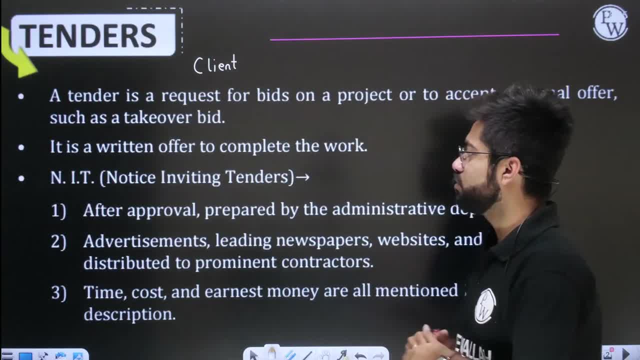 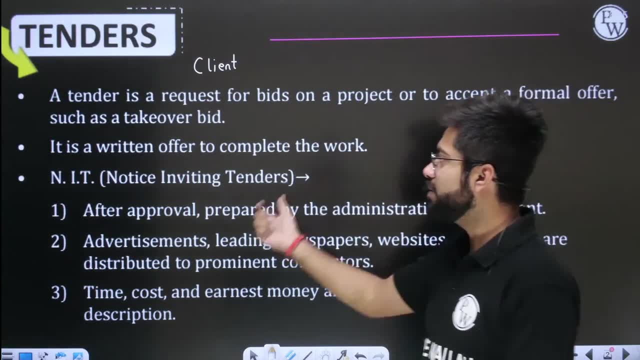 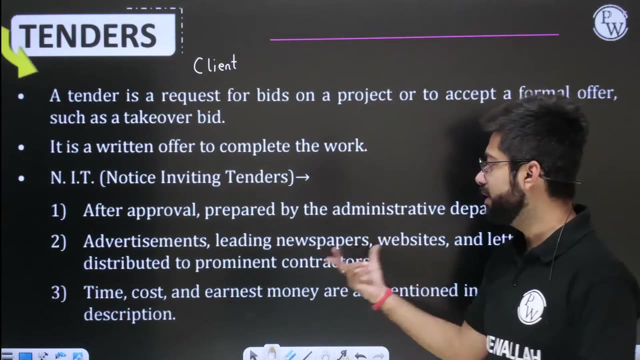 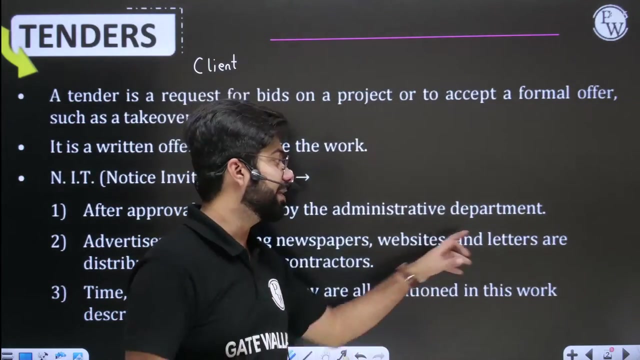 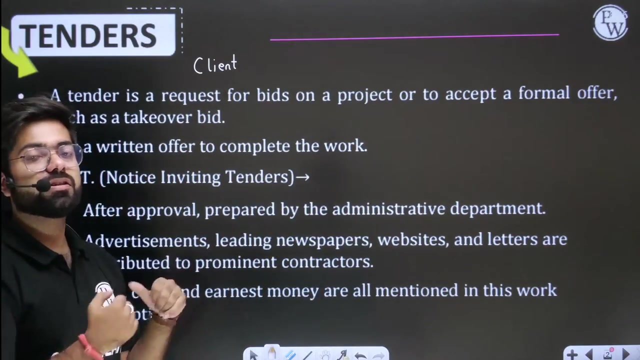 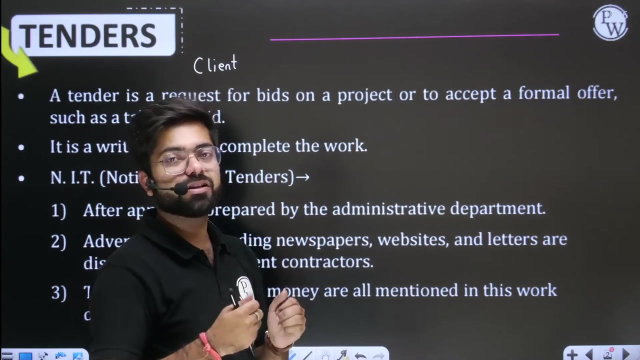 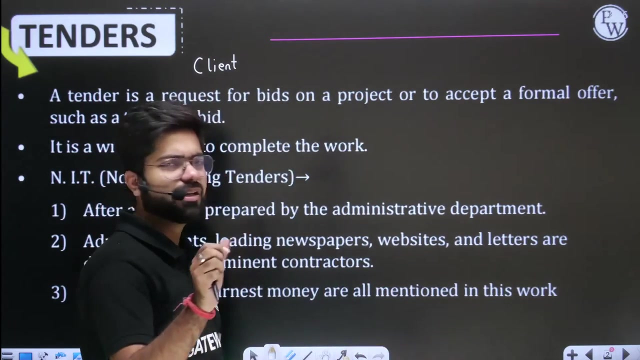 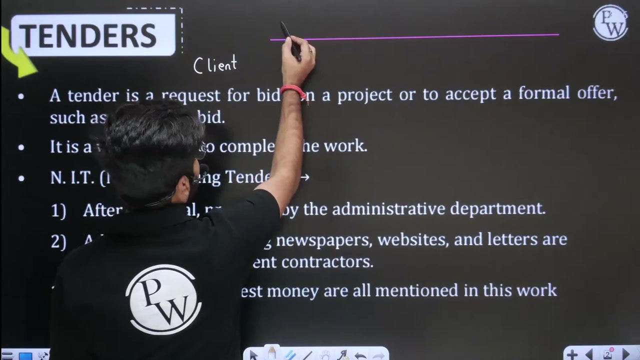 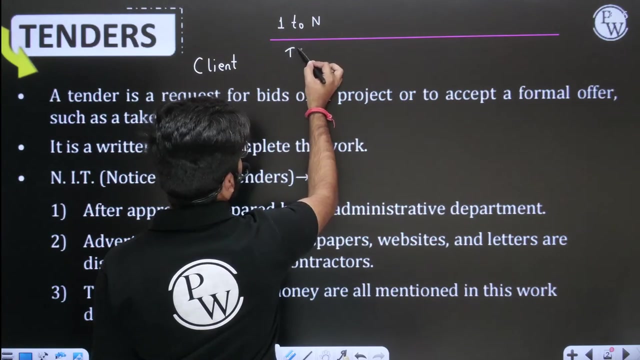 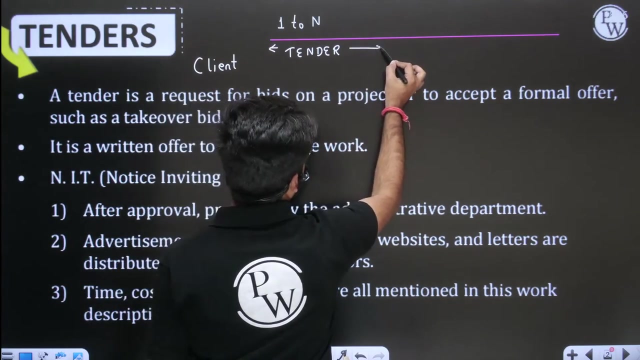 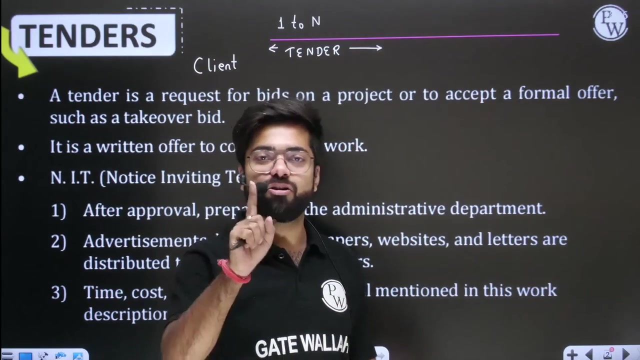 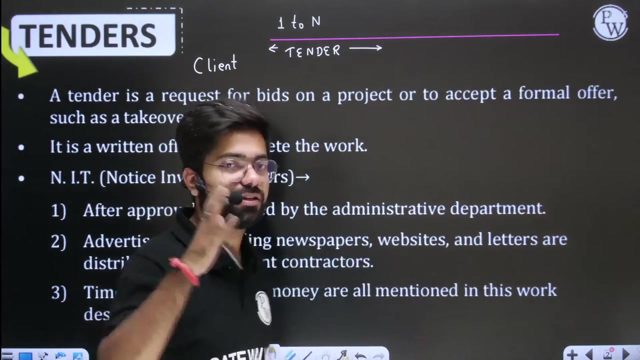 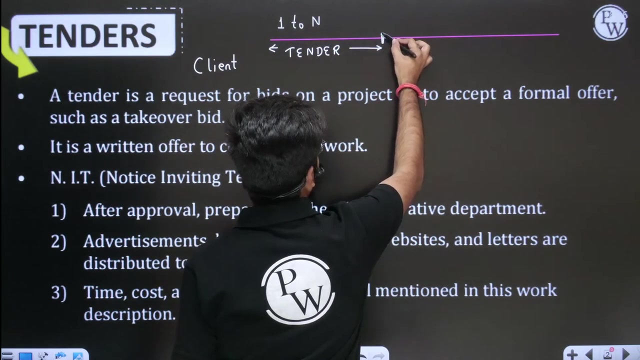 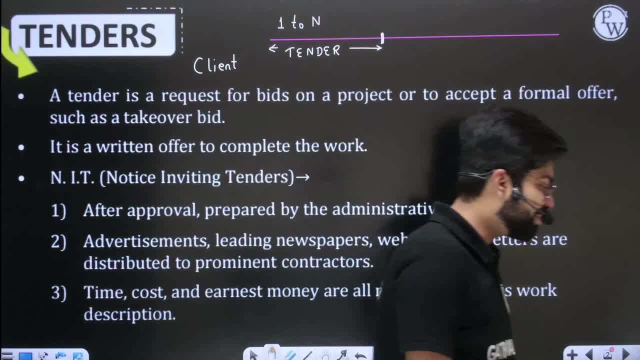 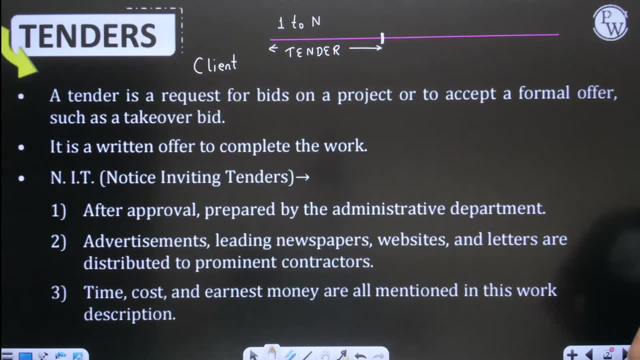 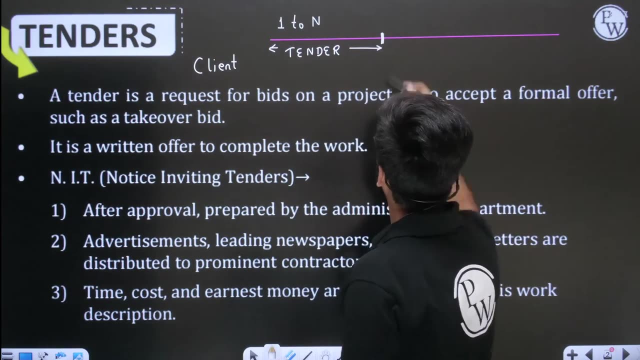 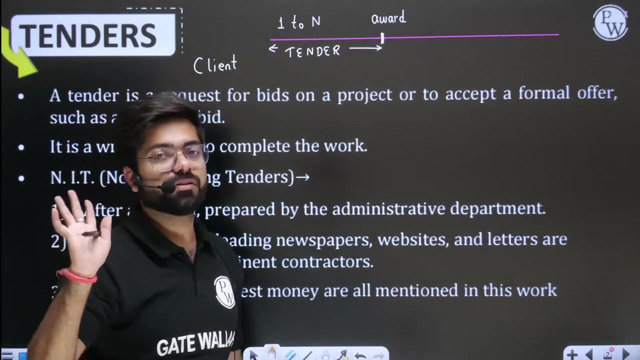 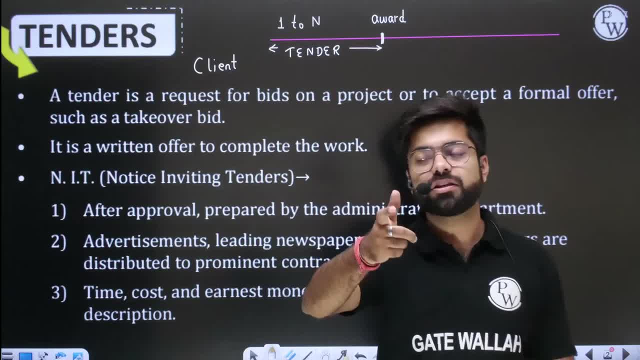 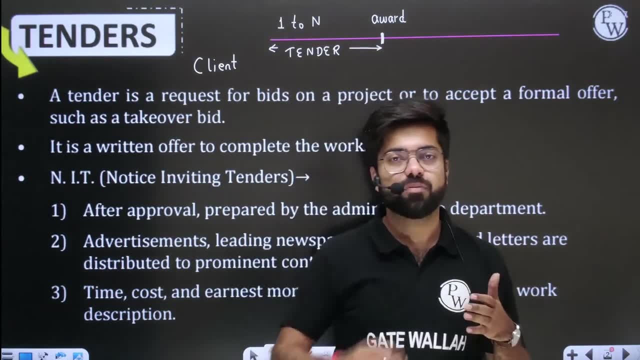 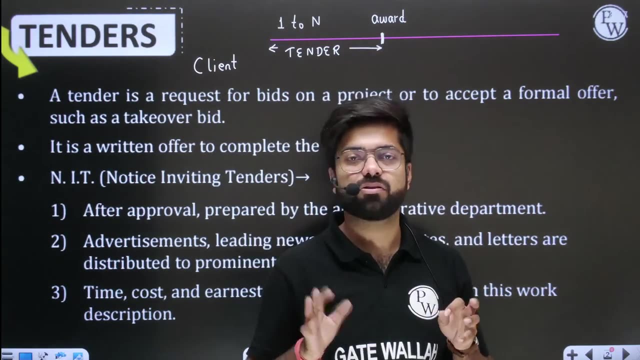 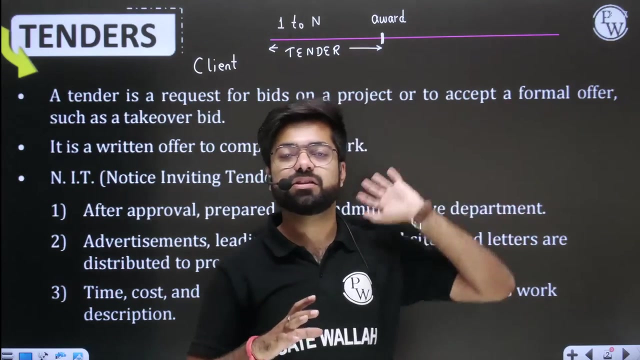 Now either there will be an agreement or a contract. agreement means that in which the law is not very involved, for example, in our house. if we talk about our house, then an aunty comes to our house and works. we have told her that we will give you 2000 rupees a month, okay, and you be happy. so have we signed anything? tell me something: if we stop paying money somewhere, aunty runs away the next day suddenly, then we will go here and file an FIR in the police. tell me if we will do it or not. think about it. 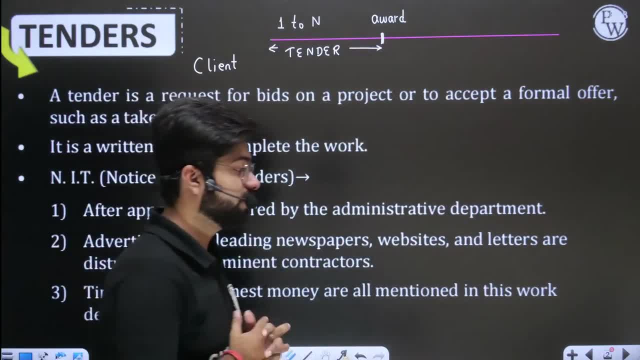 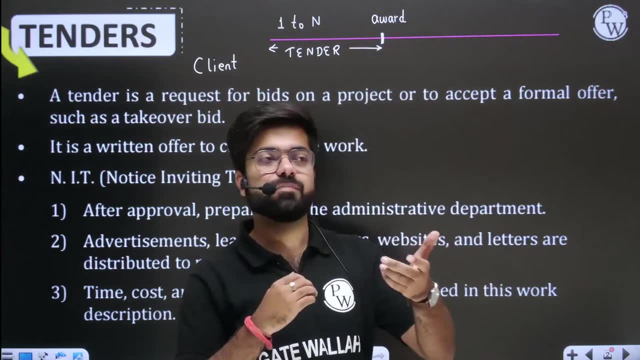 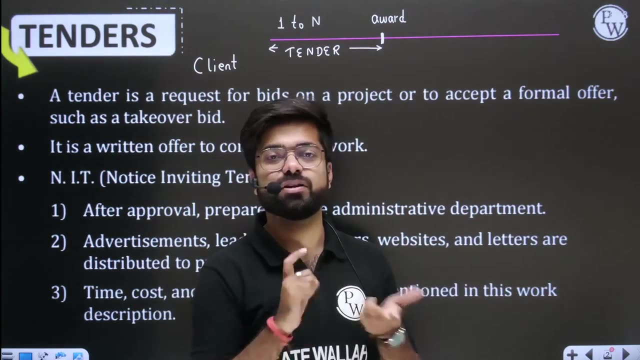 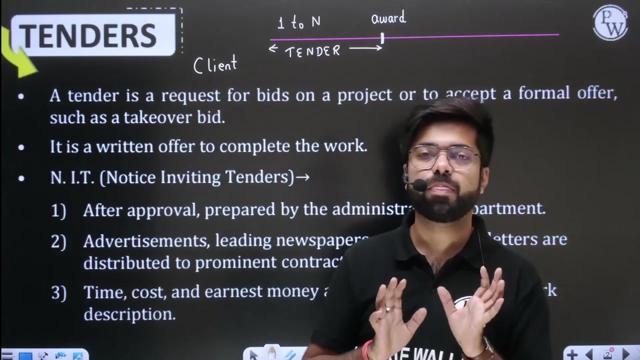 Tell me quickly. there is logic in this. I have to ask you a lot of questions today. you will understand a lot of things. what to say, sir. you can understand that there will be no FIR here. nothing will happen. this is an agreement. we talked to our aunty. she said: we will do this. we said: okay, we will give you so much money. the deal is over. this agreement happened, any sort. I mean, if there is a discussion of any form and deals are fixed in it that this should happen, then it will be an agreement. there is no law involved in it. it is not that we did not give money to aunty. 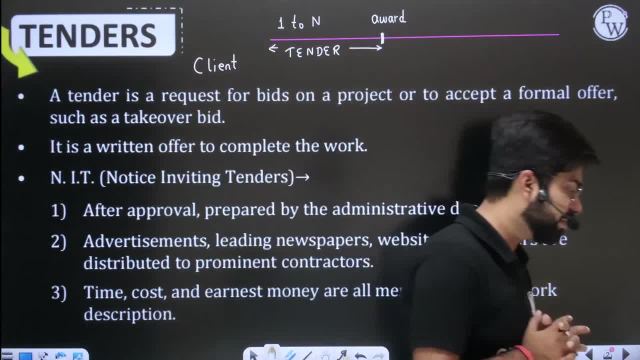 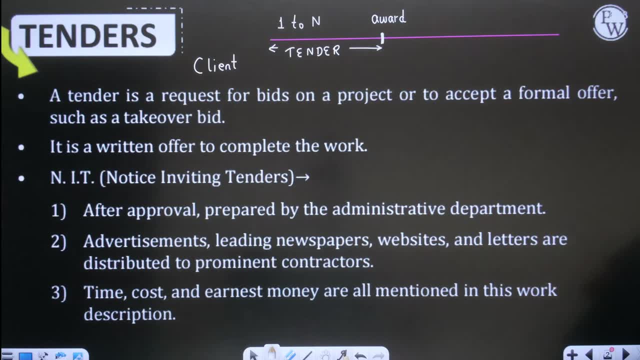 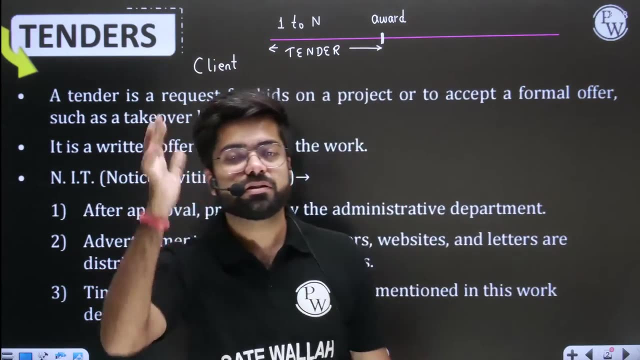 aunty ran, so we both will go to jail. there is no such thing. there is no meaning here. so what is this? Yeah, yes, Okay, if we are here, then what is right then? this means here, this agreement has been made not enforced by law. now, what is a contract? now, a contract is for big works small. 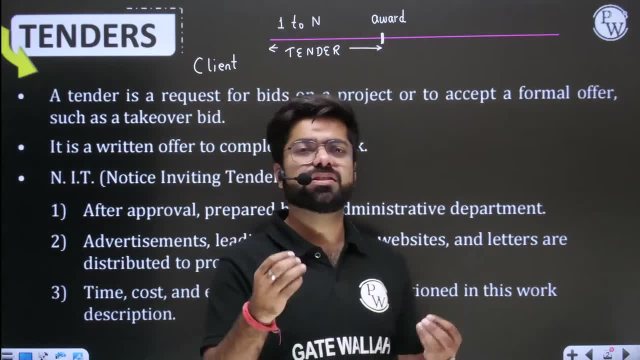 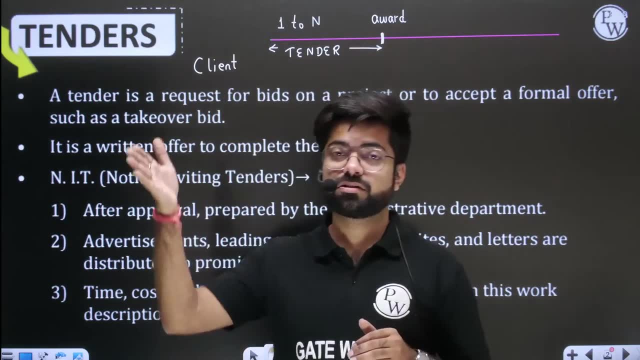 big works. let's assume you are building a house comes you took the refer in your agreement. now what has happened in contract is that both parties should don't live in the same house, has signed it in a good way, being a witness to whom the law is on the stamp paper then. 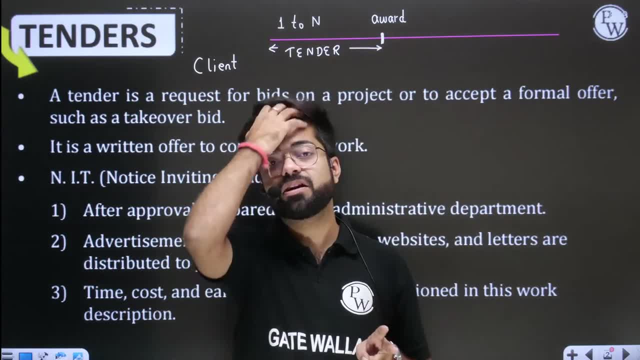 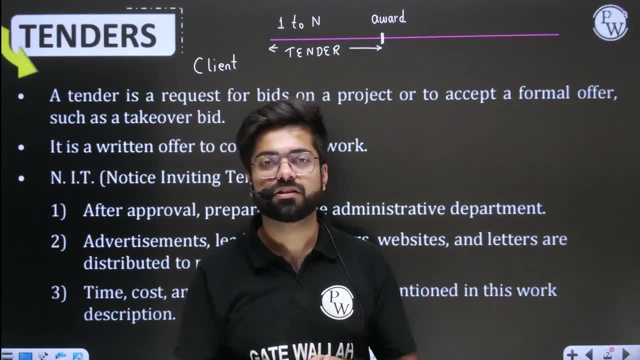 when it is signed. what is there in it? that if we move back from our terms and conditions, then the law will come in between. then we can take some jail or something that is serious action can be taken. then that is the contract. then there is only one difference between the contract and the agreement. 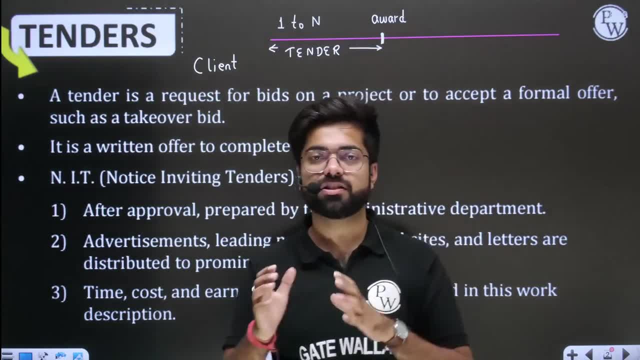 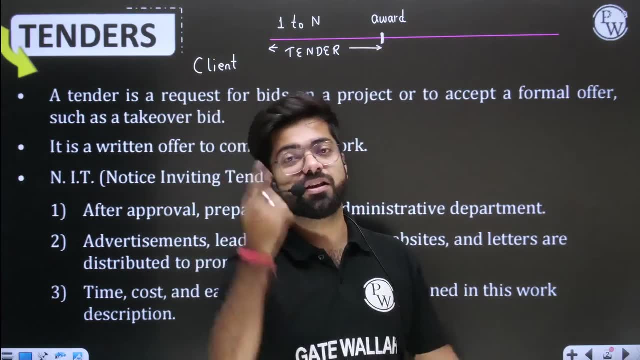 agreement and contract are the same thing. the terms and conditions will be that you will do this, we will do this, we will give you money. we swear you do this work. do as I tell you. don't start doing anything from your mind. 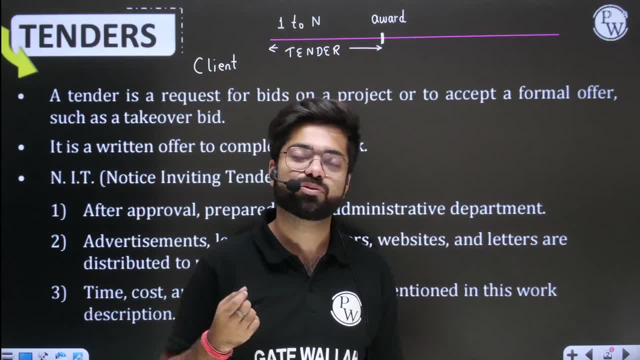 you know, if you had to put it separately, then five of them disappeared. you sold it to him. this also happens. that is such an incident, we tell you. such an incident is that when you are standing in front of you, everything is going well. 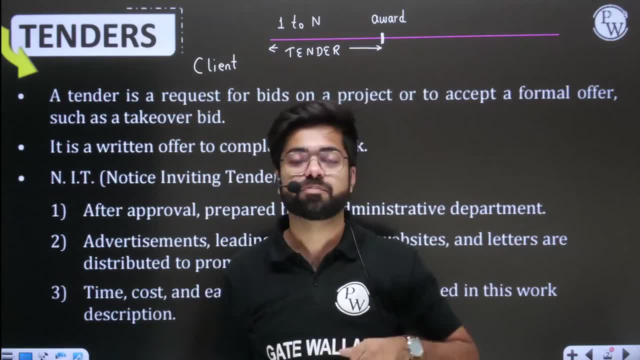 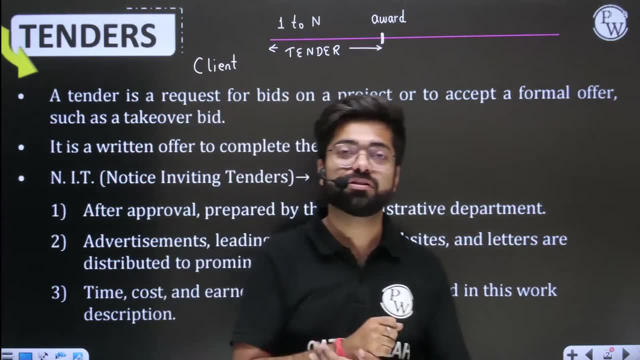 as soon as you come out, you put it on, you take it out. you are telling the truth. you put it on, you will dig it out immediately and take it out and then set it back. in this way, so much work is stolen. it is stolen, the use of money is stolen. 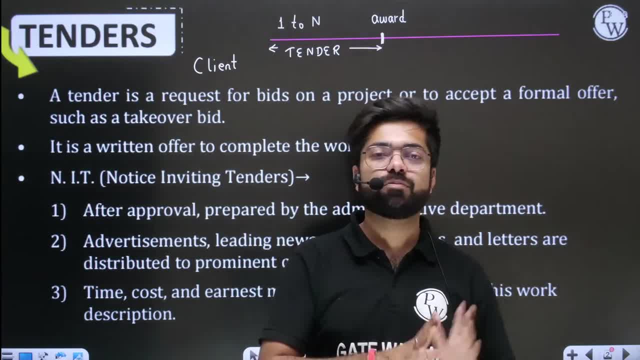 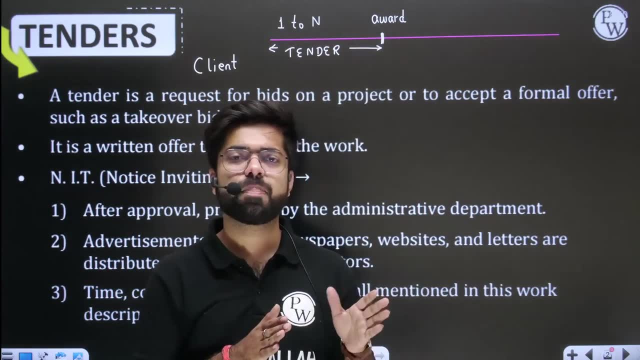 let's leave it for the time being. it is a secondary thing. so work is going well. they want client and when they get the money they want that, the work of the two people will go on. okay, then I hope you will understand. it has legal binding in the contract. you can take action legally. 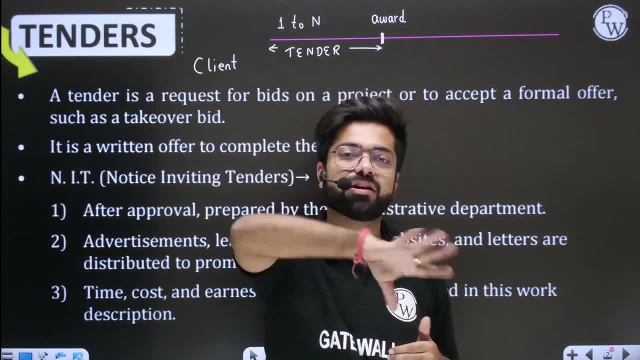 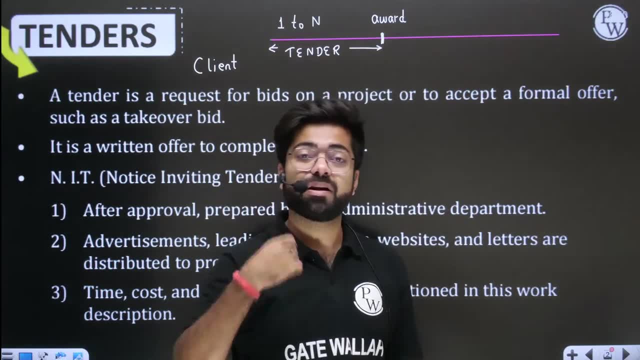 if things are not done according to you, no one got the money. many contractors do not tell me the government system understand a little. many contractors have made cases in the department, 50 of them. our education is the money, while the department is thinking something else. they don't need money. 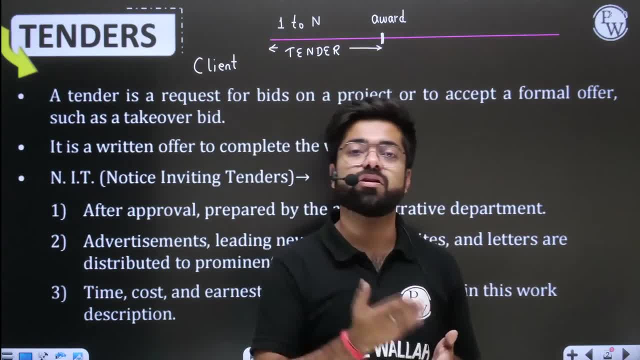 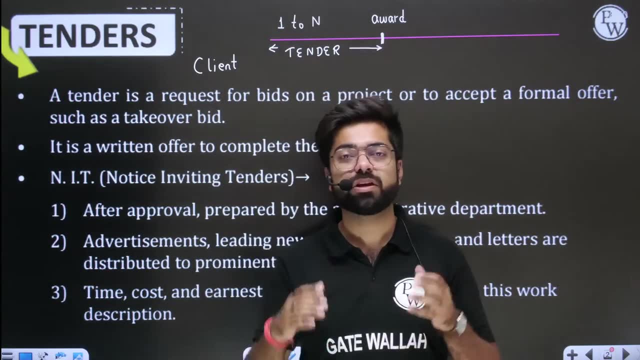 They are saying that they did not give money because the work was not good. Contractors keep fighting and court cases keep going, Because there is a contract. Court case can only happen when there is a contract, When you go to the department, when you become an AE or an AXIAN. 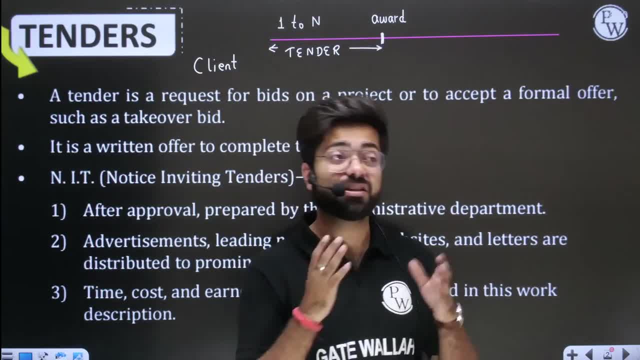 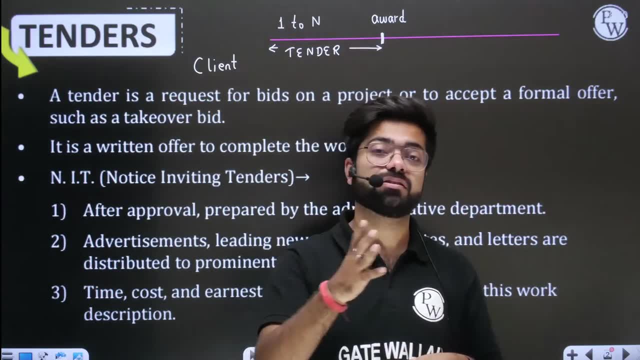 AE means assistant engineer, junior engineer. if you become anything, then you will see how many cases are going on. The contractor keeps doing the case every day. Every day, the executive engineer has to go to the court and explain that it is not like this. 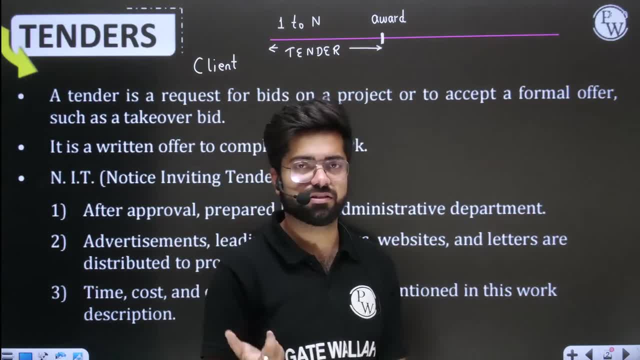 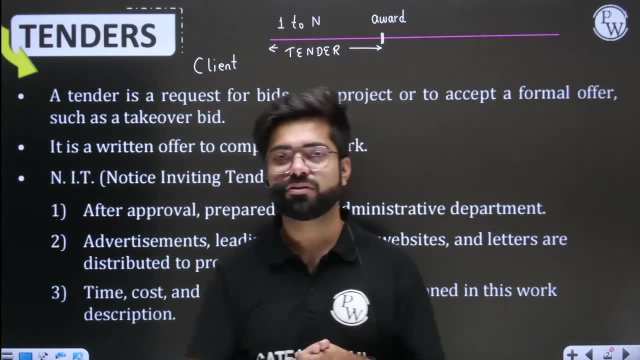 That is, you have to submit the papers. A lot of procedures keep going on Because there is a fight going on In the contract. whatever is written, it is discussed with each other. There is a fight going on. If you go to the department, you will understand everything. 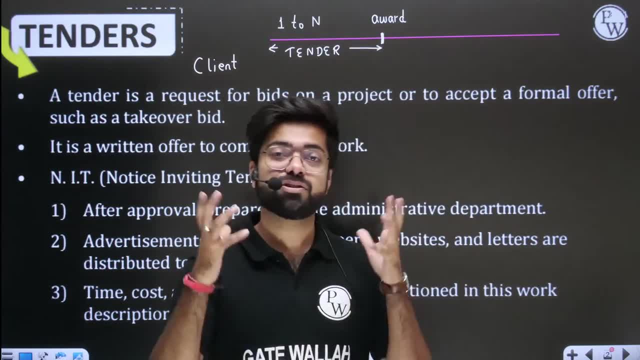 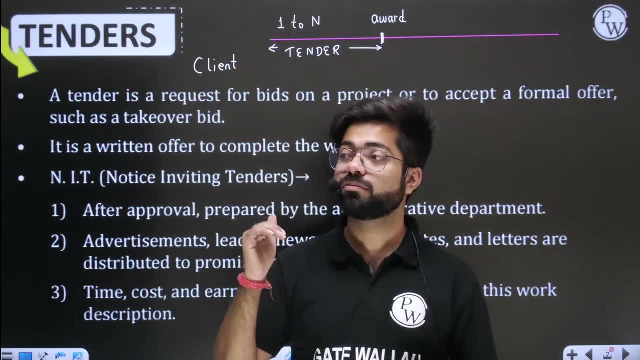 There are a lot of things, So you must be thinking that if you become an AE, your life will be very good Means you will have to learn a lot of things. What are the court cases? You have to do the paperwork every day. 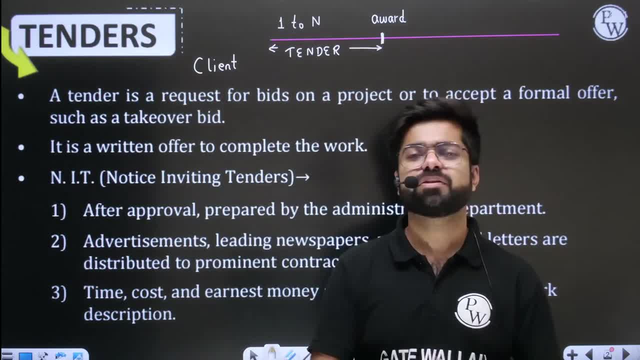 Means. when the days will come, the dates will come, then you will have to go. There are a lot of problems, So we hope that all three of you have understood the difference. Have you understood the difference? Tell everyone what a tender is. 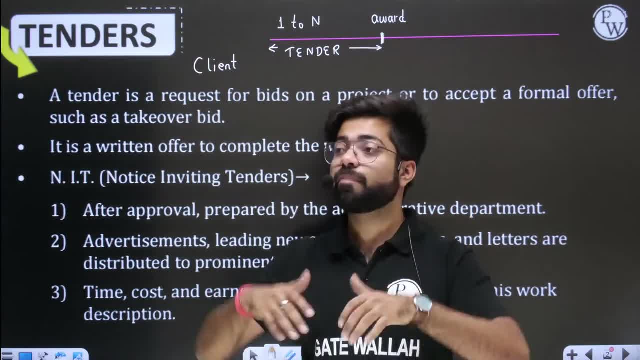 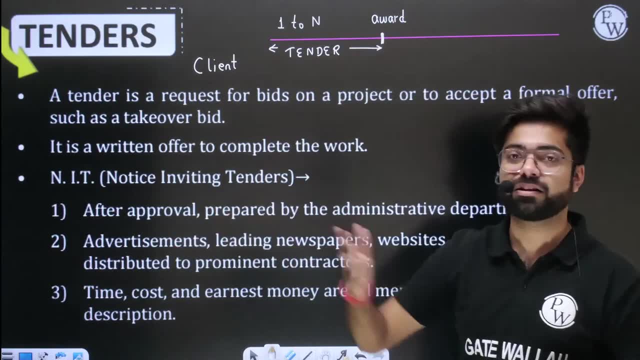 Tender means: if you are asked a tender today, what will you tell? Proposal: I will also do this work, sir. I also have to get married. This proposal is called a bid. We are applying our will. We have to tell the department that we will make a canal. 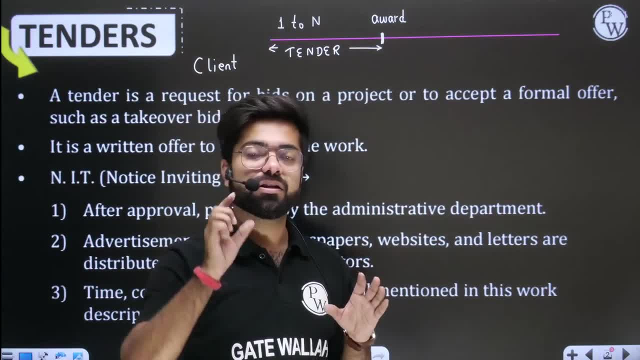 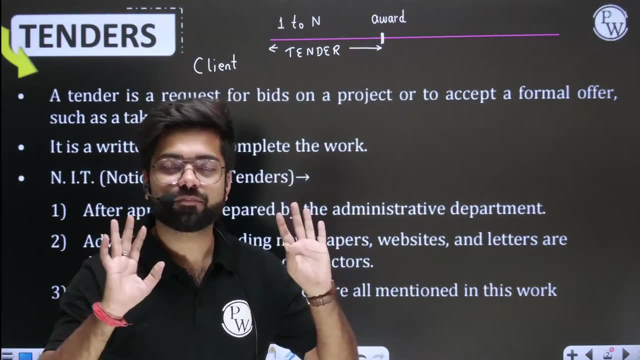 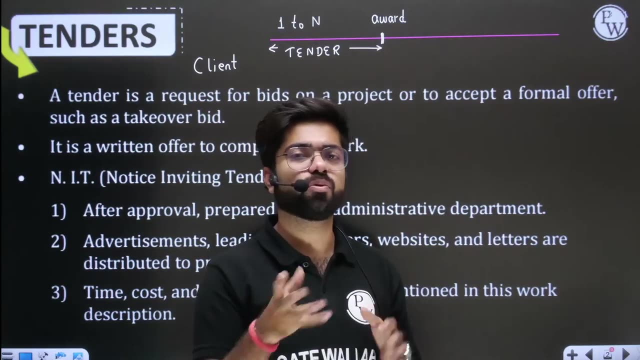 Okay, This is the proposal. Tender is done. When a person gets a tender, what will happen after that? There will be an agreement or a contract. Did you understand this too? No problem, In agreement, sir. if you go back a little, then there can be no court case or anything. 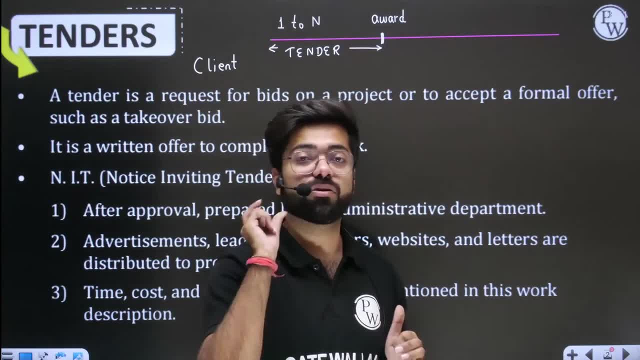 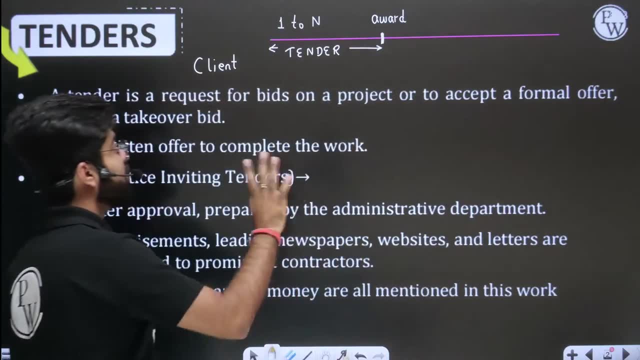 Or police action, etc. All this cannot happen. But if there is a contract, then you are legally bound, Then there will be a date. Slowly you will understand it. So there is only this difference. So you hope Now what will happen after awarding. 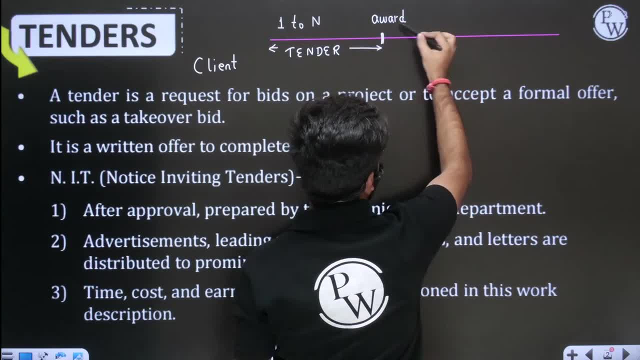 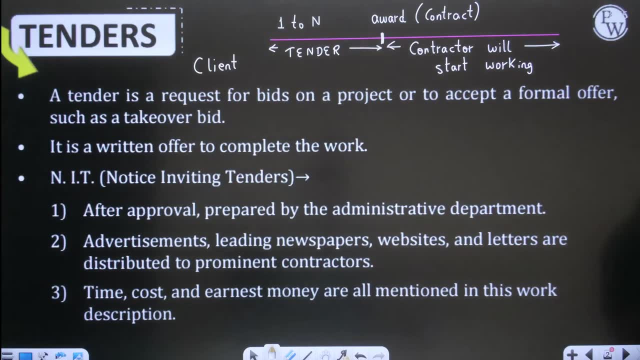 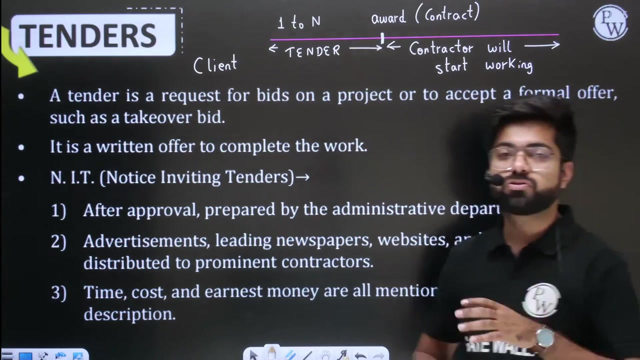 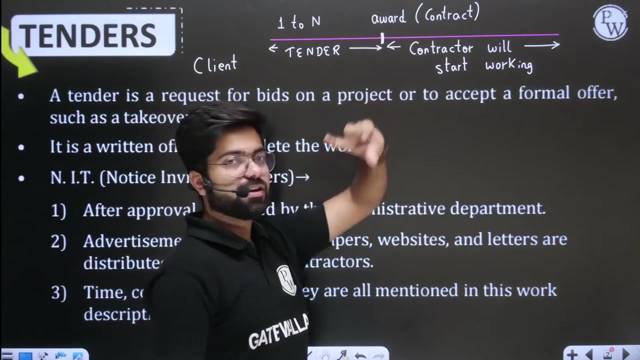 Here the contract will be with the contractor. There is an award here. What will happen here? Okay, Now you can see that the net has been broken down, so we were telling you that the contractor will be finalized from here. whoever will have to get the tender, the contractor will. 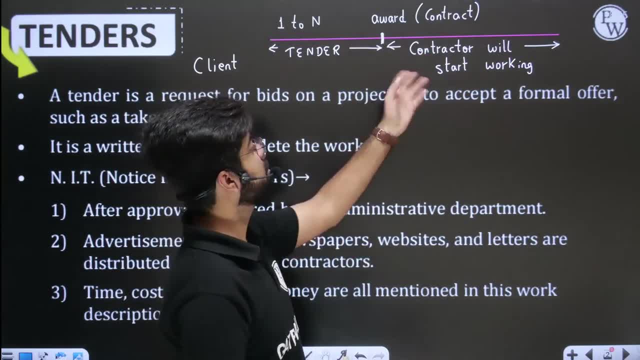 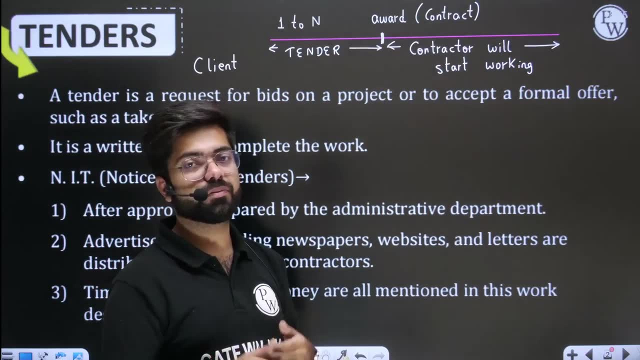 award it and will contract with it. the document will be set properly and the contractor will start working. as it will continue to work, it will continue to work. it will give its bill to the department. the department will do the payment of the bill from time to time. 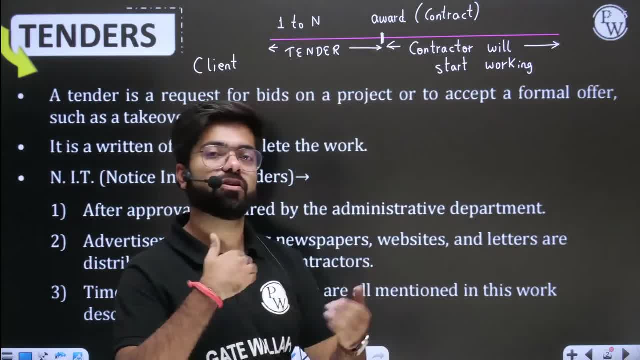 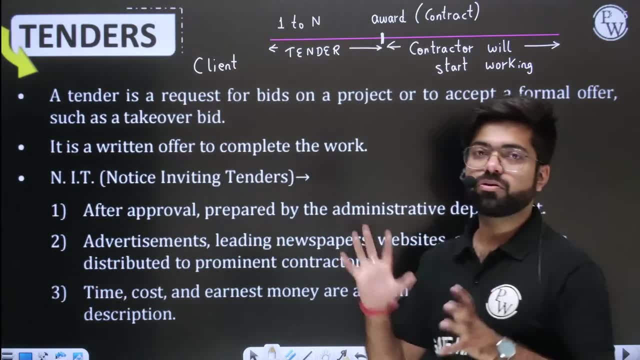 it will continue to work, it will take the payment, it will work with that money and it will get the final payment. so they are called running will. they are called running will. so now, everything will be fine. now we will start moving forward one by one. 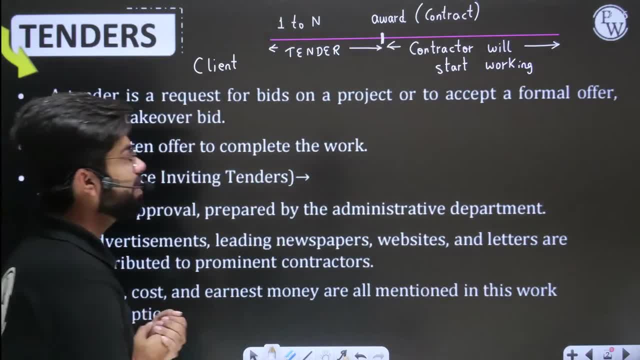 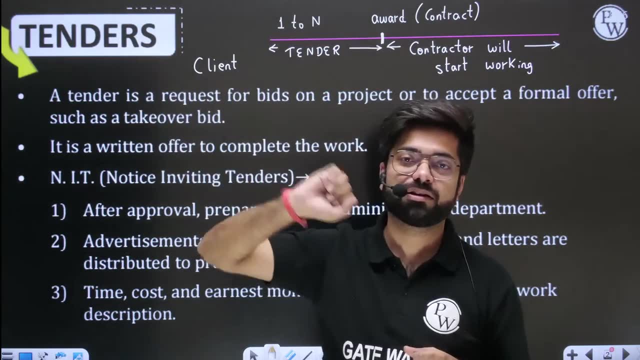 it is very simple, it is not very tough. so we were telling you about the tender. what happened to the tender? someone asked you about the tender. simple proposal that we will marry. What did you say? We will work. many people have said, but in that we will choose the best according to. 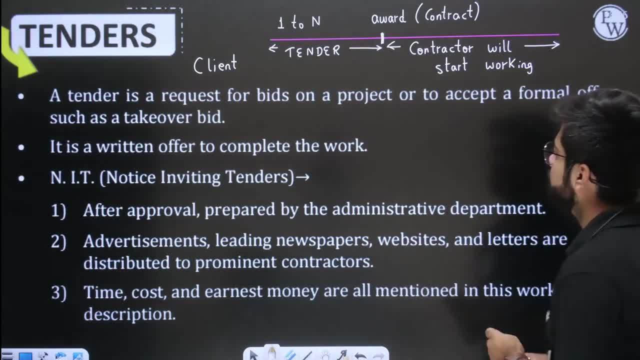 us whatever the client wants. so, in short, there are two people here, two people: one is your client, one is your client and the other party is the contractor. one is the client, the other is the contractor. and what happens in between them, sir? the legal terms. 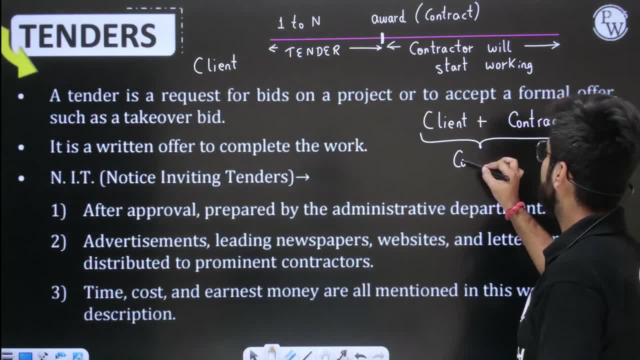 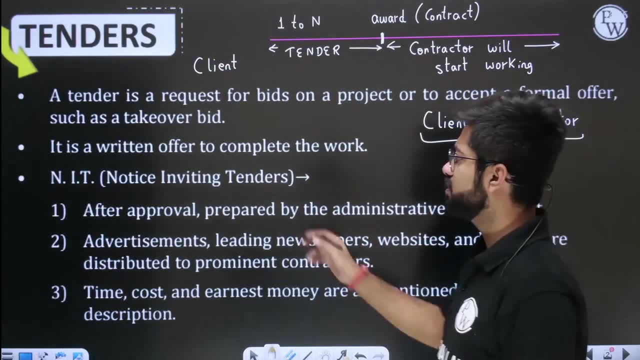 are signed, the legal terms are signed between them. we call them contract. after the contract is signed, the work starts moving forward. so this is simple, so simply. just a tender means one. what can be said in the tender form? there is a simple offer. there is a simple. 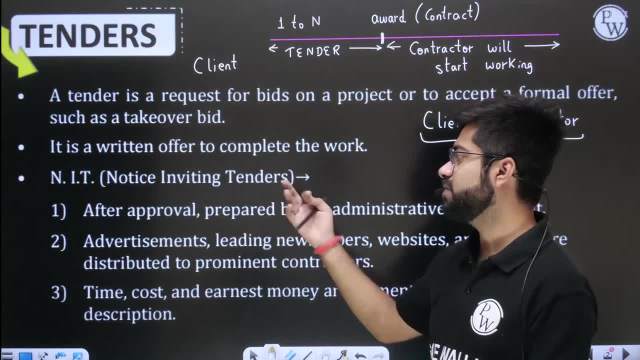 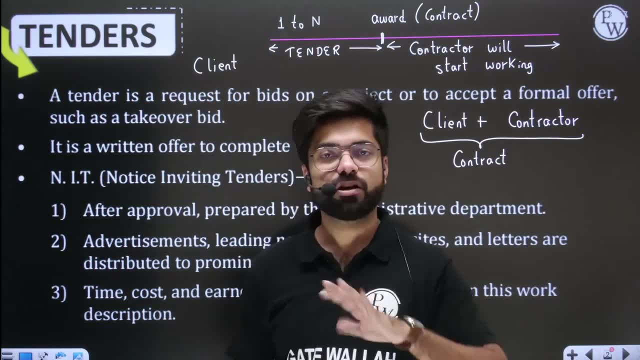 offer whoever wants to come come. then the notice inviting tender comes out. and after that, how does the notice inviting tender come out first? first of all, the department will do all its homework. first of all, it will do all its homework. and when the administration 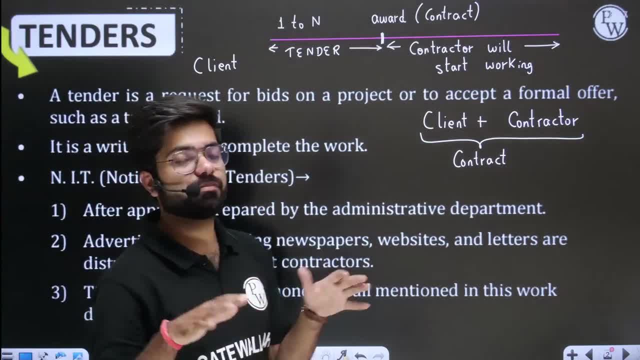 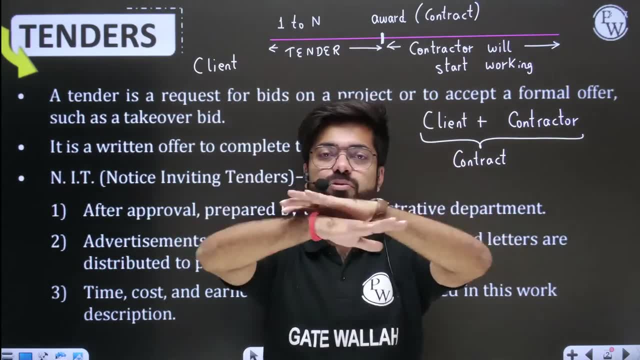 approval is obtained. what does the administrative approval mean? whatever all the departments are like, if we talk about UP, it is a state. okay, who is above all CM? there are many ministers under the CM, there are full cabinet ministers and there is a department. 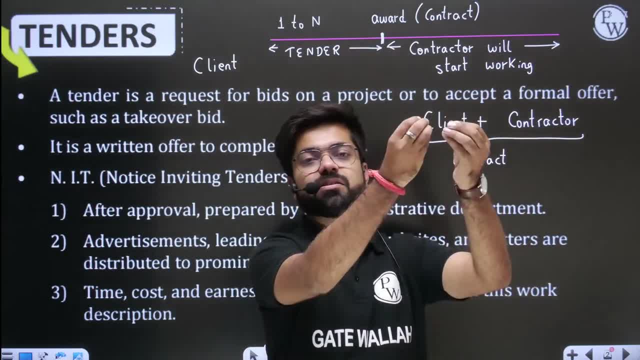 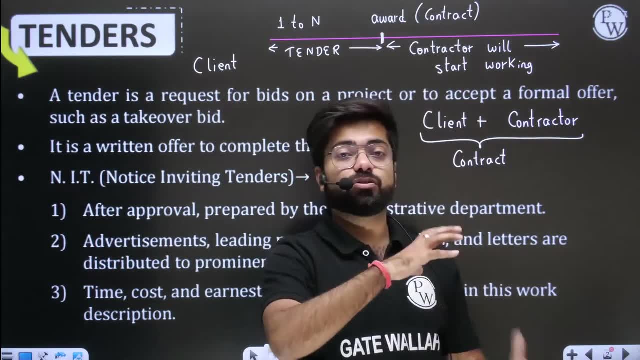 under each minister. that brother, this is the secretary minister. this is the PWD minister, this is the minister. that means everyone gets some department. now there is the administration under the minister. okay, there are many people in the administration. okay, they are all. 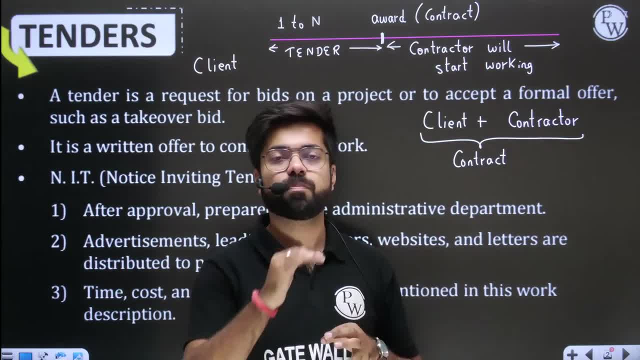 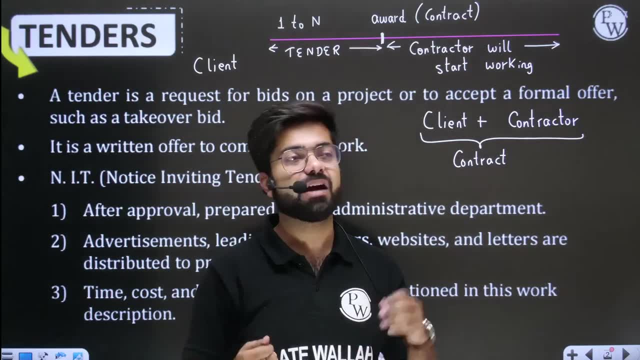 people of the secretary level. okay, there are many people, so they all need permission. the department needs people to work. this is what is going on in today's time. okay, so the administration people give approval that, yes, brother, this canal, this dam should. 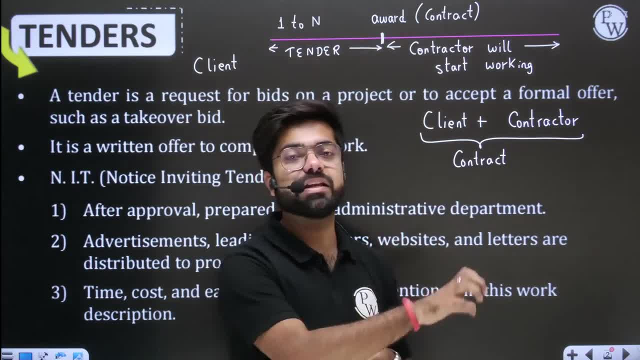 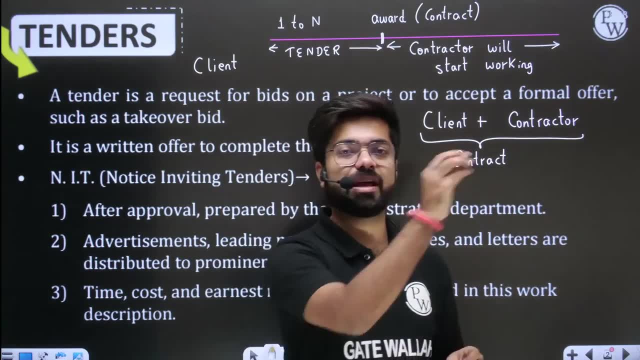 be built. the department first comes to the proposal that, brother, there is a need for this if such a work will be done this year. so much budget has come. there is a budget of 8000 crores, out of which we will put 1000 crores in the dam. then the administration will. 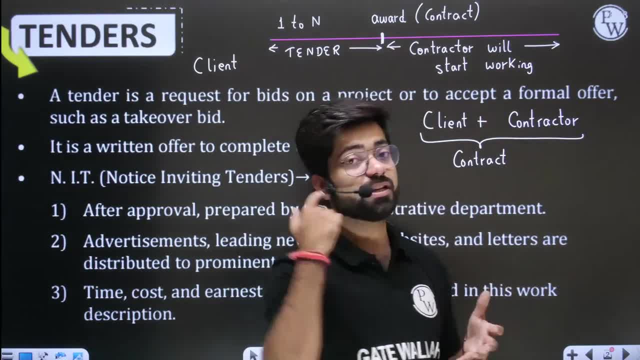 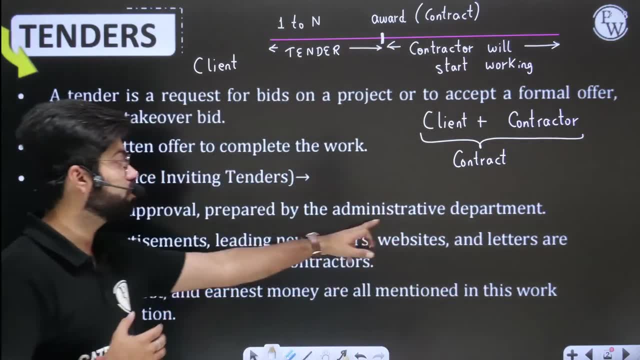 check that thing. okay, you first submit the whole report, the administration will check it. it will be approved that. yes, brother, it is necessary. you have written everything correctly here. the dam should be built then it is called administrative approval then. 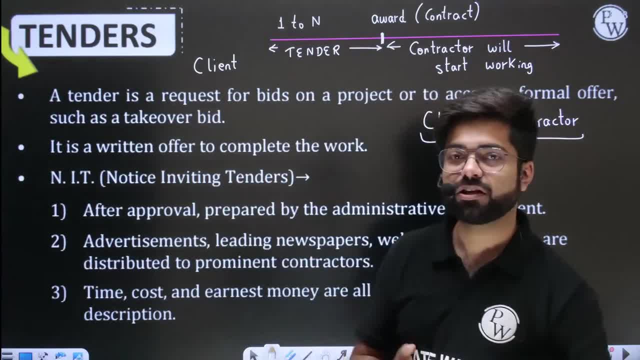 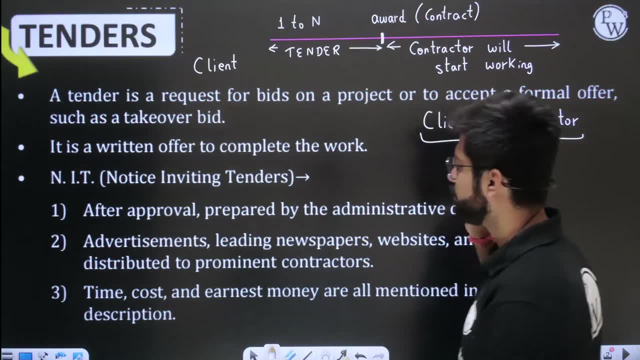 the administration has given approval here. when it will give approval, then a whole notice inviting tender will be advertised. okay, then it will be advertised and the world will reach the place. at least a small project. then at least two new superheroes came out. 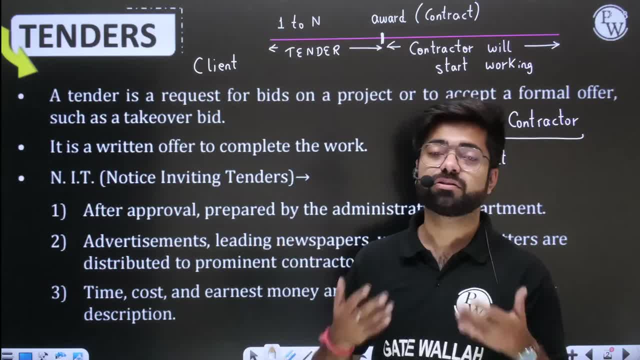 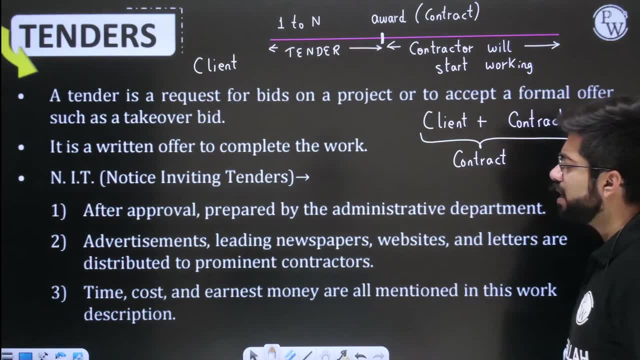 it is a big project, then it should be done at a very large scale. it should be promoted, okay, so that everyone can be involved in it. and after that, whatever you are advertising here, you should give the description of the time cost, earnest money. all these. 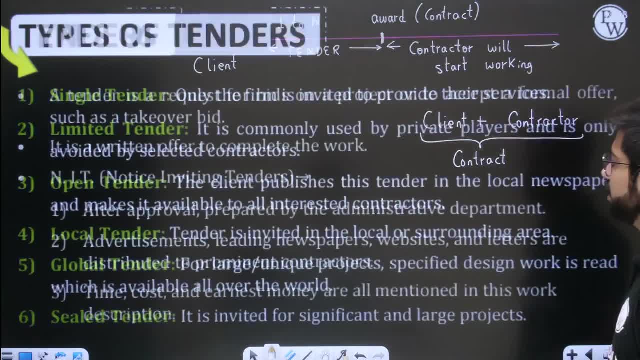 things. okay, the NIT is done. now the tender has been done. now the tender has been done. okay, now the tender has been done. now the tender has been done. now the tender has been done. so what is the kind of tender and the tourist is in the notice surpassing? 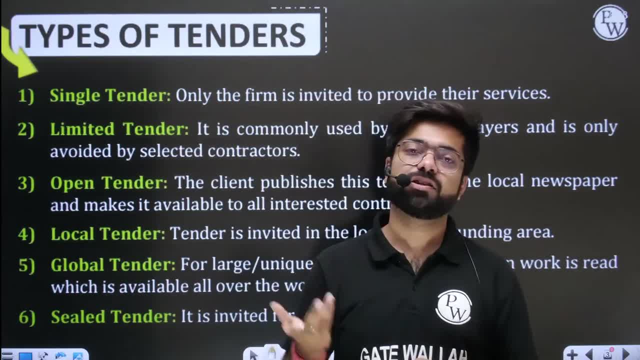 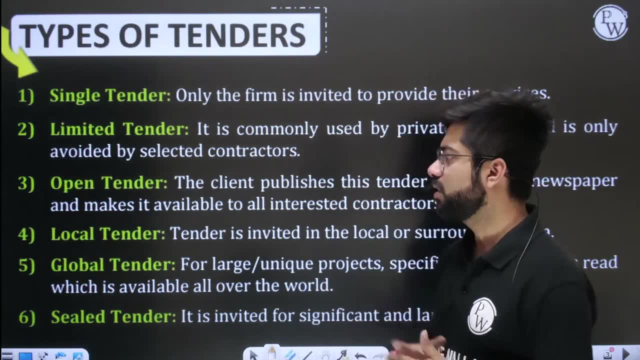 that everyone will start getting the date format in these days. we told you to know the tender. we will not be able to tell what the ticket is, where it will come out. you can see that, okay, but the people who are active are online these days. 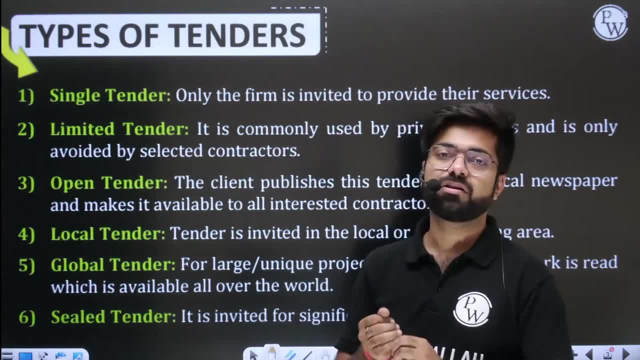 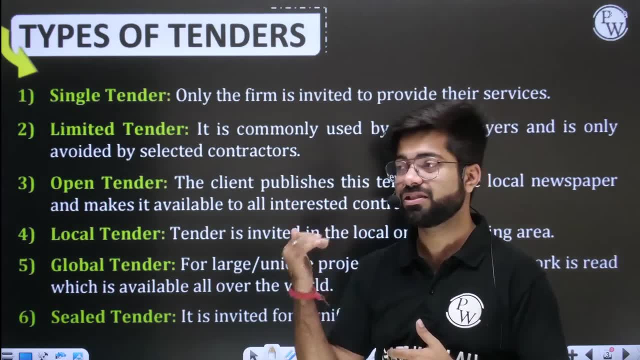 no matter what was happening. earlier there was a lot of money. we used to give money to the changed e-tender for the same. now it starts to worry about the occasion because it is online. the online is the only favor. online don't. 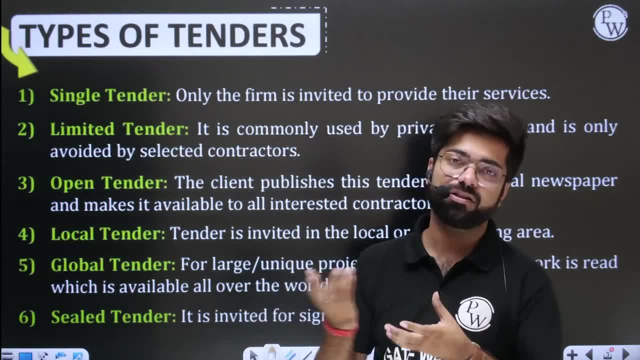 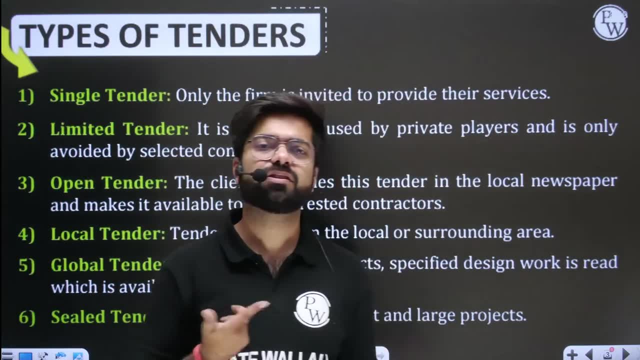 How can anything happen online? You have to fill the form online. there will be no money given right, So things are very less. transparency is very good. Why does the government do tender? Can anyone tell What is the need to make so much mess? 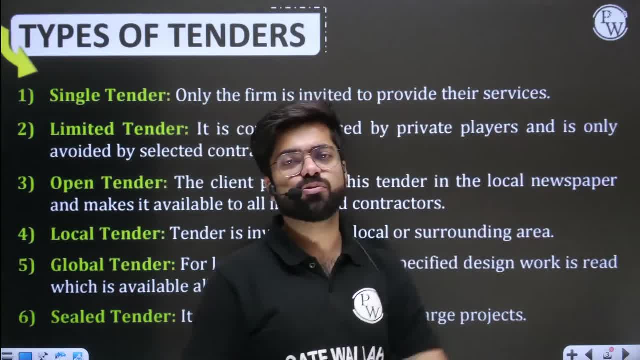 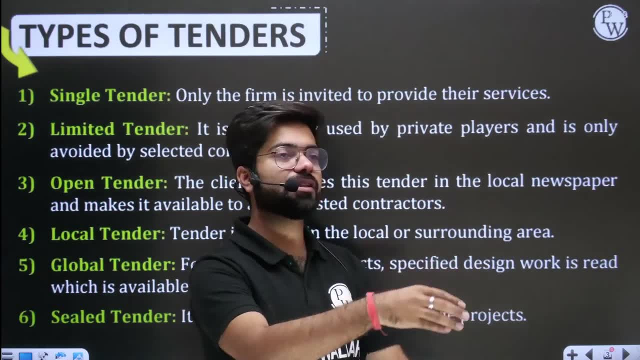 We know you, these are Shamsher. they dig their canal well, they clean the silt on the canal. they catch them right. They build a good road right. They light the lights on the road- well, they give them work. 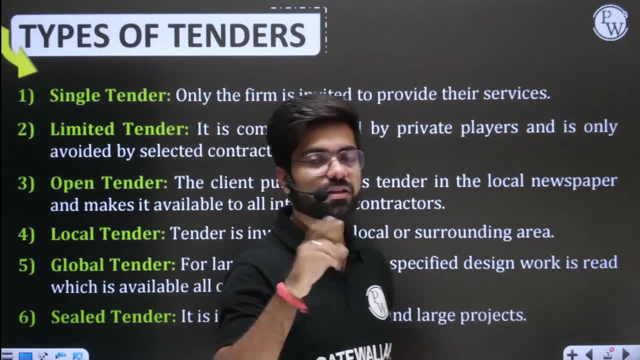 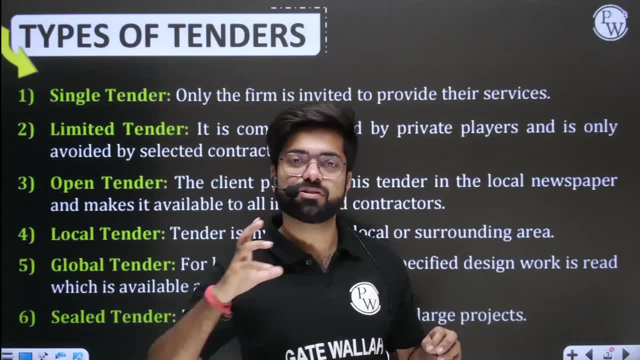 So why is there so much mess? Can anyone tell? Why is there so much mess? First, the approval comes from the government. the government checks whether the department is complying or not. whether it is complying or not, the road is being built. 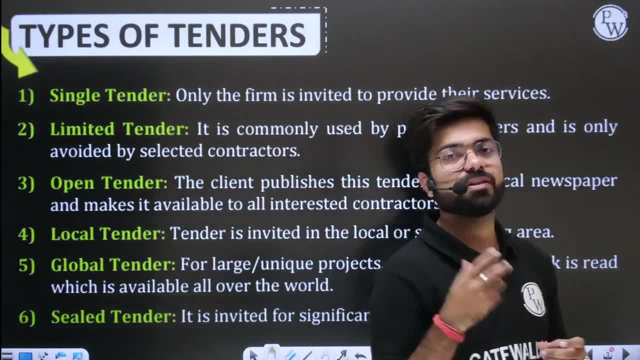 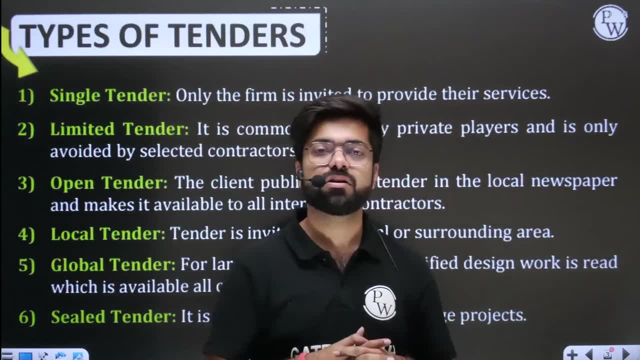 There is checking at a different level, right. So when there is such a level of checking, the work comes out very well and what is necessary? only that happens Now. so much mess is being done because, look, the money of the government is a lot of hard work. 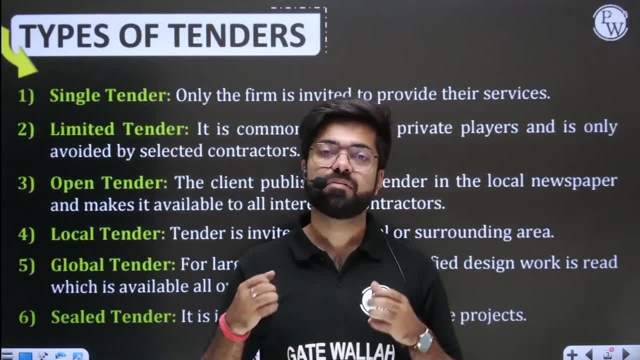 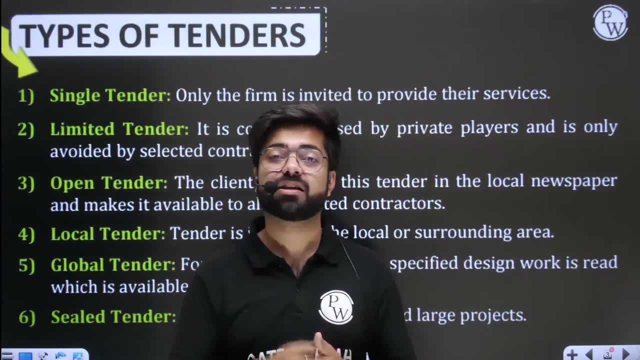 it is the money of people, it is the money of taxpayers. We work hard to earn some of it. the entire service sector, or whatever goods and services we buy, we give to all of them. We pay tax, income tax, that is, we pay tax of 50 rupees. 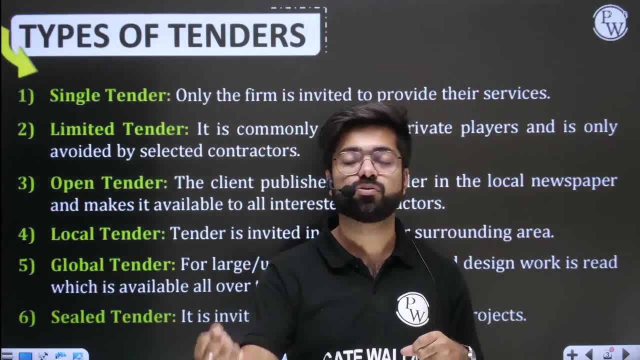 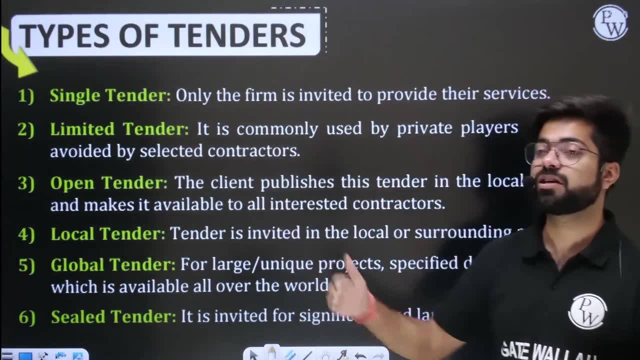 Now that money is very important money to utilize it properly, to use it properly so that no one comes to waste your useless money right. That's why so much fair process is done, so much competition is done among the people, that everyone fill the form. everyone fill the form. 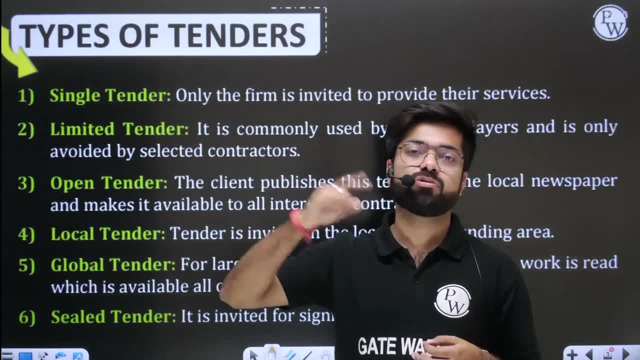 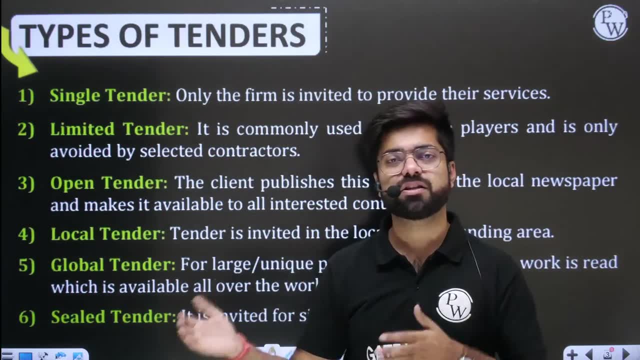 which will be the best, we will pick it up. we will pick it up and work with it so that the money of the public is used in the right way. transparency is used right Now. that is a different thing. there is a lot of competition. 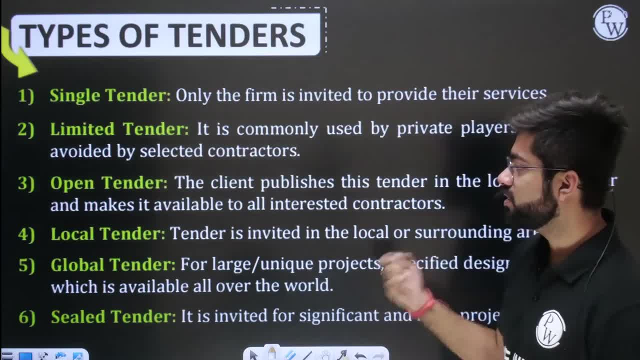 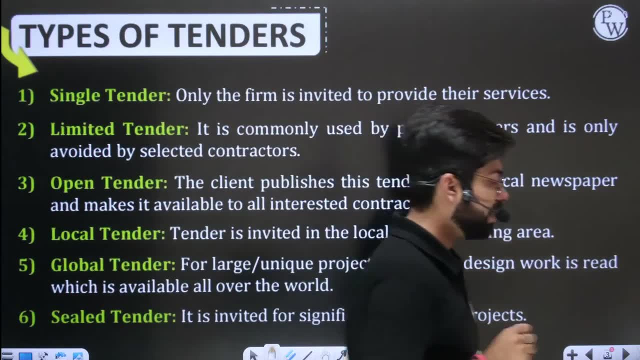 there is a lot of leakage of money. that is a different picture, but the effort is made to use the money in a very good way because it is the money of the hard-earned taxpayer. you try to understand this right. I hope you are understanding the thing right. 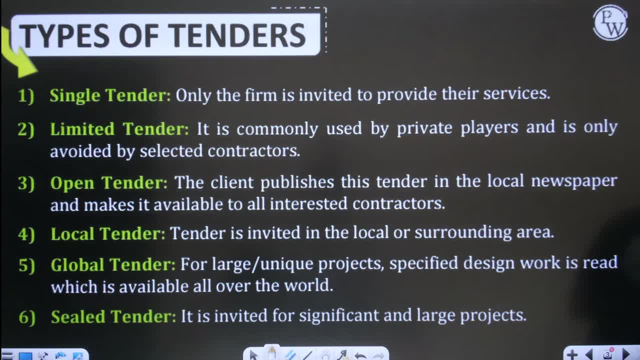 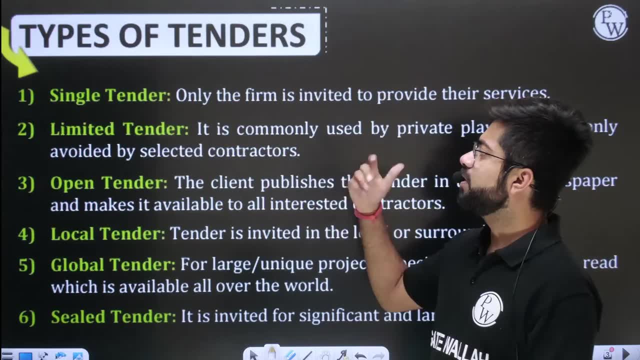 Absolutely, Absolutely. Come on, let's hope that everyone understands everything. Now let's try to understand the tender one by one. what are the different types of tenders like? if we talk about a single tender, then a single tender is very simple. 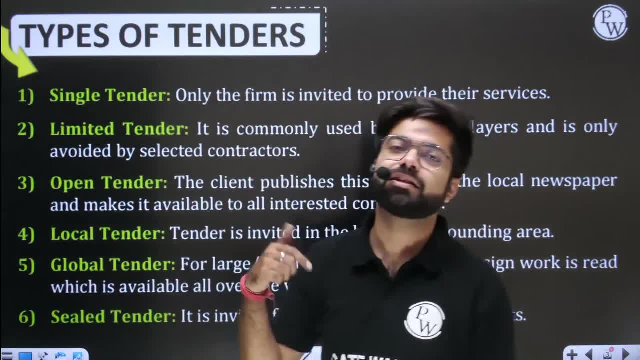 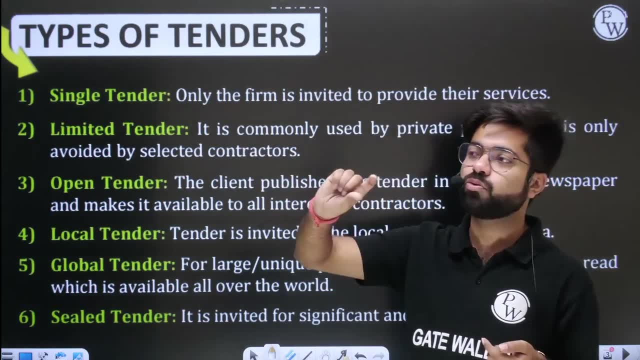 it is called a single tender. only one person has come to get married. there is no option. it is not like that. actually, what is a single tender? it happens when we have only one firm or there is only one contractor who is always doing this work. 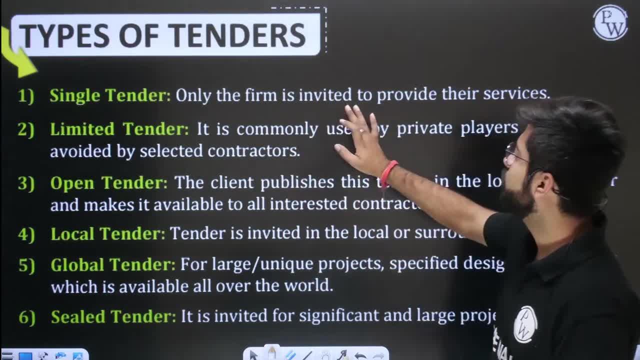 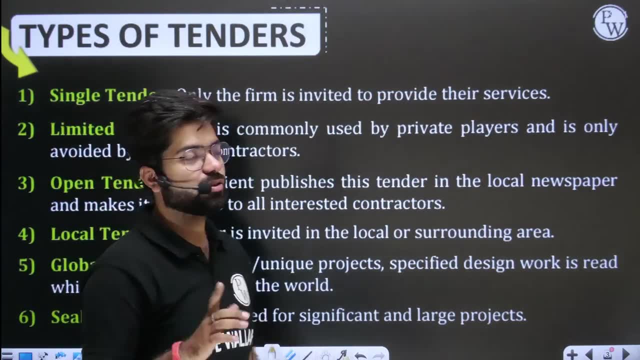 always normally so. if that firm has been invited here only because of this, because he is very competent, he is very experienced, then it will be a single tender right. So here it is written that only one firm, only the firm, is invited to provide the services. 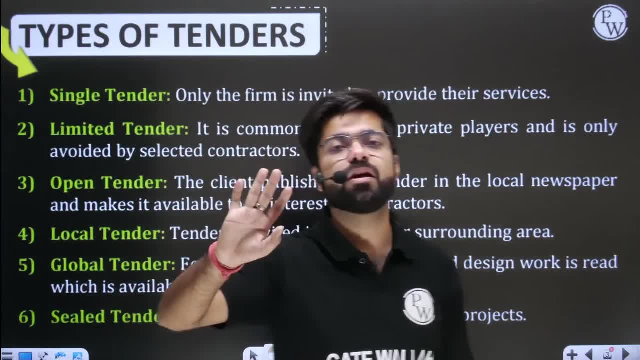 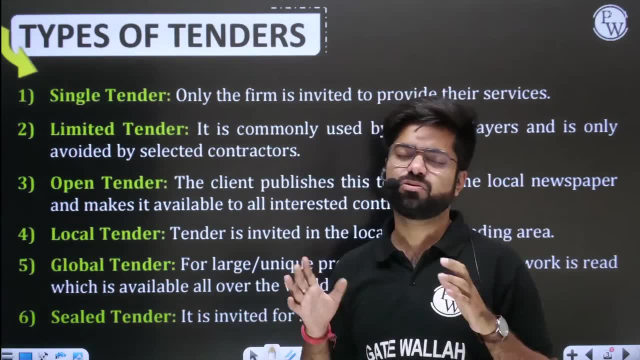 only he is invited. we do not invite the rest we do not mean it. now the example of this: as I told you, the metro that is generally made. you will see the metro now there are a lot of companies. first you will see that. 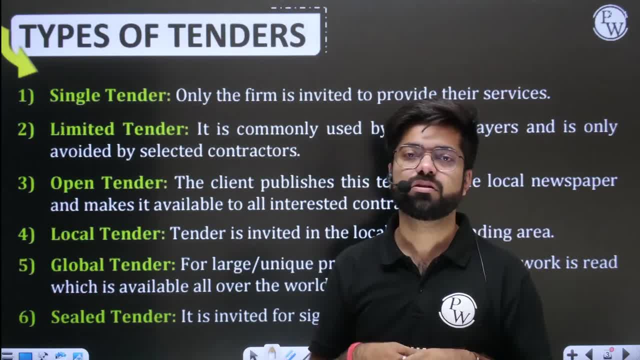 the whole work of the metro was done by L&T. you know L&T Larsen Turo right Shahpurji Pallonji. I mean there are a lot of companies of civil, there is Infra, there are many companies. 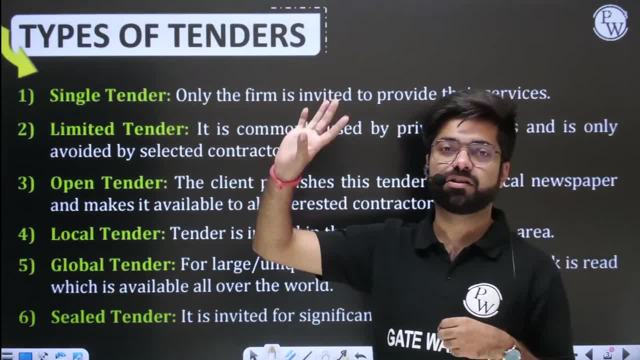 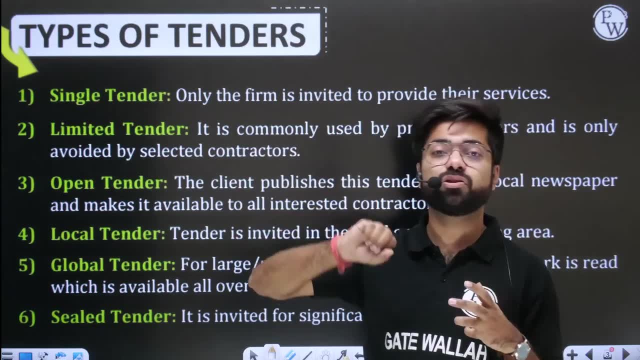 but mostly you will see that the work of the metro, everything was done by L&T, so that firm has done so much. they have done so much quality wise, they have shown so much quality wise, supreme, that they have to get every work. 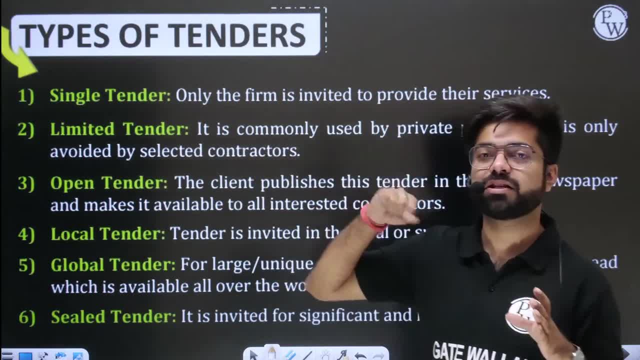 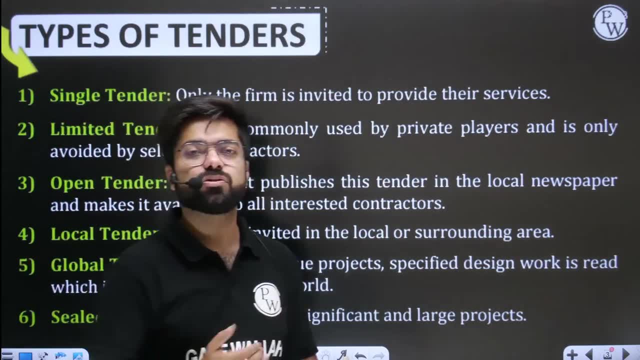 do you understand? Then single tender is done. single tender means we are inviting only one party here. we do not have to wander too much. okay, There is no competition because they have already proved themselves a lot, so every time we will call them. 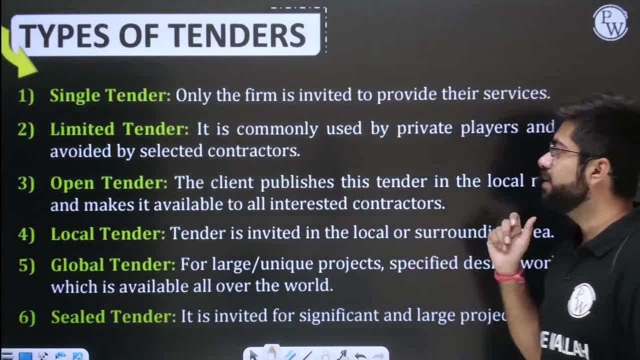 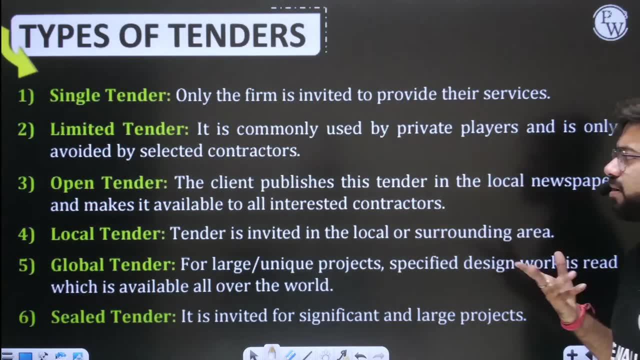 understood, sir. So single tender, then what happened to the limited tender? Look, limited tender obviously what is used by the private players, government, government bodies generally. do your open tender, government bodies, limited tender? they do not do that. 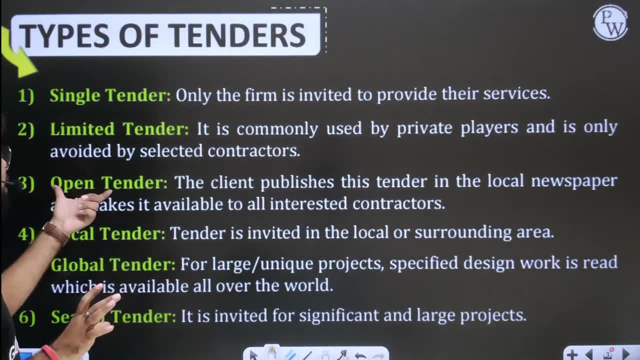 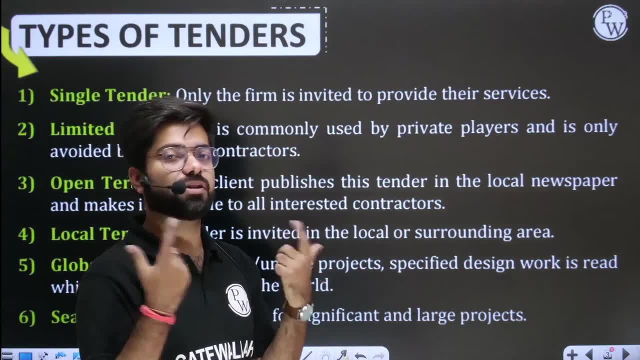 okay, Open tender- limited tender is the opposite of each other, because look what is in open tender that every person can come, open to all. you also come, you also come, everyone come to work, everyone come and we will choose the best one. 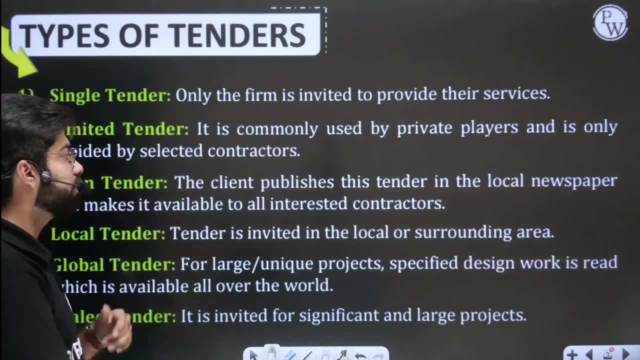 okay, What is in open tender? that the client who has to work? he will publish the tender in local newspaper, okay, Or will give advertisement in other places, will give letters to the contractor and will try to get the news to all the interested contractors. 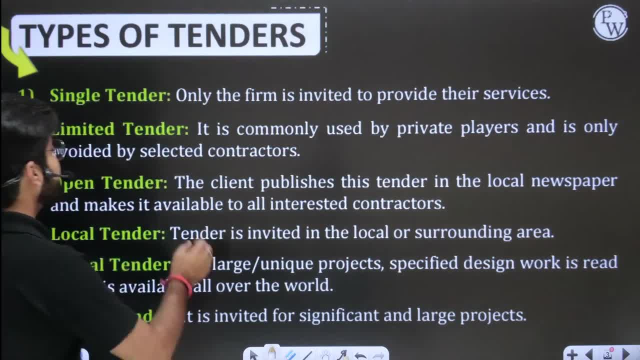 it is open, everyone can come. it is private open tender. open tender can also be done by private. but what is open tender? open tender- you must have seen that in private you don't have to do it. there is a lot of difference. 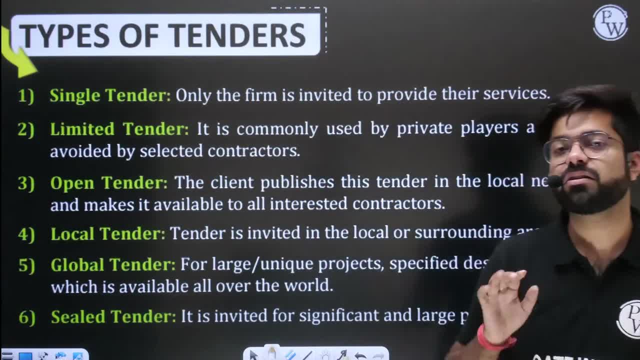 but in limited, because in limited we are choosing only selected contractor. okay, We are choosing the selected contractor, so that is called limited tender. now, limited tender is generally not done by government. government, body or department generally does not do limited tender. 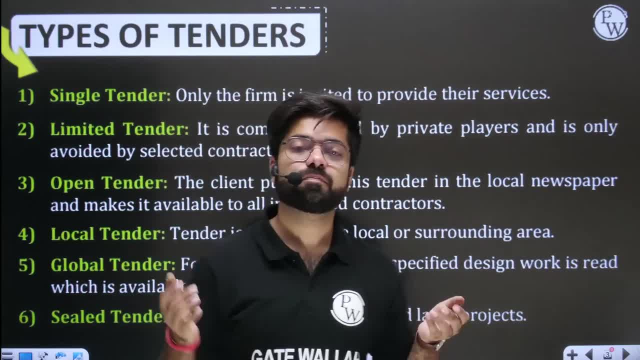 limited tender is done by private players, suppose for example Reliance. or if Jio wants to install tower wall, so Jio wants to install tower wall, so he can also do open tender and he can also do limited tender. 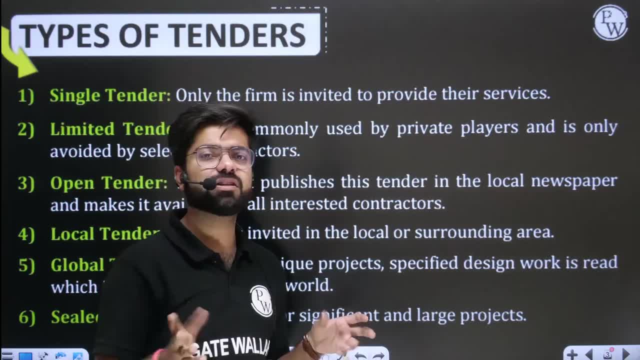 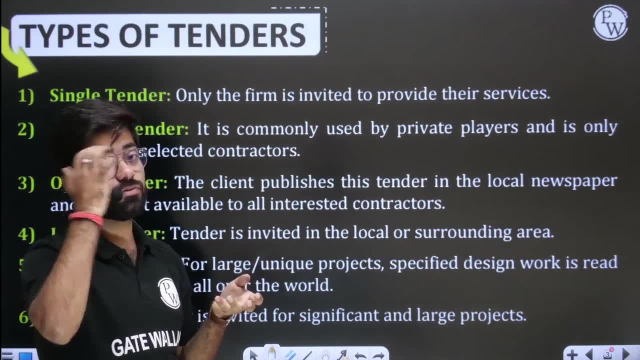 but he is a private player, he knows who works. Fiber line is there, you must be knowing it. OFC Optical Fiber cable is there, So that work is generally given to private players, private companies, to some selected contractors. 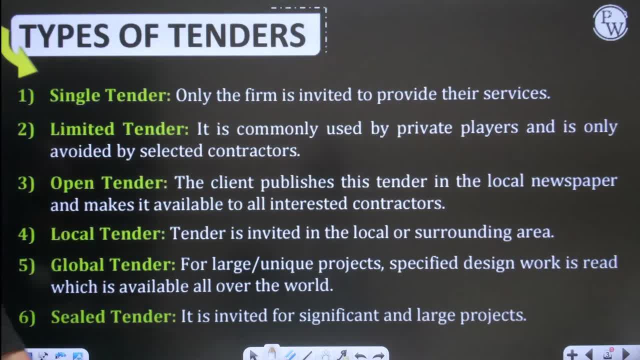 So only limited people participate in it. So when limited people participate- these three people every time, there will be a competition in these three- then limited tender is done. And when it is open to all, everyone can come, then open tender is done. 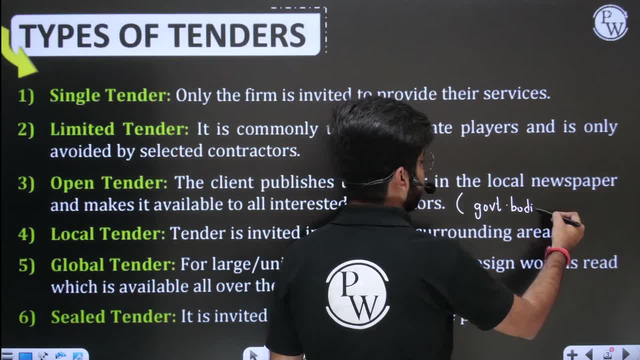 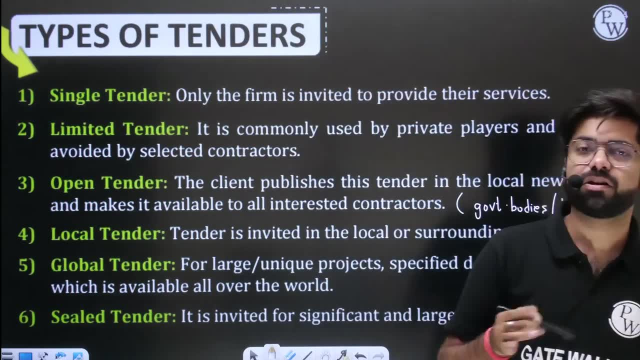 So let's write here: it is preferred by government bodies or department Government bodies or any department. there are many departments: Public Works Department, Education Department, Rural Services Department, this department, that department, there are many. So what is a local tender? 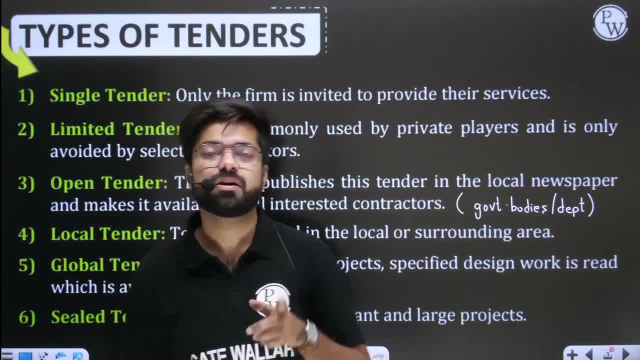 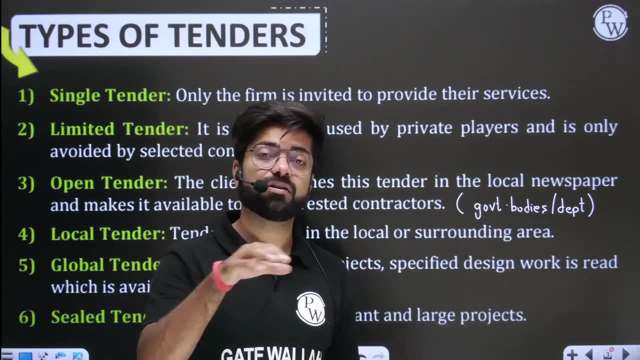 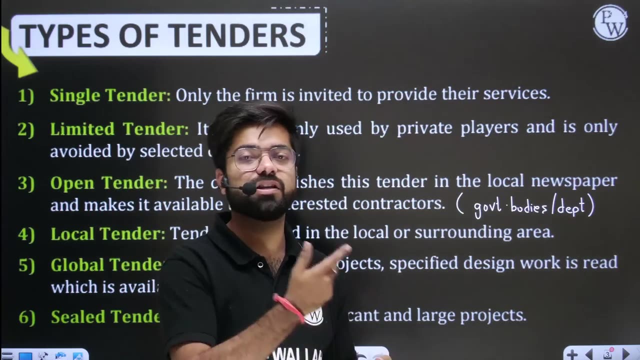 Local tender means in that area, for example. you see there are different districts, there are districts in every district means limited. it is not like there was a field, there was grass and grass and we got to know. 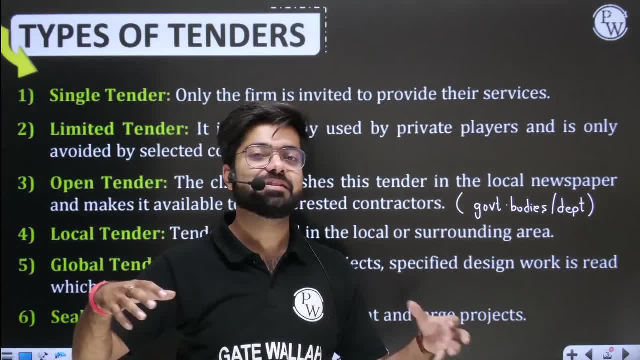 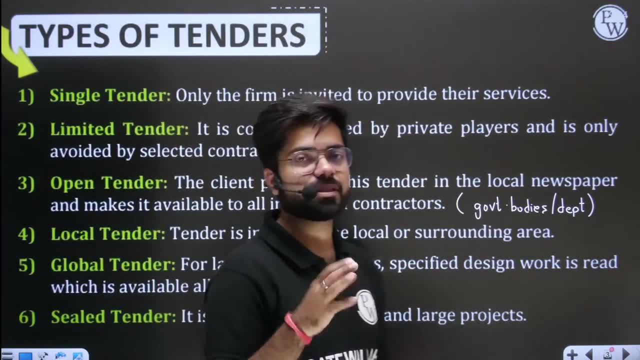 we sent a tender to USA that there is a flight from Germany. JCB will come and the work will be at the level of a banker. if there is a small work then we will give it in the local area. for that we will go abroad. 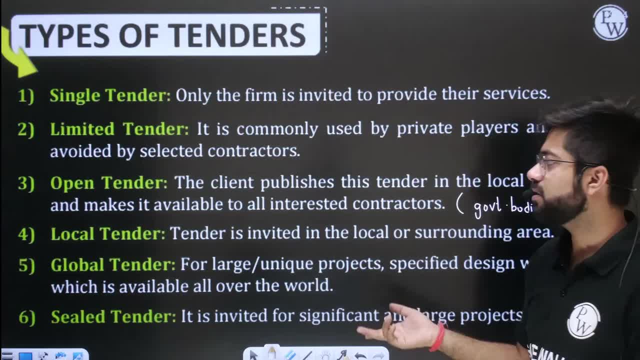 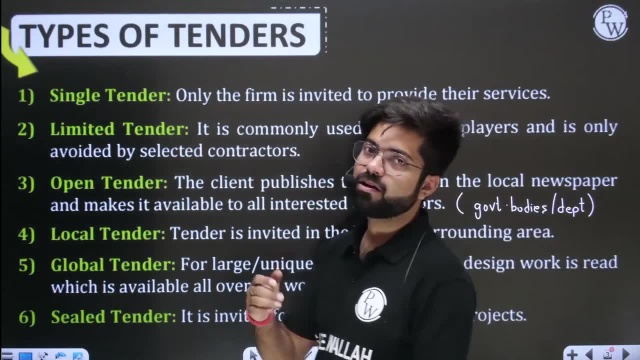 it is a very basic thing. So local tender obviously works. when we get the solution of the work nearby we will get the contractor. So for small works we give tender in the local area, surrounding area, when there is sealed cleaning on the canal. 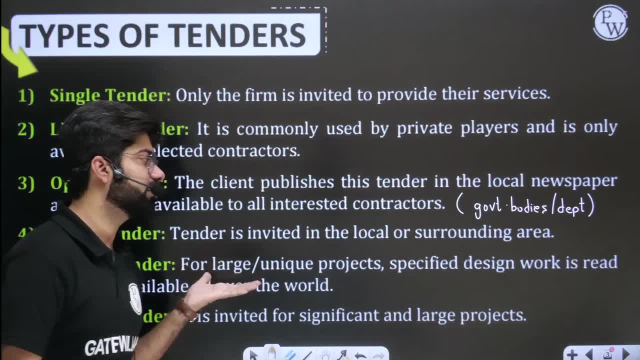 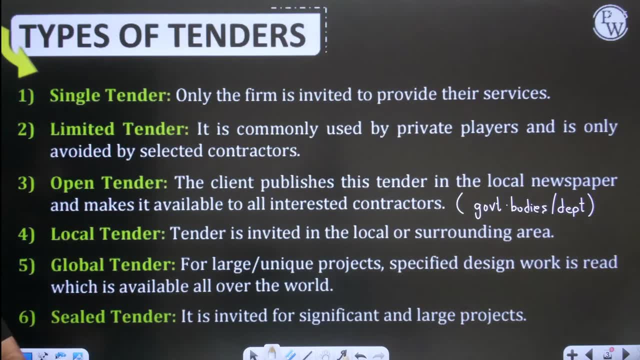 we have seen all this ourselves, so local tender is taken out in that area. the contractor who is expert in this work will be invited to this tender, and very few people participate in this- only 1,, 2,, 3,, 4,. 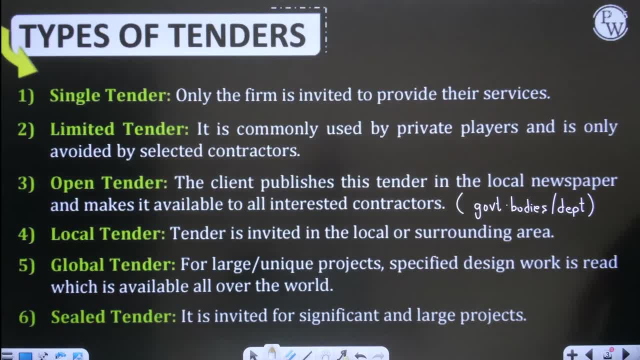 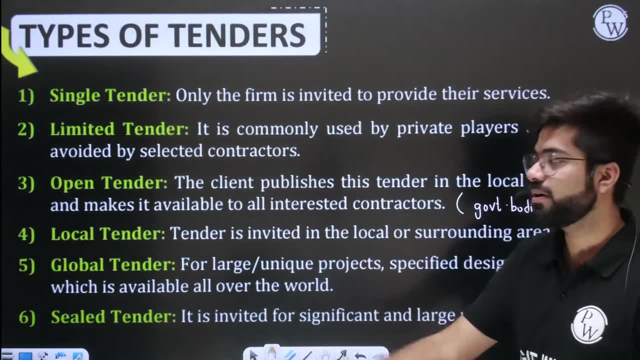 so this is our local tender. Let's go See. everyone has their own advantages and disadvantages. you are saying here that competition will not be good in single tender. transparency will not be good. they have to prove it first, then they get trust. 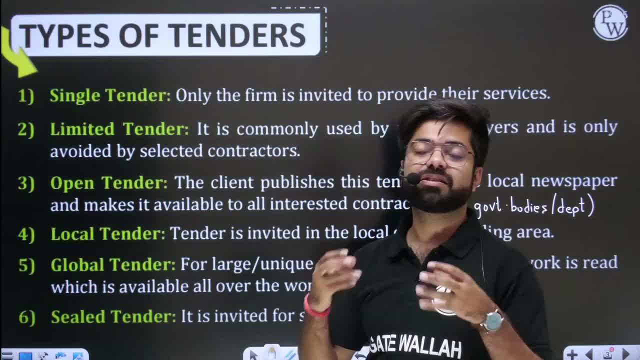 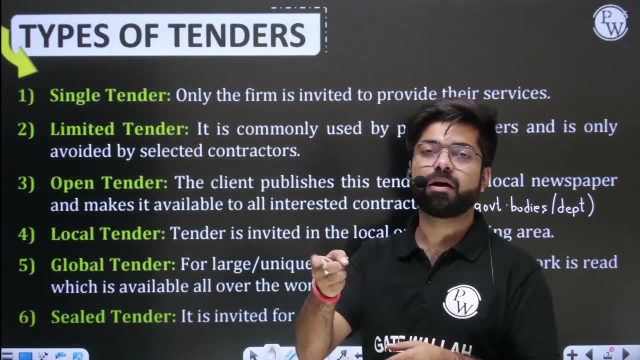 for example, someone has made trust after the competition. for example, you are 10 children. one person performed the best among 10 people in the class. so from the teacher's point of view, the child is good next time if there is any work. 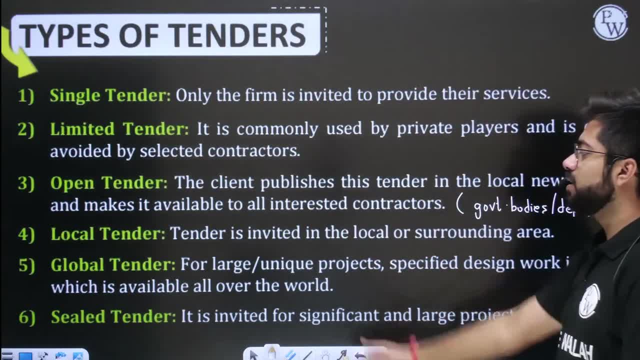 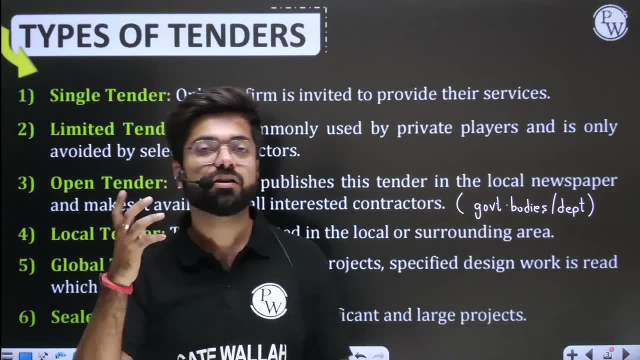 the teacher always goes to him. this credibility has to be established first, then these things happen. then what is a global tender? Global tender is a very large and unique project, like in Dubai, some big building in the sea. who are building the earth these days? 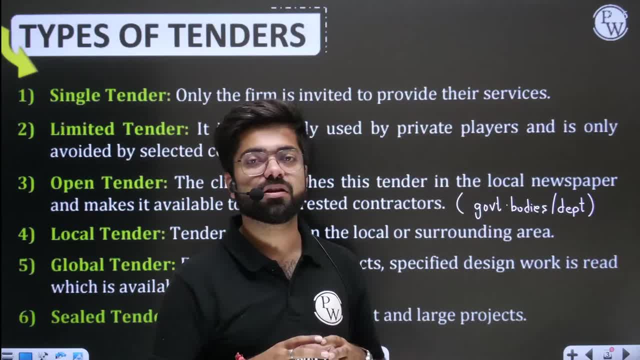 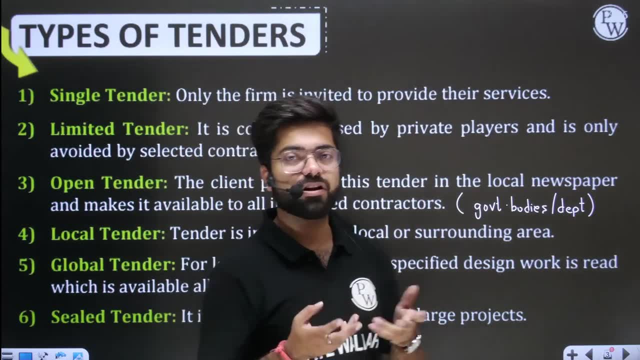 some unique and new project is being done. it is a big project. a lot of money is going to be involved. then it will not work with limited sources, not 5-10 contractors. then it has to be published in the whole world. 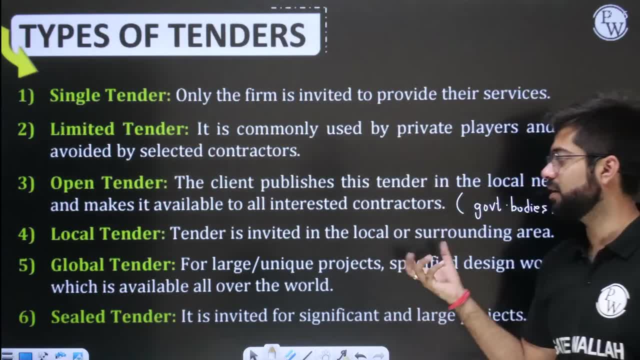 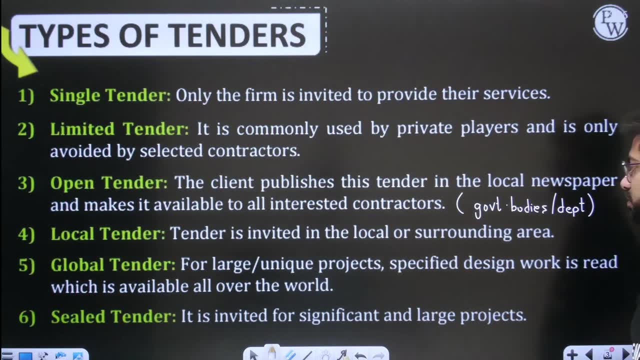 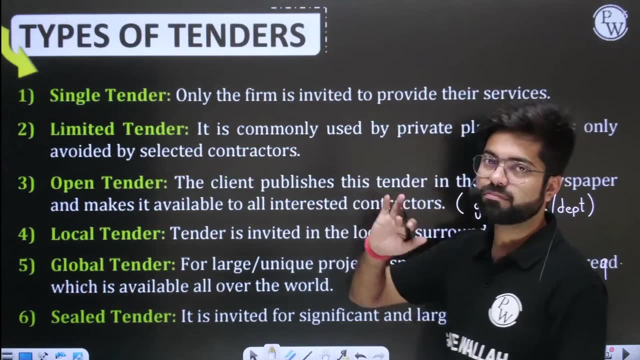 it has to be advertised so that all the experts of the world come and show their talent here. so for large, unique projects, specified design work is required here. they have written read required which is available all over the world. so we have to circulate this form. 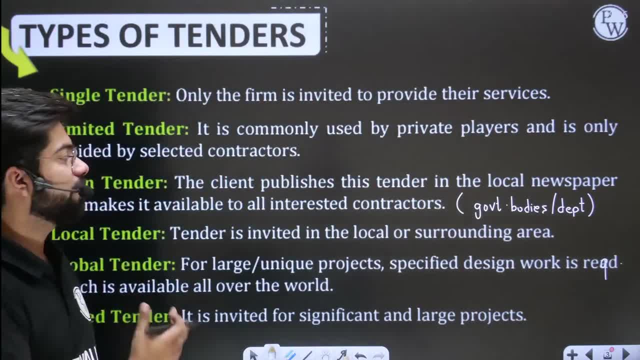 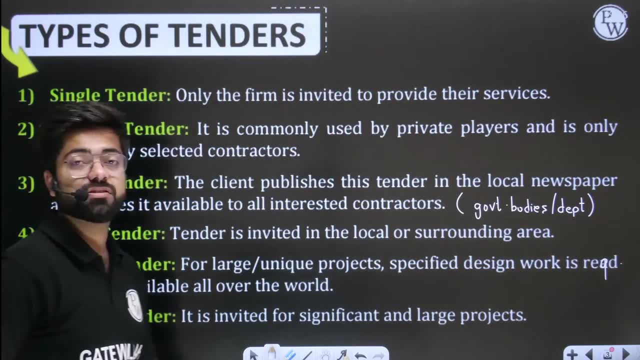 in the whole world so that all the talented people can come here and complete this work and the rest is a sealed tender. this is a different thing. this is a very good thing. what is a sealed tender? no one has to tell. 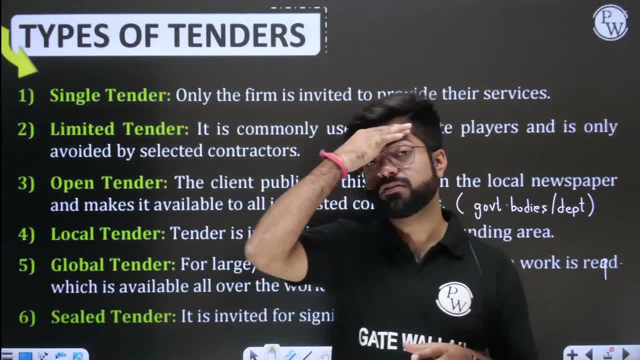 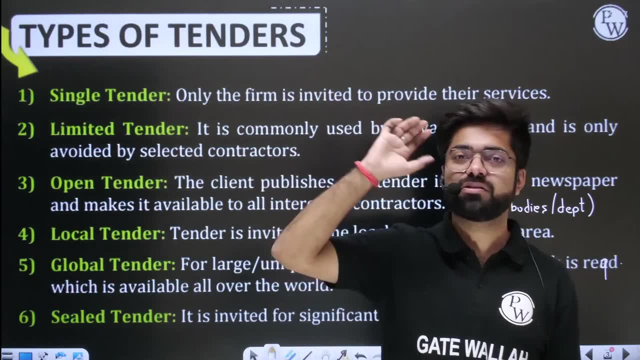 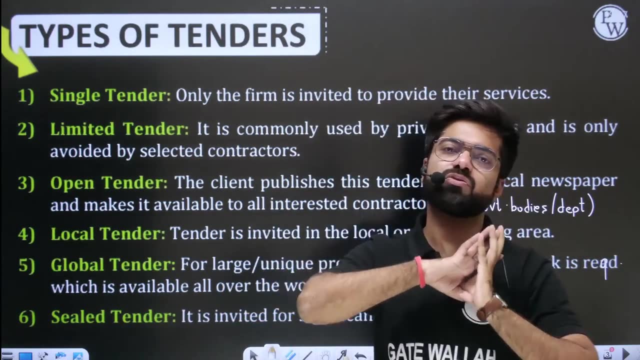 it has to be done quietly, like, for example: you know that when world war 2 happened, two people were making a lot of trouble. no one was listening to anyone. whoever came, who were they? one japan and one germany. in the west, there was a lot of destruction. 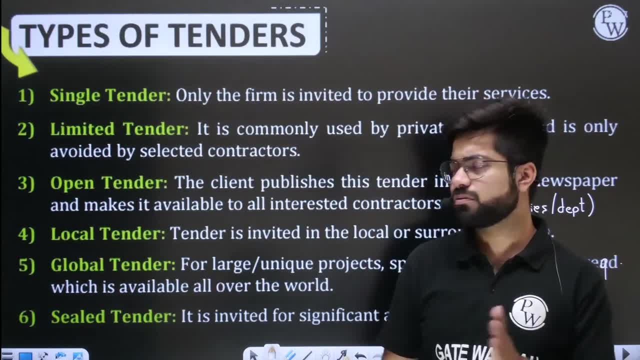 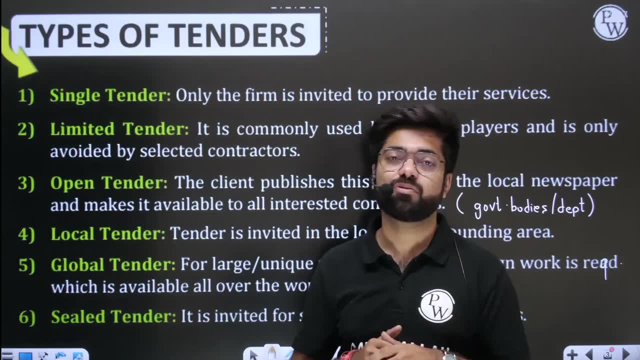 in the east. there was a lot of destruction. no one wants to listen to anyone. no USA, no Russia. it doesn't make any sense right now. they are making a lot of trouble. what should be done? the USA people were disturbed in the last. 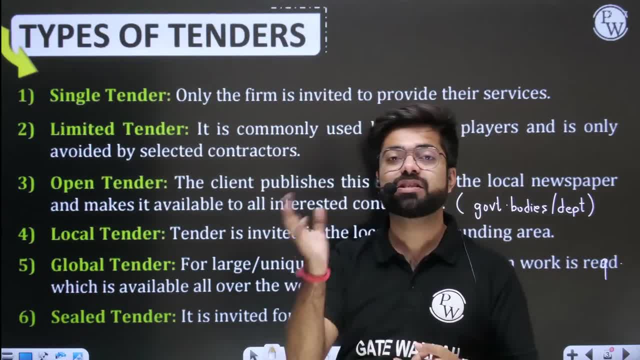 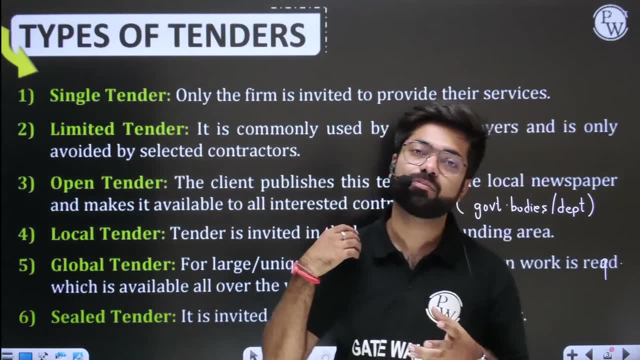 the USA was not even jumping in world war 2, once they attacked pearl harbour in the USA, they had a very big port. they had an important base. the whole ship reached in the morning. they flew the whole base for 2-3 hours. it was a very big news. it is still famous in the whole world. now what happened? the USA people were disturbed. now this has to be stopped. the dominance of Japan and Germany had increased a lot and Germany was in a mode of losing the world war 1,. 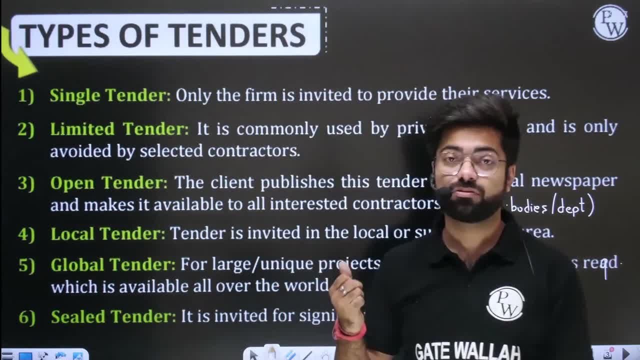 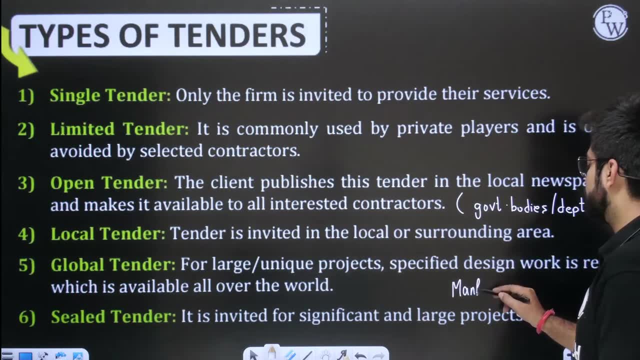 they said that they have to take revenge now the tender that the USA did at that time. they made a project, the name of which is Manhattan. this is a good story. maybe you have heard Manhattan project. then you must have heard that in the Manhattan project 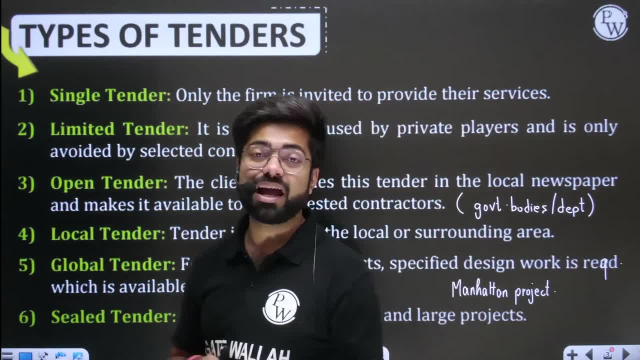 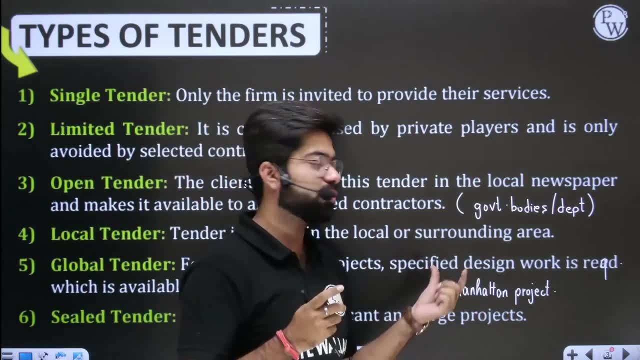 very strong minds of the world were involved and an atomic bomb was tried to make. don't you know, Albert Einstein? this sealed tender was sent to some brilliant minds at that time. Manhattan project was the name of this project and only important scientists 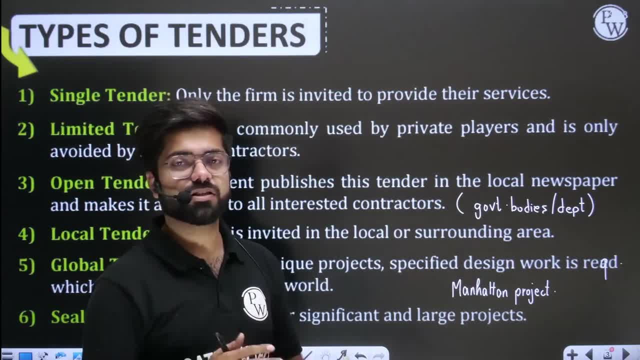 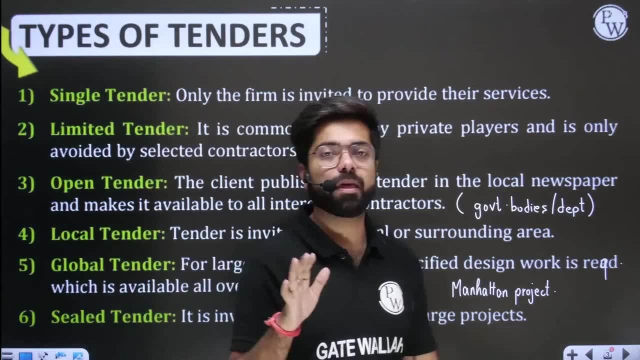 like one of Albert Einstein and I don't know who else, who made a total destruction in modern physics. all of them were sent to this tender. now, this sealed tender reached them in a very secret way and all those people together had to start their work. the whole code was working and then the atomic bomb was made around 1942, when the neutron was forged. after that the bomb was made. even then Japan was not stopping. the first bomb was dropped. you must know that there were two bombs. Japan was very excited. there was no point in stopping when one atomic bomb was dropped. there was a huge destruction. maybe the first one was dropped by a little boy. atomic bomb was the name of the bomb. then Japan came under control. 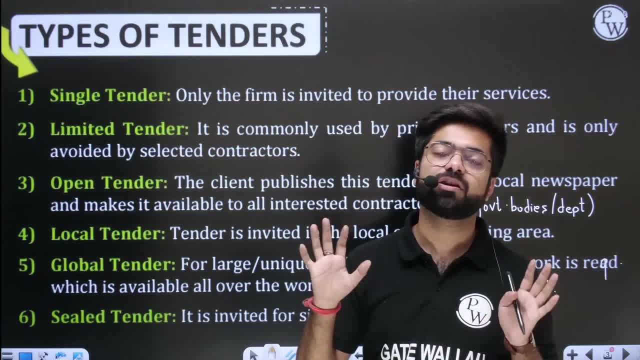 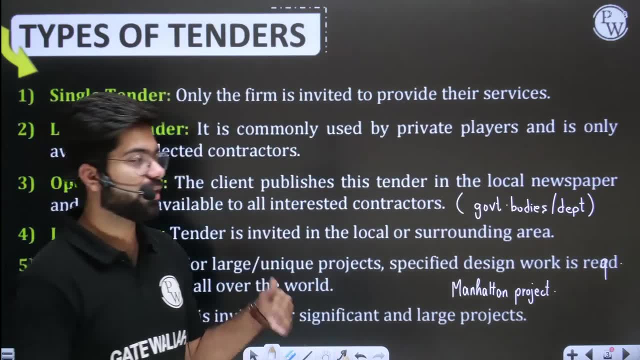 they didn't stop. then another boy was dropped. the name of the bomb was there. it was a huge power of the atomic bomb and even today we know that generations are becoming very bad. the effect of radioactive material is still there. 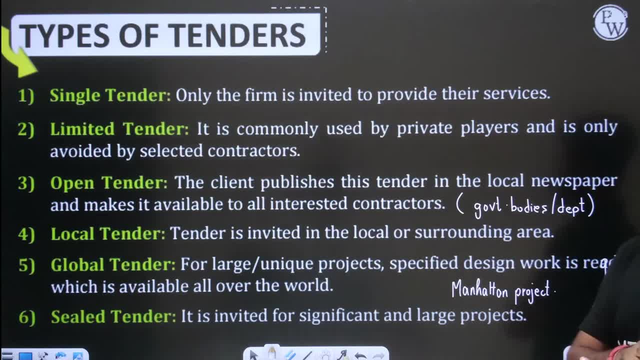 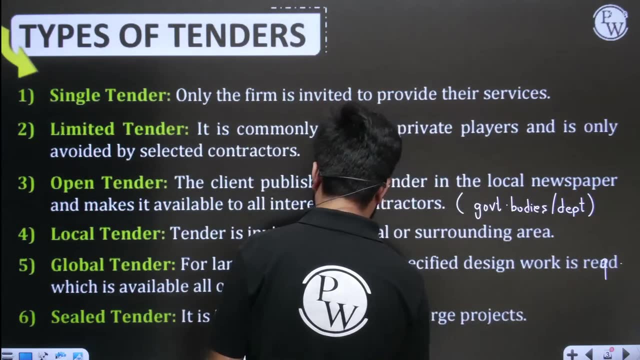 so this was a sealed tender. It is a very significant project and we have to keep it hidden and it is a big project, So let's go to that sealed tender. This is the example of a sealed tender. I hope you are clear with this example. 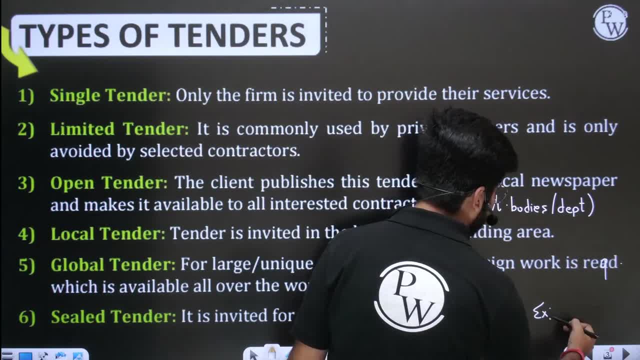 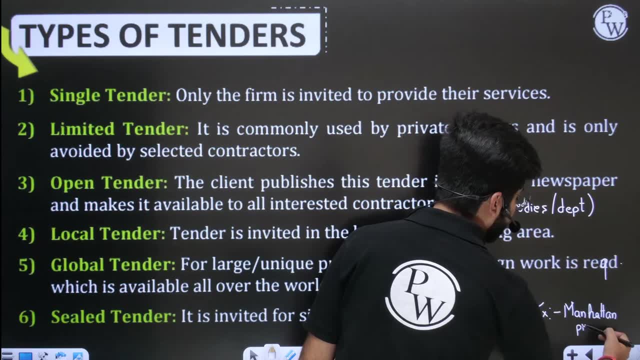 Let's write an example here so that you remember It is a very good project. There was a time in our life when we gave a lot of time to study all this. We were studying modern physics, so we knew all these stories very well. 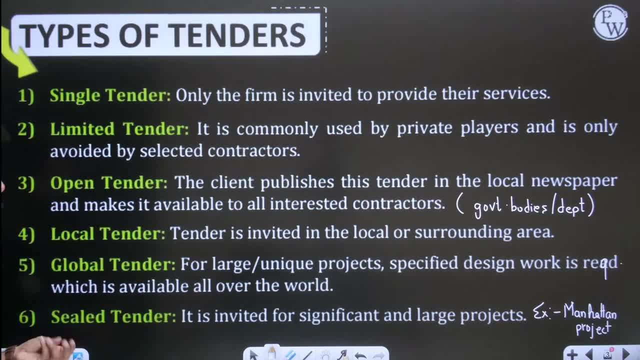 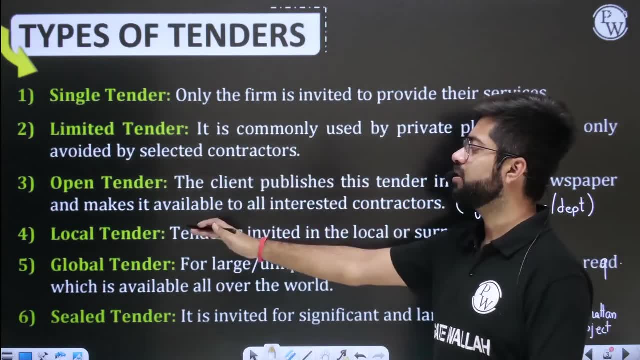 So this is our sealed tender For now. we don't care about all this. We are engineers. We will go to any department and provide services in the central or state level. So we have an open tender here. We will do small and big work. 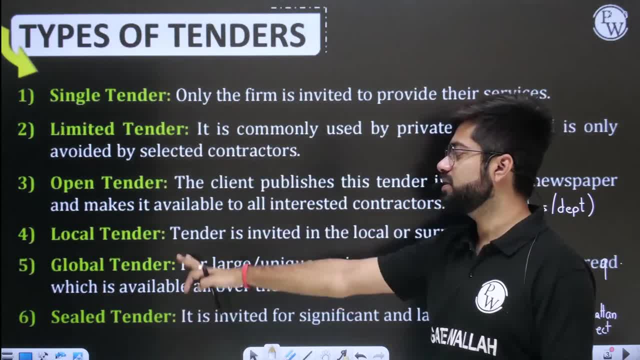 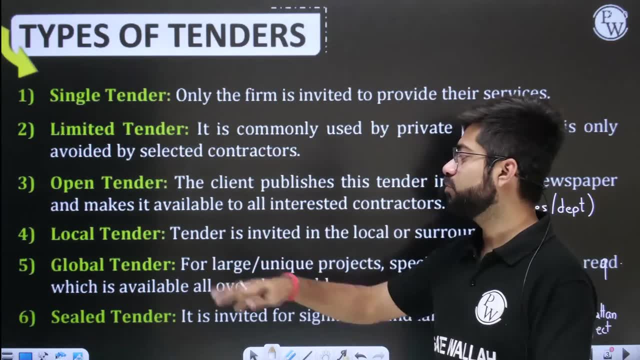 We will do local tender. We only have two or three above our means Now. you will go to a private company and work in Dubai. As soon as you start working in Gulf countries there is a lot of civil work. You may need a global tender sometime. 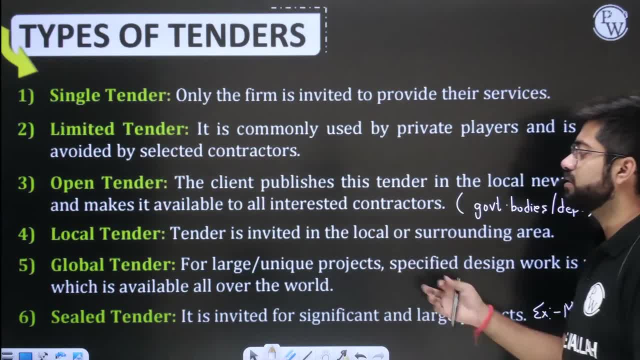 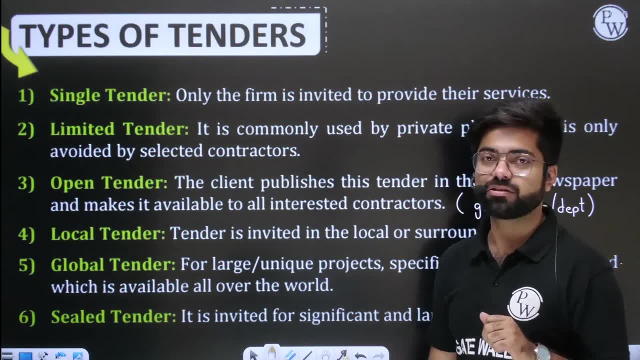 Right, That too. there will be a lot of people in it. It is better if you don't need a sealed tender. If scientists are involved in such dangerous work, then their lives are in danger. Right For now, we don't want to know all this. 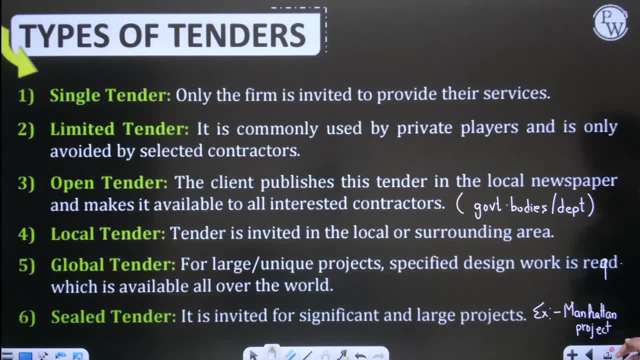 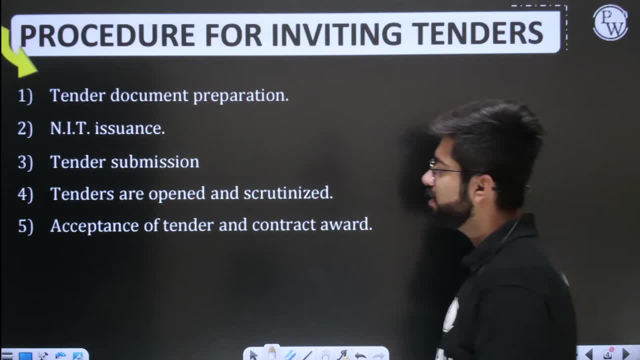 So we understood the meaning of open tender here. So these are different types of tenders. I hope you understood it well in the form of a story. Okay, let's move forward Now. when we invite a tender, what are the steps? 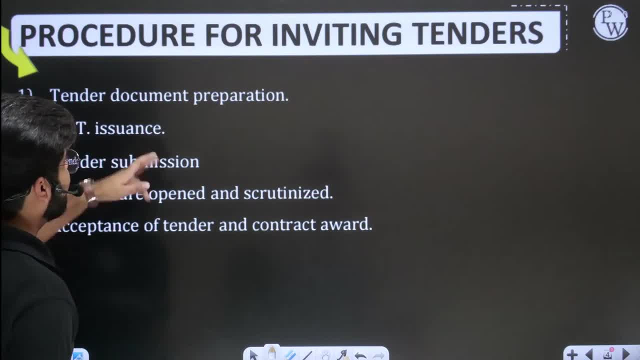 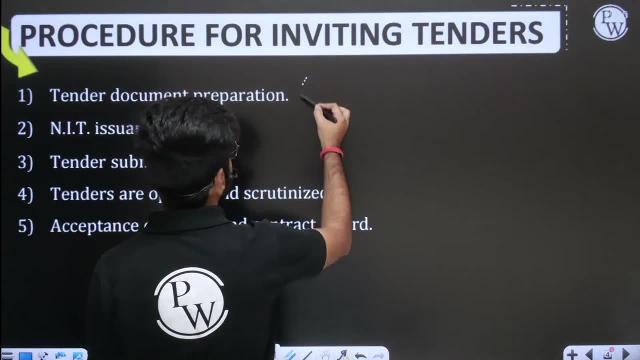 There are very simple five steps. First of all, who will prepare the tender document? Can you tell me Who will do the tender document preparation? Obviously, the client will do it. Who does it? Client? Now, there are specifications in it. 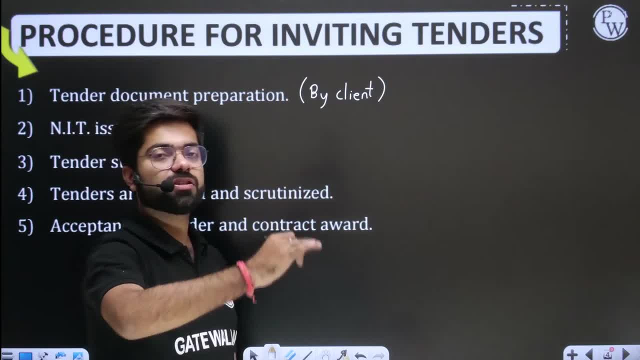 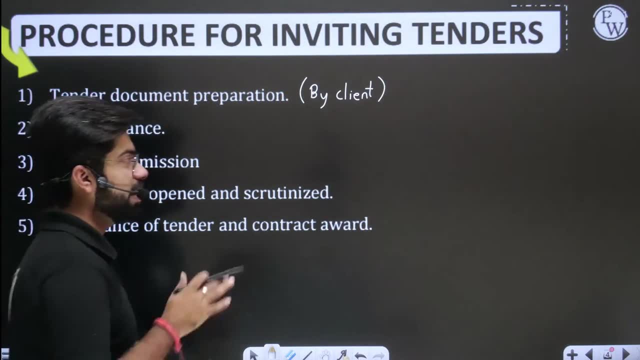 That this thing should be like this. This should be the level. There should be this much discharge in that canal. We have taken the example of the canal, So let's talk about that. So the client will prepare the tender document here That it will be like this, like this, like this. 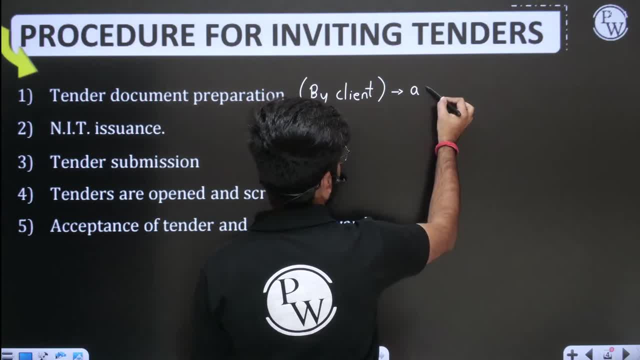 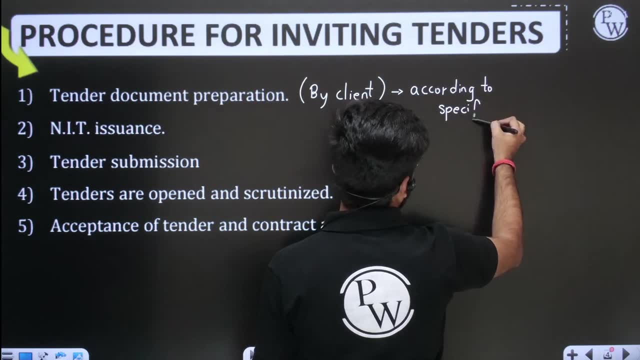 Specification will be mentioned to him. Okay, Specification will be mentioned in it. So I will write, according to specifications, That it will take this much money. It will take this much time. Capacity of the canal should be this much. Okay, There are many specifications. 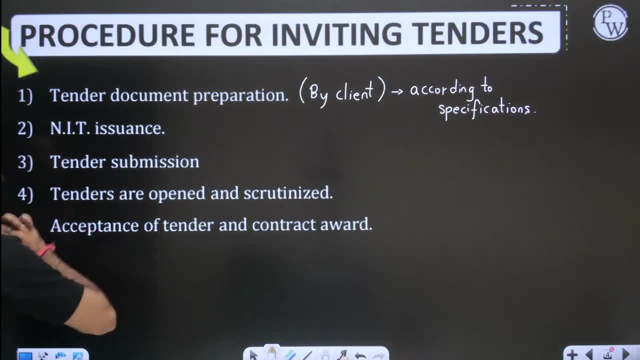 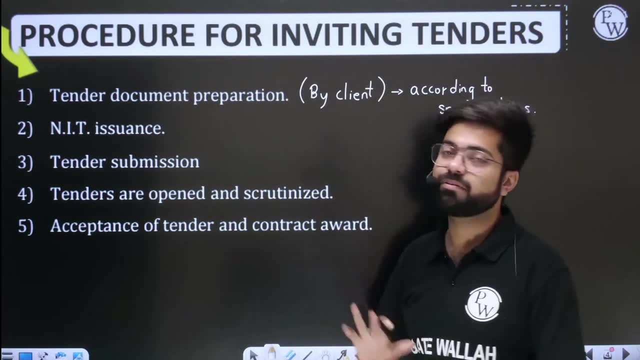 Okay That such things should happen, Then notice inviting tender will be issued. Okay, Notice inviting tender will be issued And the people around the world will see it That this work has to be done in this way. The client has told. 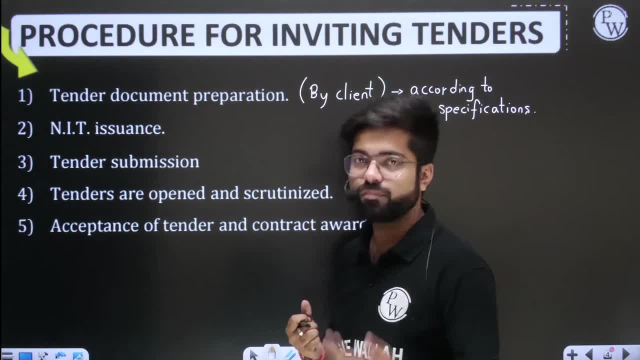 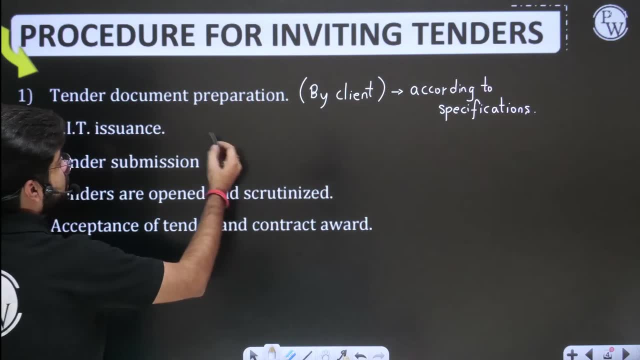 Okay, The client has told We will see it. well, Let's reach, Then the tender's form will be filled. Okay, Tender's form. So what does NIT issue mean? The tender has been published. Okay, NIT notice inviting tender has been published here. 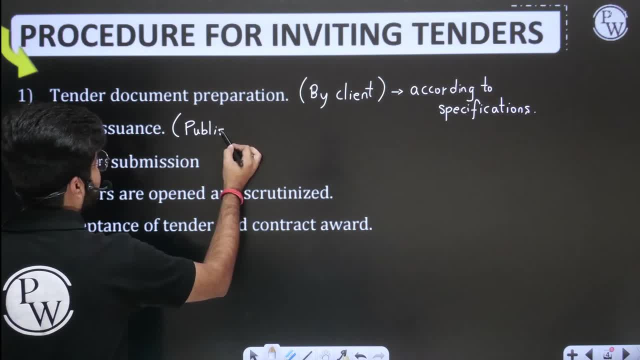 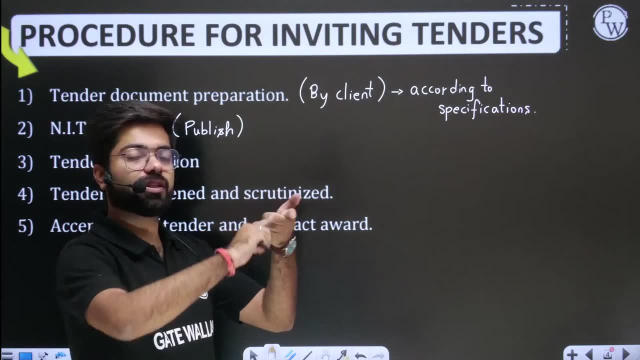 Published Now when everyone has read. So all the people who gave the proposal will come and submit their tender That we will do this work with so much quality and with so much money. Okay, Here the tender will be submitted. Now we will read all these forms: 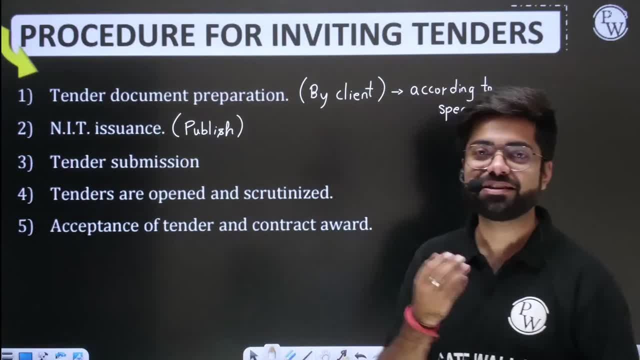 All the proposals will come to us. All the proposals will come to us. Okay, All of them will be analyzed. That who is more beautiful, who is less beautiful, Who is giving more money, who is giving less, All this is seen. 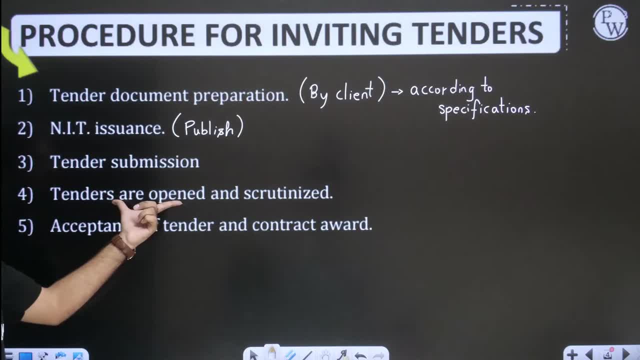 So now what will happen here? The tender form will be opened And their scrutiny. That scrutiny means their analysis will be done. Okay, Their analysis will be done. They will be compared That who is better, who is better, And we will choose L1 in it. 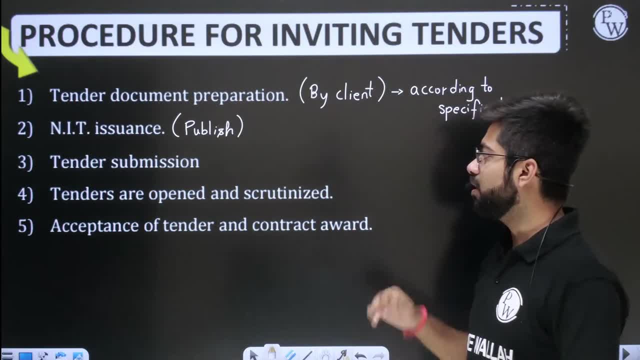 L1 means lowest one, Lowest one. Why lowest one? Because we have to work cheaply. And before choosing the lowest one, we also check the quality. There are two things. Look, Let me tell you If you will check. 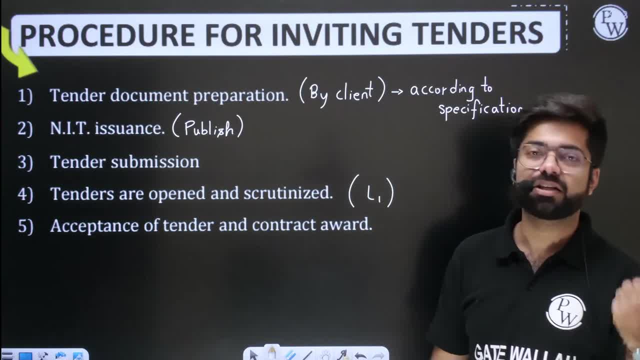 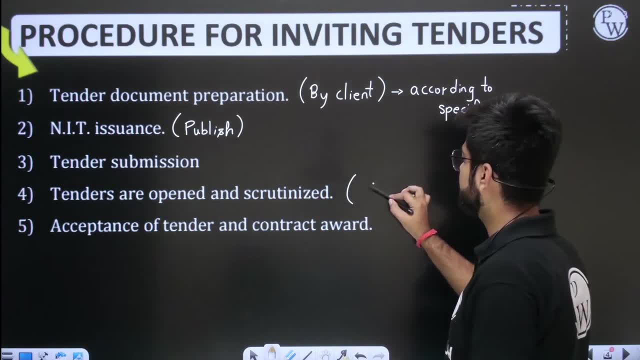 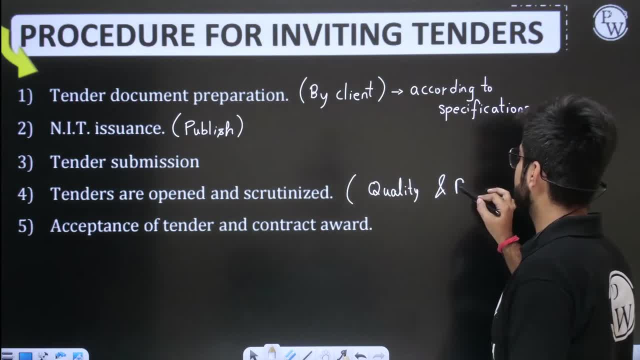 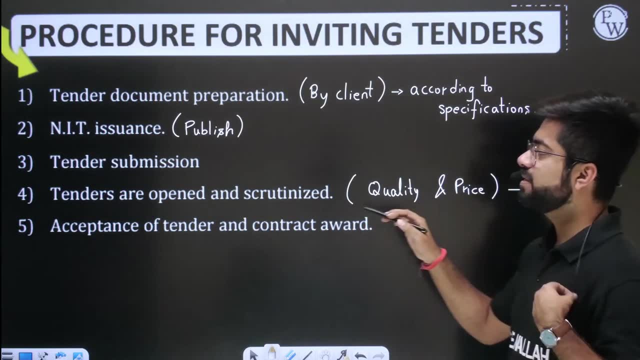 Quality- Okay, Quality, And second thing is price. If we get good quality, Then after this The lowest price. Suppose someone's price is more Okay, But the quality is good, So we can choose that too. It is not like that. 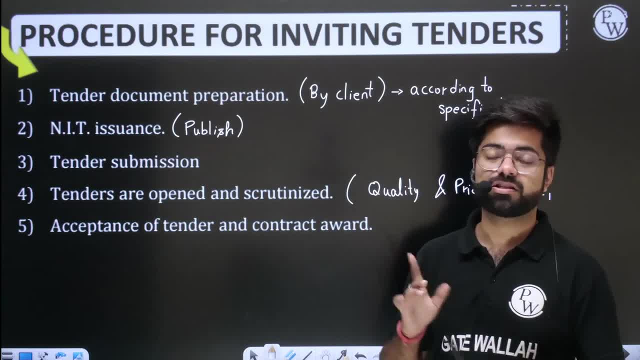 Okay, I don't understand this. We have to see the quality, We have to see the price, We have to see both things, But generally it happens That everyone has the same kind of work Form Document We had, given that we have to do this work. 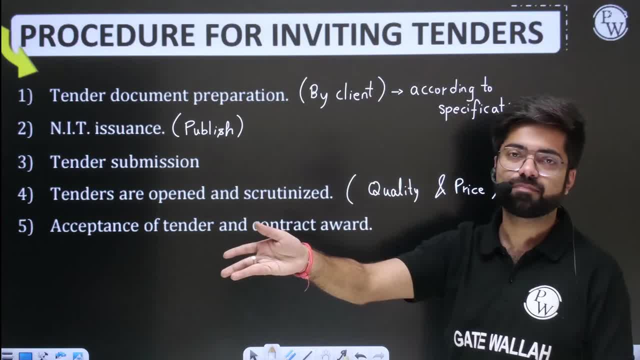 So he will write and give that we can do all this, Brother. obviously we will make your channel like this, We will make it like this, We will make it like this. So the quality is generally more or less the same for everyone. 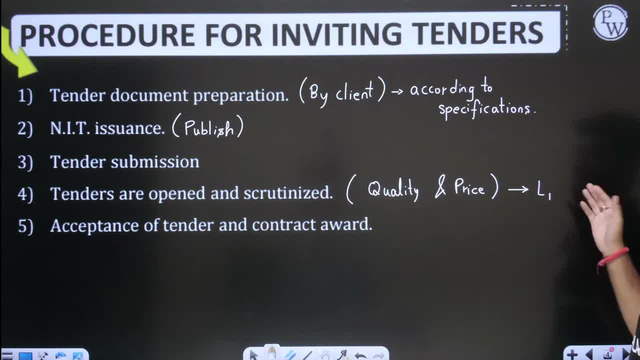 That's why we check the price And then after that we give the lowest one. Okay, But suppose, sometimes it happens that we want to work in 100 rupees, But the lowest one came in 101.. Okay, The rest of the people were doing more. 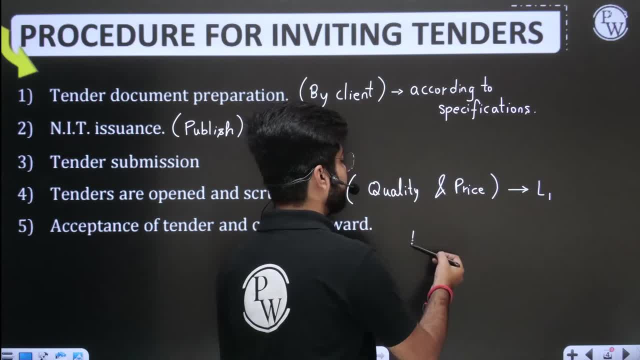 It was one, It was this, It was this. There were three people. Now we have to choose this, But this also did not come at our rate Because we wanted it to be in 100 rupees. Generally how much we want to work. 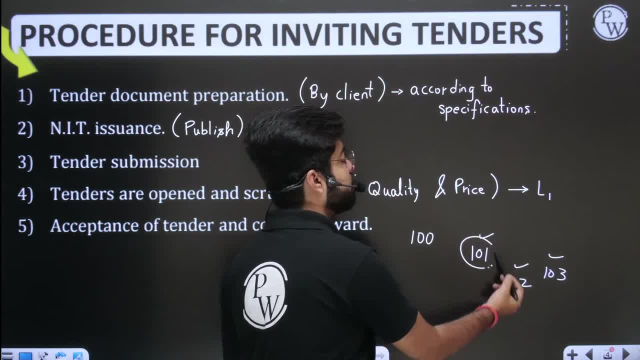 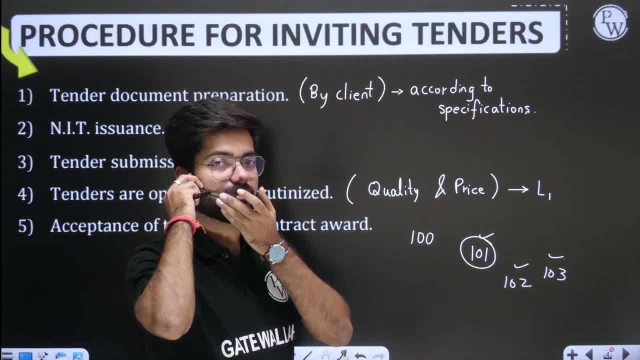 This is not written. Okay, Generally, how much we want to work, This is not written. We send a form, We give it in the document, We give it in the document And the document says that you pay, You pay. 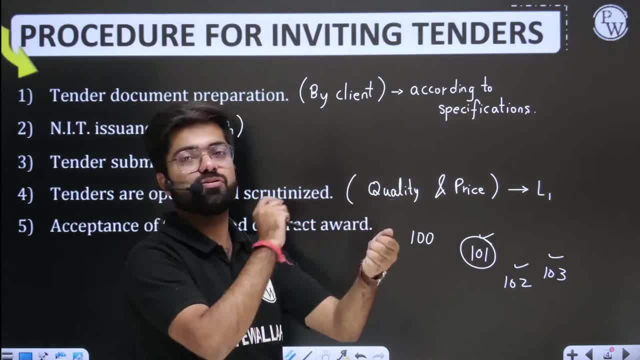 How much money you need for this work. You pay according to yourself. We do not tell. Look, there are two things. There are two things: Either you tell us in advance that our budget is one crore, Or from some letter whatever, from 100 rupees or whatever. 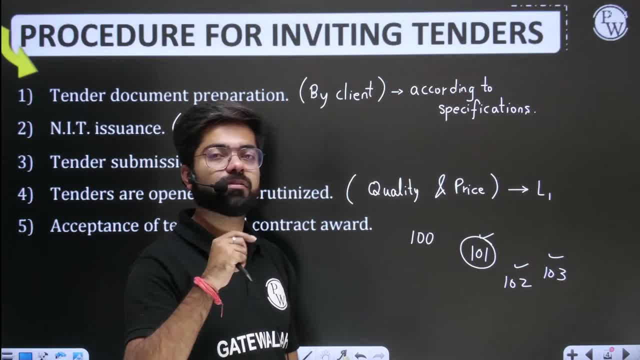 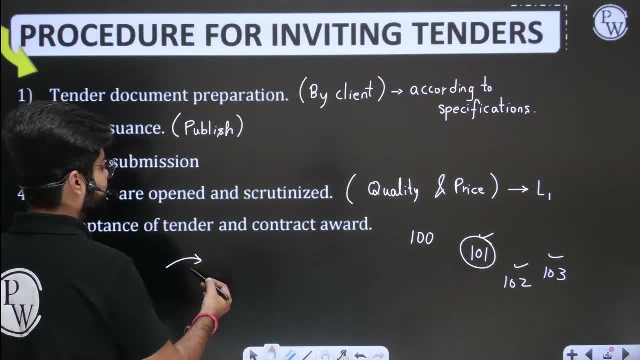 There are two things. Either we expose our budget in advance Or we know. We can tell you that we have an exam, And we know it. Then we say that we have an exam. And we say we have an exam. two things: either we expose our budget from the beginning or we ask the contractor to. 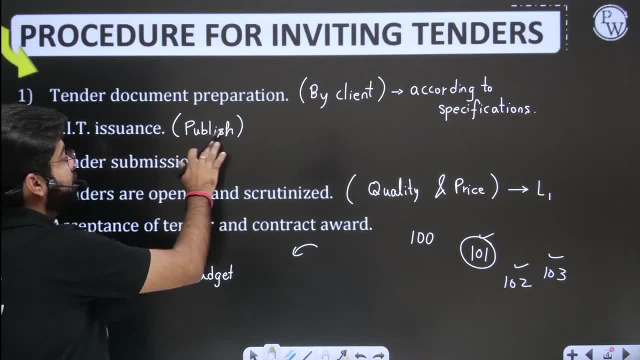 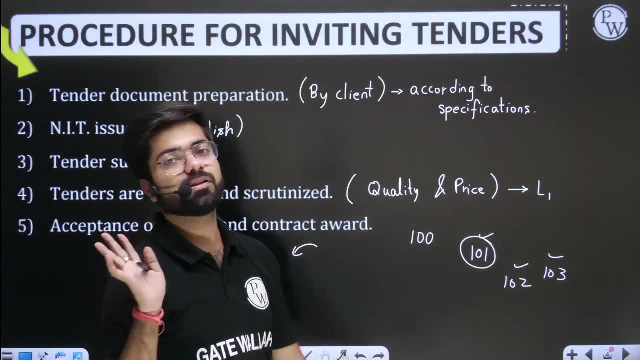 pay. When we have given him the document, when we have published it, then when he will submit the tender, then it is written in it that how much money it will take to do this work, you pay. We don't know. we don't know. we are sitting in the back, we are watching quietly, you, 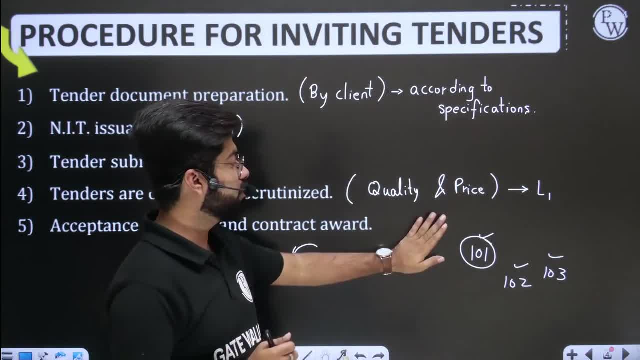 guys do the whole drama first, so then in it now, as if you have kept your money hidden. you know that you have to do the work in 100 rupees. now he has filled 100,, 200,, 200, 25,000 rupees. 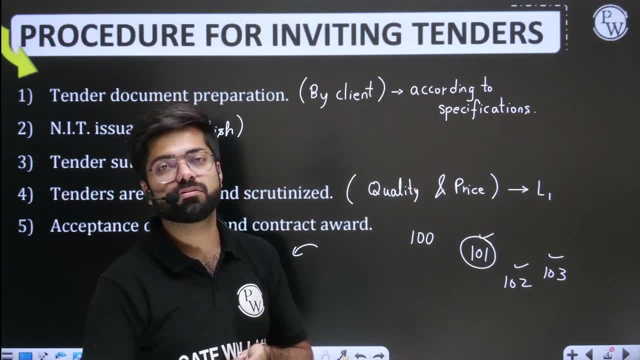 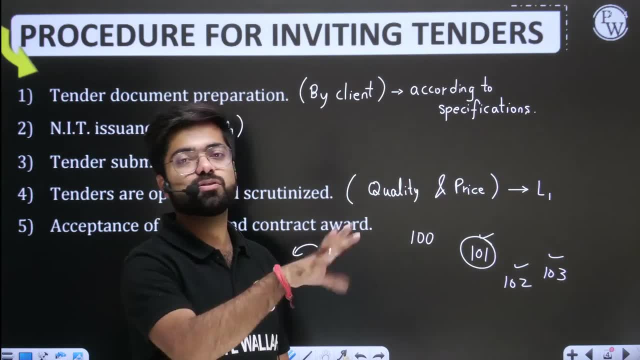 The combination of these two things will be called your contract. You will have to pay it, but that will not be in your budget. what will you do? it is not matching your budget. then many girls' photos have come. you have understood that. 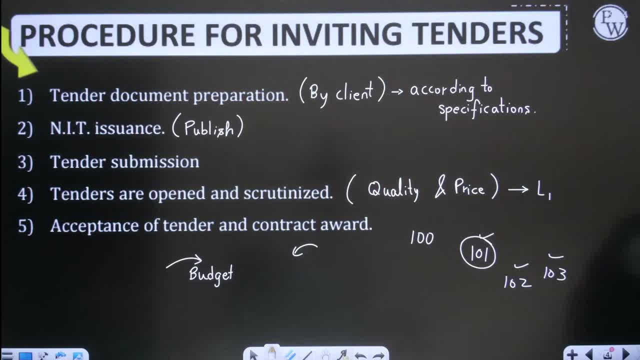 you have chosen the best amongst them, but that too, it is not matching your specification. what will you do? can someone do it again? The whole process has fallen, so what will we do? in this case, we will see the lowest of us, the one who is the lowest. 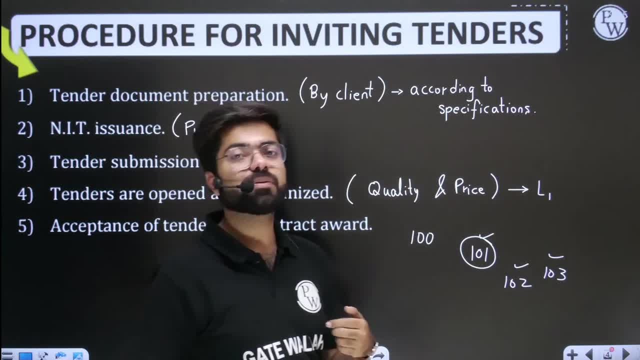 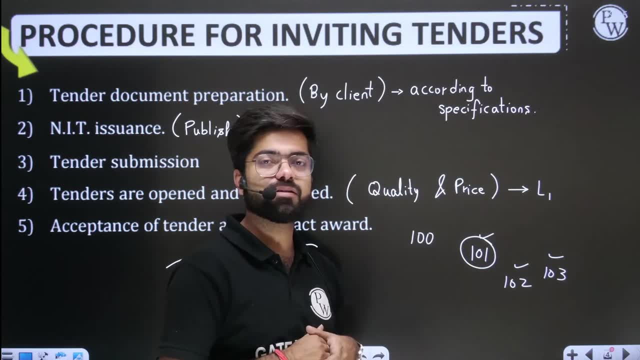 I will point out the second point: Negotiations will be done. Negotiations will be done. You understand what I am saying. Come down a little bit, Work well, Negotiations will be done. Negotiations are not happening. If they are not ready to negotiate, then we will float again. 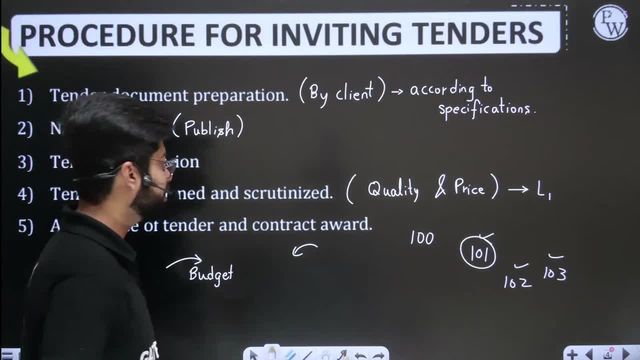 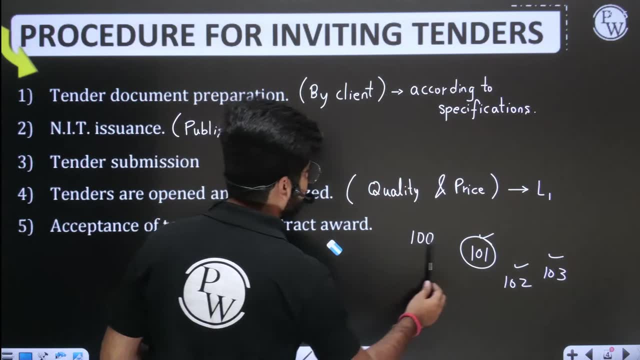 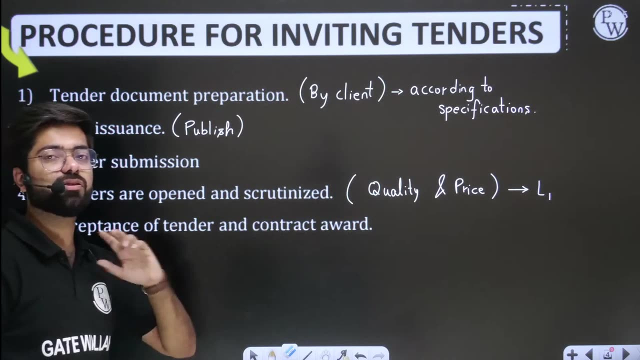 We will float again and next time we will mention. We can do this too. Sometimes mention is there, Sometimes mention is not there. You understand that this is not very tough, And as soon as we get our final Candidate, Then we accept the tender And then we about the contract. 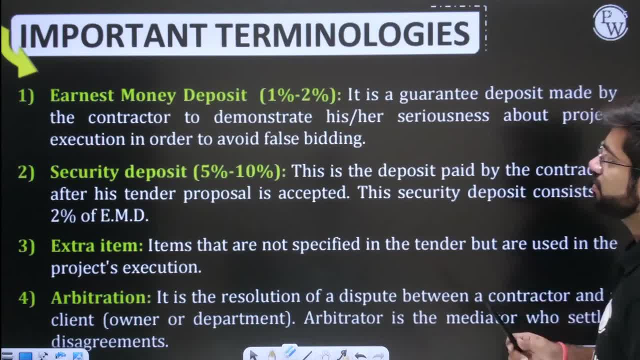 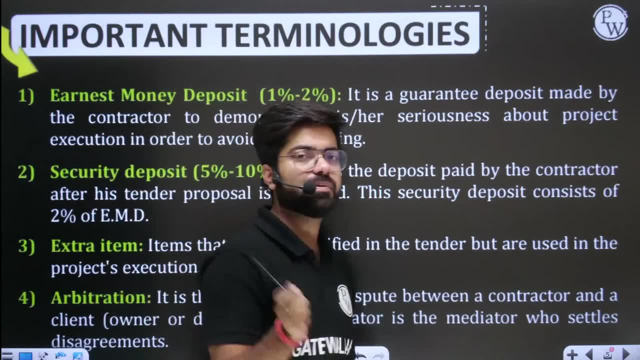 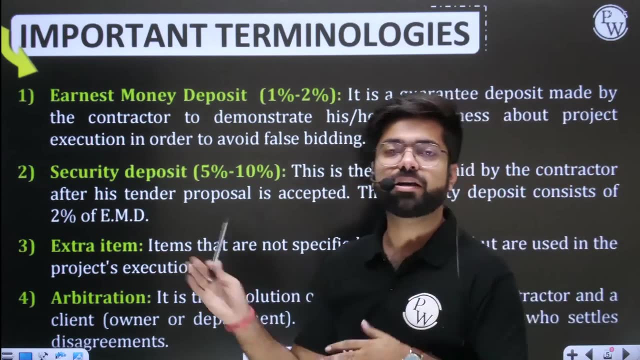 And then the work starts. So this is the whole process. Now, important terminology: All this is asked a lot in the exam When you will give SSC or AEJ paper Or ESC pre, Because the work is done. So you should know all these terms. Now you understand the story. 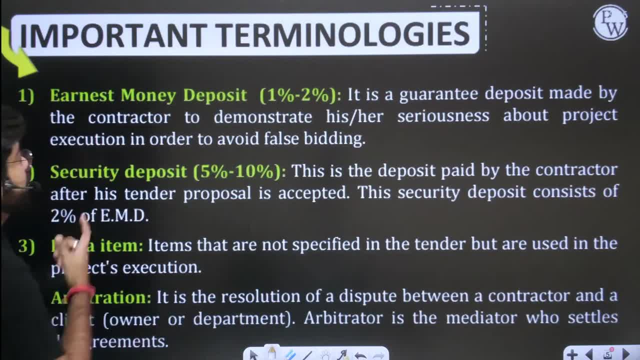 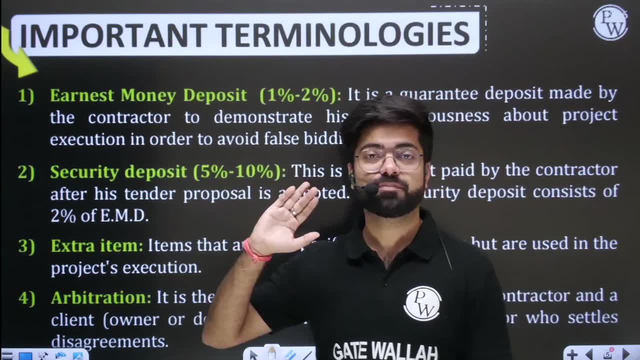 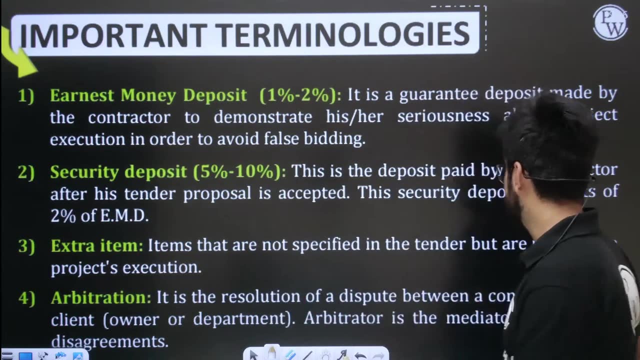 What is happening? First of all, there is a definition: Ernest Money Deposit. When the tender is filled, Then a lot of relationships come. We have spoken about relationships again, A lot of proposals come. That we will also do. But when you submit the tender form At this stage Here, when we will submit the tender form, 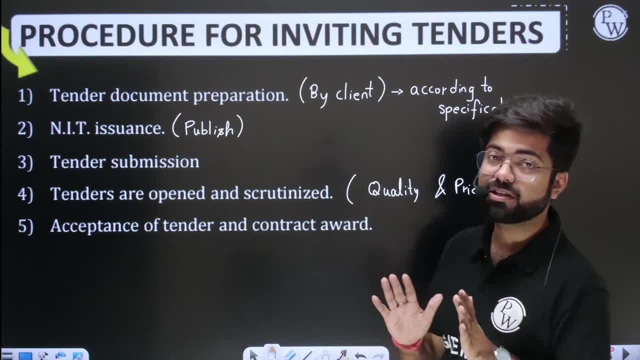 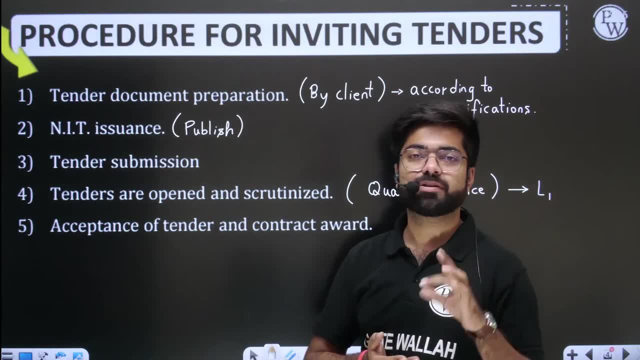 So while submitting the form You will have to pay some money, Approximately 1-2% of total money. Now here, if they have mentioned the total money, It is a project of 1 crore, So 2% of 1 crore is 1%, Approximately 1-2 lakh rupees. 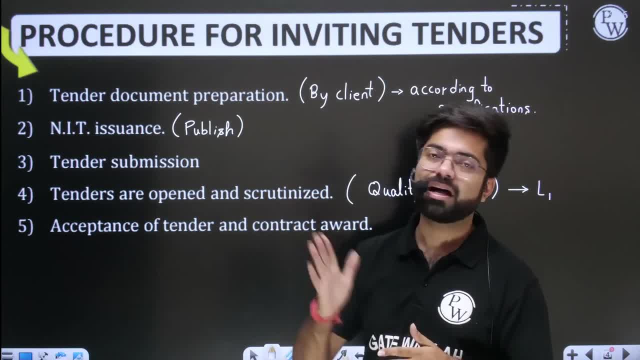 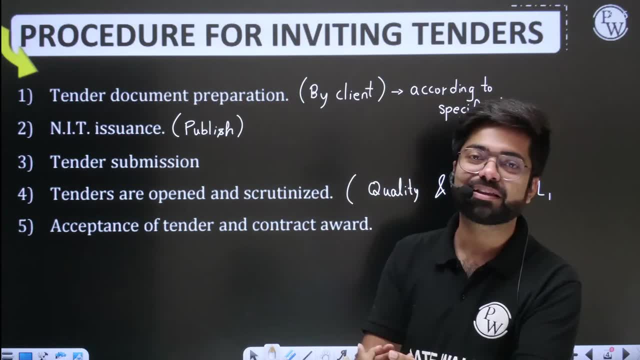 So you will have to pay 1 crore Because they are checking That you are not a useless person. Will you stay till the end? Will you be serious about this work? Will you be serious about this marriage? Will you be serious about this relationship? Just sent a photo. 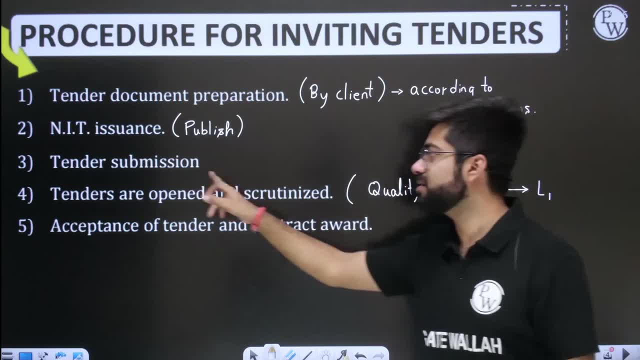 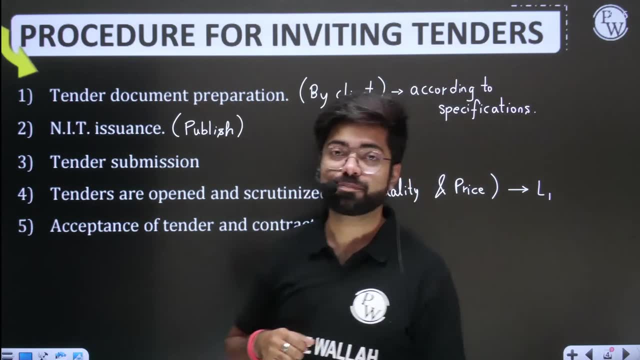 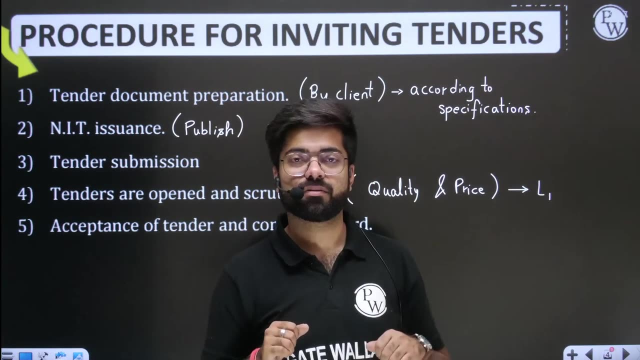 You keep sending photos, You keep filling forms To check its seriousness. When the tender is submitted, He will also submit money In the form of FD, The contractors. What do they do? They set the people. They catch only one FD. Now, the engineers are not so active That they will check the number of each FD. 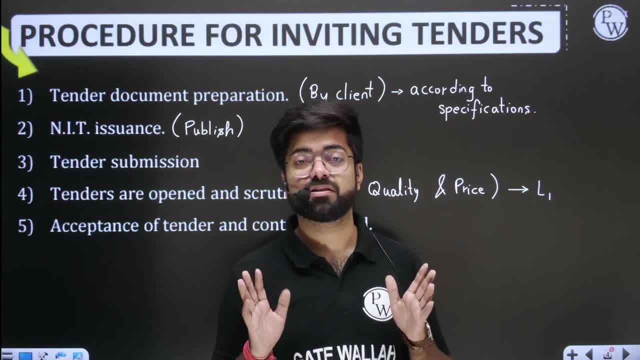 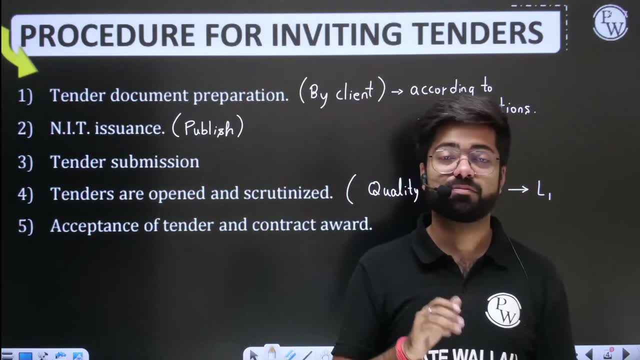 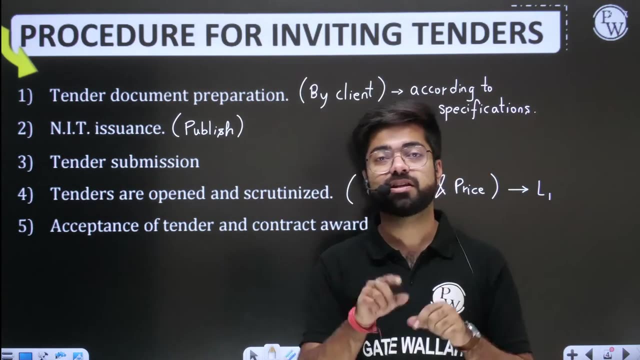 If it is fake or real, FD becomes fake. Security money is not actually being deposited. The same FD number is going up again. These are the works of AEJ. Everything has to be checked well, Because if you don't check, Then the glass will fall on you, Then there will be a charge sheet on you. 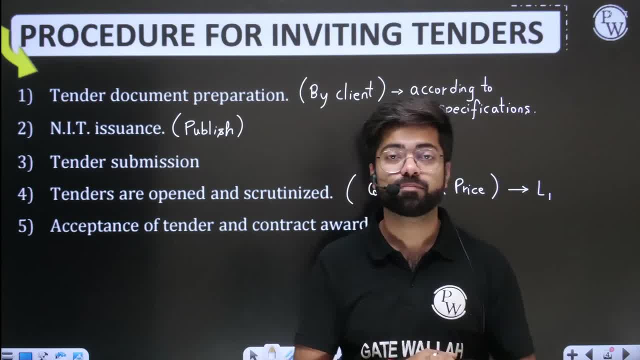 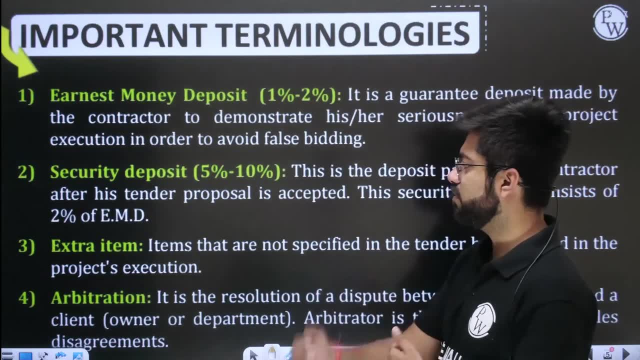 Whether it is repeated or not, Whether the actual FD is installed or not, All this has to be checked by the bank. So there are many things. There are 50 ways to do- corruption. Let's not go into the actuality. Let's focus on our questions. This is called Ernest Money Deposit. 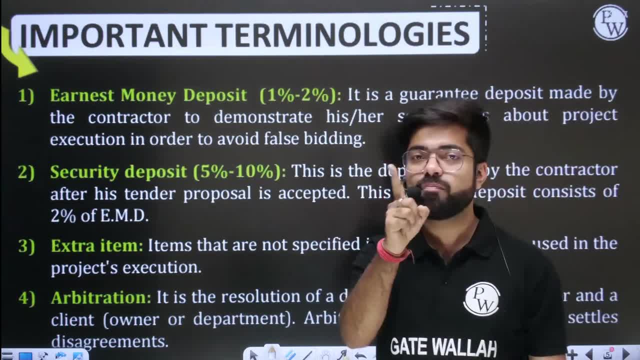 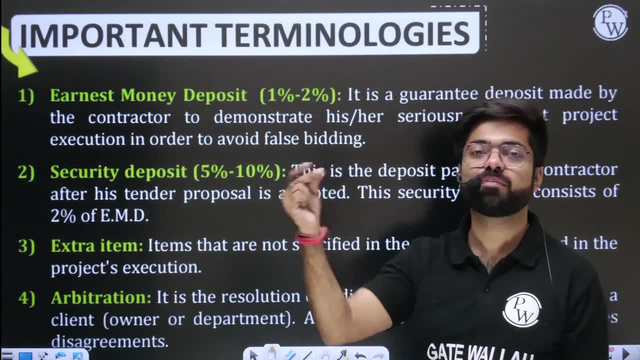 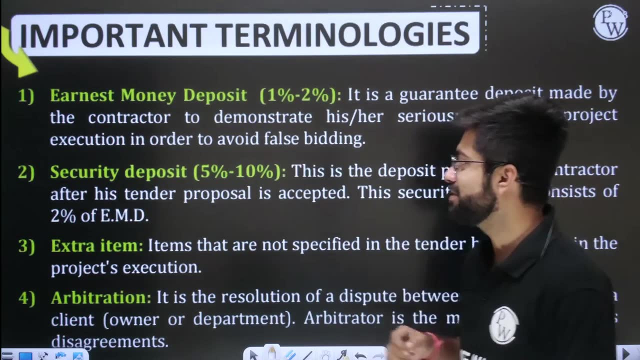 It is simply written that there is a guarantee, A guarantee deposit is taken That you are filling the form. You are sending the relationship Be serious later. It shouldn't be like this. We have selected you. We will bring a new bride. There will be a problem. This work is done for seriousness. 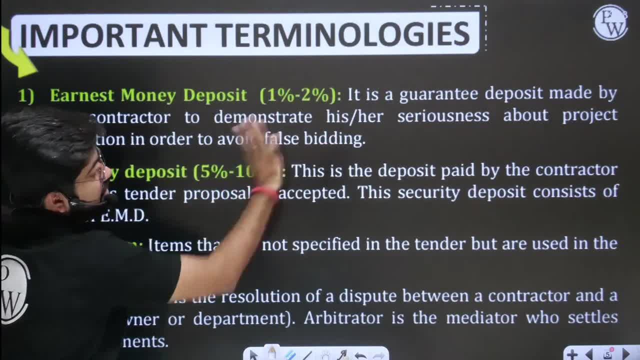 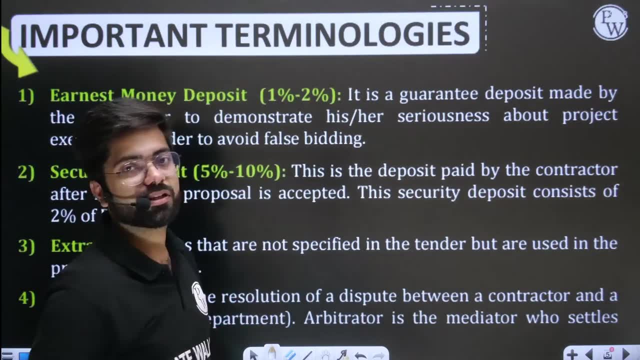 So it is a guarantee deposit made by a contractor To demonstrate his or her seriousness About the project, So that they don't do a fake bidding, Don't give a fake proposal That yes, we will do it. But if they do it later, Let's say N people filled the form. 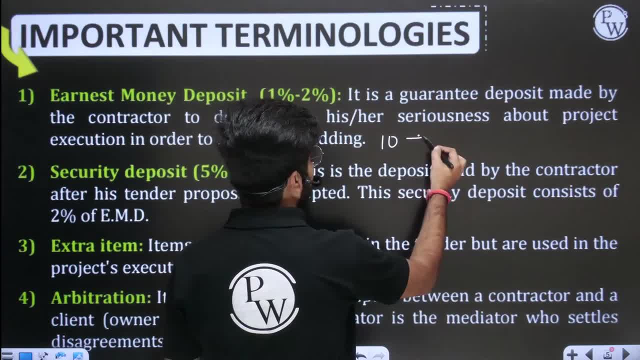 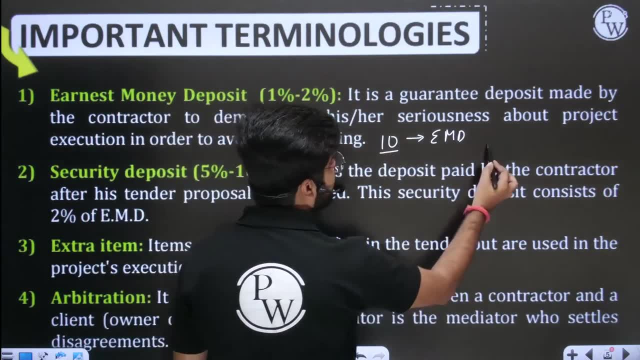 10 people filled the form, So 10 out of 10. We have to deposit our Ernest Money. Remember, this is 1-2%. Now, how many people will be selected? Only one person, The person who will be selected. He will have to give a security deposit. 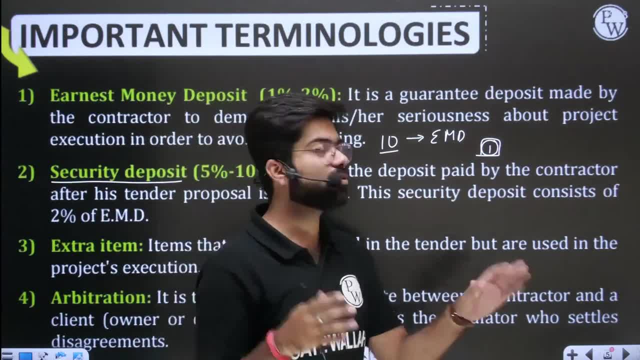 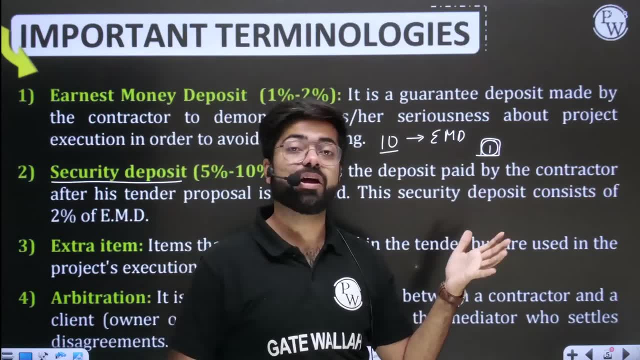 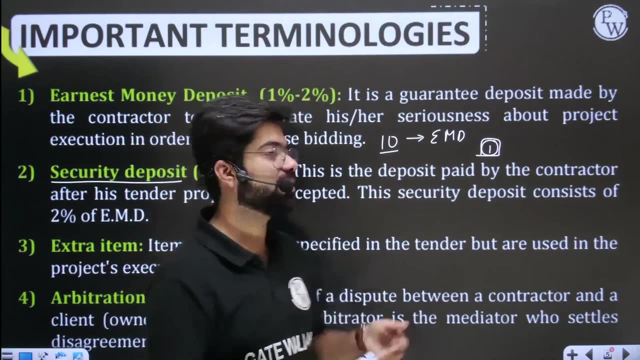 Security deposit is given because Suppose this person who has been selected, He has done all the work. Now, what happens? even after the work? Some things can happen here and there. Will it last till the end? Will it last till the end? Suppose he worked, He got some money and ran in the middle. 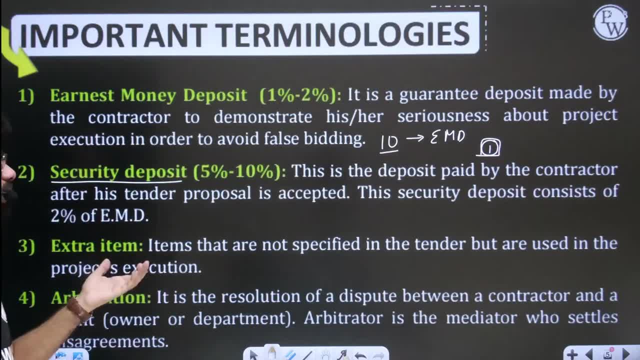 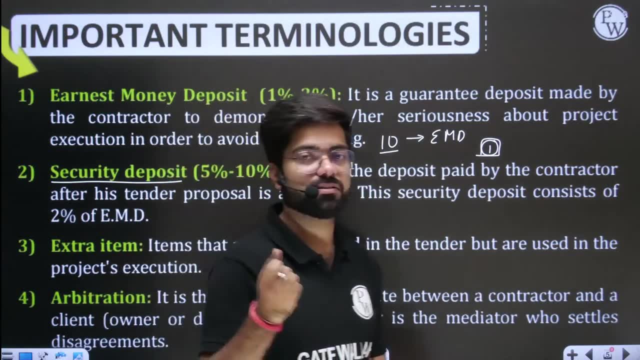 That's why security deposit is kept, So that 5-10% of the money can be used To find the person If he leaves the work in the middle. So security deposit is given to one person Who actually works. Now he must have given the Ernest Money. 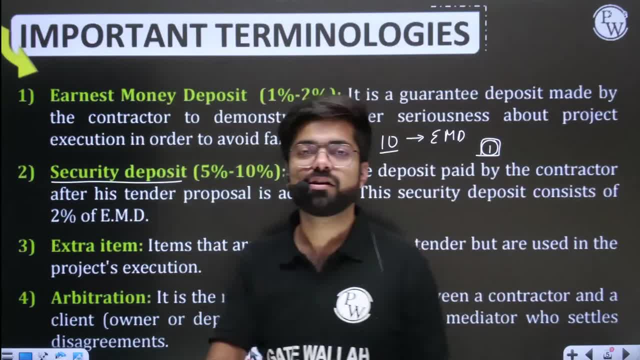 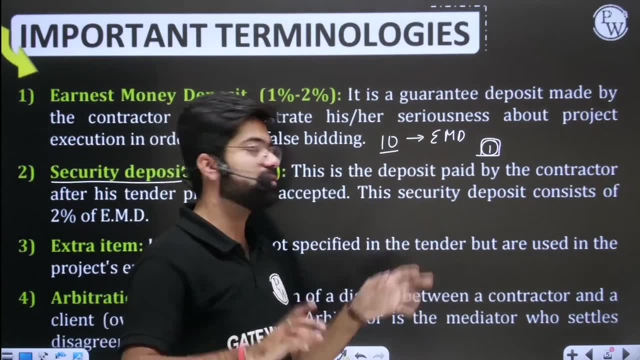 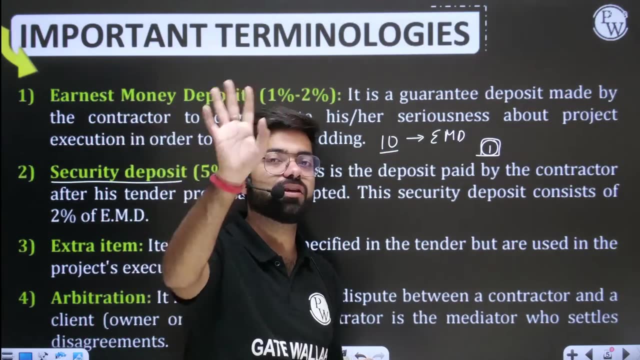 The person who has been selected. The person who has been selected, He must have given the Ernest Money. Will he get the Ernest Money back? Those who have been kicked out, Those who have not been selected, They will be returned. Their FD will be returned. Their Ernest Money will be returned. 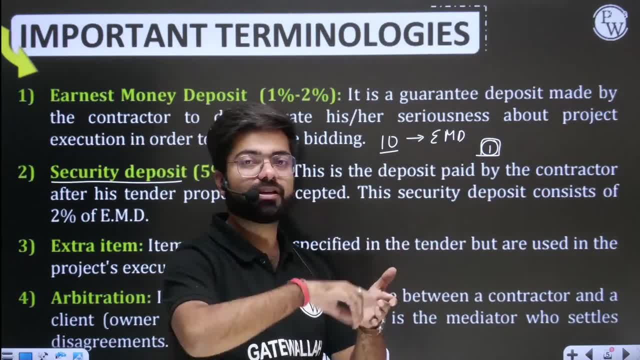 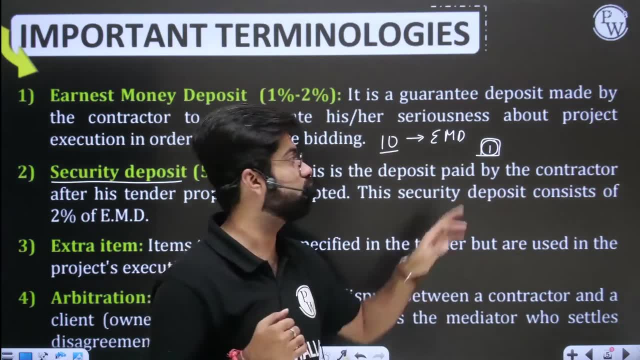 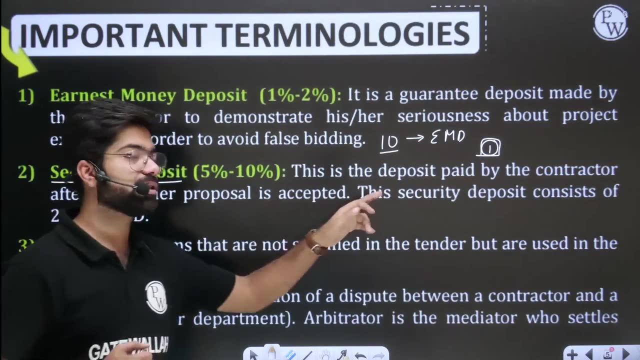 They will be called. Will they get the Ernest Money back And then take the security deposit from them? No, they will take the extra security money. 10%, That means 8%. See 2% have been taken from them. Now how much is left? So take 8% extra from them. 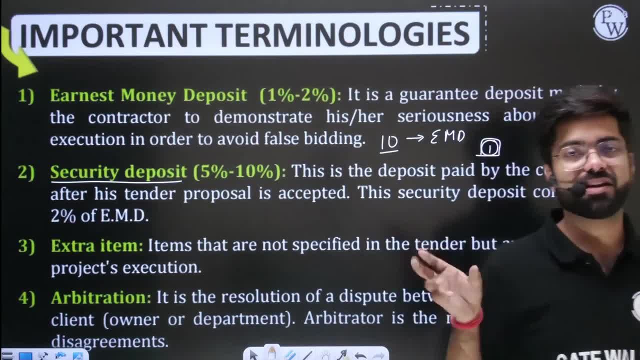 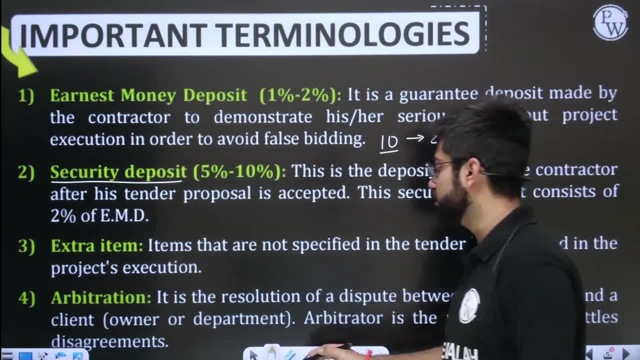 And that will be your security. So 2% is already included in the security deposit. Let's take it separately. We will take whatever extra amount is left. You must have understood. So security deposit from one. Do not take it lightly. Did not everyone understand? Did not everyone understand? 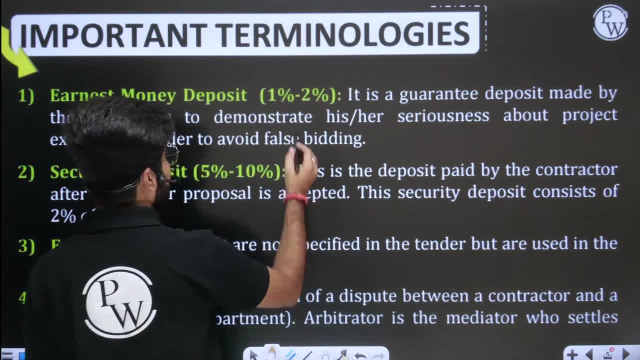 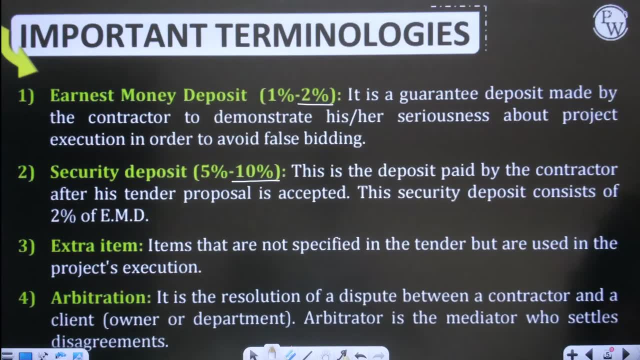 Everyone must have understood- So we have to remember the figure here- That Ernest Money is 2% And security money, Security deposit, is 10%. A lot of questions are asked. Ok, Yes, Absolutely Yes. Then the extra item is available. Now, the extra item is very simple. 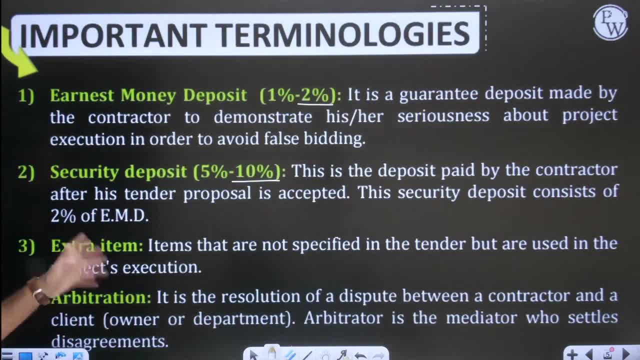 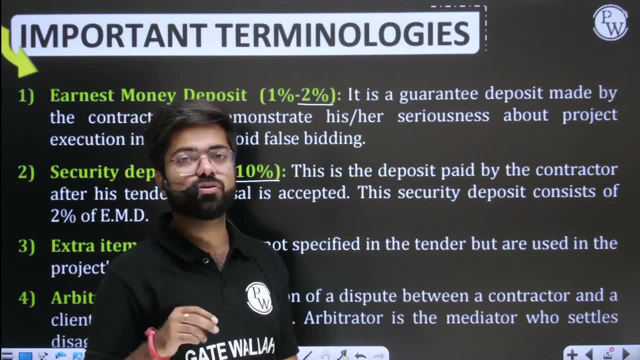 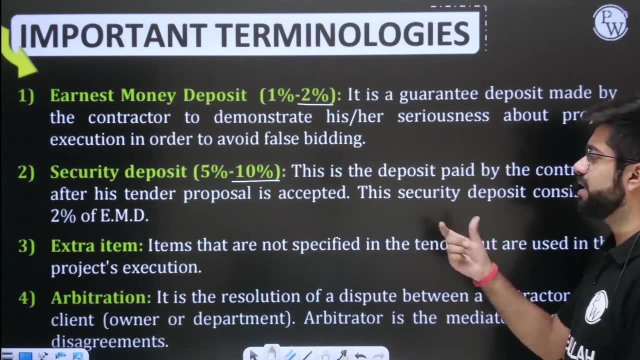 Items that are not specified in tender But are used in the project's execution. Now, not understanding the tender form, Long process of the tender construction. Something is missing in the tender, So they are called extra item, So they have separate expenses. Tender alot is Paulo, They are else. 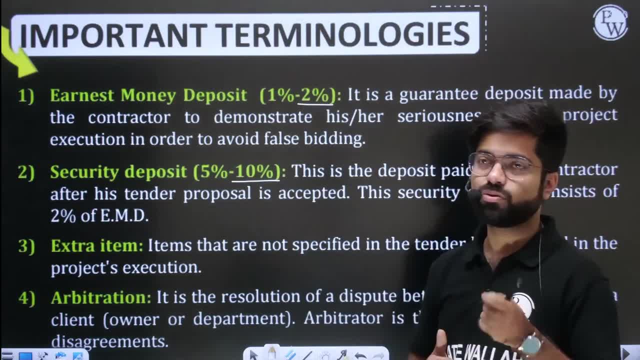 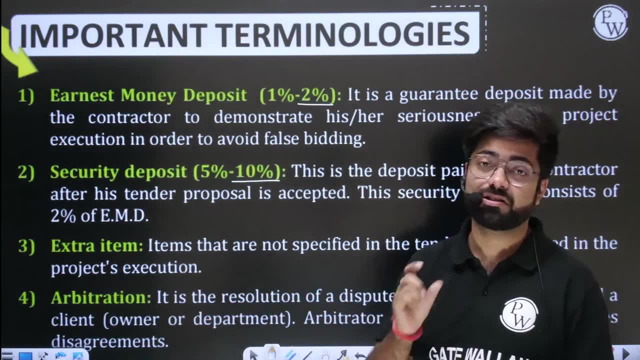 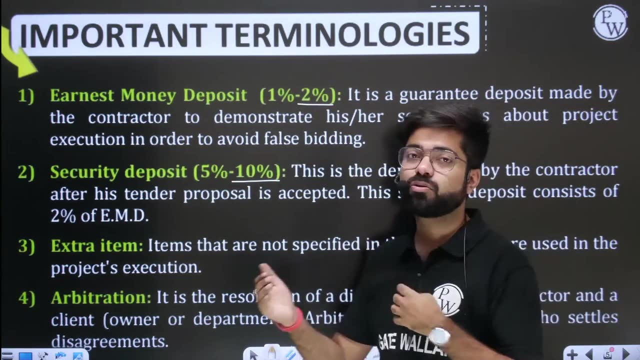 All terms which are used When you Include language of Crosswalk License Board For work gleich. Do not Take extra item. This is very important. Arbitration: When there is a riot, who does the mediation? Arbitration means that when there is a fight, there will be a dispute. 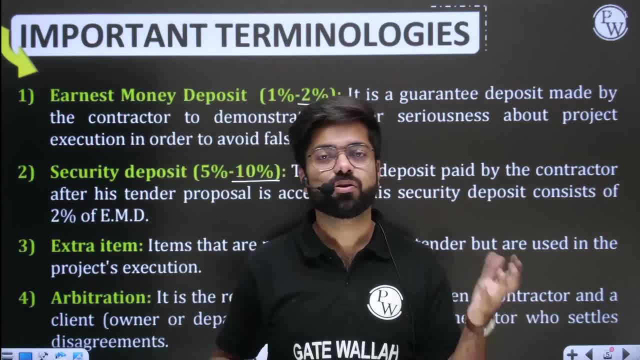 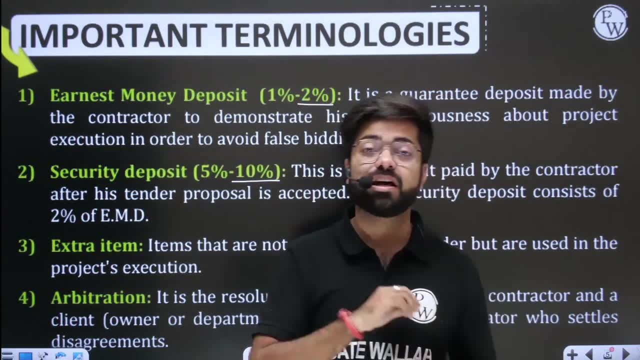 Now, a man is working. a man is working. anyone can turn back. he does not give money, he does not do the work properly. Can there be a riot or not? Absolutely, it can happen. There is a dispute, absolutely, and there is a lot. 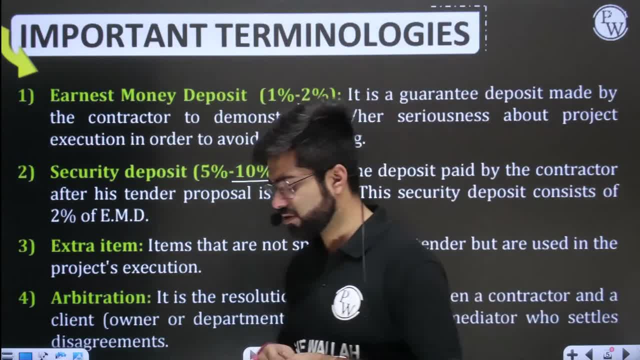 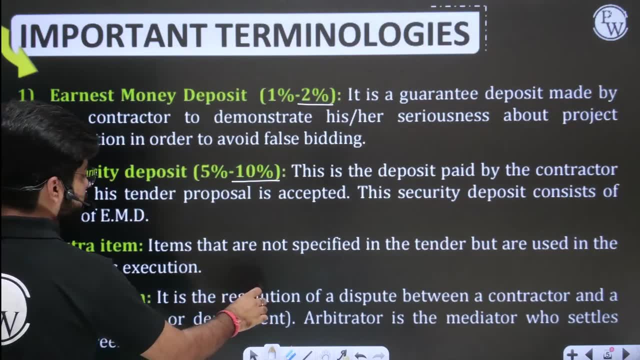 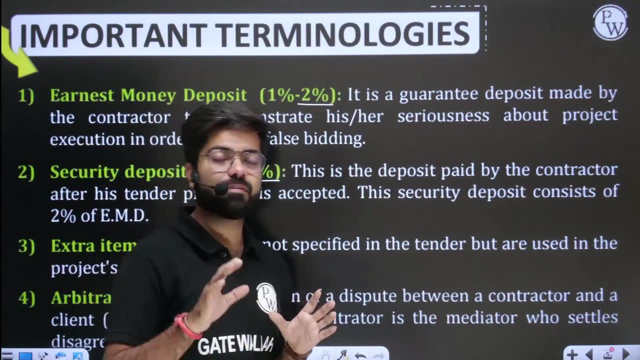 There is a lot. okay, There are 50 court cases. you see, they are always going on in the department. Okay, we will not go there for the time being. So the way out of the dispute is called arbitration And we will have to understand who is doing it. Now let's go to the court case. 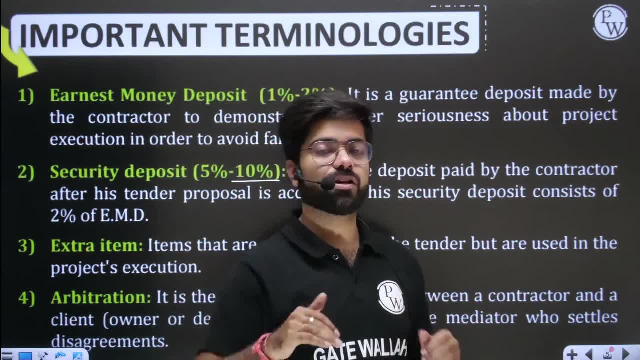 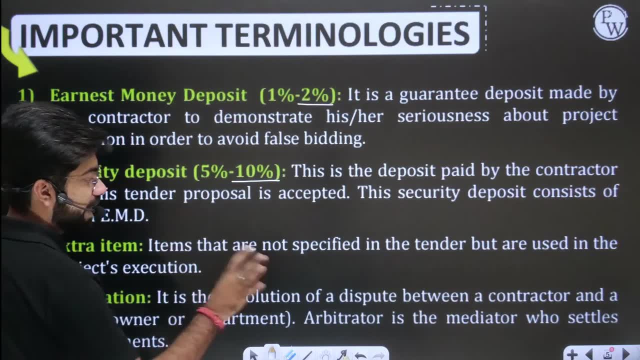 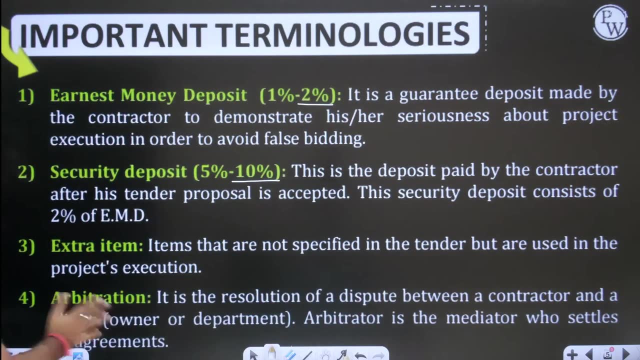 Before going to the court case, let's explain the department's hierarchy to you. Let's read this line first: Arbitration means to resolve the fight, So it is the resolution of a dispute between, obviously who- The contractor who did it, The contractor who is working and the client who is the owner. 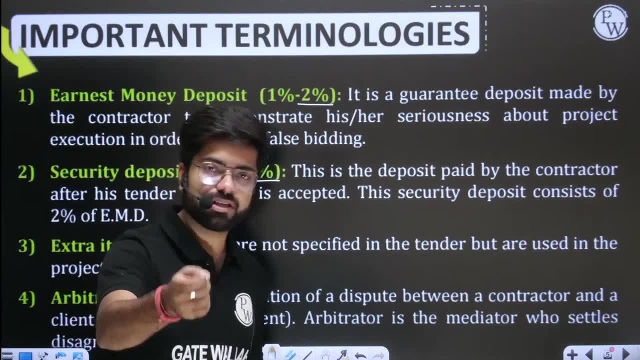 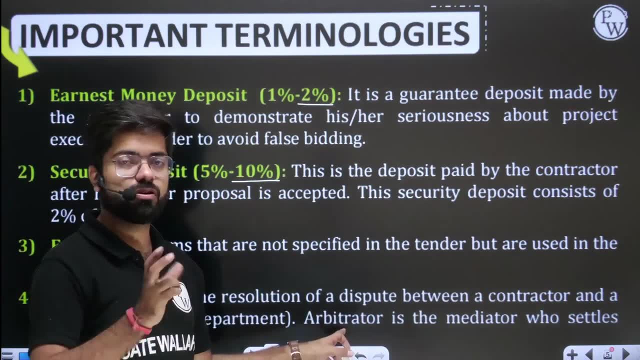 This is the department Generally. we will talk about the department because you will go to the department and do the job. Why will you give the paper? You have to select the department right And the man who listens to both sides in the middle and gives the decision. we call him an arbitrator. 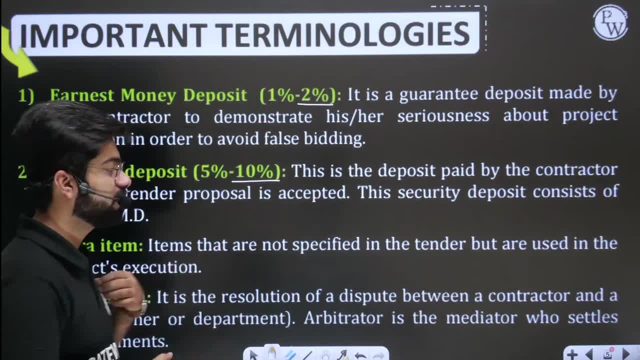 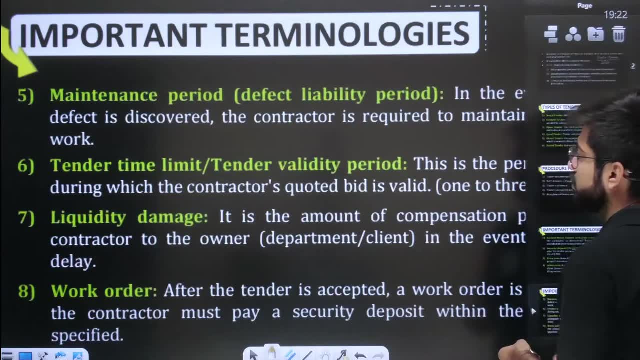 Generally, the judge who is in our court has become an arbitrator. okay, Who settles the disagreements? Now, if we do not go to the judge right now, if we come a little back, then let me show you a little bit wait. 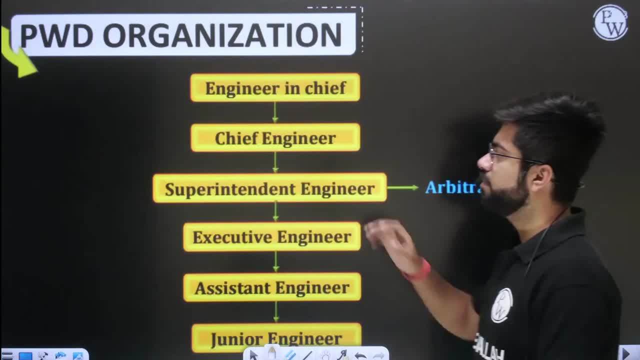 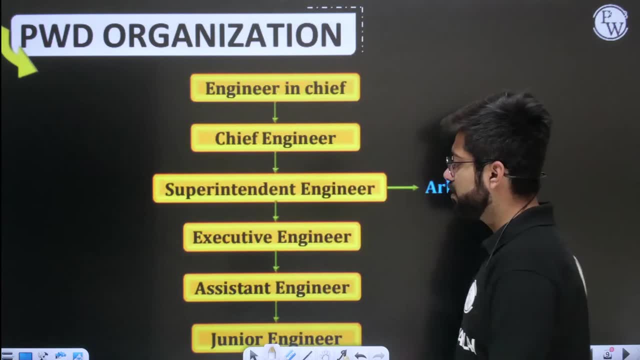 First, let's talk about a dispute. For example, let's talk about PWD. PWD is almost the same hierarchy everywhere. Don't go up, come down first. From now on, you are preparing for AE and JEE. If you study well, then you will reach this level, whether you are in the center or in the state. 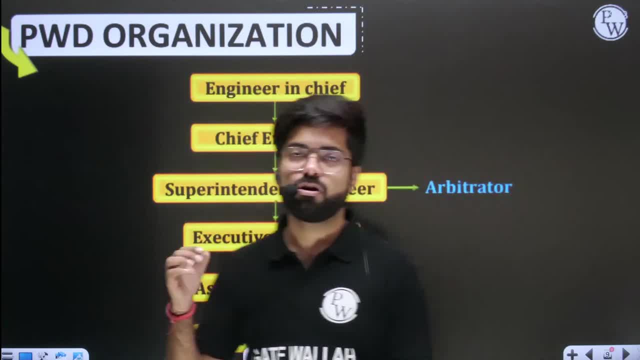 Wherever you are, you can reach the level of an assistant engineer. If you take out big papers and take out small papers, then you will become a JEE. So, in short, you will either become a junior engineer or an assistant engineer. 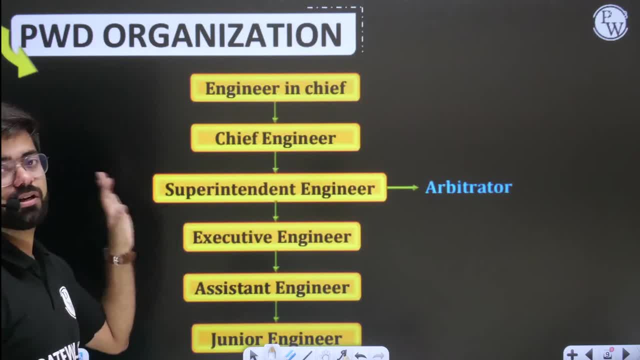 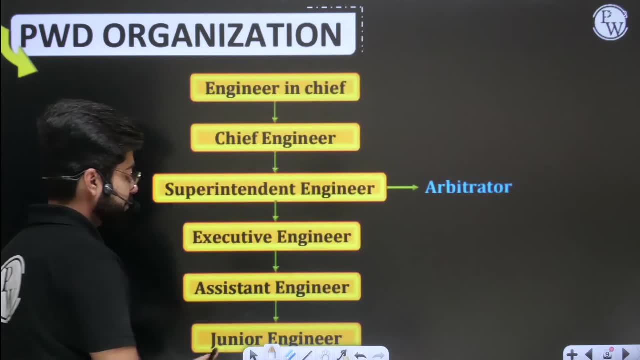 Now, the actual work that people do is very important. This is very important Because when you will enter the department, you will have training, so you will be explained all this. It is everywhere right. So you understand this a little bit today. 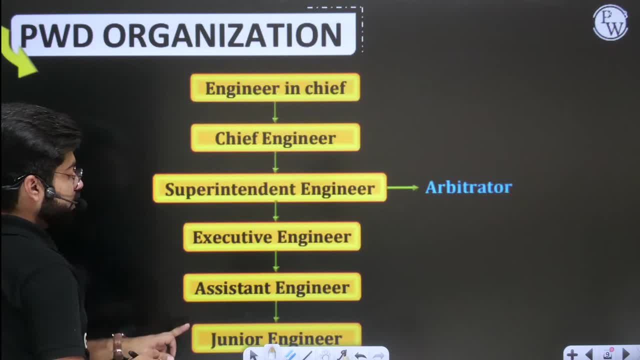 If you do not have training, then you will jump directly. you will make mistakes. Now, you will become this or you will become this. The person who is actually working in the field is this person- Junior engineer- is actually working in the field. 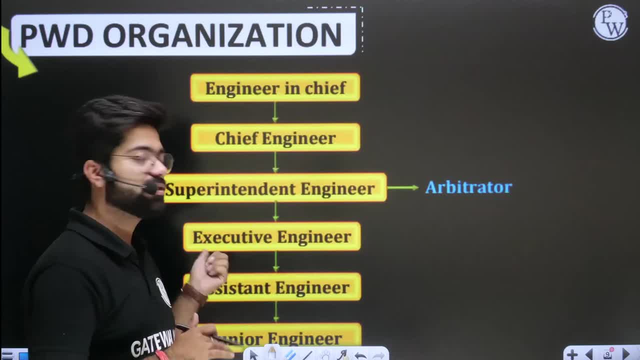 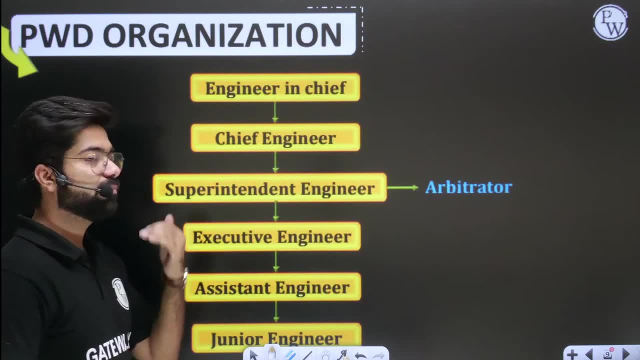 And the person who is looking at him from time to time is this person: Assistant engineer. okay, Actually, when you are building a canal, then he has to come for 24 hours. He has to do one at night. This in two days, in one day: go every day and do a round. 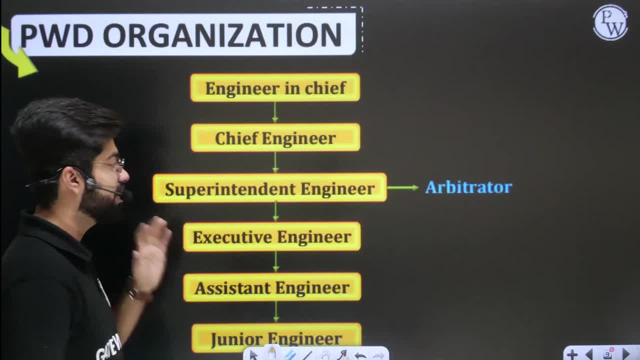 Okay, Do all this checking, supervise whether the work is done properly or not, Or whether the work is done properly or not. So this is his responsibility. He will go with them And this will give him work. Do you understand the meaning of this executive? 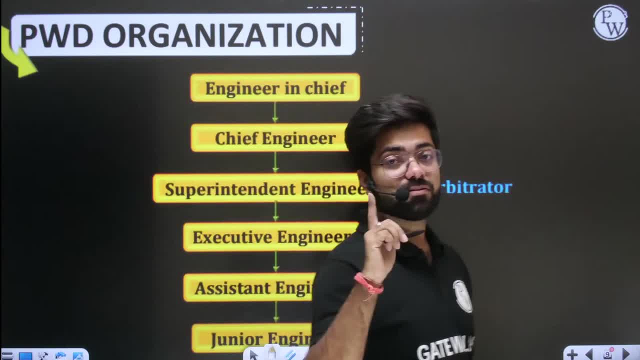 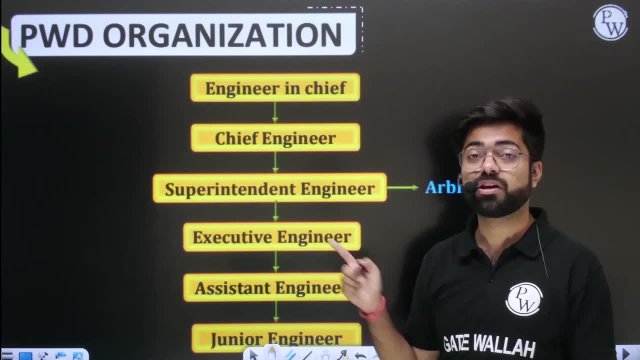 The main one who gets executed, You understand, in the entire department. the strongest engineer in the entire department is this one. Everyone is behind him. Why is he behind him? Because he has the actual financial power in his hands. He is handling all this work. 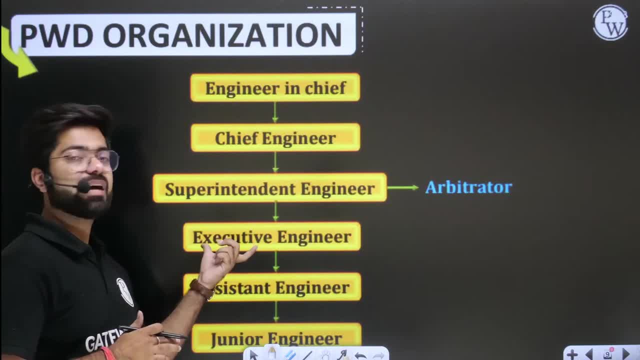 Allocating. So, brother, Whoever gets the work, the fund will come to him Money. So they all run after him. Brother, bring it, He is the boss, He is his boss. So he will say, talk to us. 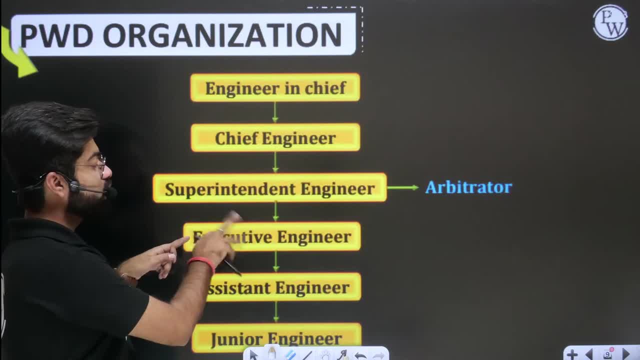 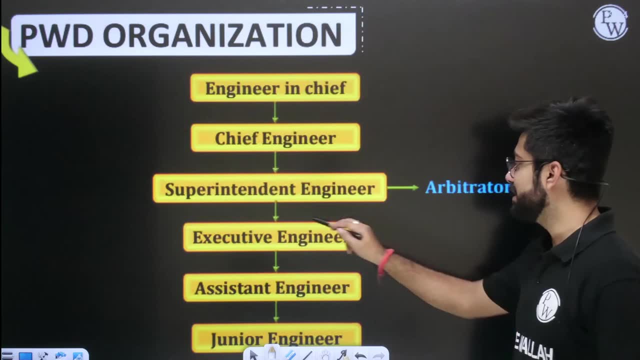 Bring the money And they all try to make him happy That we get the work. Everyone runs after work. Whoever gets the work, he will get the money. So ultimately, from all this, we can say that he is the son of the entire family. 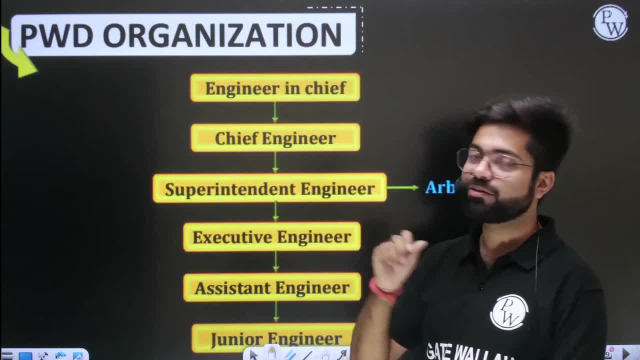 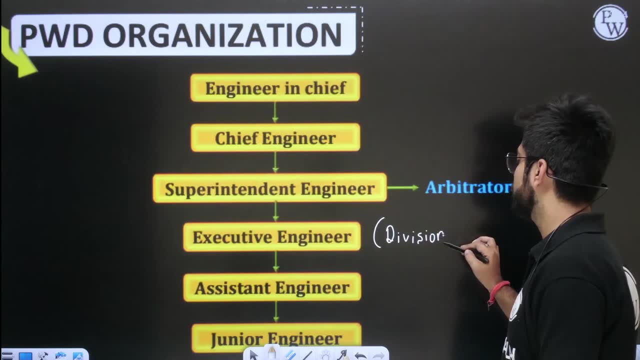 Son of the family, Isn't it? So there is a lot of respect for this. The man who actually lives at the division level: Okay, You understand that if there is any state, Okay, Now there will be a lot of divisions in that state. 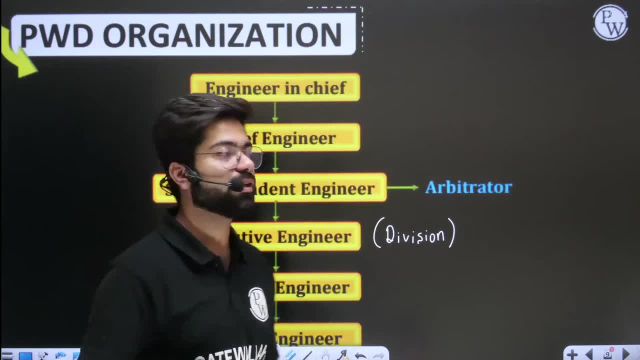 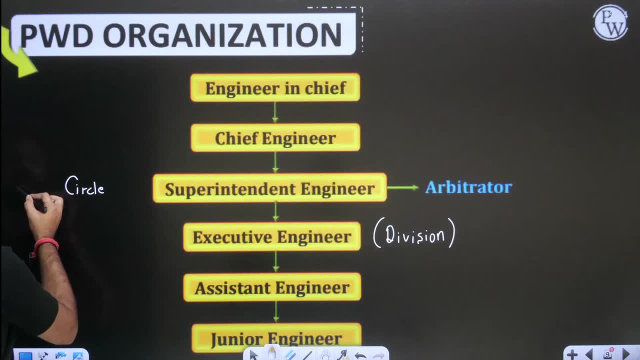 First of all, there are a lot of circles. The circle is called a mandal in Hindi. Okay, They are at the circle level. This is your superintendent engineer. So there are a lot of circles in the whole state. In Hindi, we can call it a mandal. 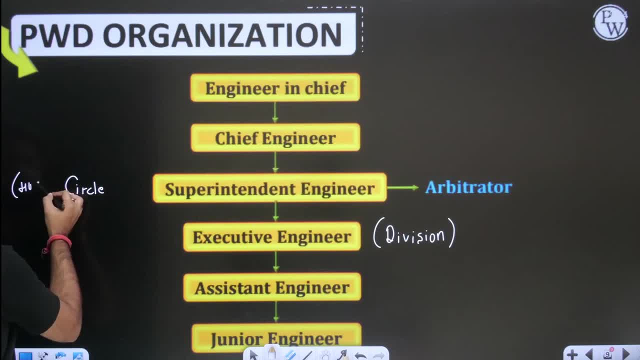 Okay, Then inside it The mandals are a little big. Okay, The mandals are a little big. Then there will be a lot of divisions in the whole circle. Okay, In Hindi we call it a mandal. What do we call it in Hindi? 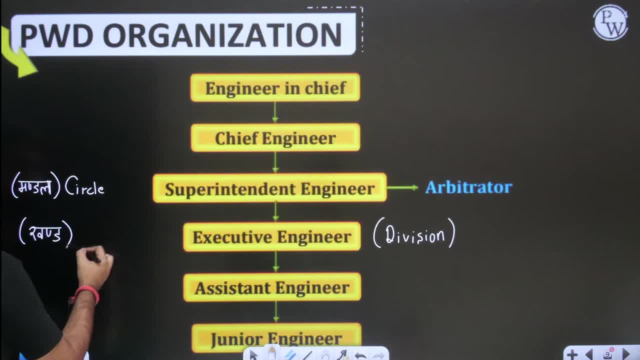 We call it a mandal. Understand all this, You will become an engineer. You should know. Okay, Then a lot of subdivisions come inside the divisions. A lot of subdivisions come inside the divisions, Which we call it a sub-mandal. 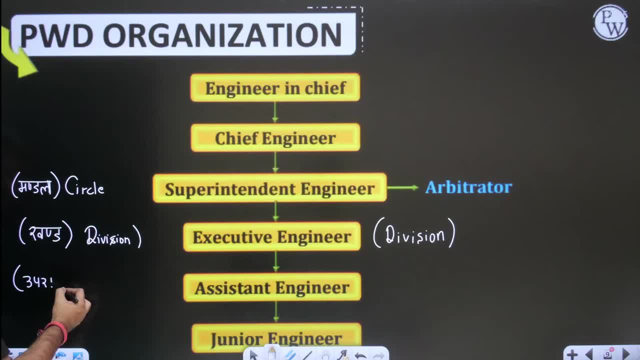 You will come here now. Okay, You will come here. If you become an AE, then subdivision. See, you can't go directly above this. You will have to work for 7-8-10 years, Then you will reach here. 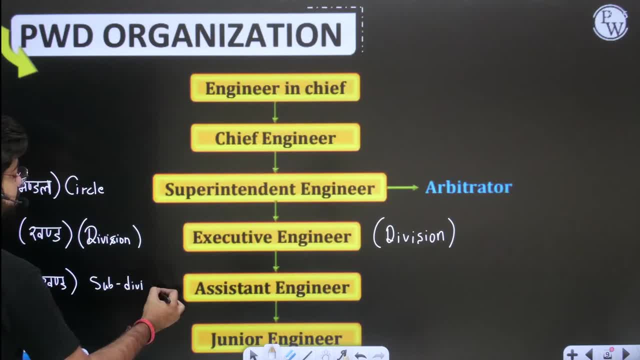 Okay, This is a very good thing. Here you will enjoy the real life, But there are also a lot of pains, Because as much as you work there, you will have a lot of pain. The chief minister will call you directly. The minister will call you directly. 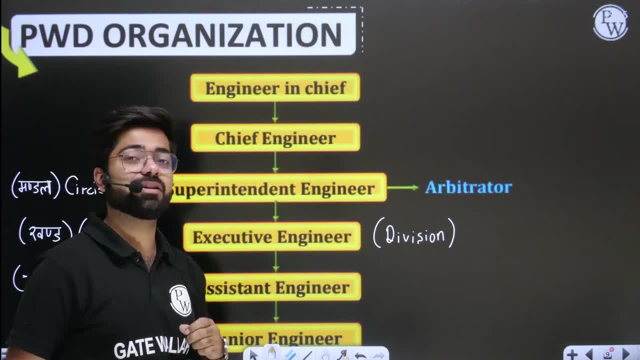 Go, make a print here, Make a ripper print, Make a journey through the university, Directly click, Because the actual power of doing all the work is in your hands. And when the political pressure rises from above, then there is also a little turmoil. 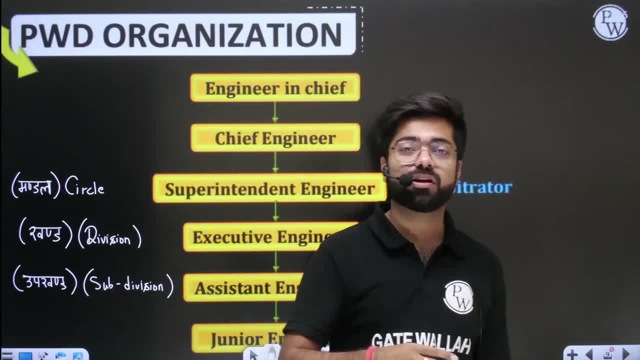 Okay, Let's not go into all this. Let's try to understand a little. We are just understanding a basic format And let's say that a junior engineer is a JEE. You don't have to go to the JEE. You don't have to go to the JEE to study. 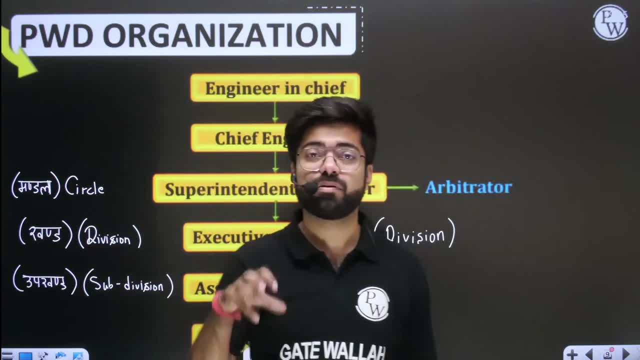 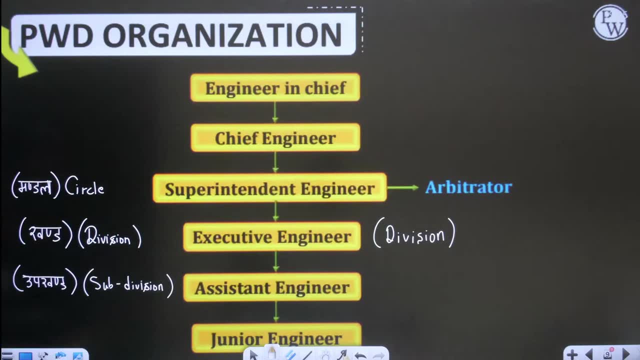 You don't have to go to the JEE to study. You don't have to go to the JEE to study. You can study in the JEE. You can study in the JEE. You can study in the JEE. There are many small sections in the subdivision. 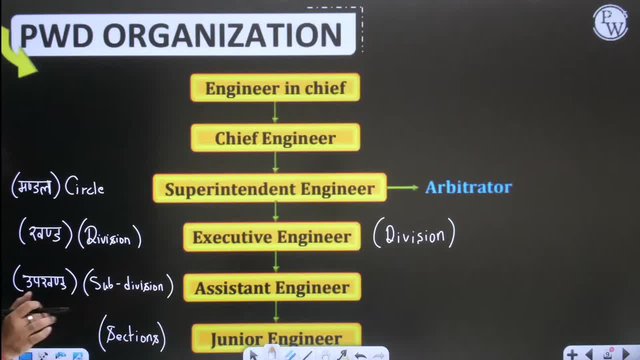 Like canal system, there are many small streams in the subdivision, Then there are many small streams in the subdivision, Then there are many small streams in the subdivision. So the work is divided like this: They are doing the actual work and supervising 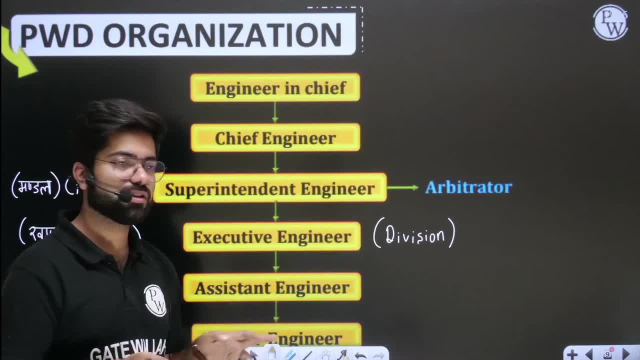 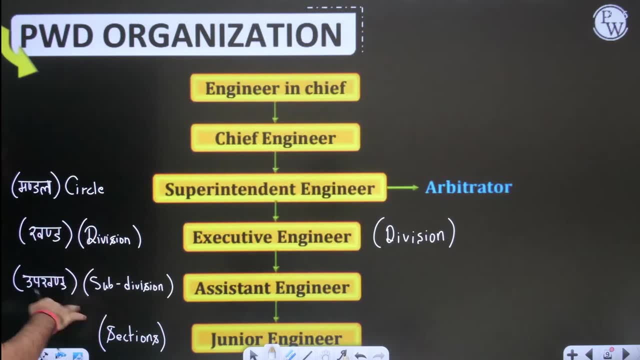 There is nothing in their hands. They are middlemen. There is no load. If they make a mistake, they will get stuck. If they sign above, they will get stuck. Their job is to do it from here to there. So you are able to understand all these things here. 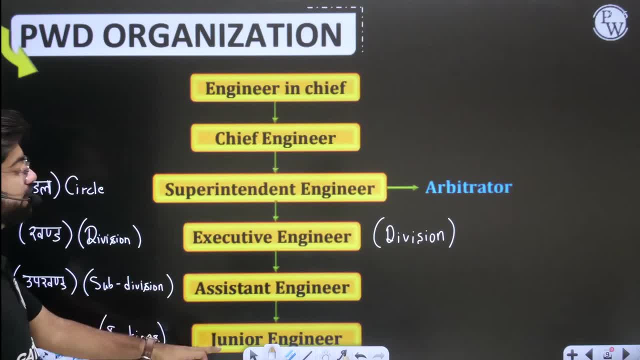 So they will be the strongest man, And actually they are the ones who execute the work in the field. They are looking at all this from above. They will have four children. They will have four people in each of them. So this is how the work is done. 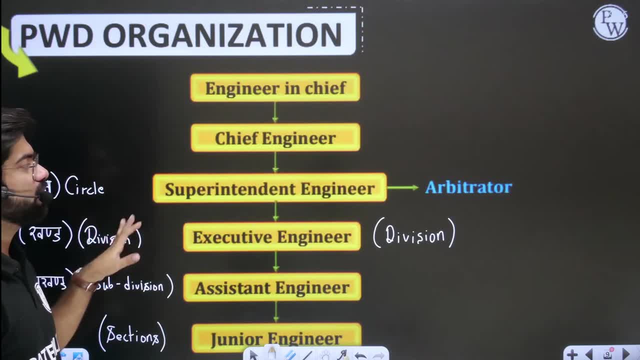 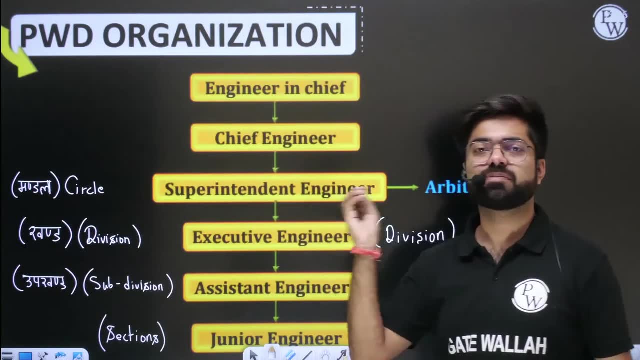 Then superintendent and engineer are office people. They sit in the headquarters only. There are very few chief engineers. There are few chosen engineers. Chief engineers at a slightly larger level That the whole stadium will have 5-10 chief engineers And above that there are chief engineers. 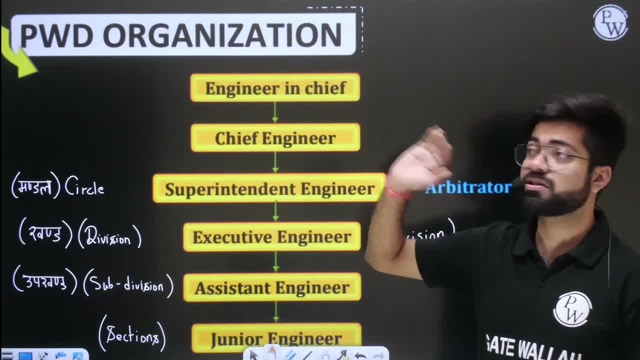 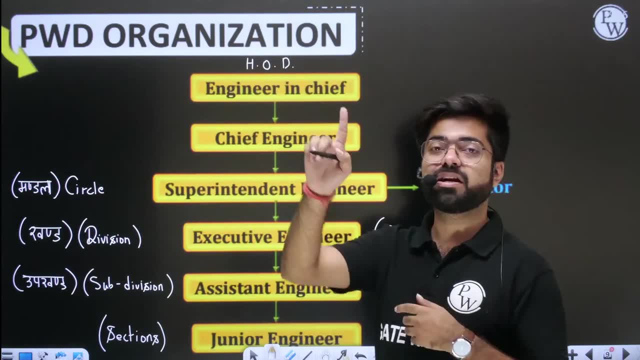 You understand this. The whole department is the topmost position Above. this is the head of department. There is only one HOD in the whole department, Which is called head of department. There is only one person who represents the whole department And he will be directly in the contact of the minister. 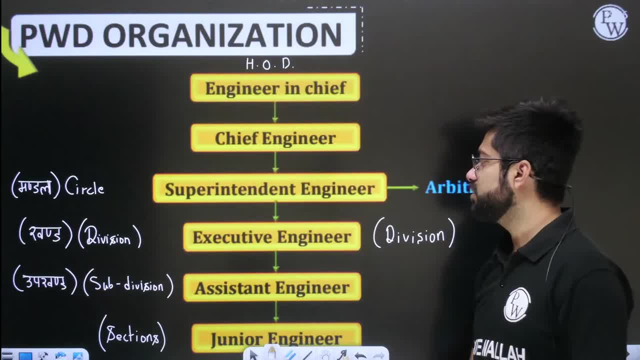 Okay, He will be directly in the contact of the minister. So this is how the whole hierarchy runs, And from here you are called an officer. From this level we start calling the officer. Now there is a fight. We were talking about the fight. 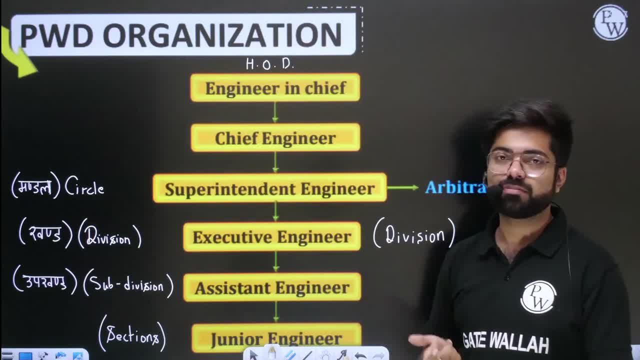 So now, who is the one who gives the job? Executive engineer actually gives the job And he says that this is the boss, These are the big bosses and these are the small bosses. Okay, The big boss tells the small boss to go and get the job done. 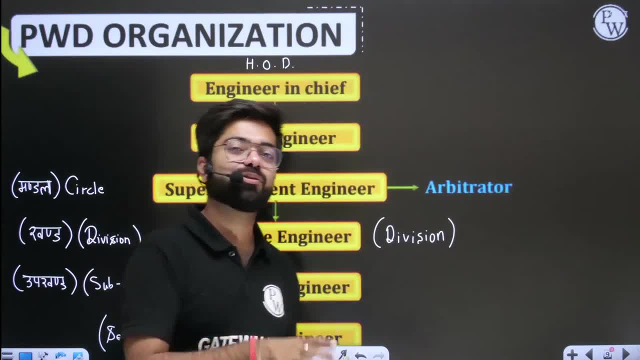 So the small boss becomes active immediately. The small boss becomes active immediately And everyone starts searching: Who is the one who makes the notice? This one, Who is the one who checks everything properly? This one, Who is the one who will tell all the things? 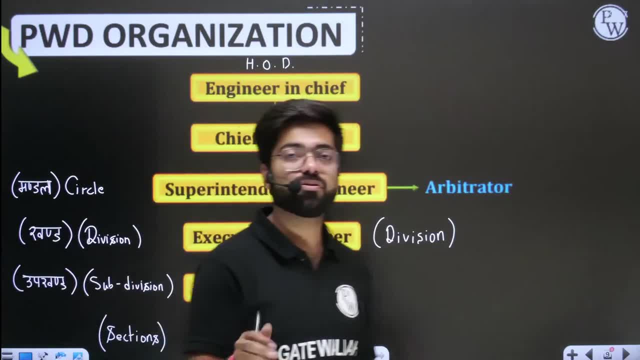 Who is the one who will write that thing on paper? Who is the one who will check? Who is the one who will sign? Everyone is AE. AE has to do a lot of work. Okay, There is a lot of responsibility on it. 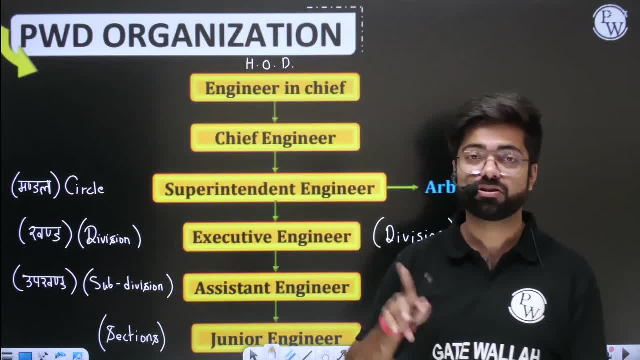 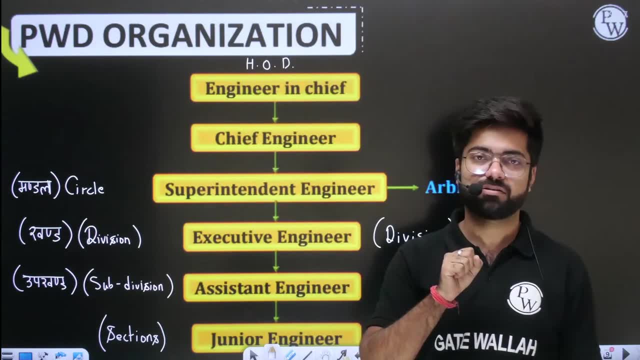 Did something wrong. There will be an abuse from here And he can abuse them That. go and bring it properly. Okay, Look what is the best responsibility of AE. AE is able to control its juniors and juniors properly. Okay. 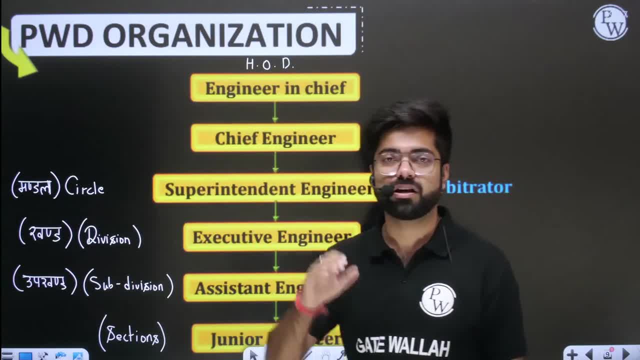 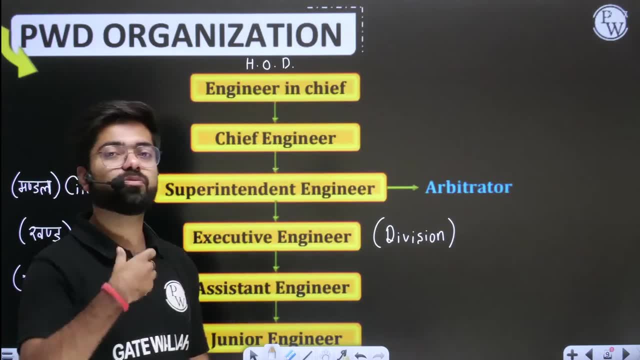 There should not be much confusion. Work should come out Okay If he is able to make his JEE work properly. Okay, And he is relying on AXIAN on his own. Relying on AXIAN on his own means that AXIAN's work is not going on without AXIAN. 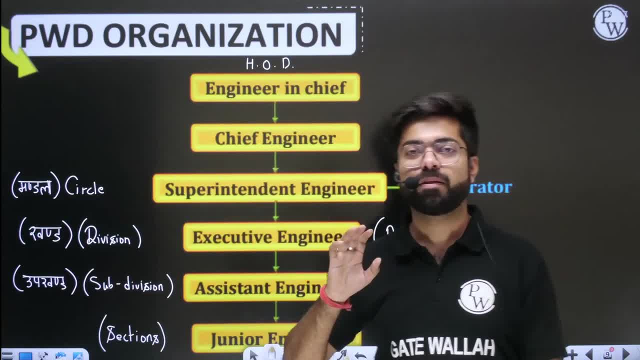 If AXIAN is ever in trouble, then he says, brother, you tell me what to do, Tell me how the work has come in it. The minister has called: Tell me how to work, Tell me quickly. So this position is very strong. 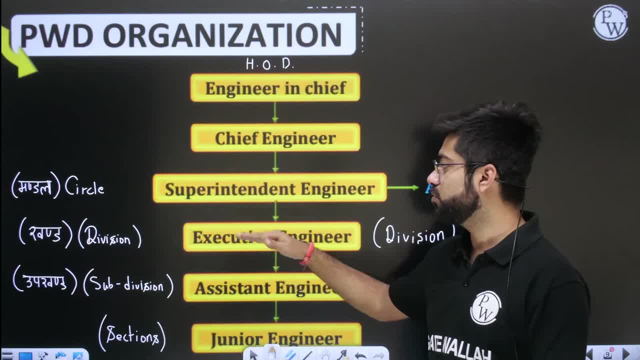 Because you understand that the department has a very important position, Because you have to take the work from here And you have to delegate it down and actually get it done in the field Okay. So this is a very strong position. There are a lot of responsibilities here too. 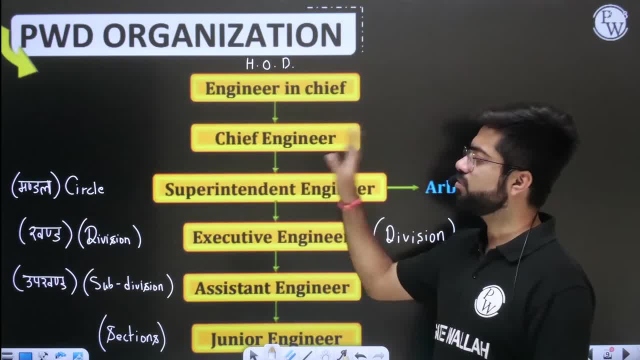 And if you reach here, then there will be a long chaos, Okay. Then after that the load reduces a little. In the same way, things become a little easier, Okay. But there are a lot of informative things there. There are committees. 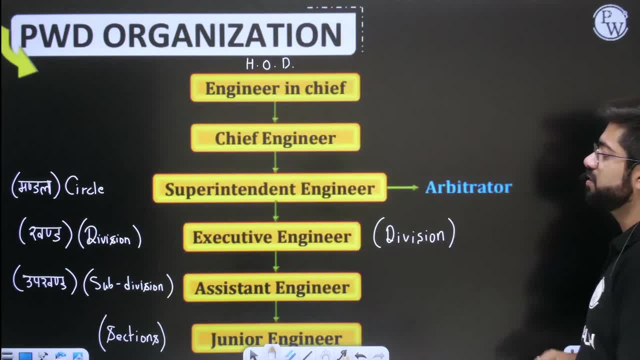 There are seats, There are a lot of things, So it is written here. Who is the arbitrator, Superintendent, engineer, First of all, like they are doing the work Now, let's assume that AE has actually seen the chaos in the field. 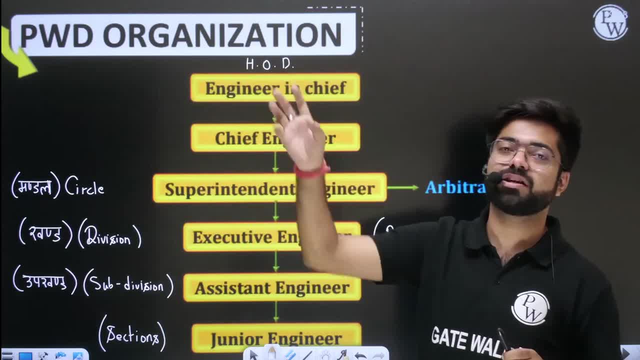 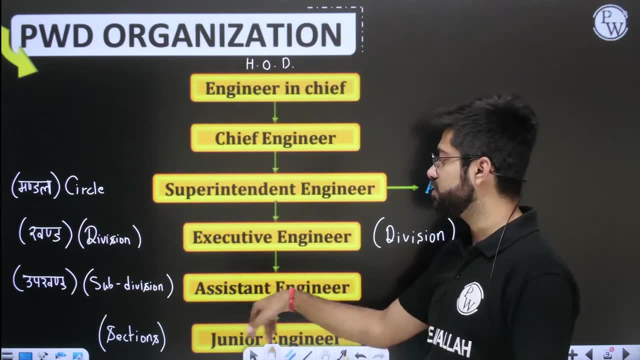 The contractor is running. He is acting here. He is acting there. He is taking away the contractor Forcibly, trying to make his influence. He is making a lot of trouble. Contractor who is working? It turned out that he will get to know JEE and AE first and foremost. 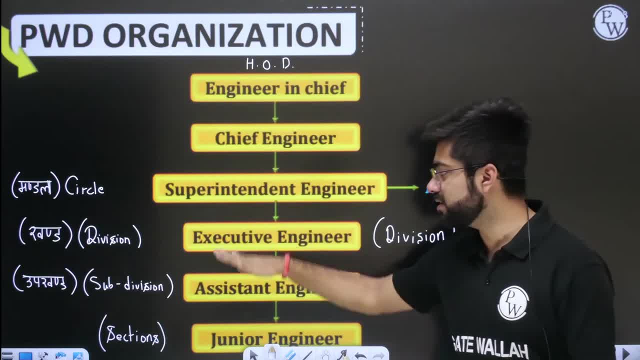 They will tell him. They will tell him: Okay. Actually, these are all the people who are working. These three are on the level Okay, So they are not very involved Because they have a very big area They have to handle four AEs below them. 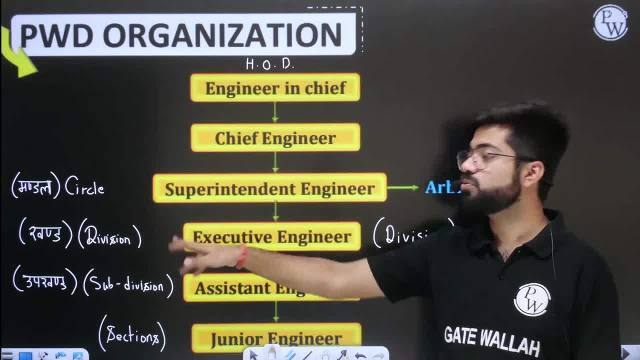 They will talk to one AE. They will talk to the other. The third will take everyone's report. every day They keep running and running. Okay, Let's go to the court case at 50.. They are running here and running there. 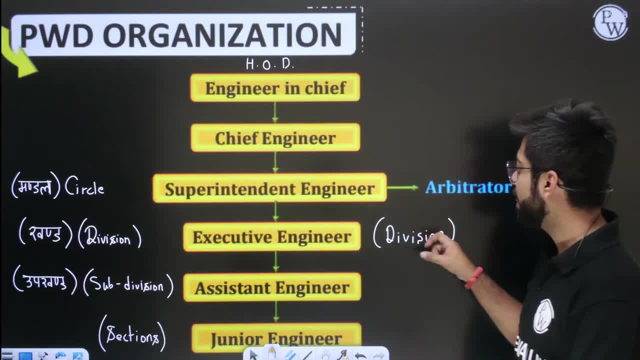 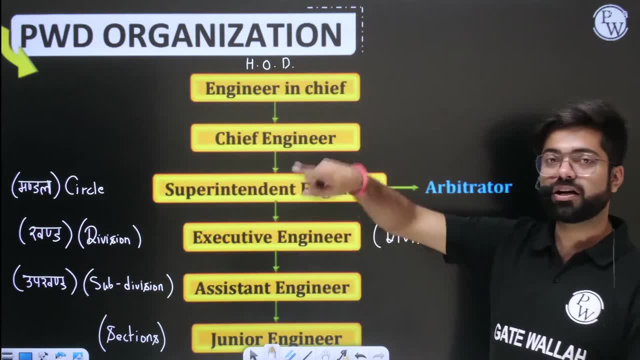 Okay, So they don't have that much time. So they don't have that much time. They are stuck, They are working in the area in which they are working. They and they and the contractor will have to tell the ASE, sir first. 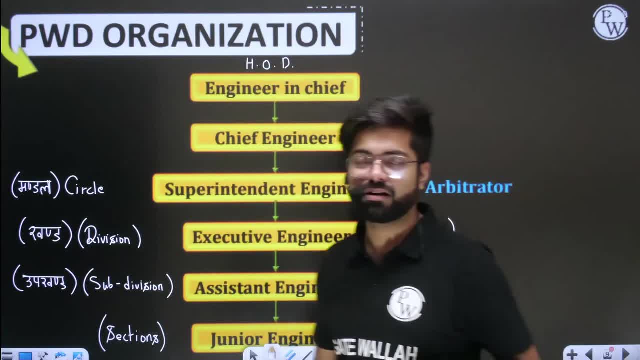 Who is the ASE, sir? Arbitrator? Okay, Yes, tell me what the matter is. Okay, you are saying that Now it is obvious that these are of the department, So they will give their partner, Isn't it? 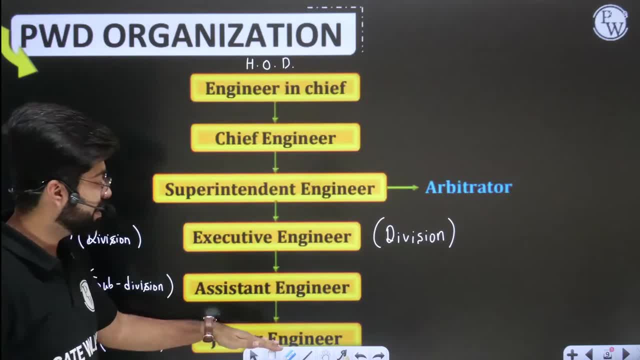 So you know that in the department it happens This, this and this Good friend And this and this. See, a direct boss is not a friend of a friend. There is a problem in the direct boss. Do you understand? Yes, 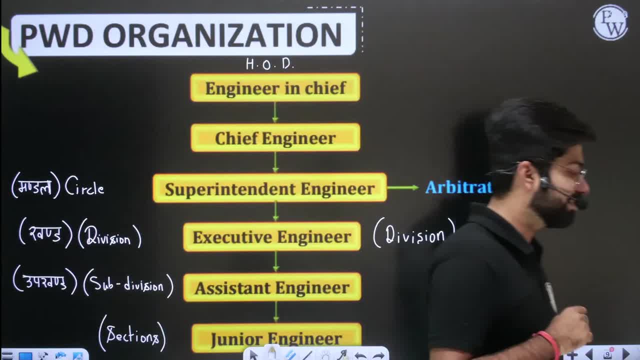 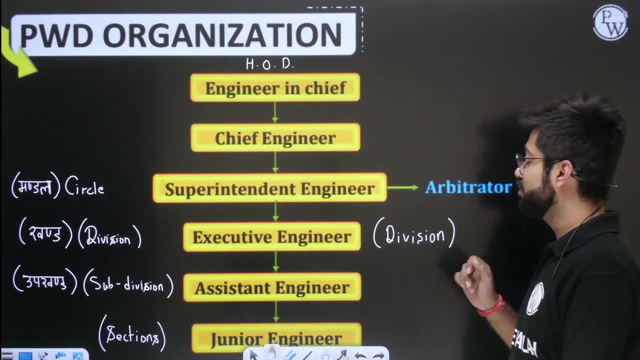 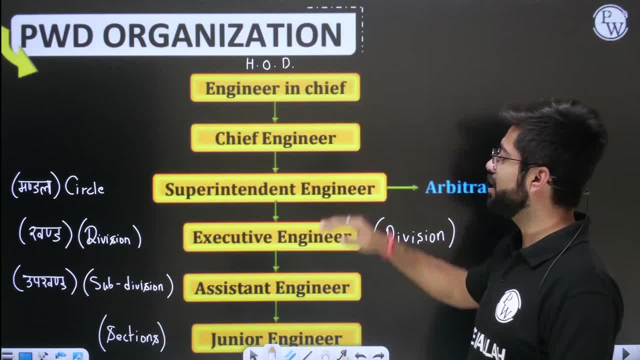 if an AEO gets a good Munitions, life will be richly. if not, we do not get it, we will eat doctors every day. So it remains: this is an alternate, which is that we are friends at an alternate level. 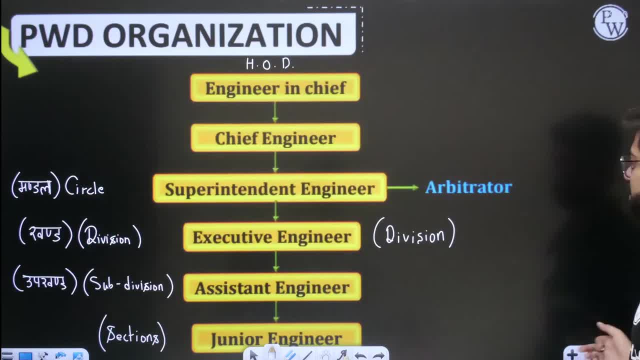 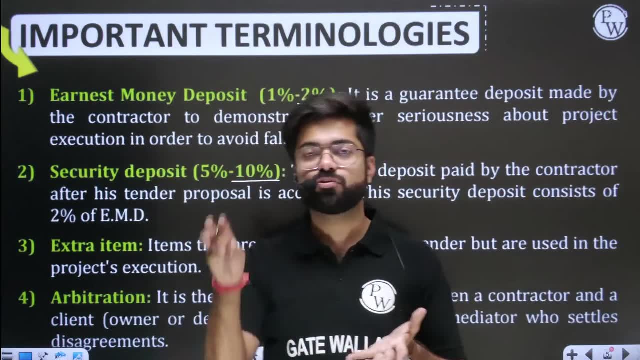 So for now, supretended engineering hereralists that if any such system is happening in the field, what is it called in engineerё? inside any engineer it is complete Taking tips. you know, optimal between this, between the contractor, because see who is the client, the engineer will tell everything. 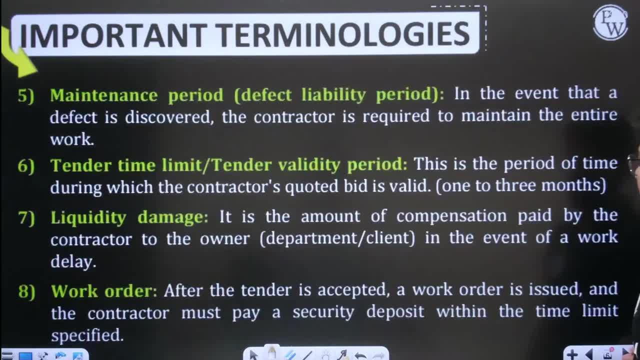 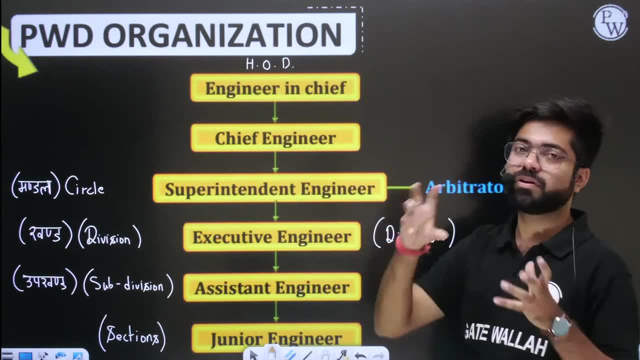 completely see approval. any big project is to be done- for example a dam has to be built- then obviously all of them will see that a dam has to be built here. it is the responsibility of all these people that they will make a plan. and okay, let's say they told that a dam has to be built in our division. 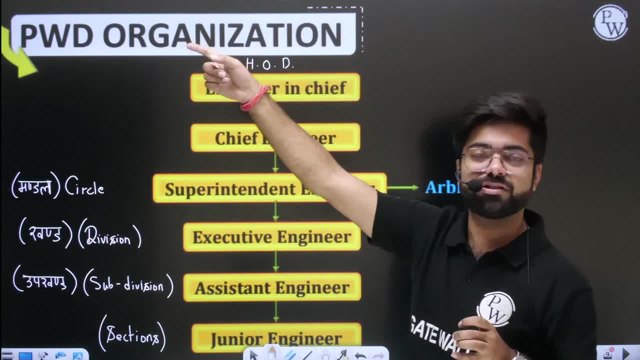 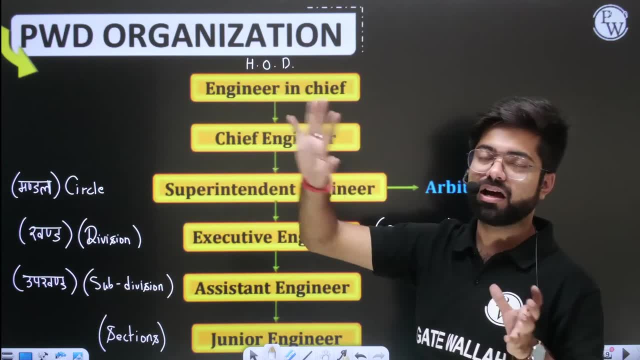 they told all of them they passed it and then it will go to the administration. it will get administrative approval. that is where there is a technical sanction. it is correct. there are two levels of sanctions. it gives the approval first here. This thing is right. After that it will come back to the departure, the technical. 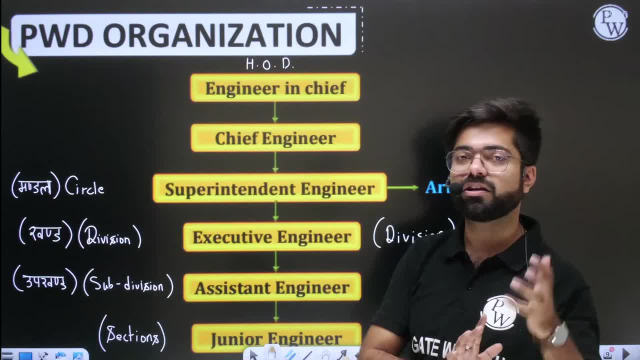 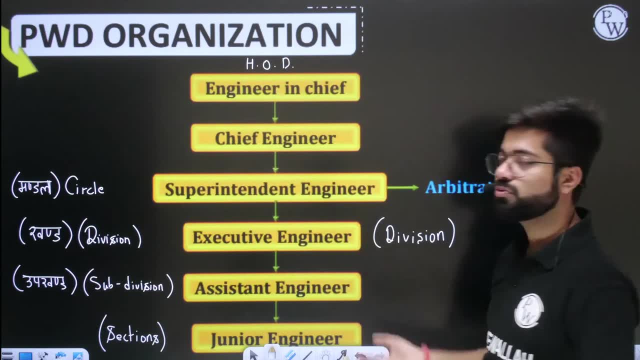 sanction of the disorder. they will say that all of this is all right. Also, they can do that all that is out of sound. then the time comes for technical financial approval. then the work begins. After that there will be time to do it all the work comes here after this time of. 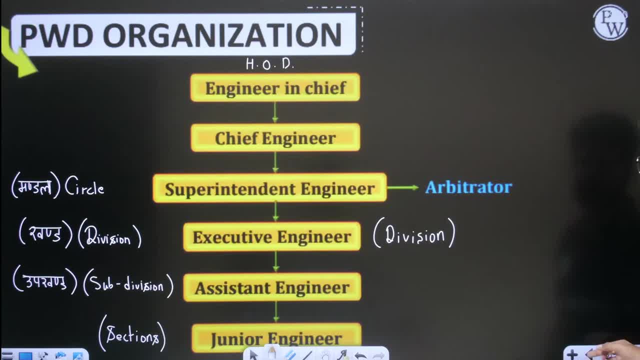 tender. all of them will do tender. they will order a word card. there are a lot of things. okay, then the work will start. then there is a lot of things. you will see one level of tender and then the work will whole, will go on right. 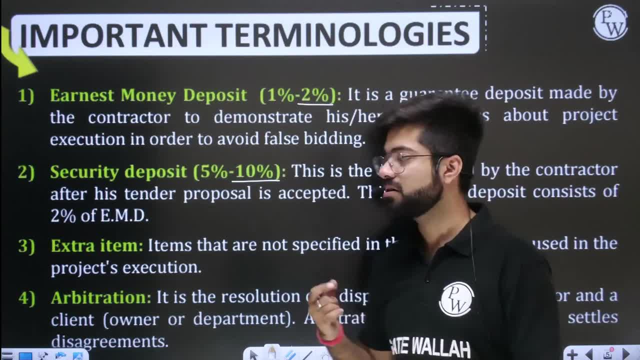 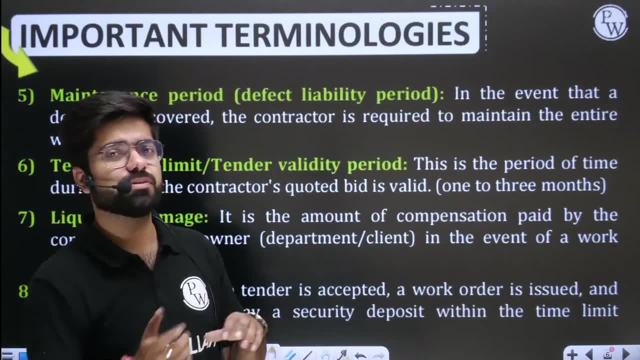 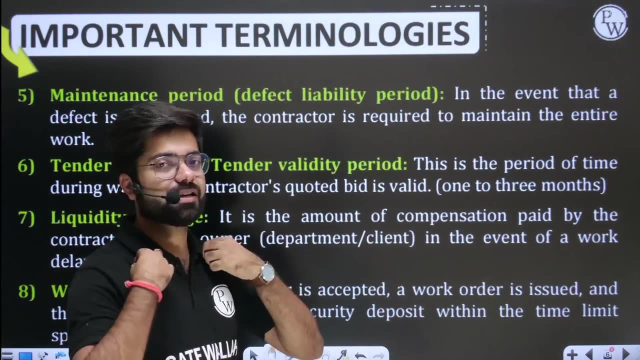 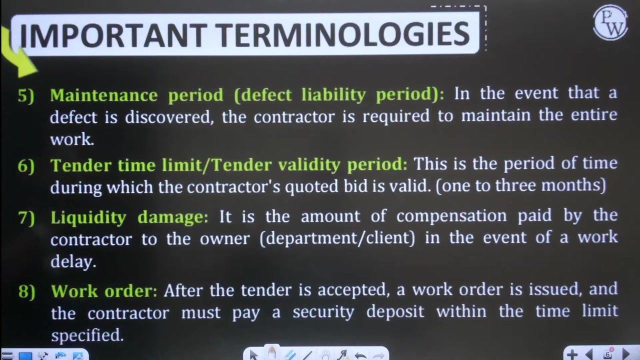 That is why, when this money is sent every time, so only in a month. If you do this, after two weeks you will see tehy bank, because you have to. who did the arbitration? SC superintendent engineer. okay, so this is all you should know. I gave you an idea that if you go to any department, then generally this is the hierarchy. it is a little up and down, like if you go to irrigation department then you have to go to two levels: level 1, level 2, okay, there is something. there is something. some changes have been made according to themselves. okay, but this is the same hierarchy that you have just seen. let's move forward. let's start reading the terms further. next is maintenance period. what does it mean? what does maintenance period mean? look at its account. 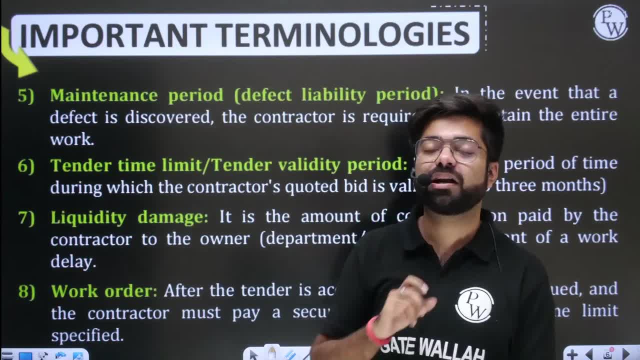 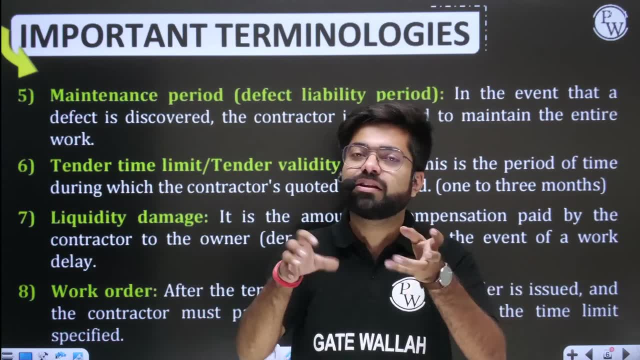 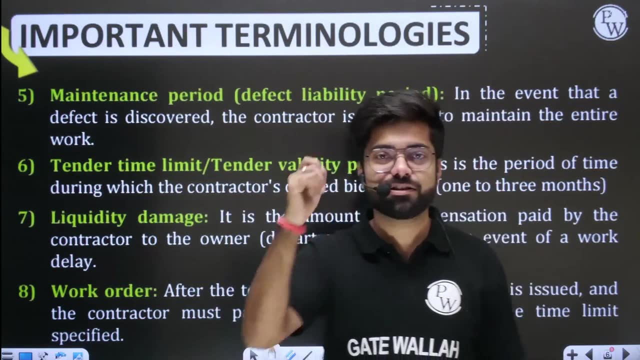 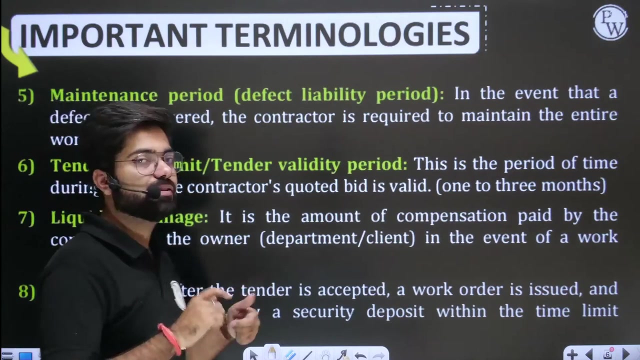 what is the name? what is written? defect, liability period. defect means failure. now, sir, the contractor, the man who worked, he turned out to be a little smart. he thought he does nothing inside. he makes a hole inside. he makes a nice dent on the top by applying paint. if paint will be applied on the top, then what is inside no one will know. this is what contractors do. you will understand everything when you see the actual work. you will understand. so there is a responsibility on the contractor that whatever work he is doing, at least he, at least he will. 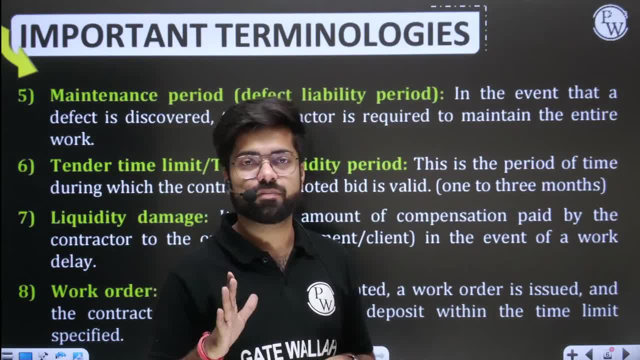 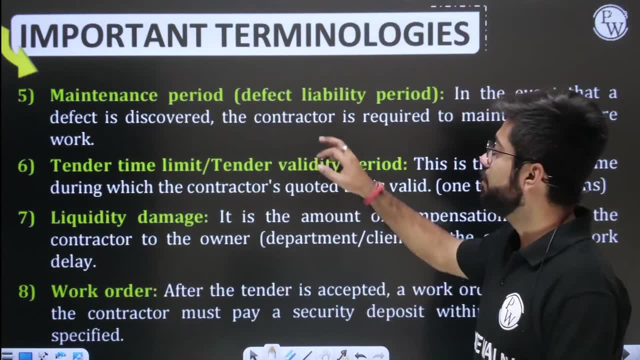 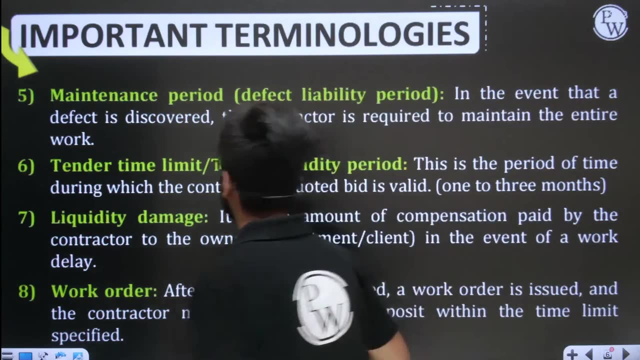 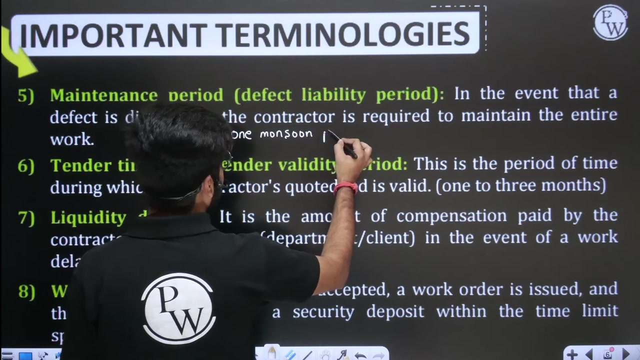 take half a year or one year by making a canal. he will endure a rainy day so that the truth comes out. so the period which is complete is called maintenance period or defect liability period. one period will come out of the six months. let's write it here: a rainy day is generally seen. okay, one rainy day, one monsoon period will come out. that work will take either. six months will come out at least. 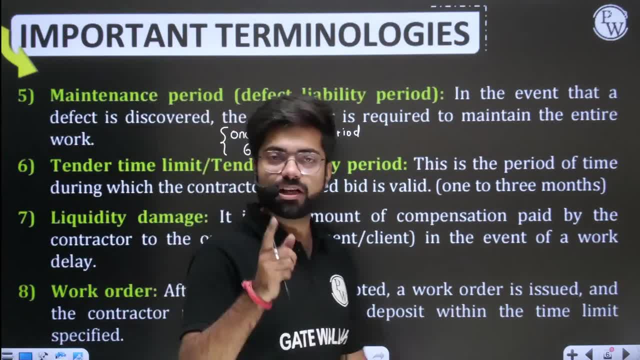 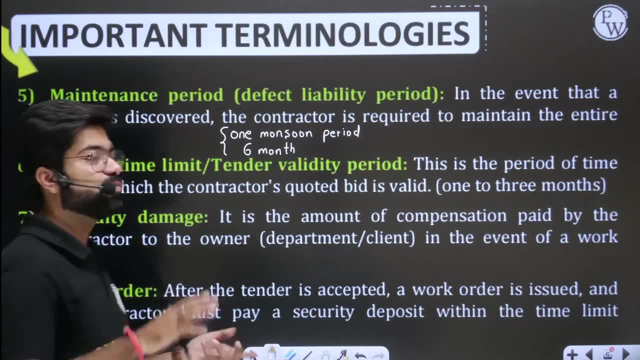 Then they will return your security money. Don't be too fast. Then they will return your money completely. Till then you will be stuck So that you don't know that it came out of nowhere. Then it became a matter with you In the event that a defect is discovered. 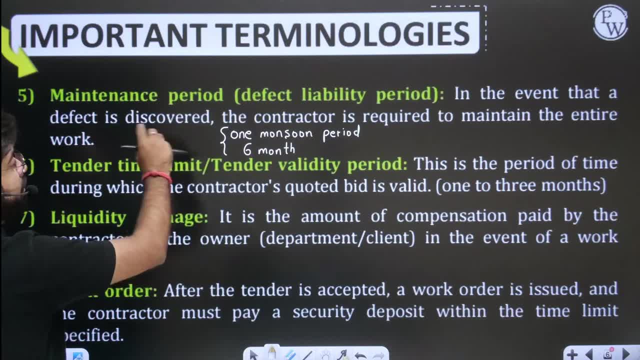 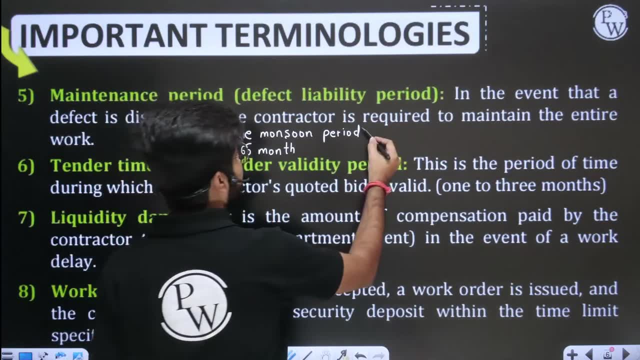 If, in this one rainy season, if there is a defect in the past six months, then it is the responsibility of the contractor to fix it immediately. So the structure is checked for six months. We can say this way: Then tender time limit. 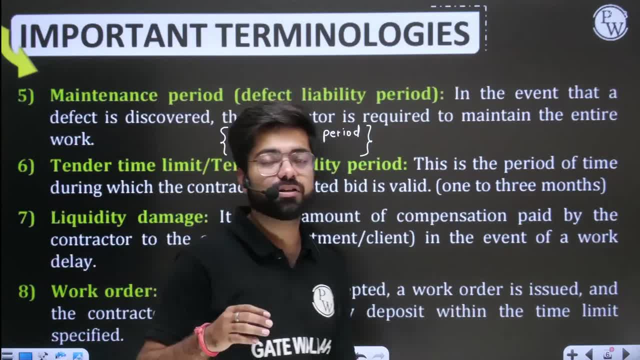 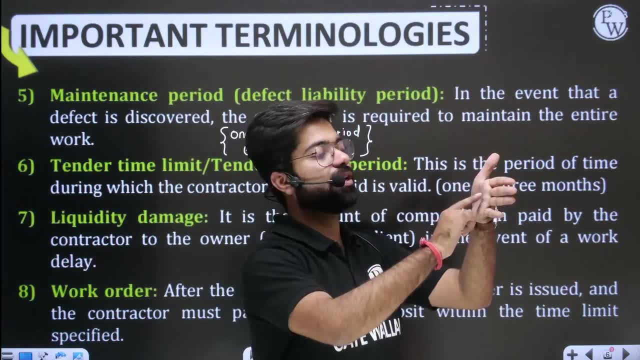 Yes, this is very important. What happens in tender time limit? When the form was floated in the starting, everyone went to everyone. So everyone fills the form. Yes, we will do this work in 100 rupees, Sir. we will give it in this amount. 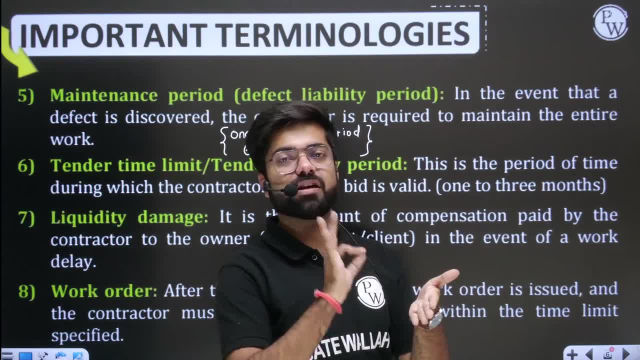 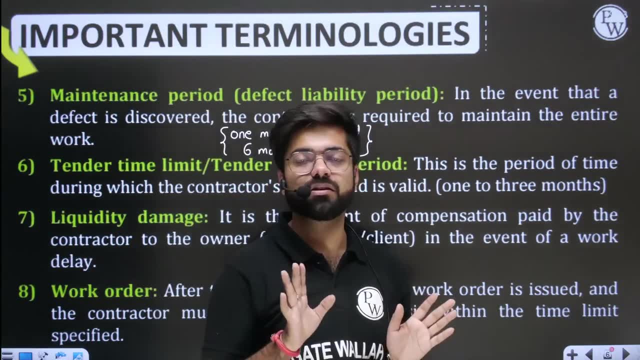 There is a long form In that the contractors write their own accounts Like this, like this, like this: Now, when it starts to fill, then it has filled, Okay. But whatever it has filled, how long will it be valid? 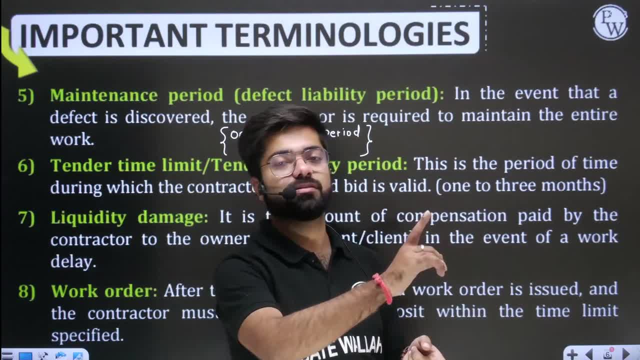 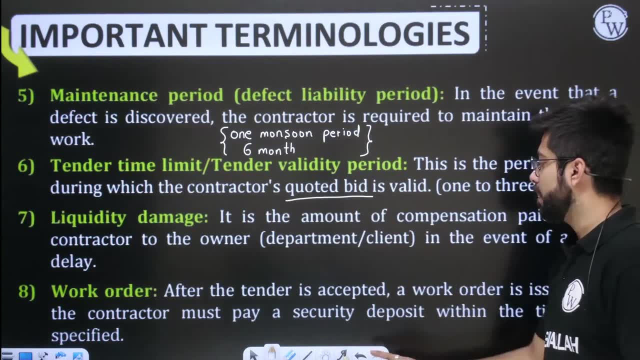 He said that we will do the marriage in this amount. We are not taking the example of marriage. Take any work. we will do this work in this amount. So whatever he did in his bid court, whatever promise he gave, whatever the promise he gave to do the proposal. 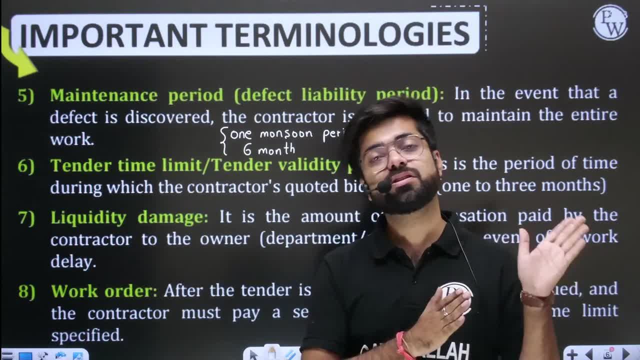 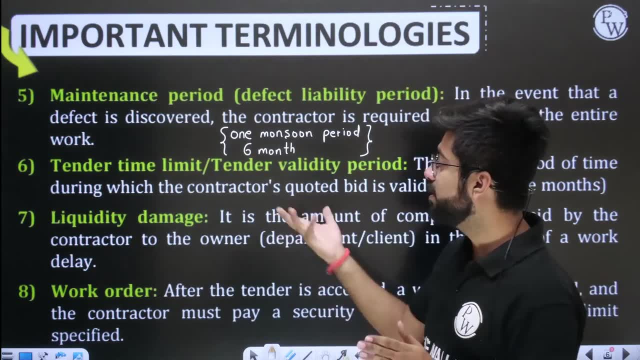 how long will they not agree? It turned out that he said clearly that this work is of this amount. After six months the rate increased. So what is the time limit of the bid court he has done? What is its time limit, Can you tell? 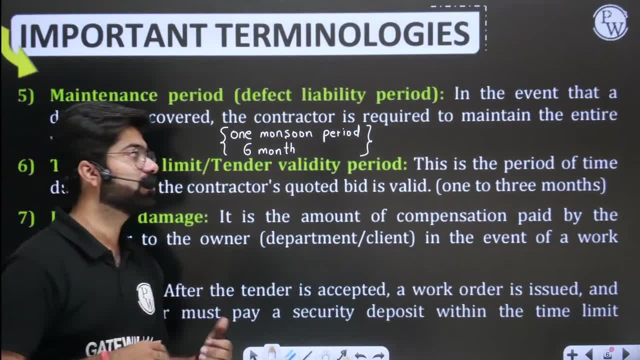 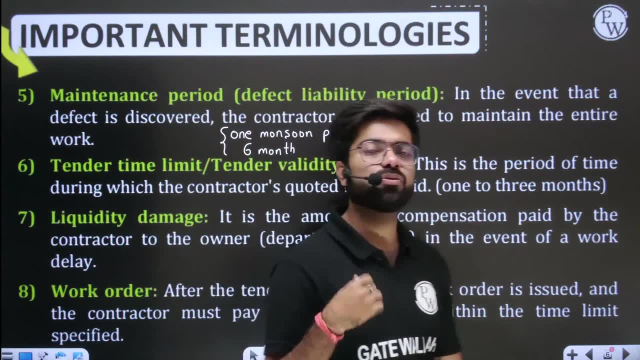 That is called tender time limit or the validity period of the tender. So to fill the form, generally it is like this: For one to three months, what you have written is true. After that, if you want, you can do changes and so on. 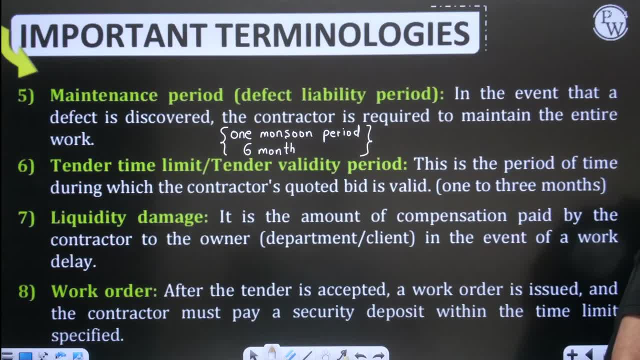 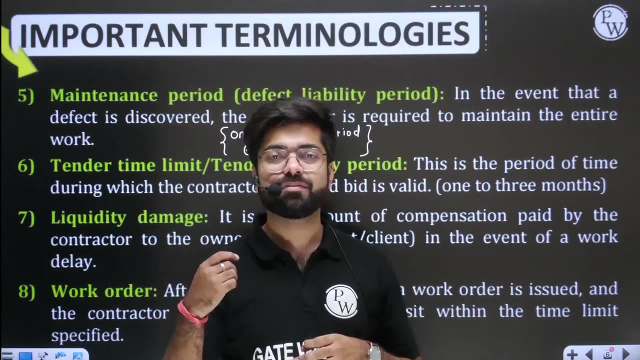 But it doesn't last that long, Okay, Until then the work is done. Hmm, You must be understanding the thing, right? Okay, Come on, the net is here, Hmm, Hmm, Yes, so suppose the contractor is late in the work? 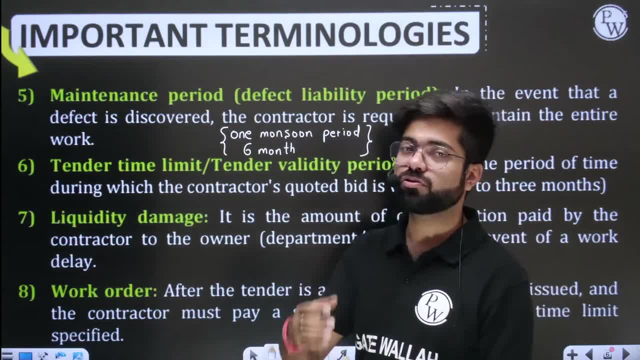 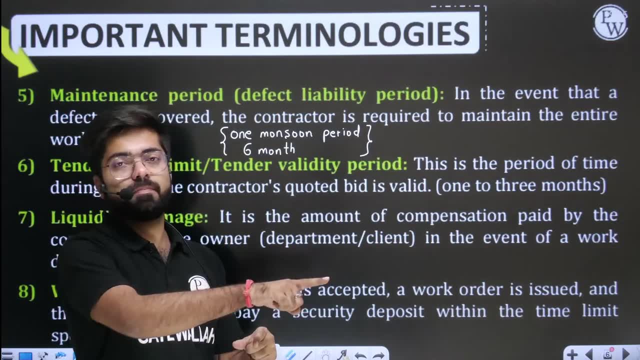 The contractor is late in the work. So whatever department it is, it can apply some fee. it can apply a penalty fee. It is called liquidated damage. So this is a compensation which has to be given to the contractor. The one who is working has to give it. 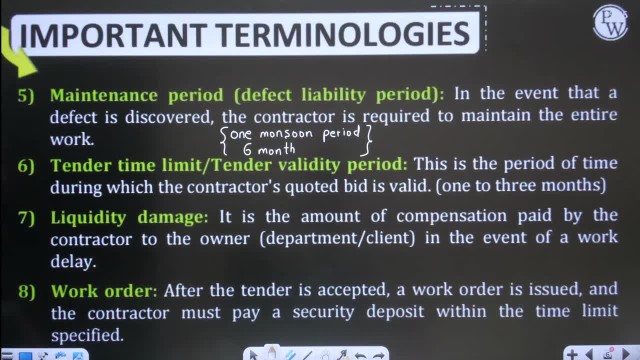 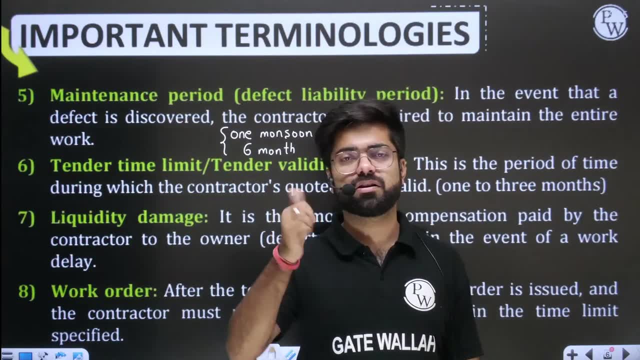 If he is late he will have to give it. Okay, Like yesterday, we read the indirect cost. Do you remember Yesterday we read the indirect cost. We read yesterday. Yes, it was increased yesterday. Indirect Cost, That is it. 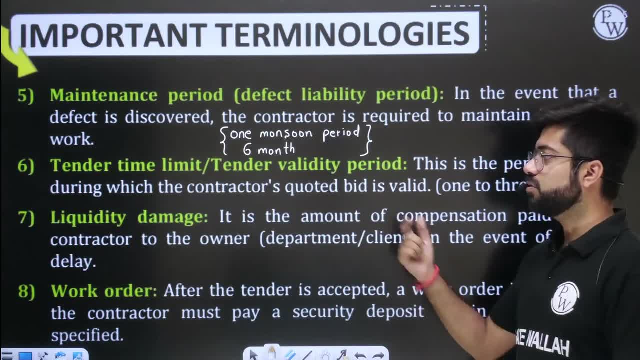 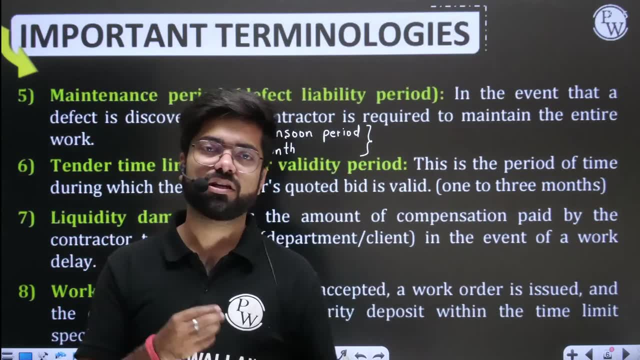 In Indirect Cost Penalties are applied. so the Liquidity Damage will come in this. only Then there is Work Order. Work Order is generally done by these people only Work Order is generally done by these people. only Executive Engineers do it. 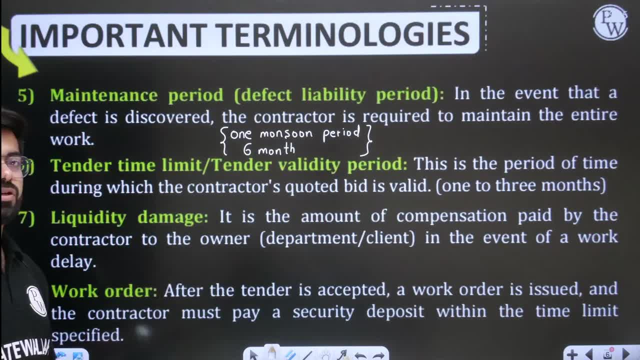 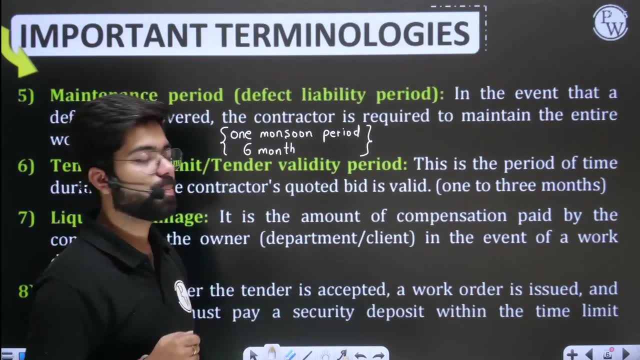 When your tender will be accepted, work will be done with agreement. then Work Order is issued. Work Order is the order to do work. Work Order. Copy of Work Order is given to one JEE, one AEE, one Executive Engineer and one Contractor. 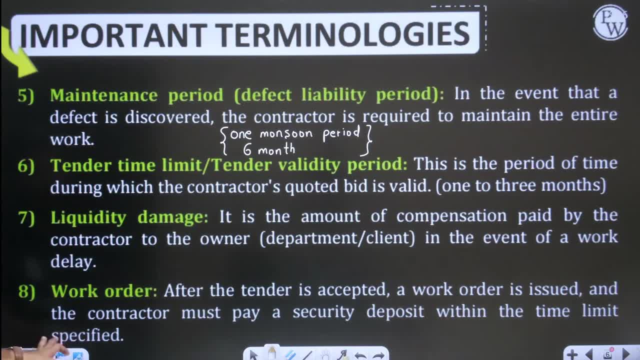 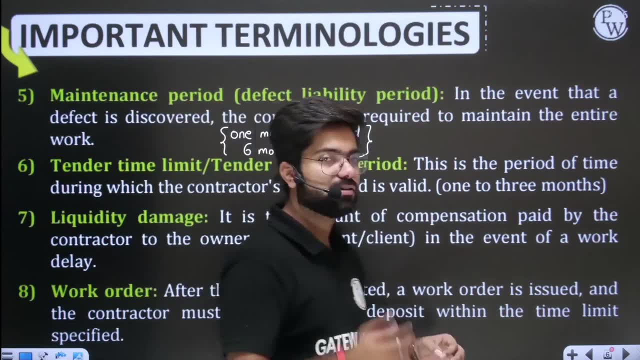 In this way, four people will have one copy. It will be issued and the Contractor will be given a security deposit and work will start. Work Order is a very important document. You will understand everything when you do the work. Then there is Corrigandum. 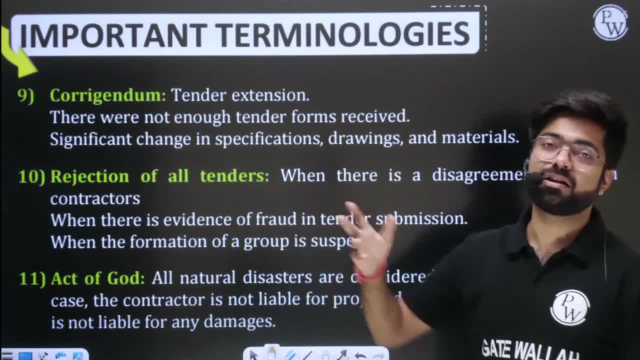 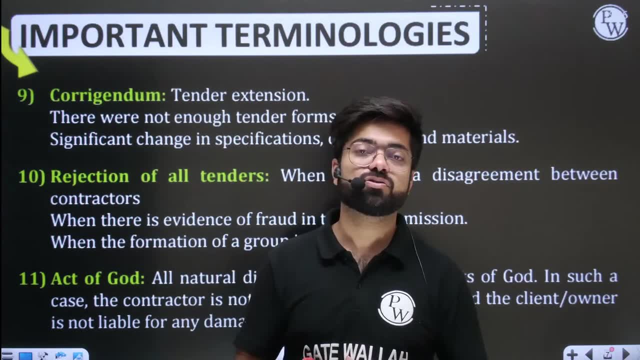 Corrigandum is to extend the tender. When is tender extension? For example, We gave Notice Invited Tender. We thought that five people will come and we will compare who is good and who is bad. Suppose we did not get sufficient tender. 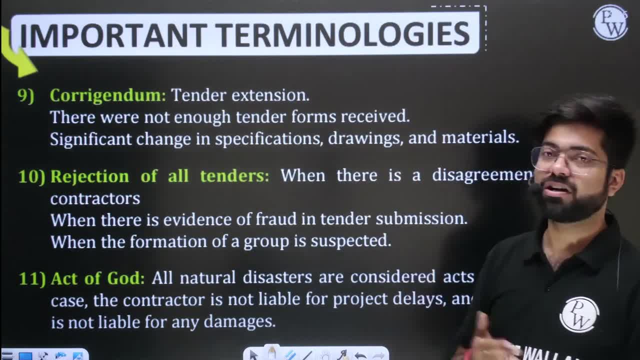 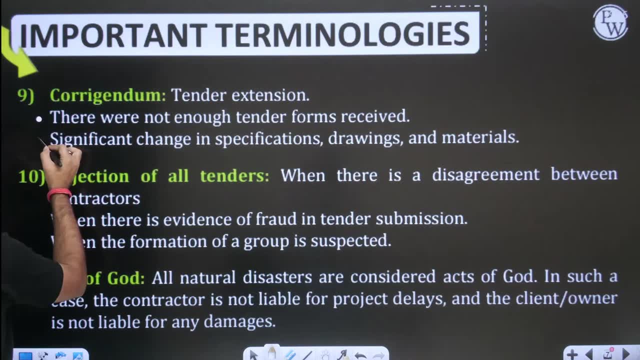 There were not enough tender forms received, So we have to extend the tender. There are some conditions. There are some conditions. Suppose your mind suddenly turned and you said that there are some significant changes. There are changes in the materials and drawings of the work you were thinking of doing. 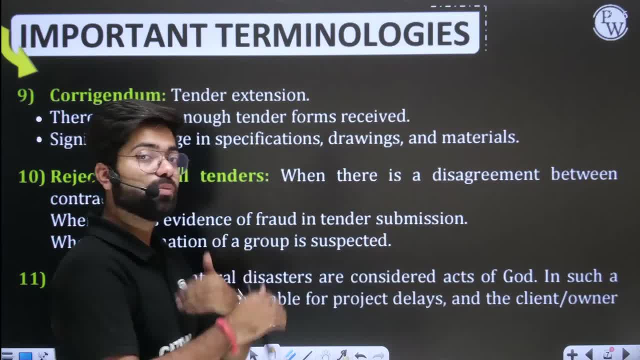 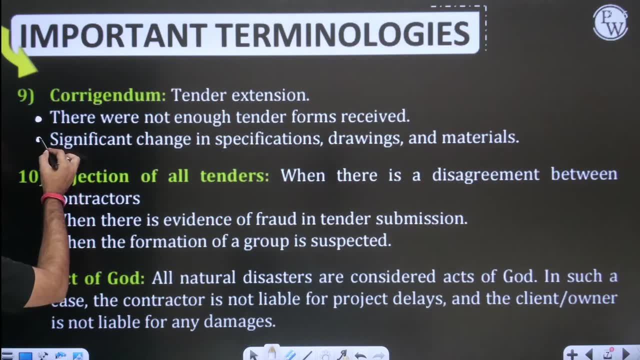 These things have changed completely. Then you will tender again. Okay, See, here It is a tender extension which has been extended. These are some conditions in which we apply Corrigandum. Corrigandum means Simple tender extension. In this case, tender is extended. 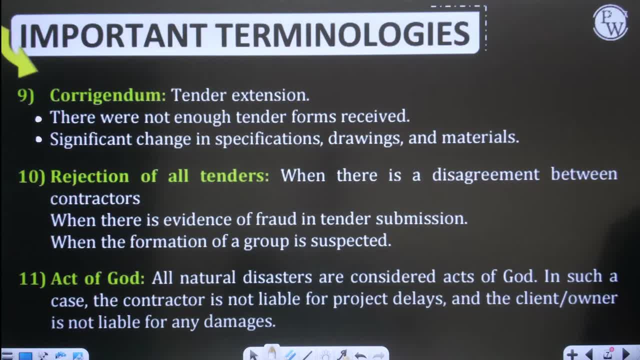 So these conditions keep in mind. There is a question here: How is the rate of increasing materials compensated? That means tender can be cancelled in the middle. No, no, it doesn't happen like this. Look, if there are changes here, then the contractor will tell in between. 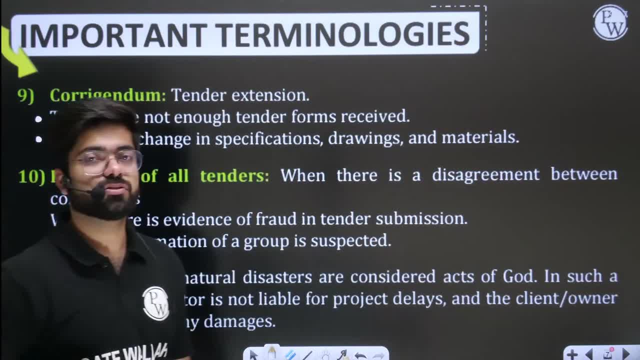 Okay, that thing is heard from time to time. Nothing like this happens In the beginning. whatever rate you have coded, it is not like you have to work in it. Now the rate is increasing, so he revises things and tells: 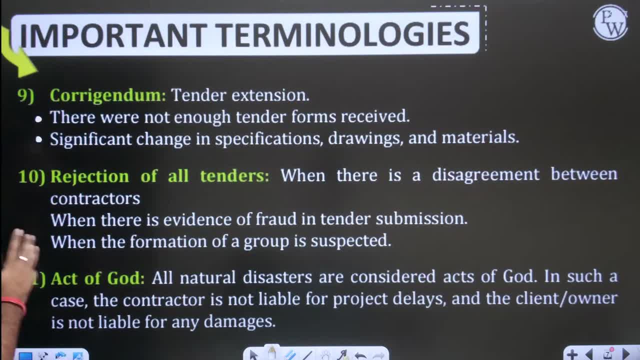 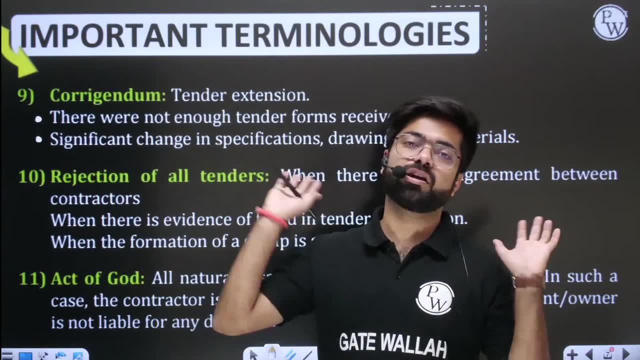 Okay, there are provisions in between. It's not like. this is exactly this, then this is the same. Then the act of God also comes. Act of God means, let's say, if something suddenly happened, you did so much work and everything was broken suddenly. 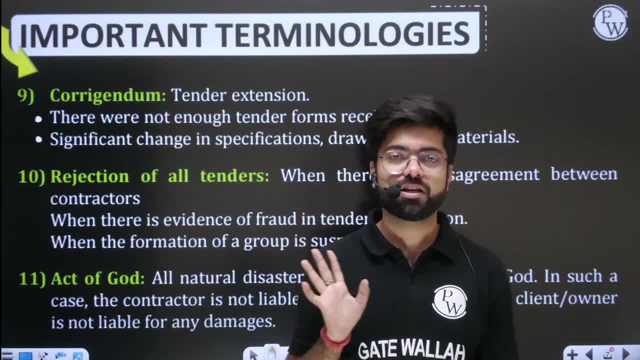 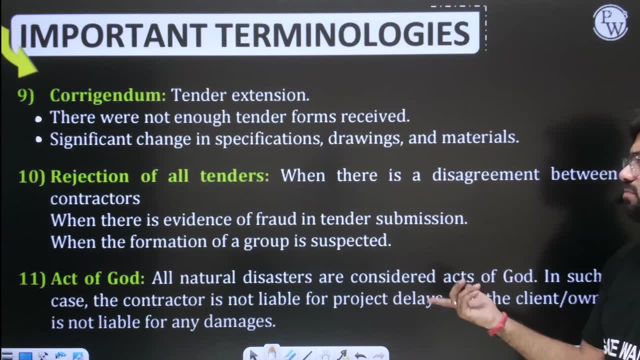 If any disaster or anything came, then there is no mistake in the contractor, Then there is no mistake in the contractor. Understand this: What will happen? in the act of God, All natural disasters are considered as an act of God And there is no responsibility of the contractor in it. 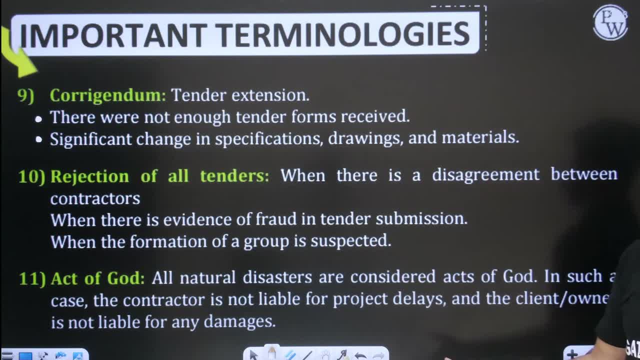 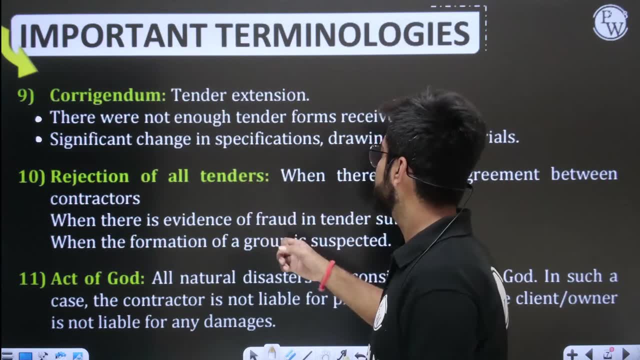 It was known that there was a delay in it or the money was wasted. Okay, if the money is wasted, then there is no responsibility for that damage. Okay, the contractor is doing his job. Okay, then there is rejection of all tenders. 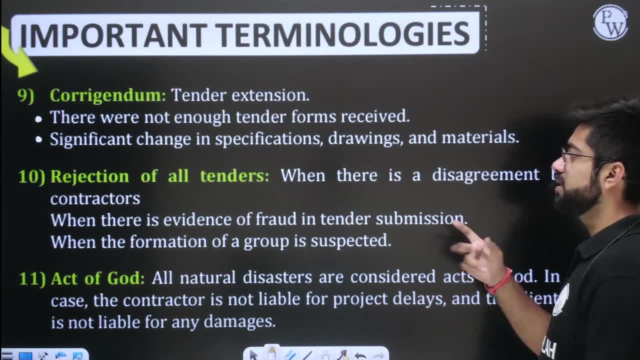 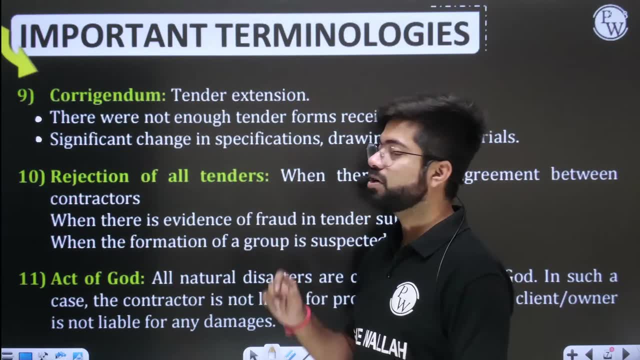 When there is a disagreement between contractors, Okay. rejection. When does it happen? Like a lot of forms have been filled. There are three conditions. Sometimes there is a fight, Okay. Or there is a fraud. You know, everyone is very fast. 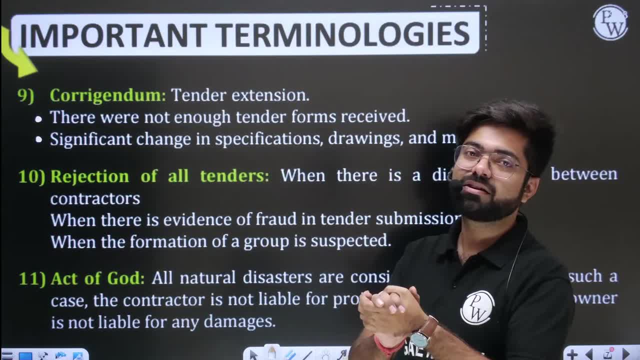 What the contractors do. Two or three people will set it together That we are putting this much. we are putting this much And the one who gets it among the three of us. we will share it with each other and eat it, Right. 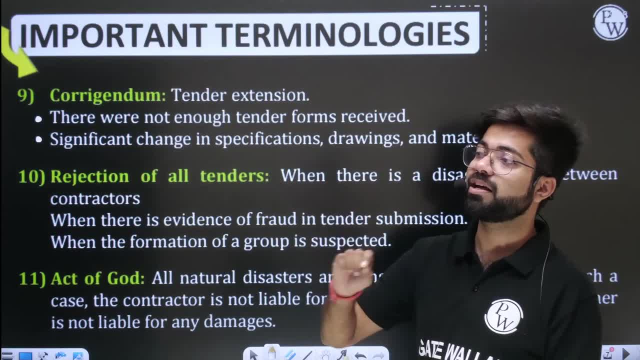 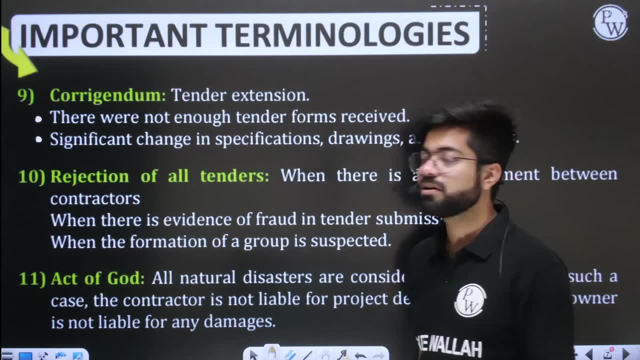 So a group becomes a group inside. Understand Means: we are going to form a form. Now there is no competition in this Fair If there is cheating. So sometimes a group is formed Or some fraud is caught. Okay, Or let's assume that the agreement could not be made between the client and the contractor. 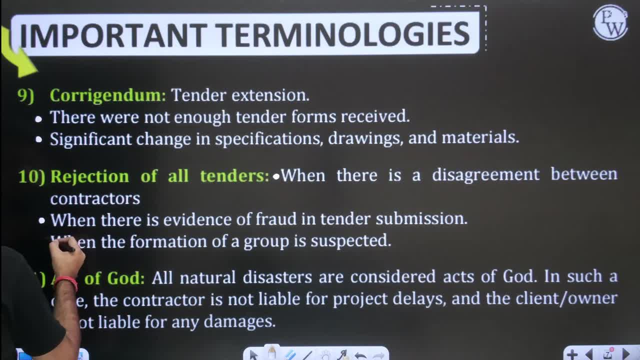 Then all the tenders were rejected here. Or let's assume there is only one form. Only one person came to work, Then what Fun? Then there is competition. At least we will do it again, Right? So these tenders are rejected in that case. 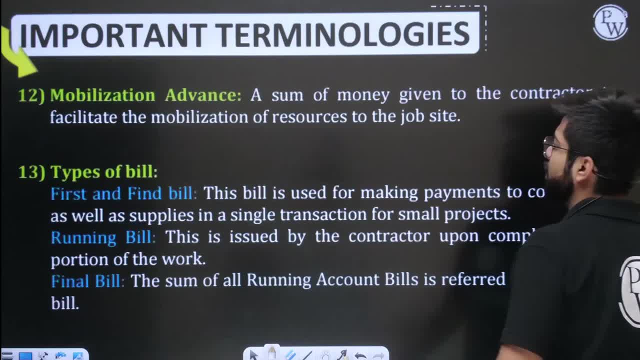 So these are all the definitions that should be known. Okay, All of them have been told to you. Then, mobilization is advanced. What is mobilization advanced? That money is given to the contractor, Brother go. It is like this: 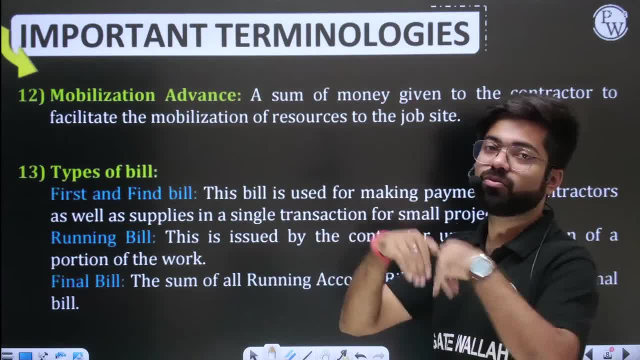 One by one. Take everything and reach the site. Mobilize there The material Manpower. Okay, Take all the resources and reach the job site. This is called mobilization. You will go only if you take money. So that is called mobilization advanced. 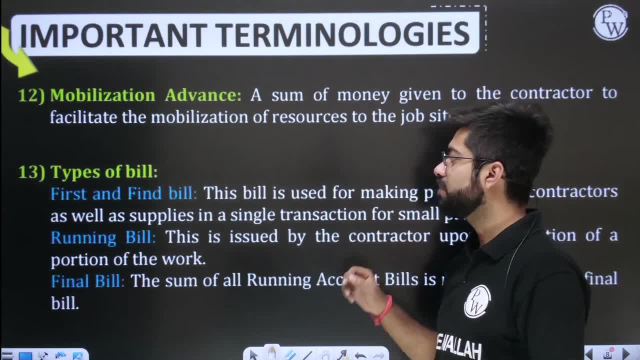 Then types of bill. So one is first and final bill. First and final. Okay, This bill is used for making payments to the contractor, as well as supplies, in a single transaction. Small work has to happen. Take one lakh together Go. 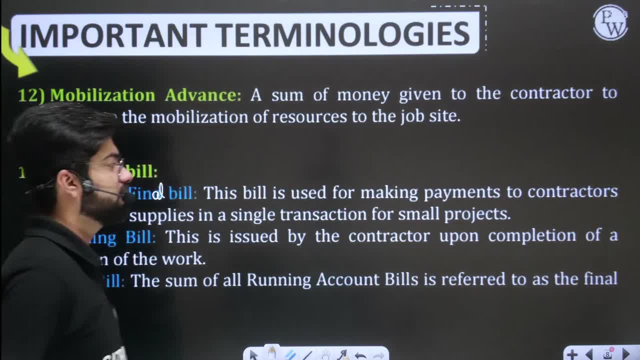 Work and go. This is called first and final bill. Okay, Generally this does not happen. Generally, the work that is done is not done. Generally, the work that is done is not done. The work that is done is done. The work that is done is done. 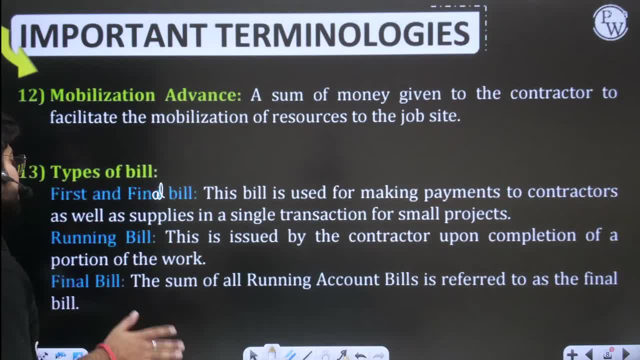 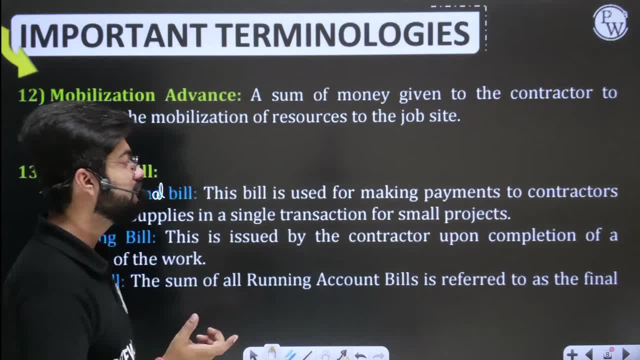 Then the bill is given, Payment is done. It is done in this way Now: as the contractor issues a little work, He has issued, did a portion of the work, He gave the bill And when we sum the running account bill and sum everything, then we call the end bill. 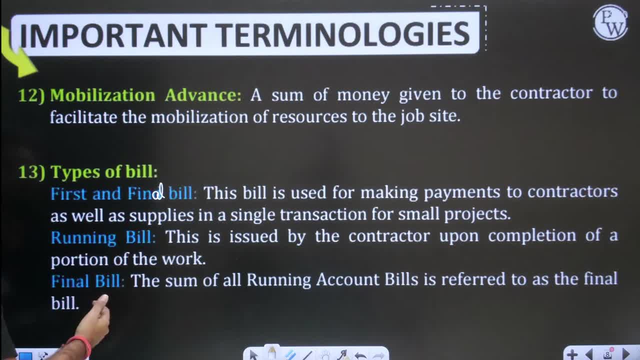 We can club these two together And this is our first and final bill. It is the same, It is given in the end. So first and final is given. So this will be the final one. Then you will go, then we call it the final bill. 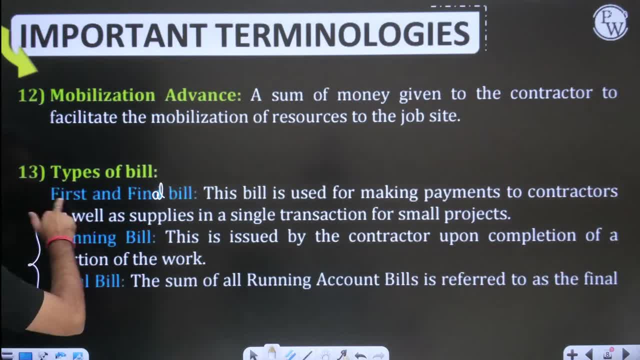 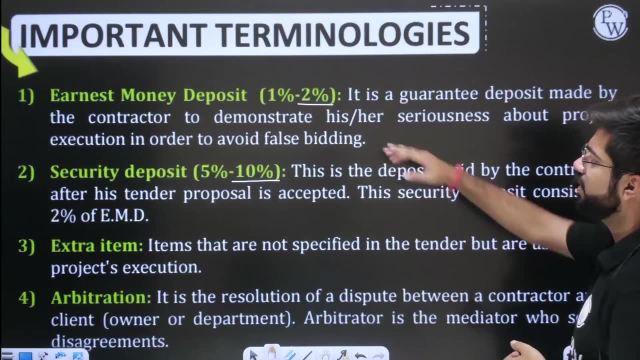 we can club these two in one, and this is our first and final bill. one bill is given in the end, that's it. so all these types of bills, many things, are here. we have told you all the terms. we can ask you the most important questions. these two are very important. 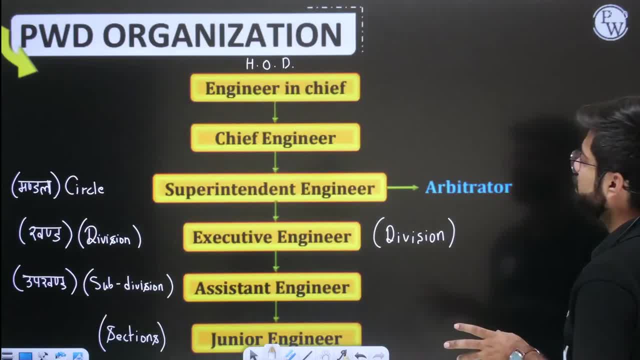 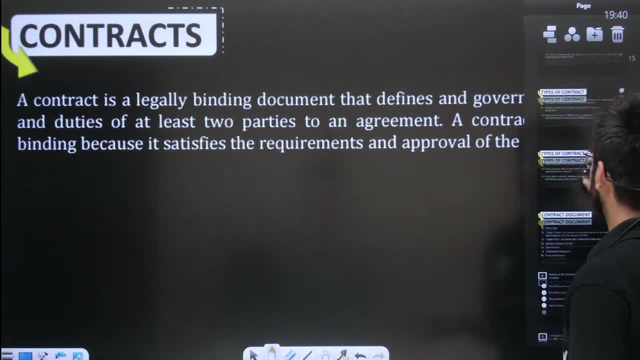 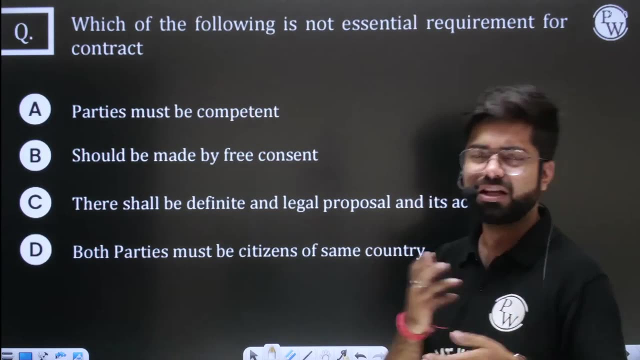 we have understood the types of tender. we have understood all the important terminology. we will understand contract first. we will do some questions. then we will explain you different types of contracts. it is very easy. we will do some questions. question is fun. let's see some questions. which of the following is not essential? 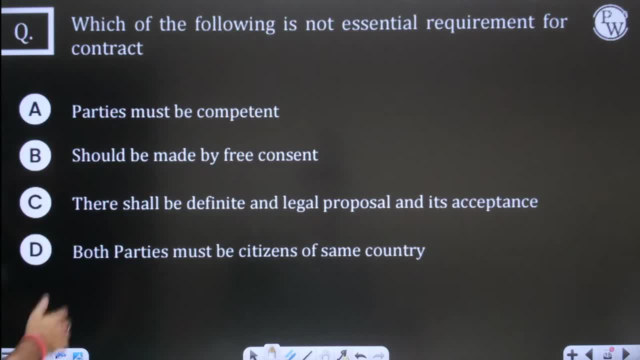 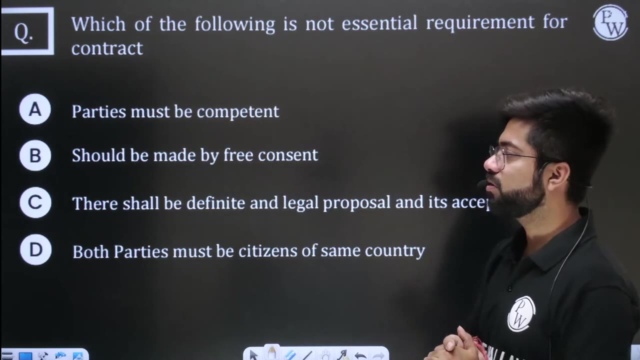 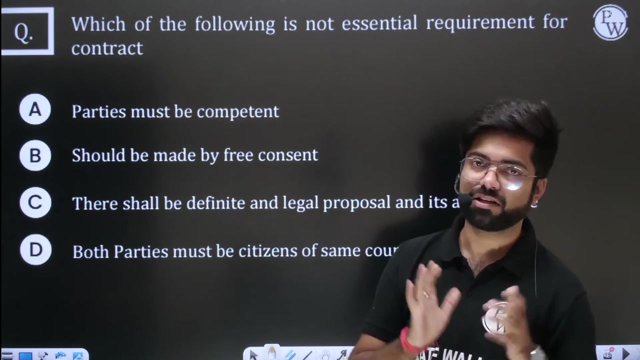 requirement for a contract which is not essential and which is essential. tell me from where to give the question. here it is said: parties must be competent. both parties must be competent. if you become an engineer, you must be competent. now some work is going on. this should not happen. 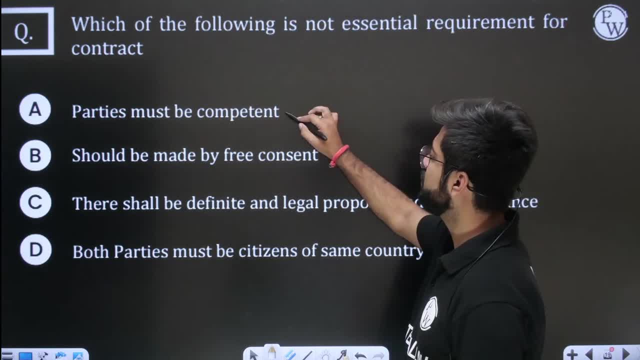 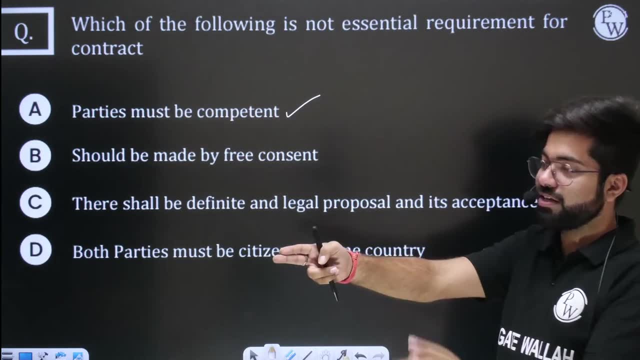 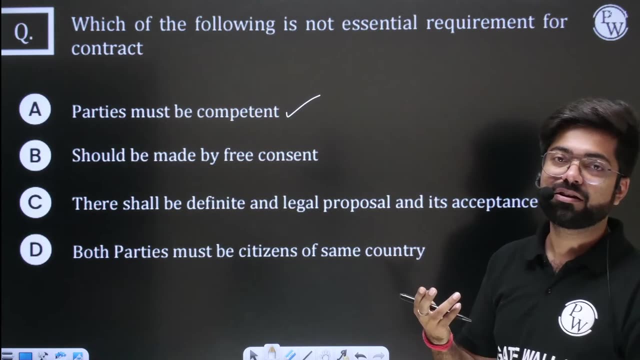 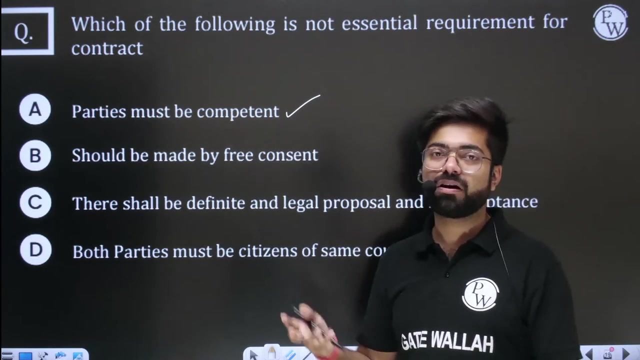 this should happen. this is an essential condition- should be made by free consent. both parties must agree, not like a bullet cross sign up. this should not happen. we are also ready, but it happens. many engineers are shot and some people die. this is a true story. there is so much pressure on engineers. 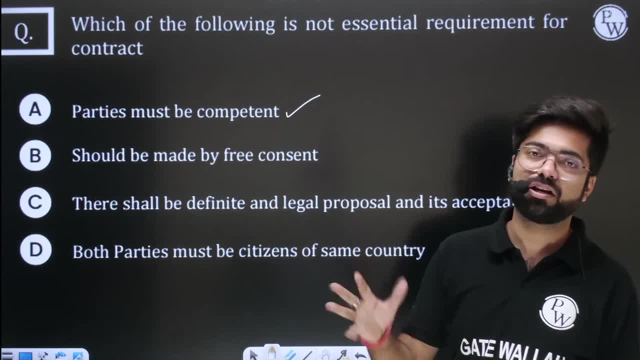 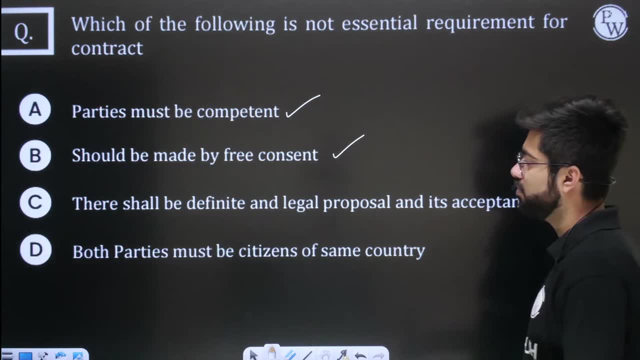 in the state. there is a lot of political pressure. contractors are under so much pressure that contracts are snatched. they don't want to give, but they are snatching. free consent should be there. then only the system is good, then only the taxpayer's money is getting justice. 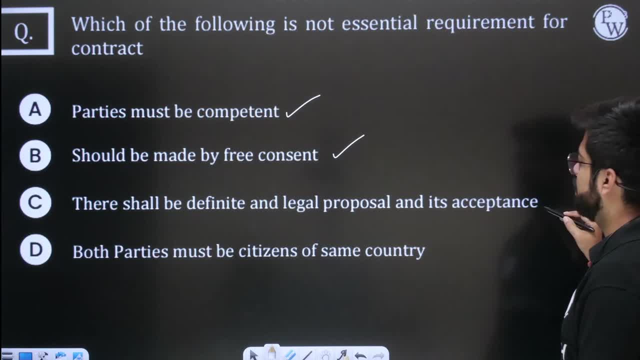 and work will be good. there shall be definite and legal proposal and its acceptance. there shall be definite and legal proposal. both parties must be citizens of same country. this is not important. this is right. this is not important. this is not written anywhere. D option is right, which is not essential. 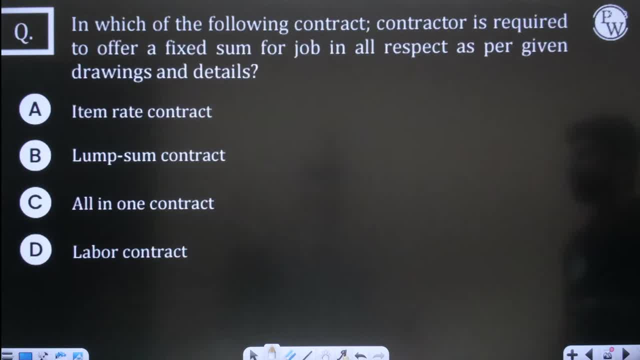 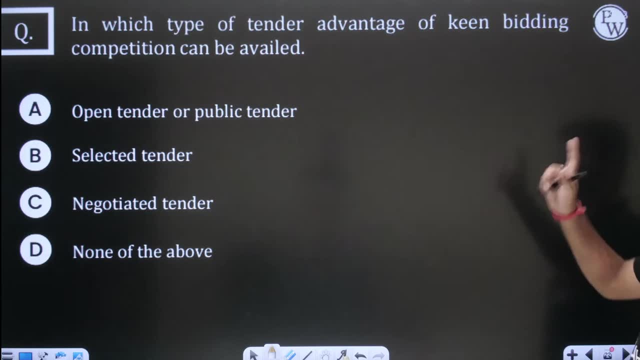 which is not essential. so this is asked. everyone is able to tell D. very good, now you have not told your type of contract, so leave this question, remove this. tell this which type of tender advantage of keen bidding competition can be availed- keen bidding competition can be availed. 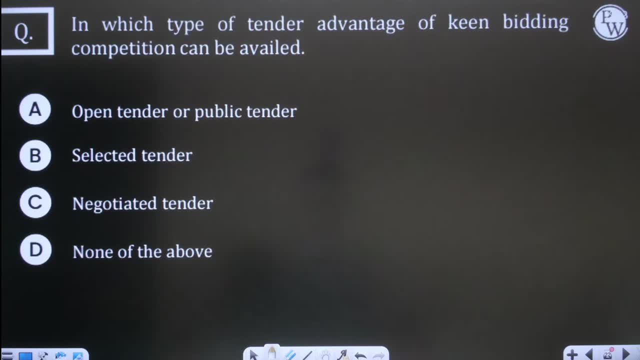 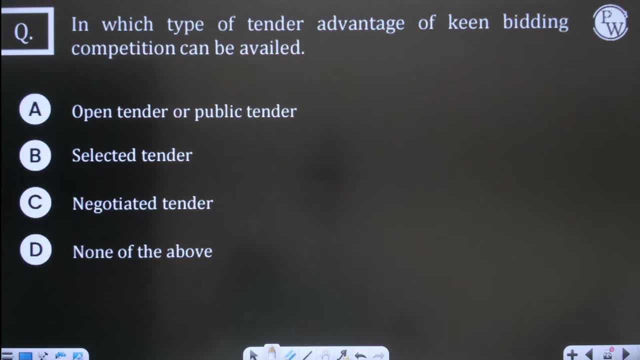 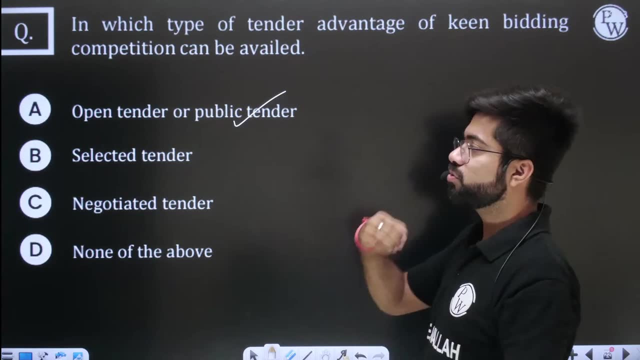 To get the benefit of competition. This will only happen in A. I will tell you all three: If you do public tender, everyone will fill the form. It will be a good competition. Those who want to compete in real. They will have a good competition And the one with the best quality and lowest price will be selected. 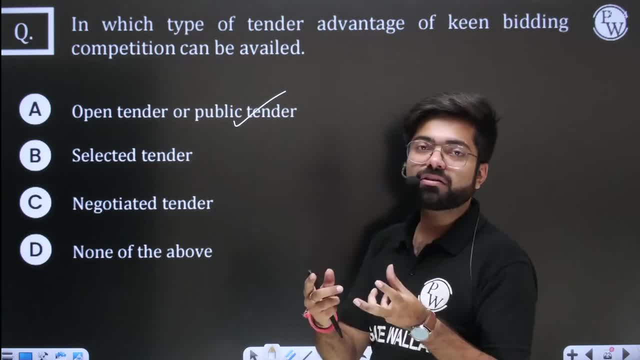 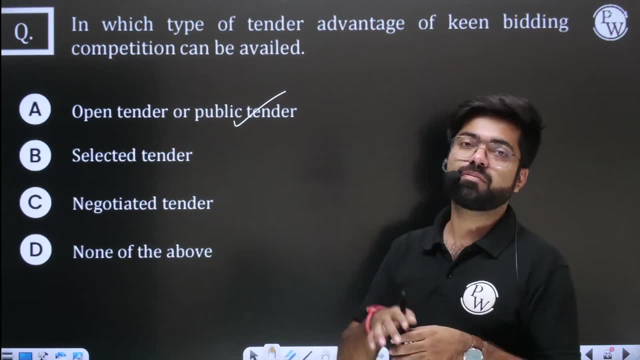 A option is absolutely correct. Only limited people will come out of the selected. Then it will not be a good competition. And what happened in the negotiated tender? In the compulsion There was a person with whom we had to negotiate. He was the lowest But he was not in our range. 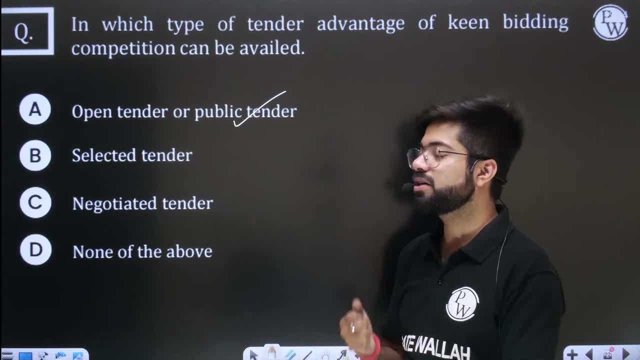 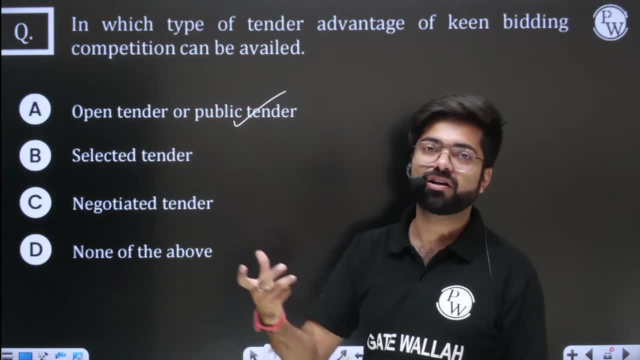 So we talked to him: Brother, agree, Negotiate, Agree, Then it will be a negotiated tender. So in all this, Now that the negotiated tender is selected, You will not get the advantage of the competition, You will get it in public, When everyone is free. It was a very basic and easy question. 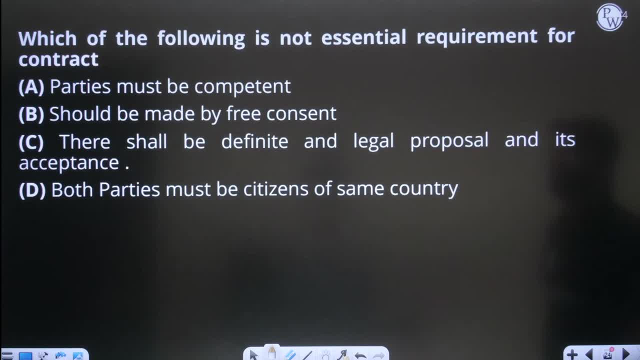 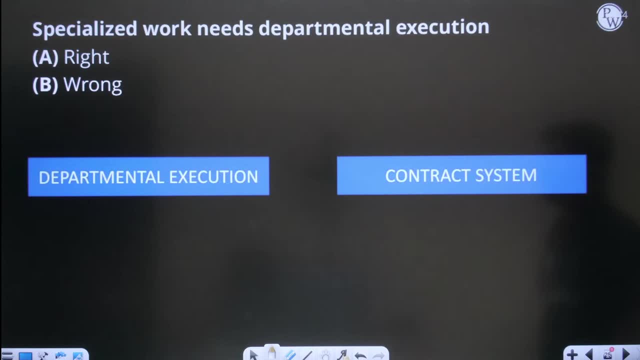 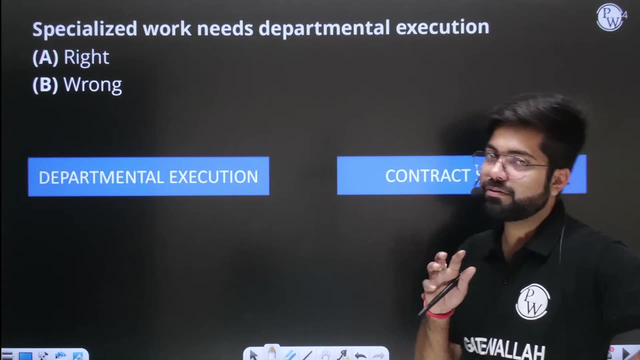 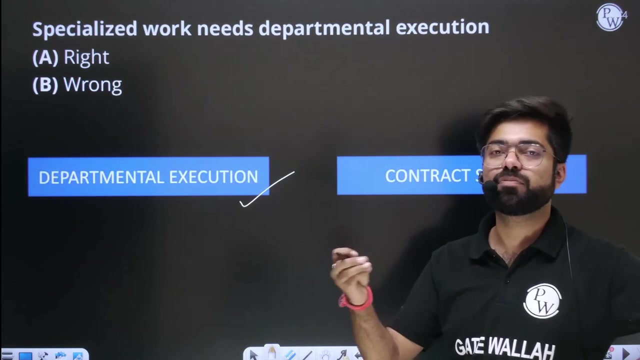 What is this Now? this is the answer: Yes, tell me. Specialized work needs departmental execution. First look to understand the question. You will have to do two things. first, Work: either the department will do By itself PWD or irrigation, If there is any department. 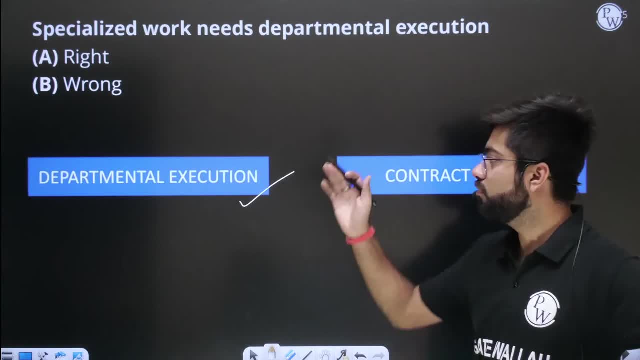 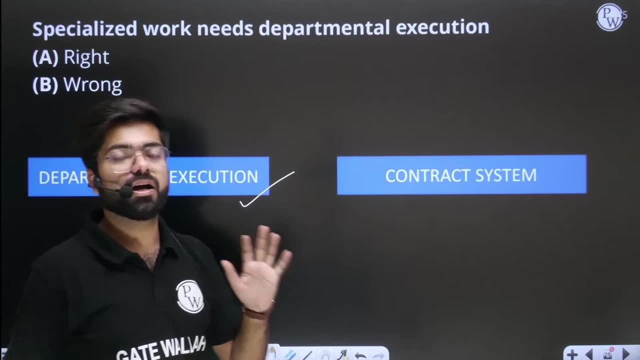 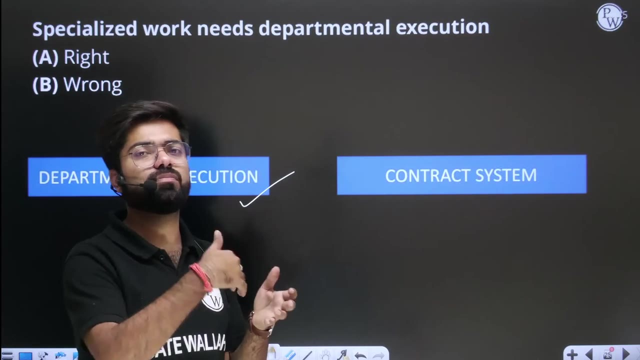 Then he can work by himself. Either he will go to some contractor contract system, third party- if department itself is handling everything inside, like if you have to do some work at home, then you have done it together, third person has to be called from outside. then it is called third party system. 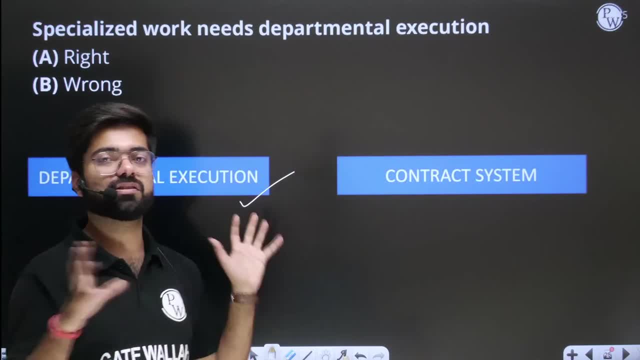 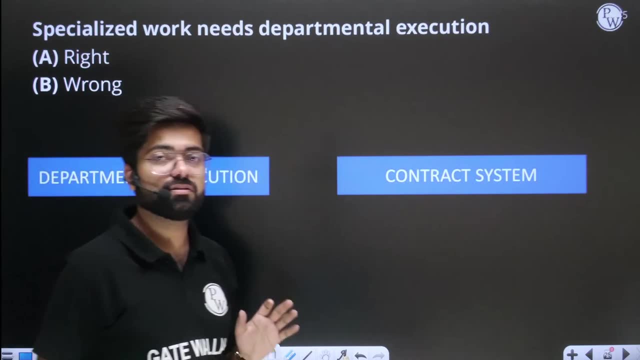 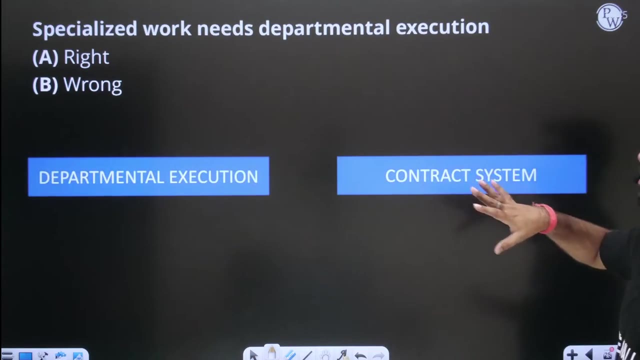 contract system, third person from third company will come and work. well, so there are two systems here. now understand the question. if there is any special work, if there is any specialized work, then will department do it or outside will be required. now tell me right or wrong. now tell me the answer. 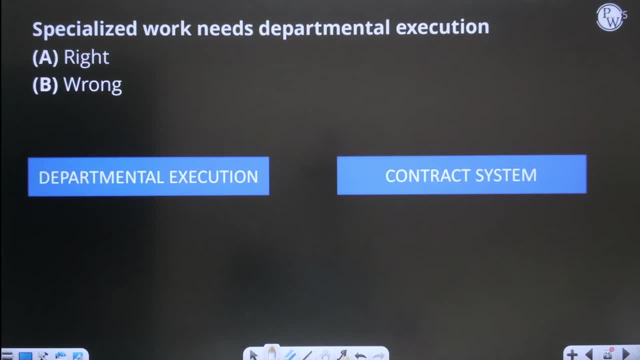 no problem, its pdf is available in app. ok, its pdf is available in app. so most of the people are going with right. its absolutely right. you are telling right no, right will not be the answer. you think there will be any special work department has no idea. department can only do what is already happening. 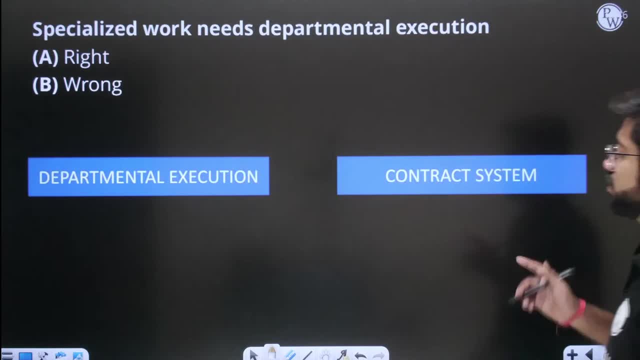 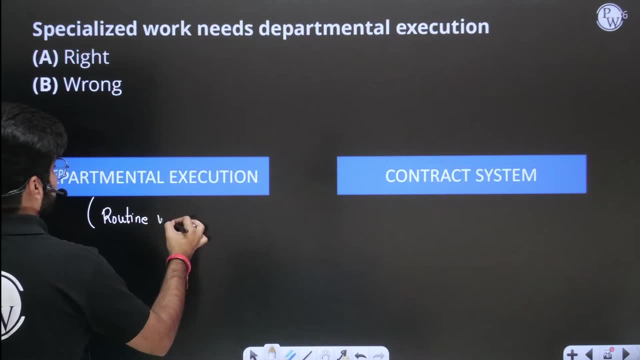 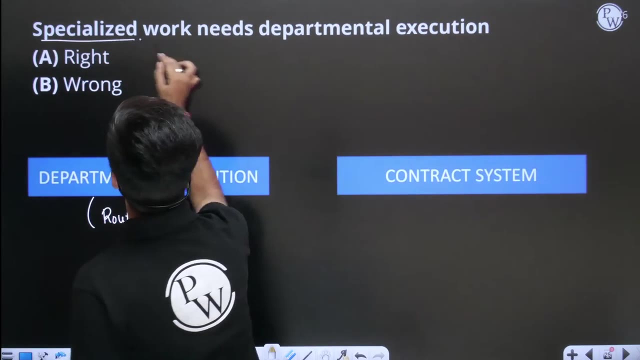 normal routine works. those who are thinking wrong are thinking right. department does routine works here if there is any special work. if there is routine work, then he will handle it alone. but if there is any special work, then obviously he will have to apply contract system in specialized work. 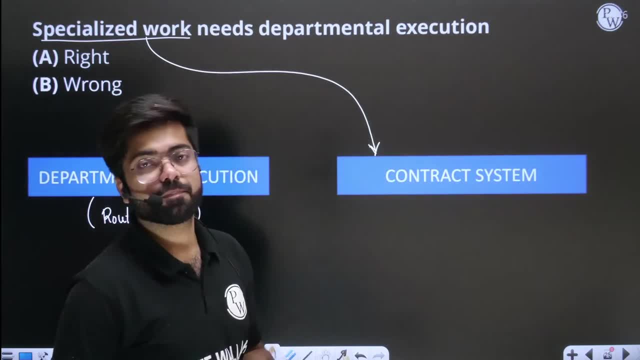 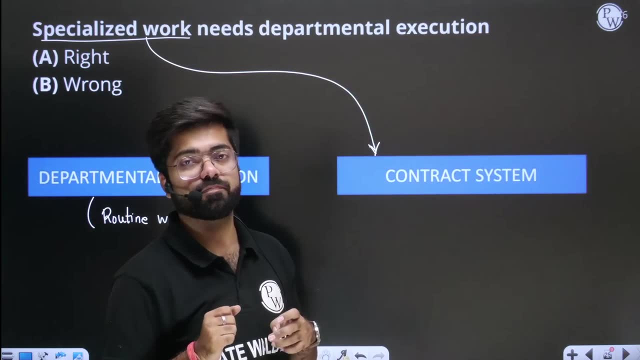 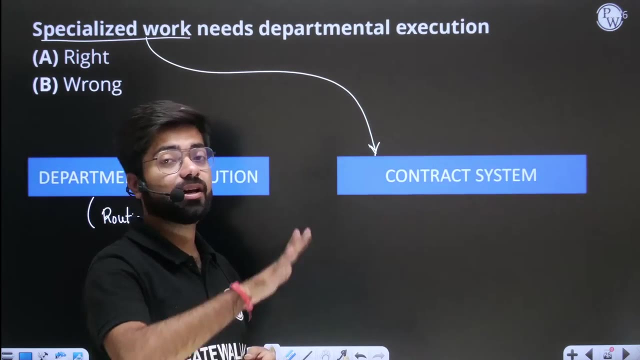 in contract system you have to give to contractor. now, for example, there is a dam. behind the dam there is a leakage in the wall. there are holes, so water comes very fast, so the holes have to be grout. there are holes deep, so there is need too. 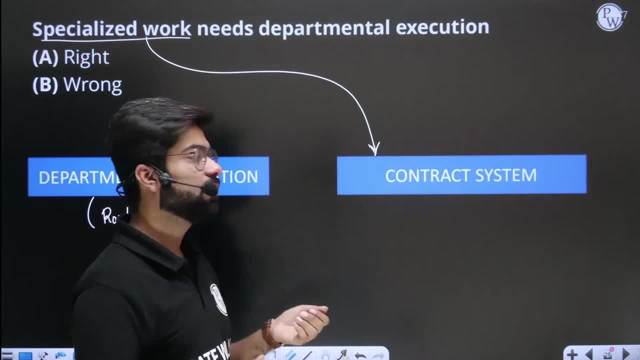 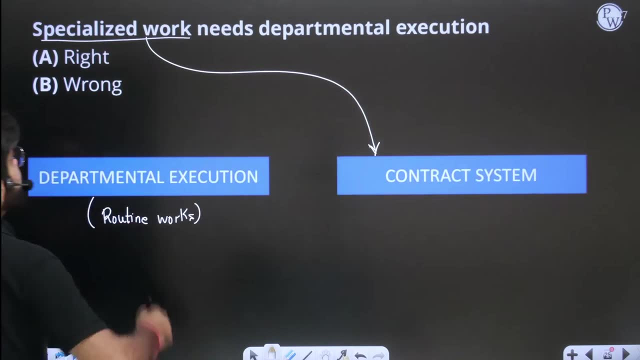 so not every work can be done. there are private companies that can do it. the department people do not work in sub-reservoir, so this is wrong. specialized work need departmental execution. no Specialized work needs contractual system where third party come and show their experience and do the work. 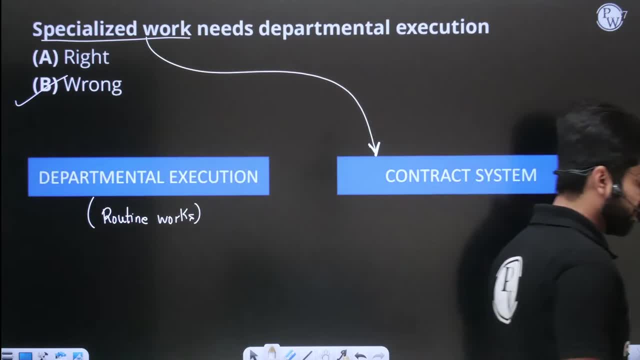 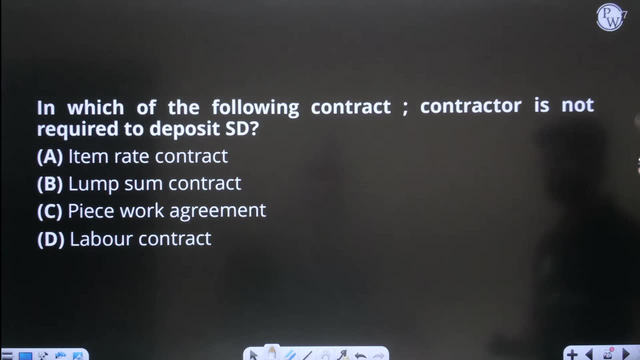 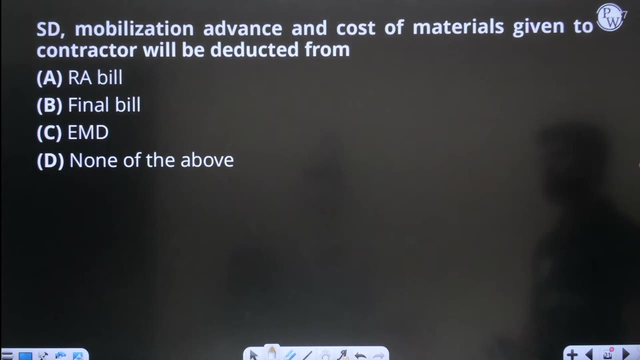 go ahead, lets look at more questions. Okay, wrong is correct, wrong is absolutely correct. then we did not tell you the type of contract. let's do one thing: let's teach the type of contract first. it is necessary to teach the type of contract. tell me this. we will give the answer to this question. some things will be clear here. it says SD means security deposit. SD means security deposit is done. 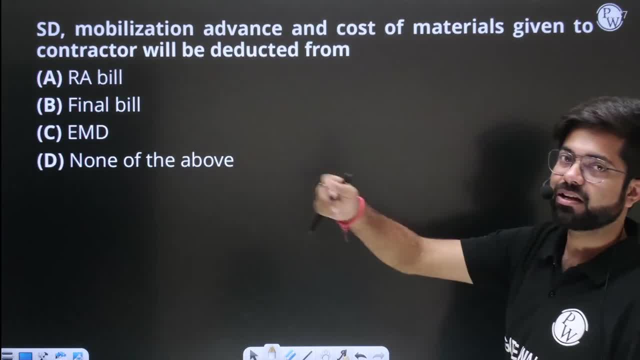 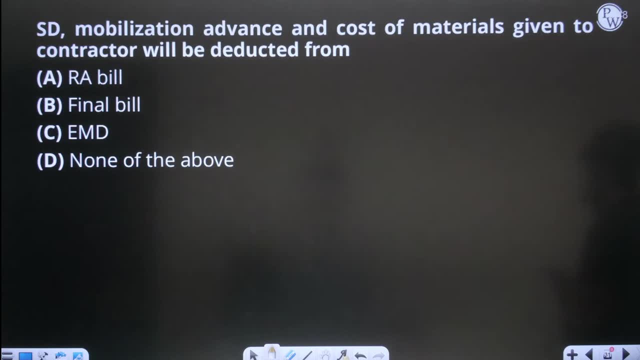 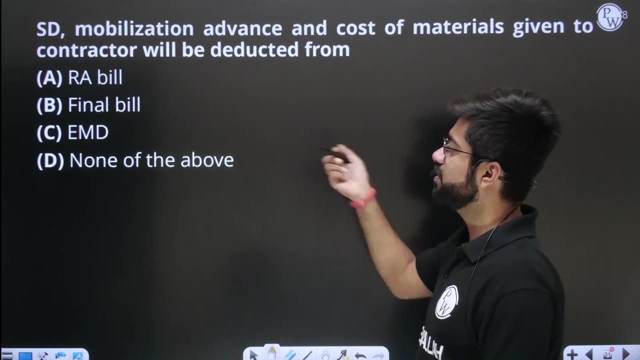 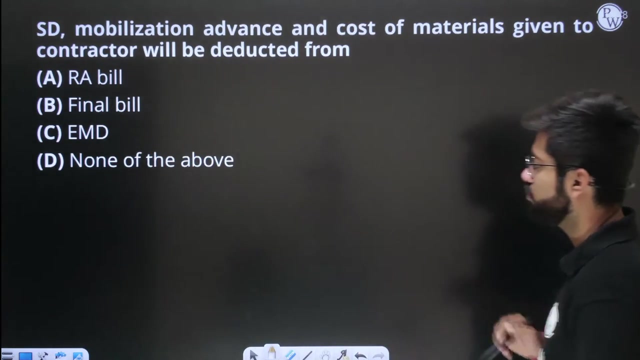 the money of mobilization advance has been given the cost of materials that are given to the contractor from where they are dated. he said that he needs so much money. he will pay the bill. right, he will pay the bill. then where will it be adjusted? from the earning deposit, from the final bill or from the running account bill? it is very important when you do the work, then only you will understand. now you remember it okay, generally see what happens in a big job. 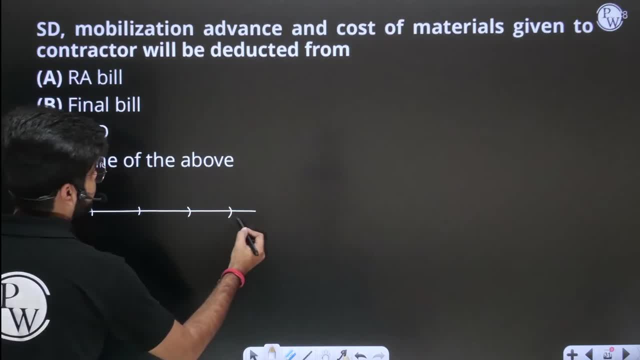 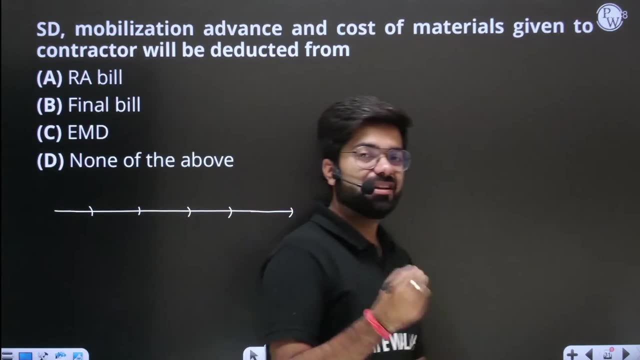 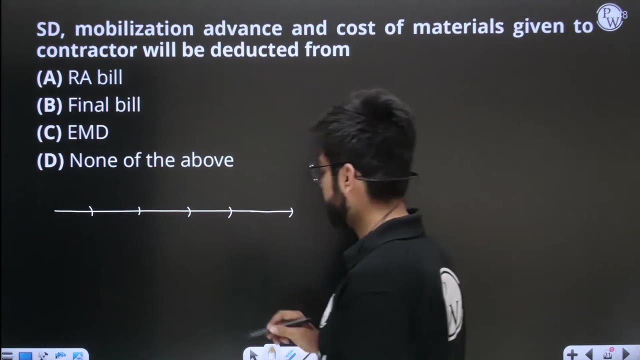 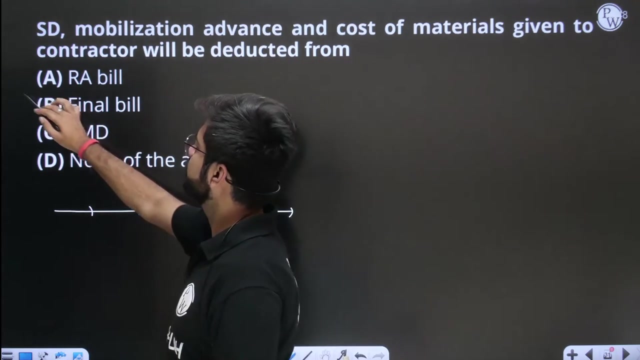 running account bills keep running in small steps. running account bills keep running as the work keeps moving forward. okay, so in these running account bills the money given is adjusted, the money given by the client is adjusted. okay, then its answer will be, as you are telling, most people are going here with C and B. no, it is not like this. running account bill is its answer. okay, RA bill: SD means security deposit. understand all these terms. SD means security deposit. 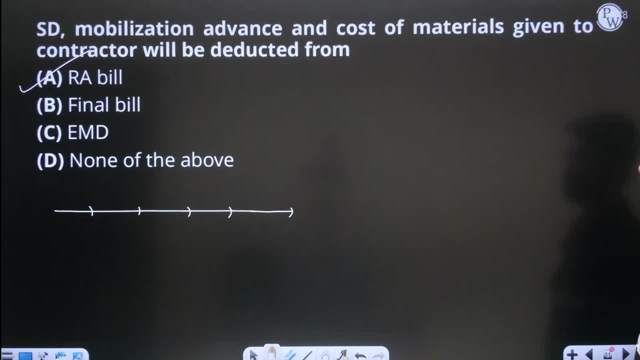 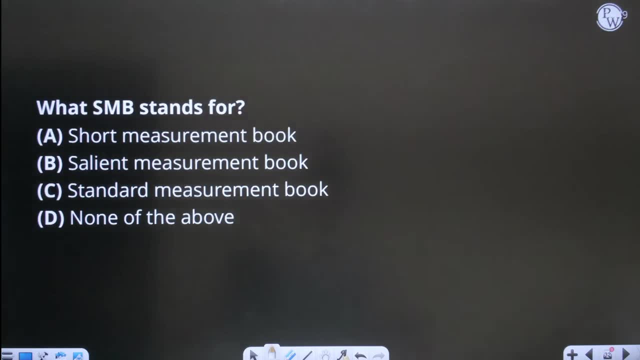 SD means security here, EMD means earning deposit, so it is adjusted in the running account bill. okay, SMB stands for something here. tell me the full form of SMB. no, let it be wrong, try it. but then only things will sit in the mind. we will make the full form of SMB. 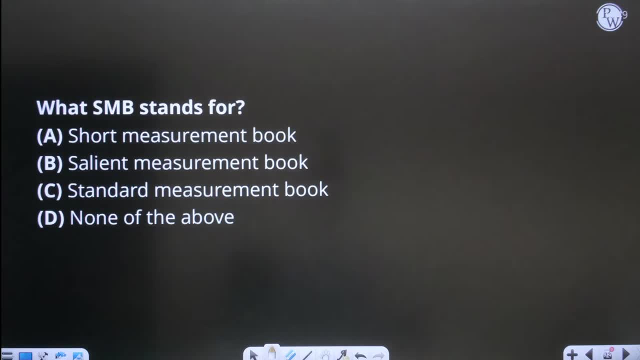 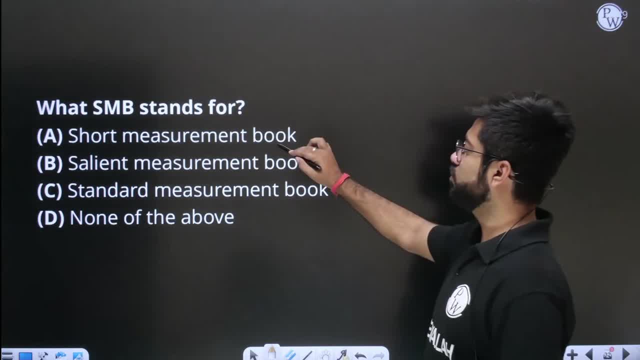 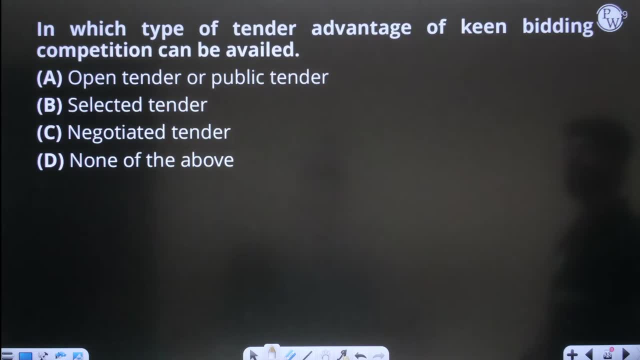 Iran. yes, yes, he said a good job, except he made a move broice the end, yes, yes, but is notebook? yes, okay, we should extremely, if you have any questions, animal without bidding competition is availed. this is your open of public tender. nothing has been repeated. 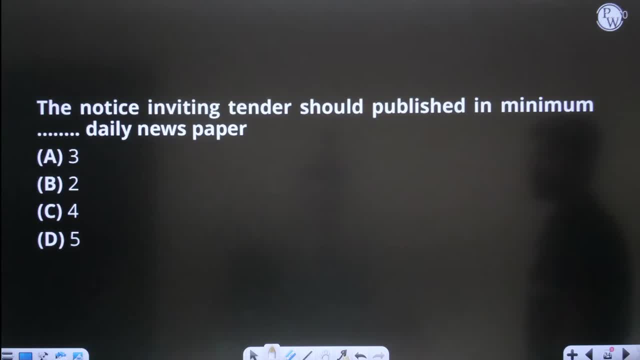 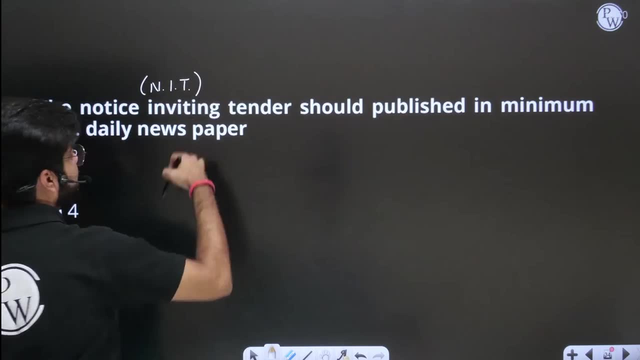 there is no problem. Yes, tell me this. the notice invited tender, which is NIT. it has to be published in at least how many newspapers. generally it is published at the division level. division level means the executive engineer or administrative engineer. executive engineer in Hindi is called. 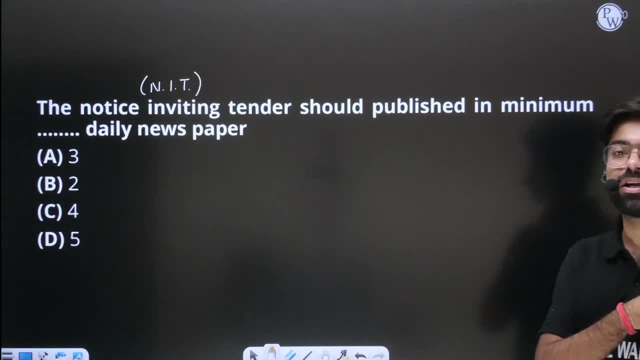 administrative engineer. at least it is published at that level, that at least people reach the news. then at least how many newspapers have to publish it. then at least how many newspapers have to publish it. I am telling you three. two of its correct answers are like this: 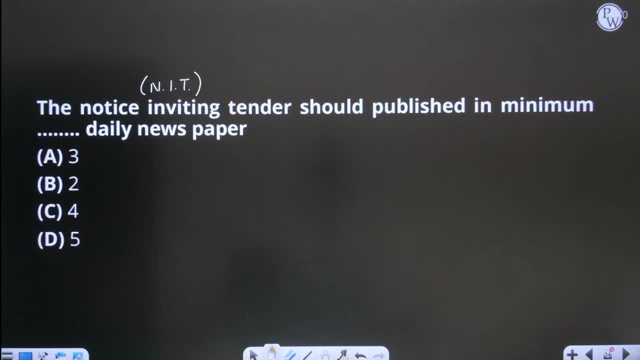 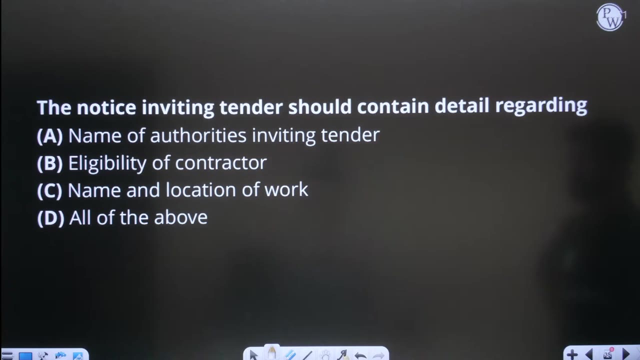 Alright, it is right that the b which is here is called 1, ē2 is the correct answer to this notice invited tender. so I tell you again: the Notice invited tender should contain: contain what suitable details. what should be the name ofon the NIT button? 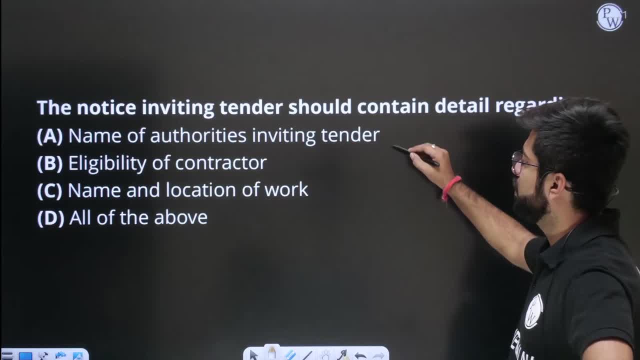 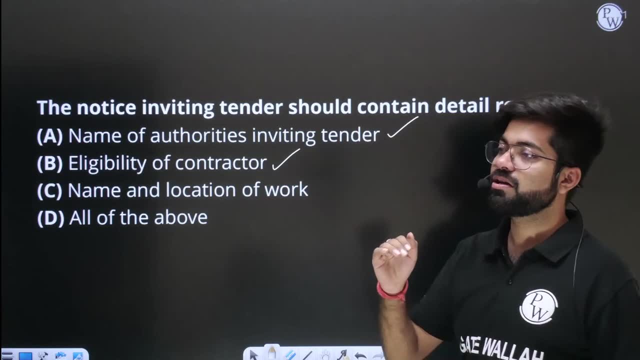 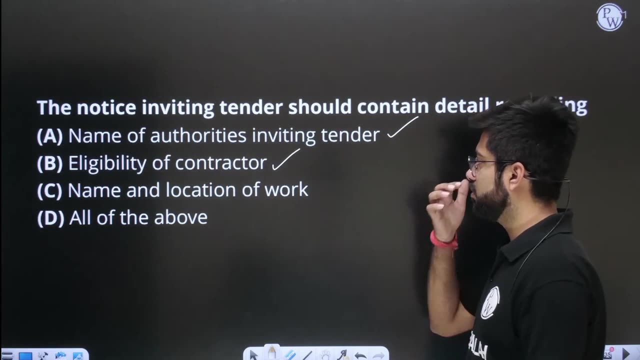 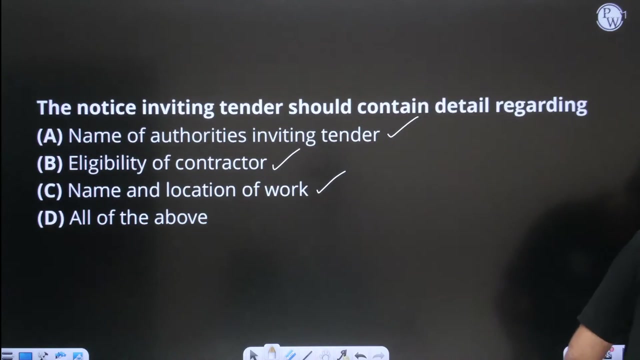 that means the selection of the department. alright, this should happen. if not, what should be the contract then? what to expect from the contractor? What are the expectations from the contractor? what should be the eligibility? you should have done so much work. they have to give their certificate, GST details. they have to show all their things to the contractor. and what are the expectations from the contractor? they are all written in the NIT and where to work and what work to do. all this is told. this is a very basic question D people are telling. D is absolutely correct. 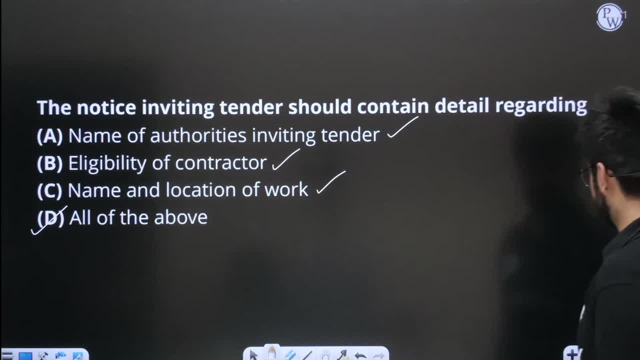 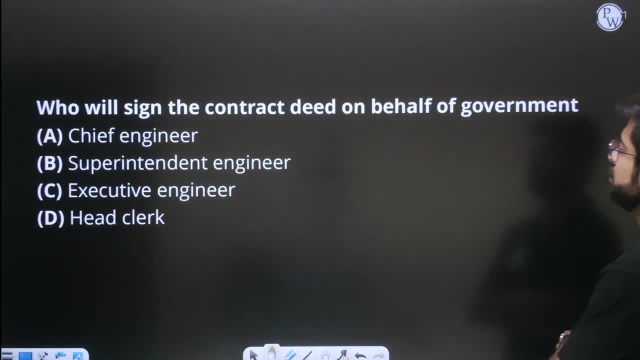 In NIT. all the things will come. obviously, who will sign the contract did on the behalf of the Govt, so you also know that these are all engineers. leave the Settings of E hee alone. you have Ae executive engineers, then Arjan and another engineer. then there is a assistant and then just a blissful engineer and then a big boss. there are two things which should follow in the rule of law. if yes, then there will be two people staying in, other else then they are not scream all people and both are noise in in the required case, then a present female unknownチャンネル is a sculpted likes to play one here. 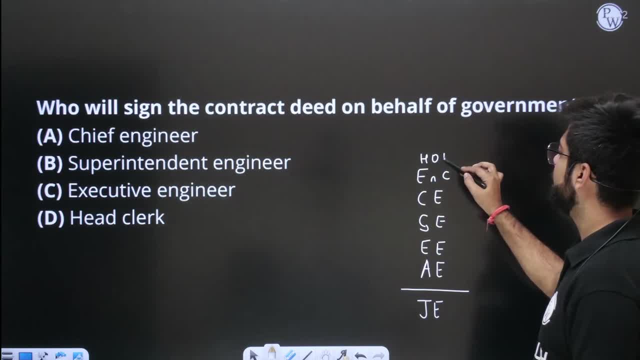 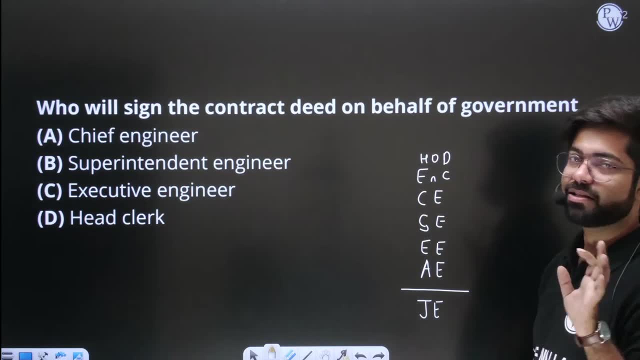 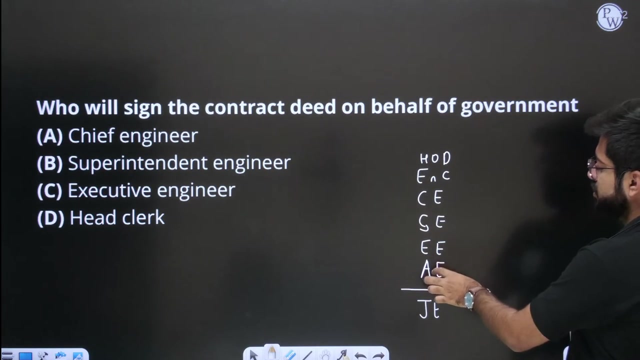 NC engineering chief HOD. these are all the people. look, all these people are made later. everyone starts from here. if you are selected by giving an exam, then the assistant will definitely stick to it, because the executive cannot become a direct because if the experience is good for him, then the problems will increase. if you are not directly reached here, then there will be a problem: work for 4-5 years, then you will reach here. it is a good thing. directly you can reach the highest level here, okay. so here, when you reach here, here comes the officer level. okay, group B, group A. it goes like this: then your 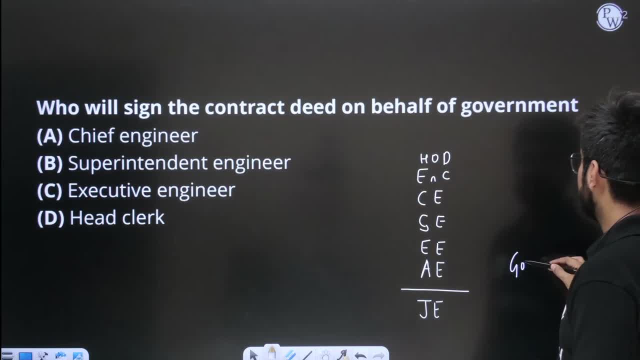 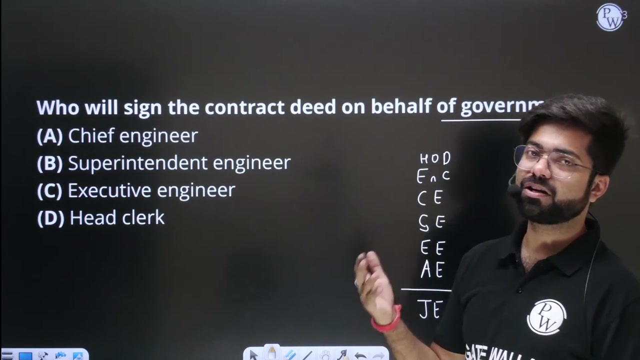 officer and this governor appoints you. okay, the governor has appointed you. whenever your joining will happen, then the governor will sign in it, whatever the state is. if the state is correct, then it means that a big authority will execute you here. so, on the behalf of the government, on the behalf of the government. now you can become anything by being promoted, depending on how soon you have come into service, what is your style of work, how much good work you have done. it depends your report, etc. is there? okay, it is ready, it is seen in it. confidentiality: 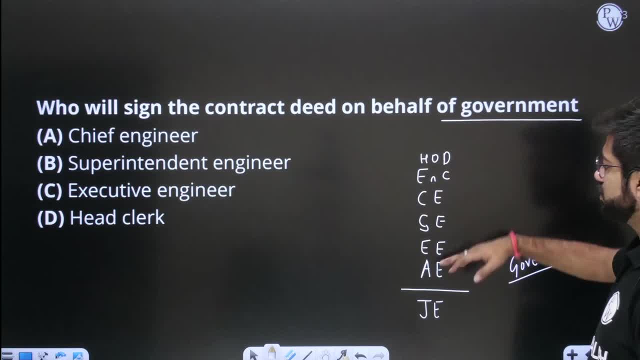 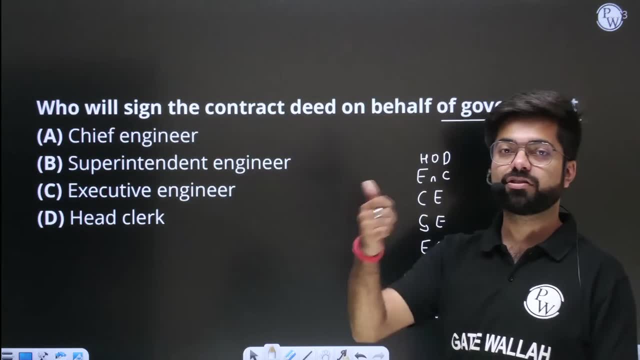 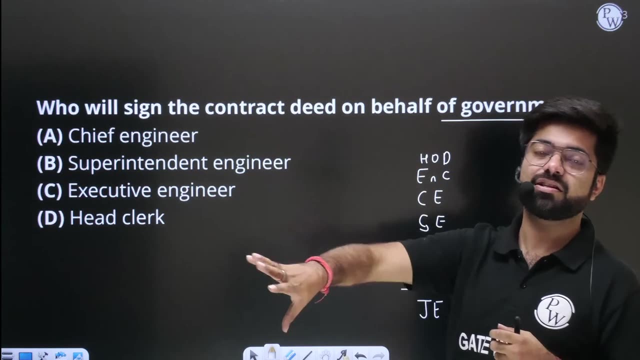 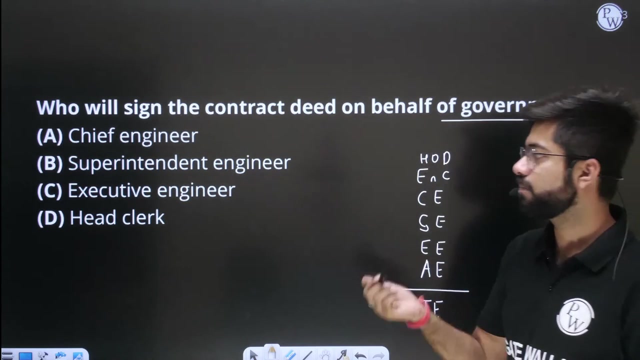 reports are made how your performance will be according to your profession. in short, all these engineers have gone up from here. all these governors have appointed on their behalf. that's why it is called an officer. there are rights on the officer. the officer is called in Hindi. that is, some rights are wasted on him by the government, right? so you have some powers given so, on behalf of the government, who can sign the contract? tell me? it is a very simple answer. if you understand the logic, then you will tell. everyone is telling. if it is not executed, then it is absolutely correct. 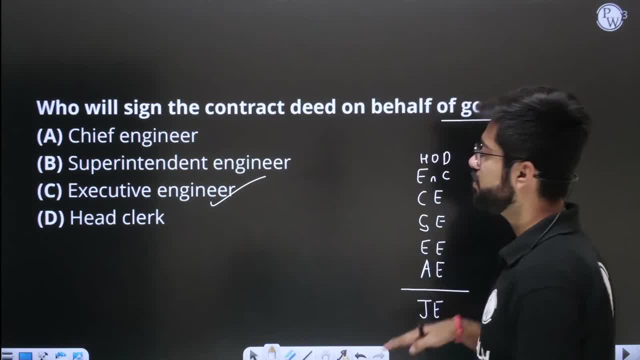 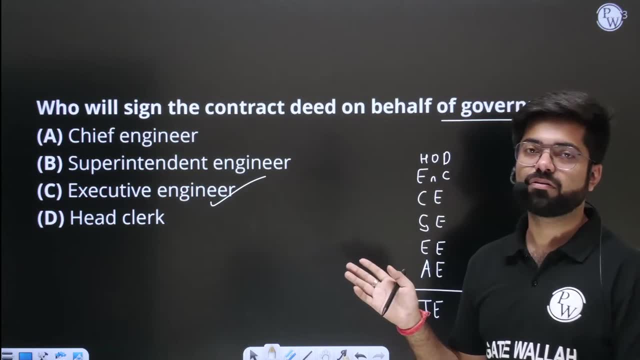 you have thought that is what I means. then, executive or division level, all the work comes to him. you have to sign the contract. if nothing works in that work, then you will be caught. okay, butaria, leave it. it is very common news. when the work of Lakna Riverfront, a lot of big clutter appeared and all the executive engineers involved in that time. 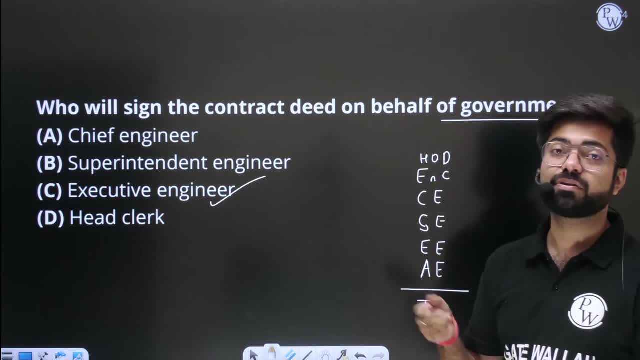 could understand. now a lot of troubles happened. see if your paper is strong enough. if your paper you did, then take a paper without paper last day. what is done on the cover of Zugurkla? you need to be back. even if the support took the sub-level first, what you have done is definitely not correct. 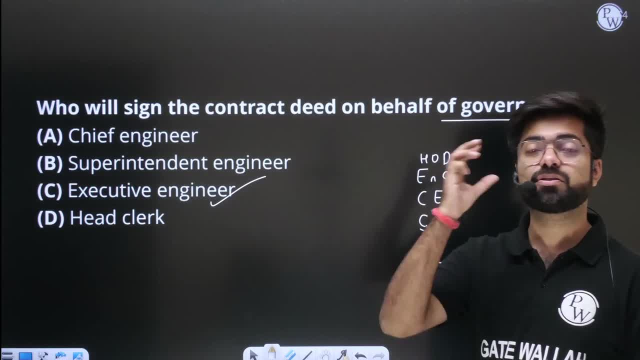 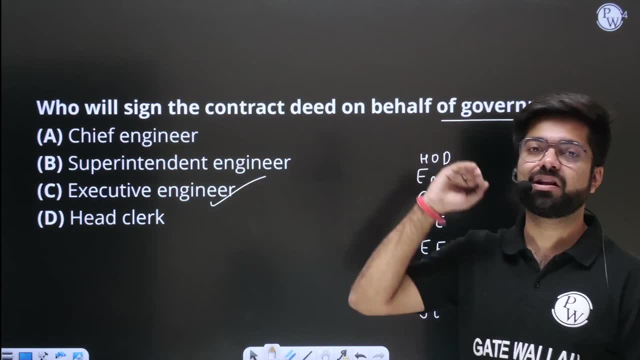 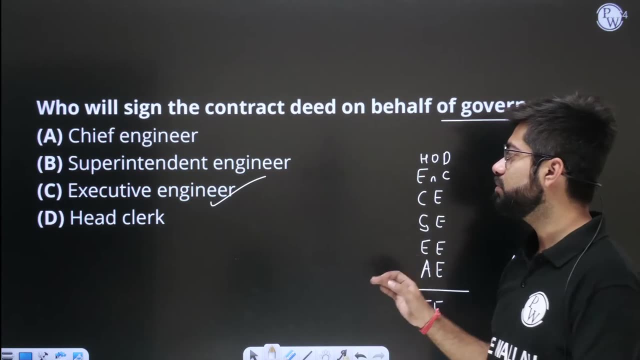 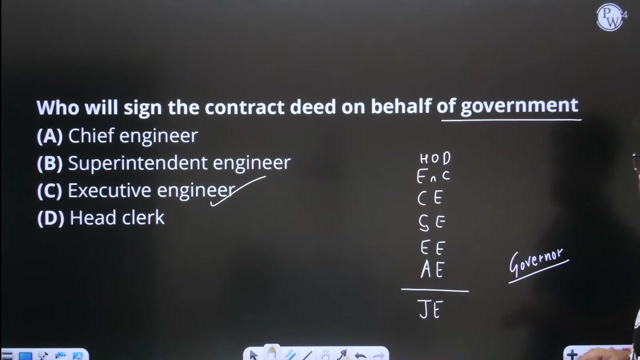 what you do in that, reaching into the industry, make a high system, then everything is taken care of. for a moment to stop interest studies. If you start working without paper, then there will be a problem because later when there is a checking, there is a survey of CBI. if there is a checking at any level, then the paper should be strong that yes, this work has happened like this. if those things are correct in the paper then it will be considered correct, otherwise it will be a problem. then how far will the fake paper be made? 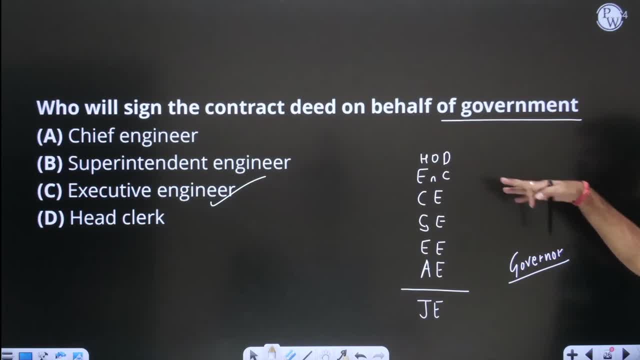 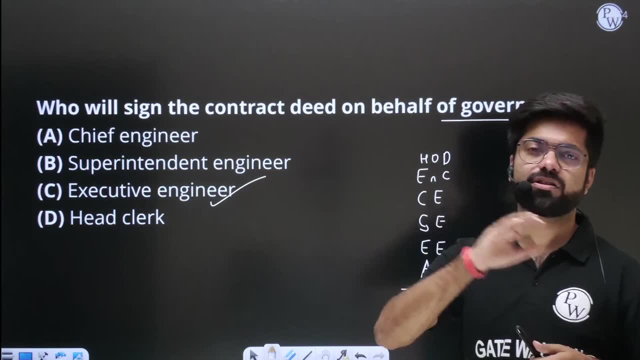 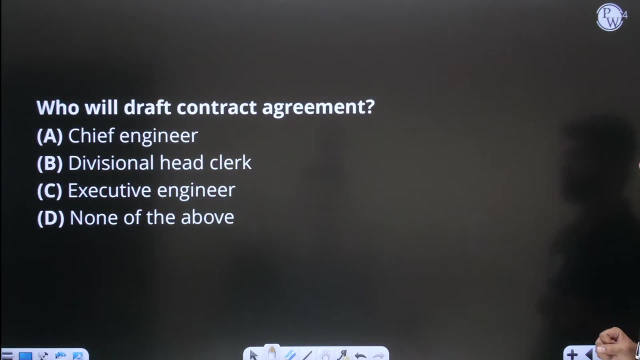 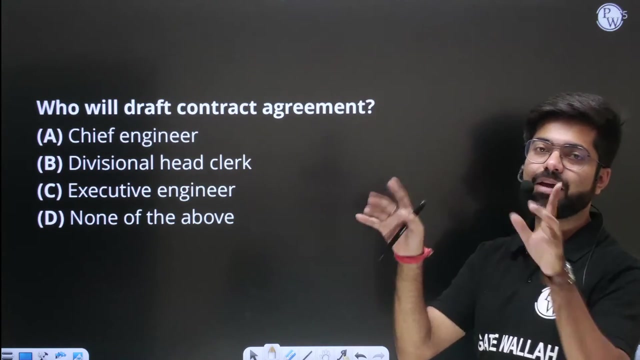 So for now, the government, that is, the power is given by the governor. to whom? To the executive engineer that is. you know all this. there are all the rules. there are very big books. in those books all the rules are written, that who can do what. so how much power does everyone have? there are financial handbooks in which everything is written, so they can read it and put an idea. then who will draft the contract agreement? when there is complete typing in the contract agreement, what should be the terms and conditions, what is the name of the work and where will the work be done? 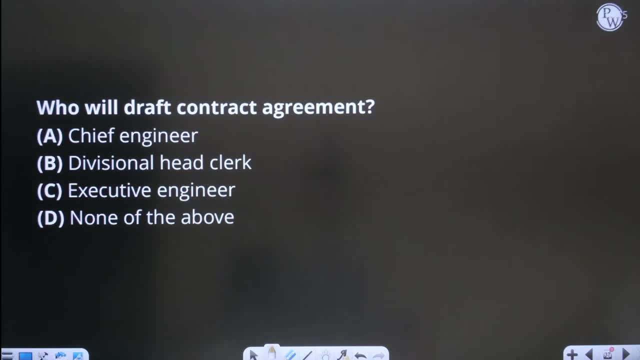 who will do all these things? who will do the draft? tell me who will do all these things. who will do the draft? tell me. Some people are telling D and some are telling B. The answer to this is that the executive engineer will not do the job of drafting, but he will do the job of signing. 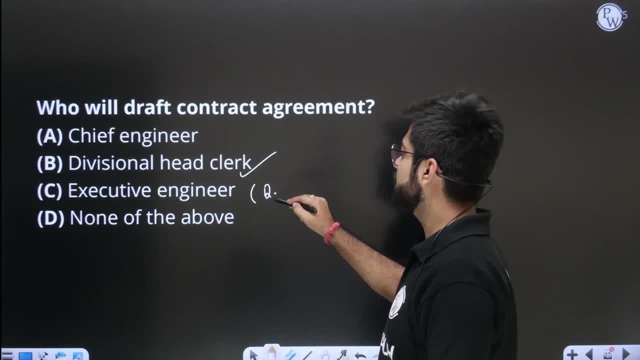 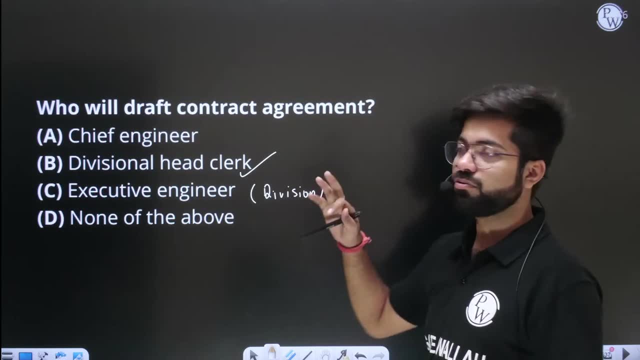 This work is done by the division. Who is the king of the division? Who is the head of the division? The king of the division is the executive engineer, Adhisha Sevinda. The head of the division will do the draft and the original document will be signed by the executive engineer. 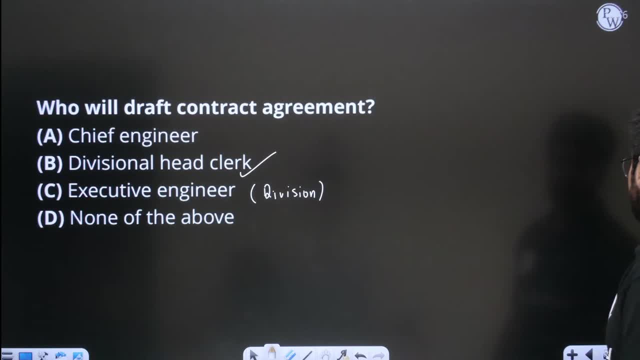 He will keep the original copy with him. Copy is done everywhere. The next question is that the original copy of the contract agreement remains with. Who has the original copy of the contract agreement? Tell me Who has the original copy of the contract agreement. 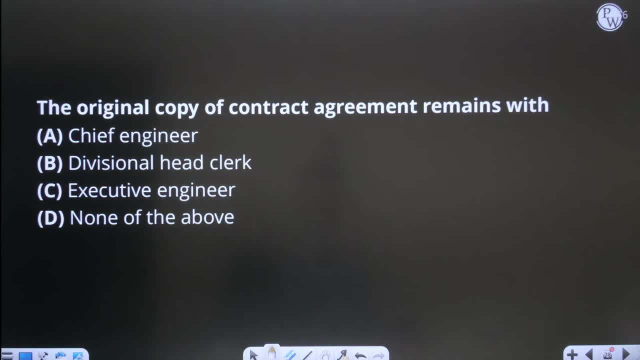 The work of J is to get the actual work done. Get the actual work done. Go to the site every day and see whether all the labor is coming from time to time, whether the drawings are being fulfilled or not. Who are the actual contractors and contractors? 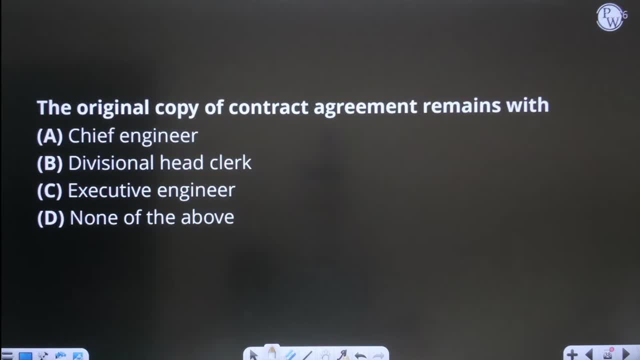 They are J. A is not doing anything. A does not have so much time to get the actual work done. Who is doing all the work in the field? Who is doing the actual work? J And who is supervising A? And A makes a full report and gives it to the executive engineer that today this happened. today that happened. 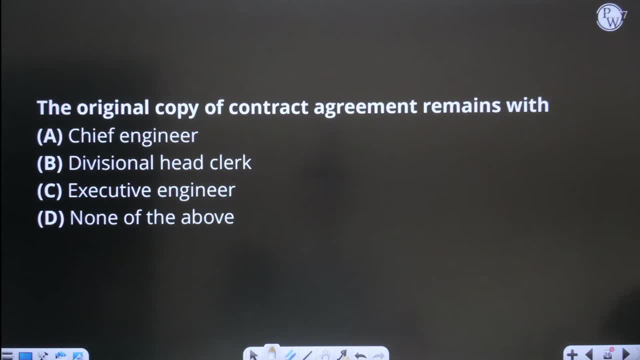 You understand. Look ahead, Take a report from another A. Okay, All the field work comes in the hands of J. What does field work mean? To do all the measurement, To become MB. All the books are made. Actual checking of things. 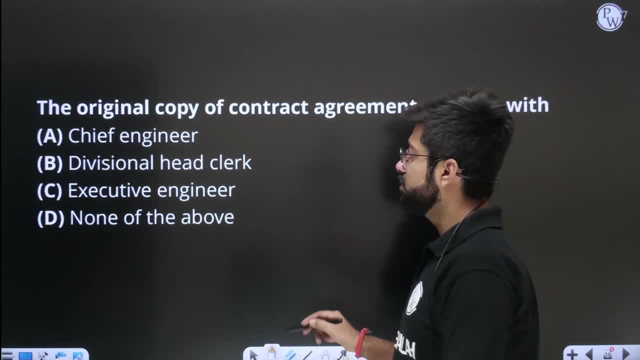 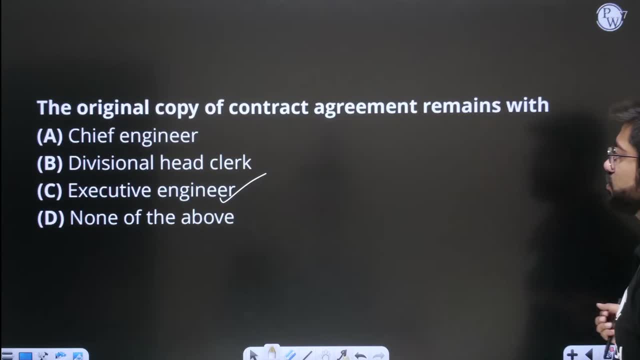 Quality checking. Everything is in the hands of J J. people earn a lot of money. Okay, For now. yes, Who will have the original copy? Obviously, the head of the division. The head of the division who is the executive engineer? 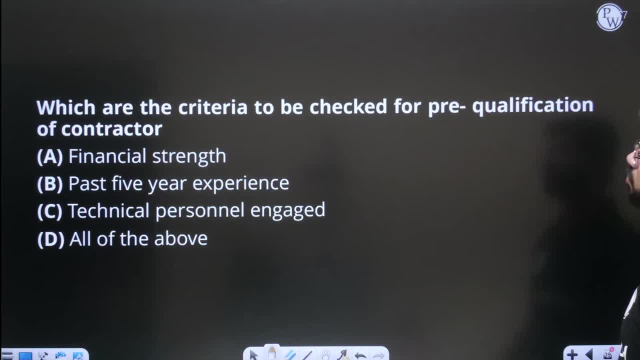 What are the criteria to be checked for? pre-qualification of contractor- Pre-qualification: Okay, First of all, you didn't tell me about opening the tender. You will have to explain how the tender opens. This is a very important topic. 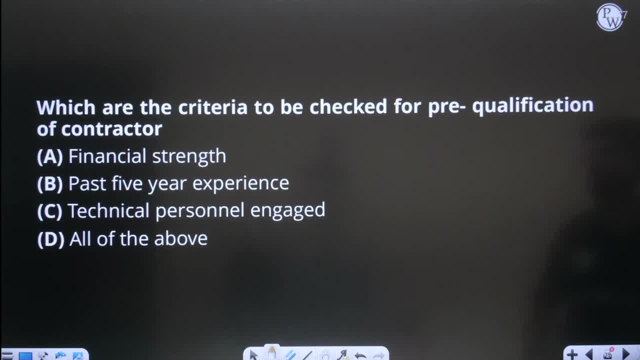 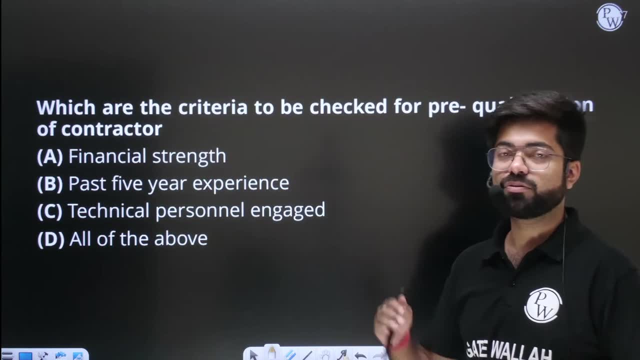 Let's tell this first, Then we will move forward. Tell me this first. So we, What things? J's promotion is done, Why not, Why not? Promotion is done Now. you will take out the exam in one or two years and become a J. 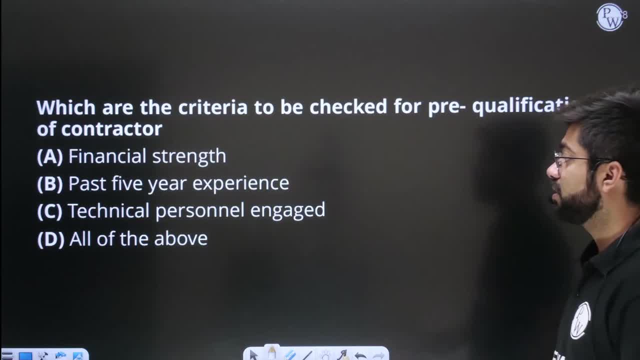 And if you become J, You will have to stay in the tender for ten years, Ten years, fifteen years. There is no limit. It takes a lot of time. That's why people prefer to take out the paper. What is in it? 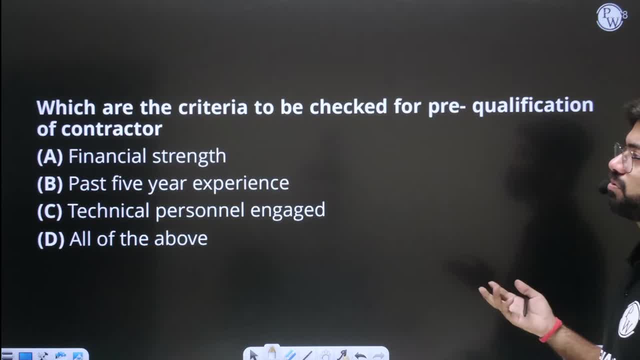 Otherwise, whatever you become now, the father will never be able to become J, Isn't it? There are different systems of all this. No tension, Yes. So what is in it? We will understand the financial strength of the contractor. Is it strong or not? 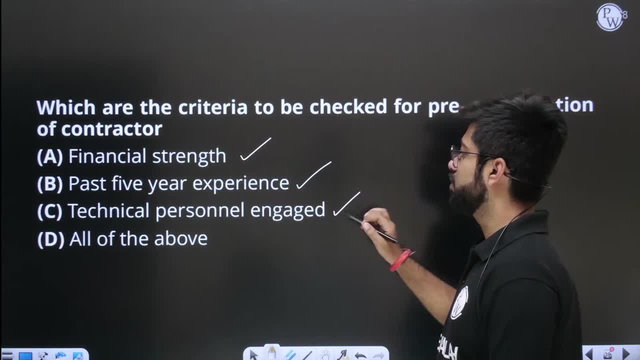 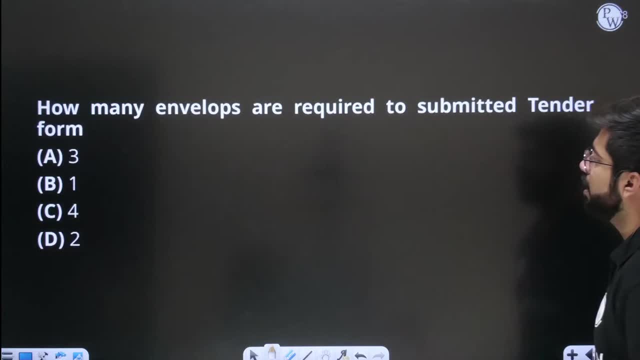 The past five years of experience should be at least good, And It should be technically sound. He has already done a lot of work like that, So obviously its answer will be D. Okay, The next question is that when the tender opens, 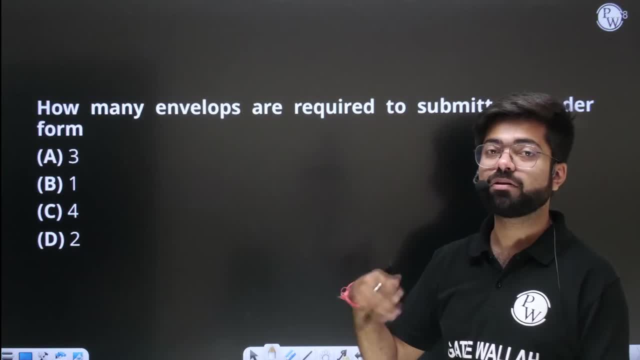 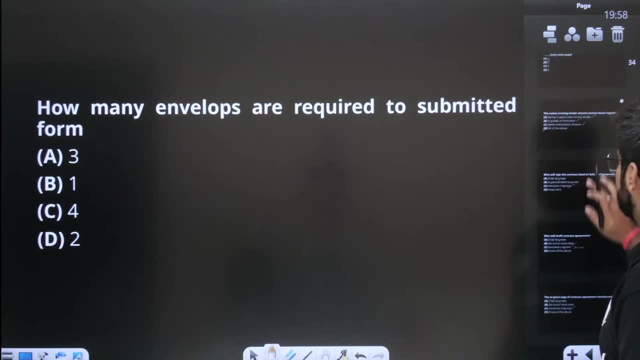 Different people have filled the form. So when the tender opens, how many envelopes open? So to understand this, we will have to add a slide here first. Or should I tell you here? Let's tell you here. But tell me here or tell me behind. 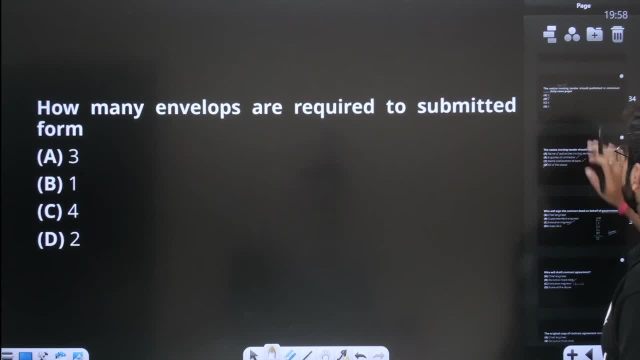 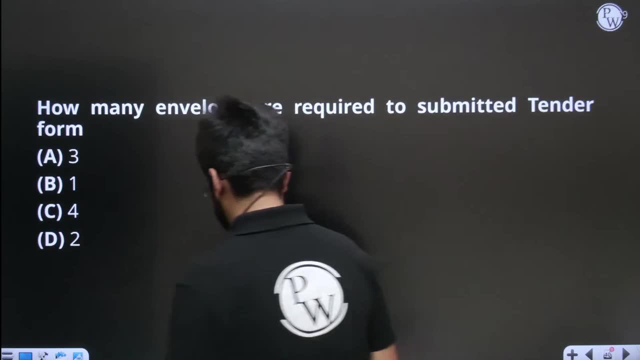 Let's tell you here. What difference does it make, Isn't it? Yes, Let's tell you here. So see how many envelopes there are. Let's make a little here. Listen very carefully. This can be asked in your exam. 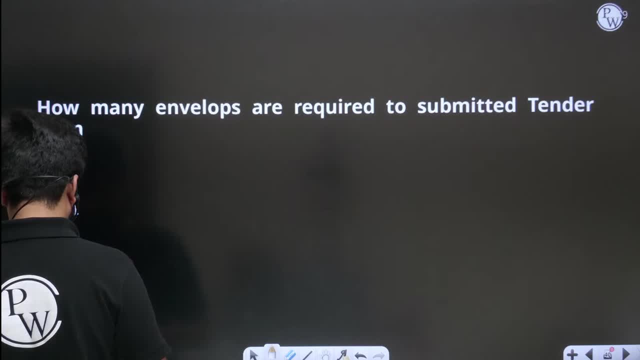 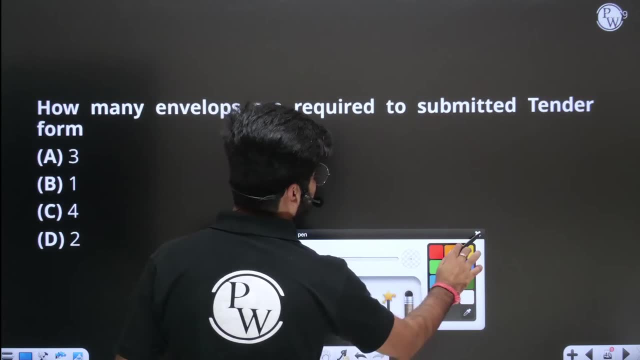 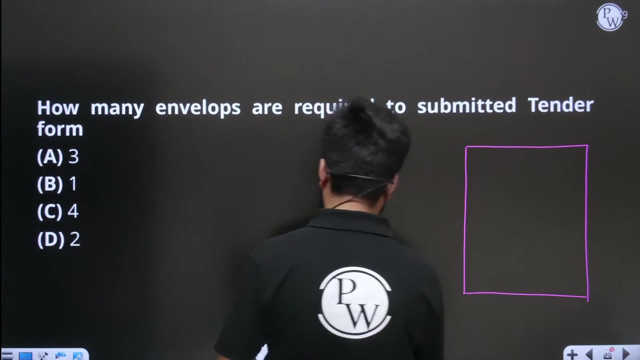 Okay, Everyone will pay a little attention here. It's not very tough right now, Anything in it. So there are four envelopes here. mainly, Let me show you one by one. See brother, One, One One. He is our envelope number one. 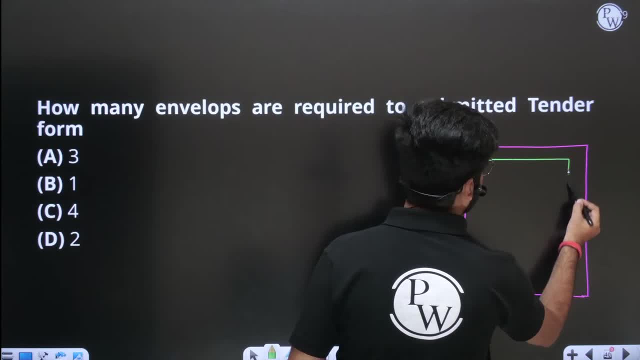 This has become our envelope number one. This is our envelope number two. Generally it happens okay. Generally, when you go, you will get it done. once When you become Ajay, all the things will be understood at once, okay. 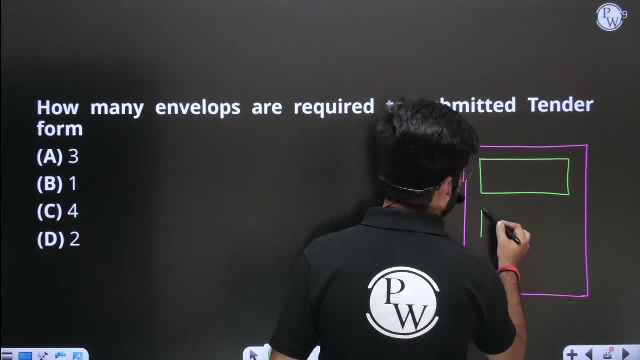 So now look over, there We are doing numbering. This is one, This is Ajay, This is Ajay, These are the ones. Yes, Yes, Yes, Yes, Yes, Yes, Yes, Because the number works. Yes, 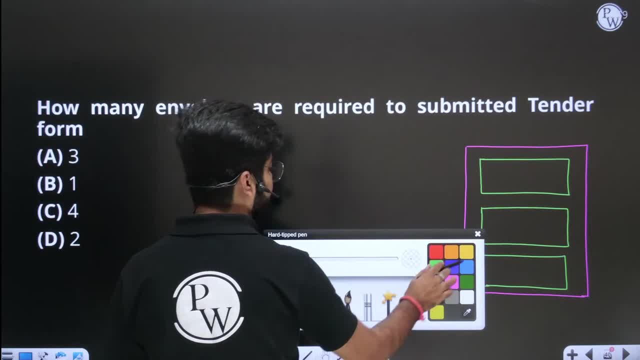 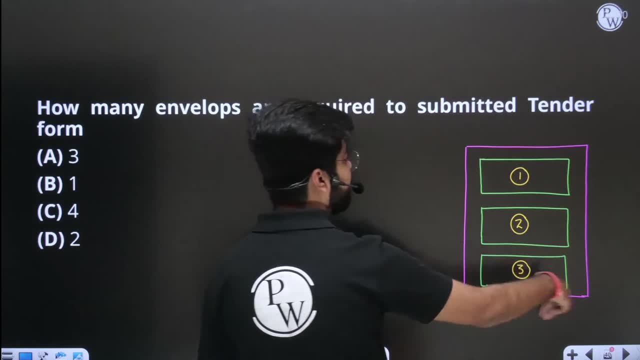 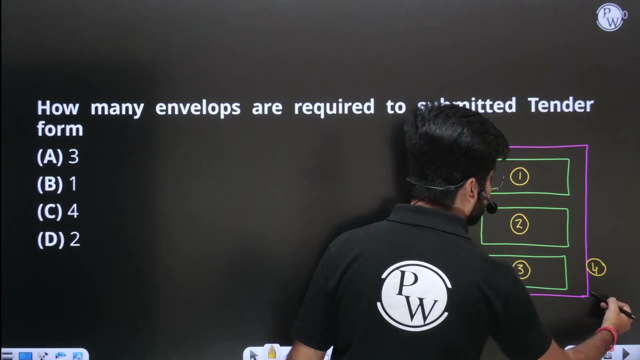 Yes, Yes, Yes, Yes, Yes. this is 2,, this is 3, and 4 is a big envelope which contains 3, this is a very basic thing, because in this way, every contractor will submit their own envelope. now the client will open it to check. 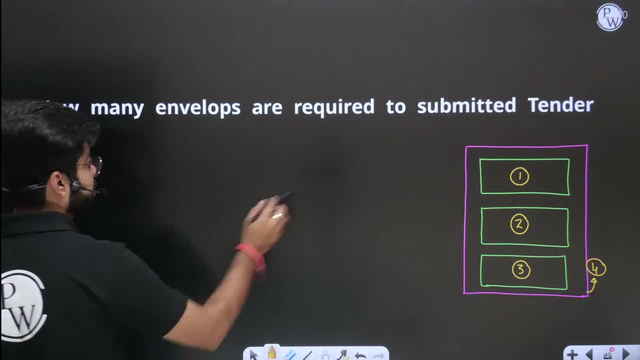 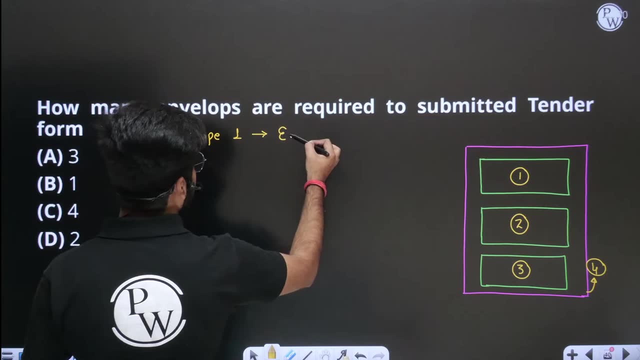 so we will tell you how the checking will be, what will be seen. so, first of all, the envelope 1, what will be in envelope 1, it is the earnest money deposit. generally it is FD. in the earlier times cash used to run. 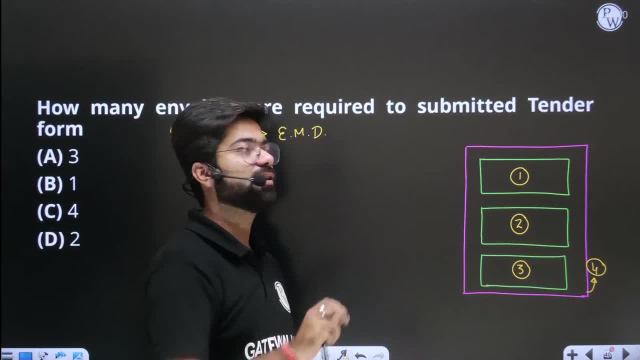 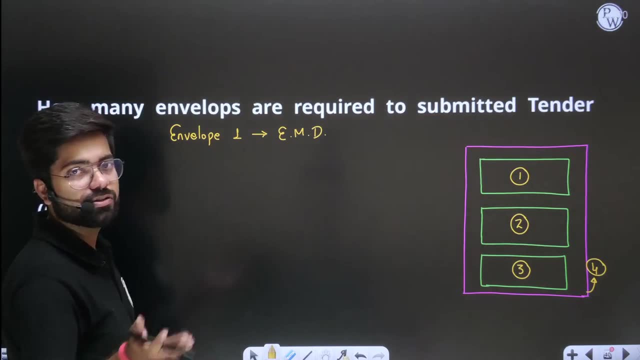 so it used to be kept in the cash chest. the cash chest used to be kept in the division okay note etc. so in envelope 1, the earnest money deposit will happen, which every person gives, every tender which will fill the form will give. 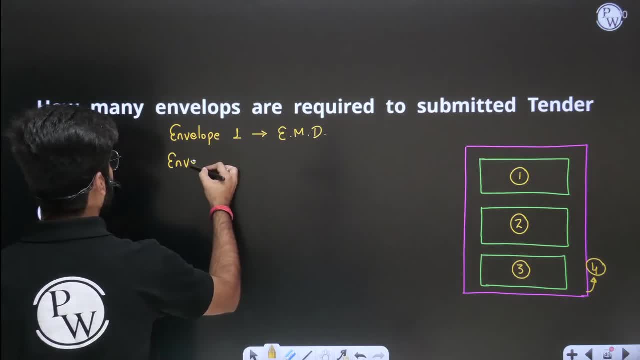 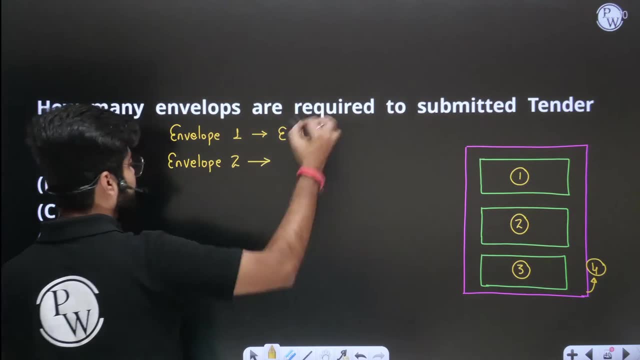 so in envelope 1, it will be EMD. what will happen in envelope 2,? in envelope 2, it will tell about itself that how much technically we will submit. we have this amount, we are like this, we are like that. okay. 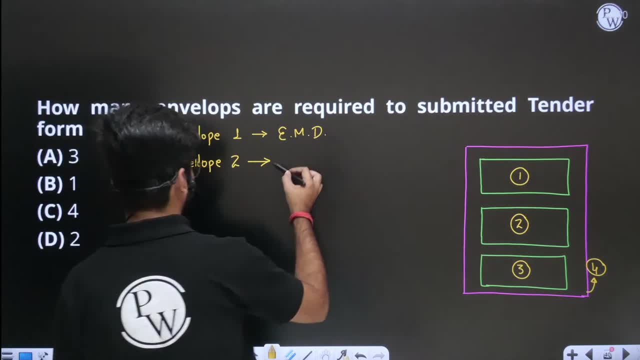 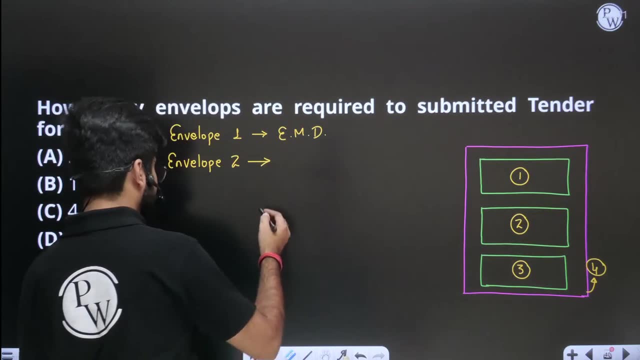 all the technical quality will be written here. the technical certificate of the contractor: okay, it has some standard certificates, all those things will be in it. okay, let's write here. the technical soundness of the contractor is written in this envelope, okay. 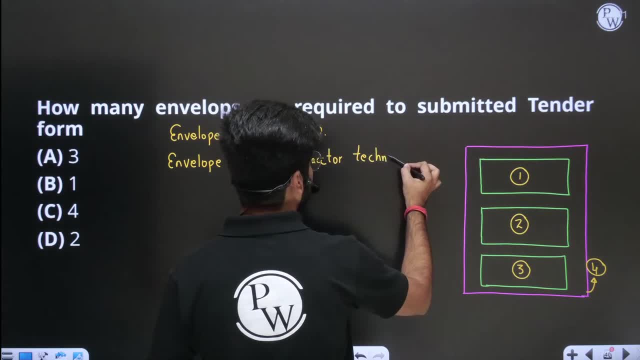 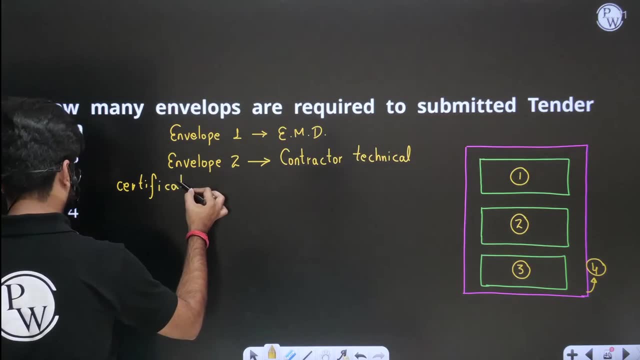 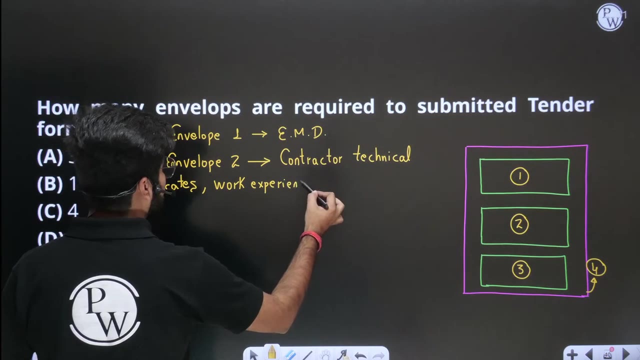 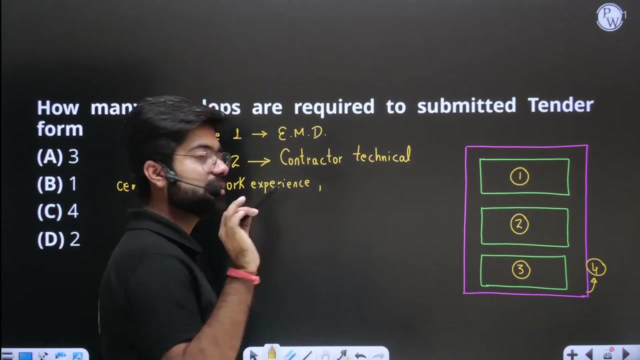 so the technical certificates of the contractor, which were asked, the technical certificates of the contractor, are written over here, okay, okay, How much experience does he have in his work? The work experience of the contractor? His registration form, whether his company or firm is registered or not? 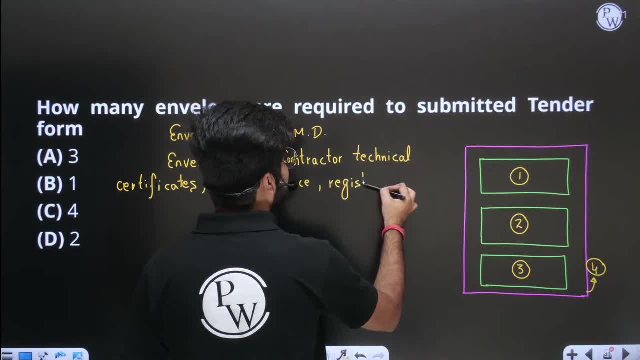 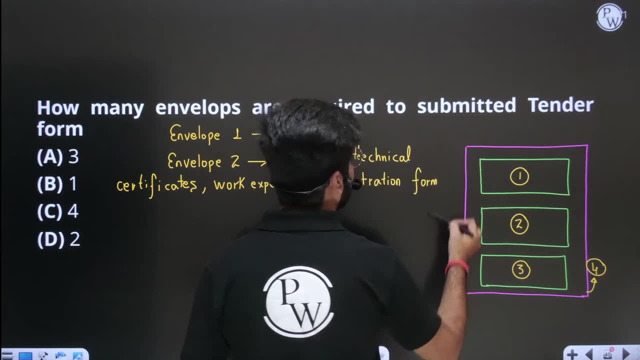 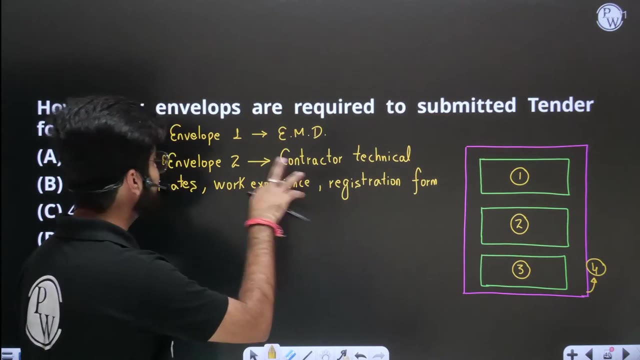 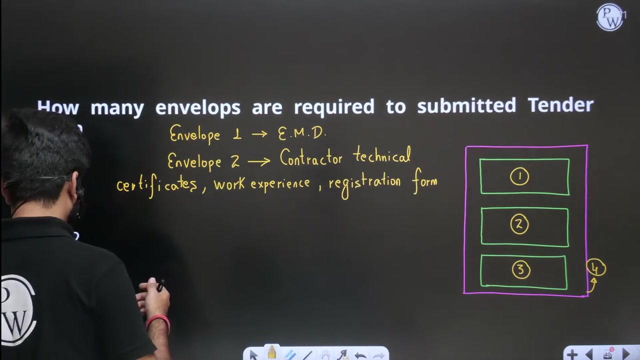 Tax details, GST details, etc. When you fill a form for an exam, what do you ask? 10th mark sheet, 12th mark sheet, etc. These are your technical specifications To fill that form: registration form, Tax details, etc. 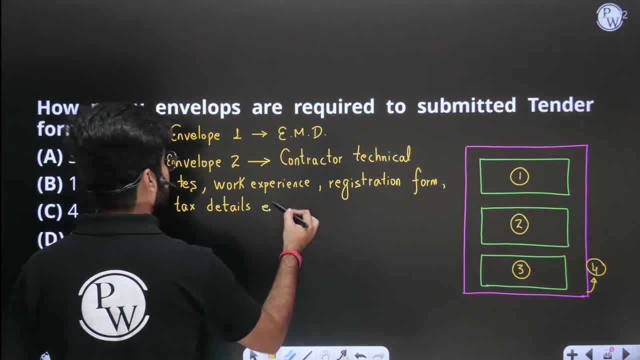 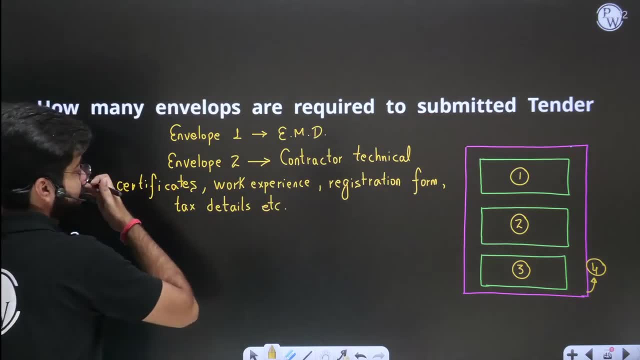 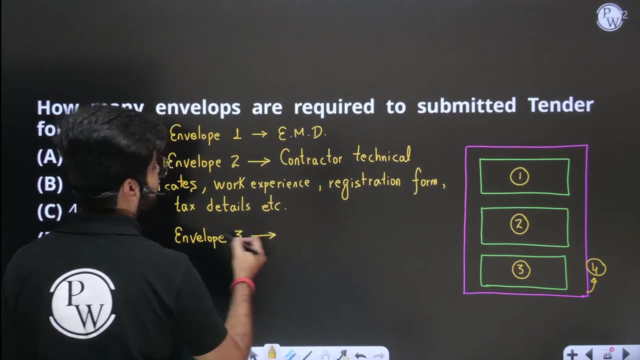 Or, if you want to add something to it, You can see the achievements of the project. What will be added in 3rd mark sheet? The real thing in 3rd mark sheet is money, The amount of money you want to invest in the work. That is in 3rd mark sheet. 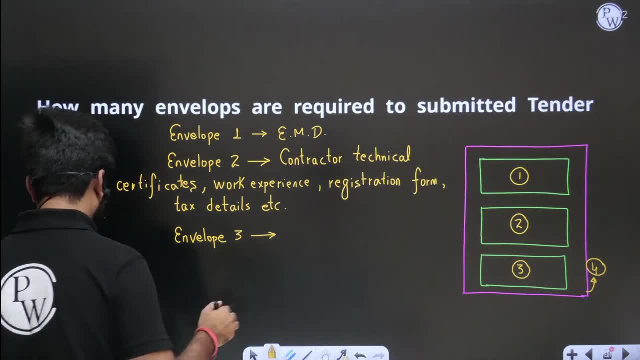 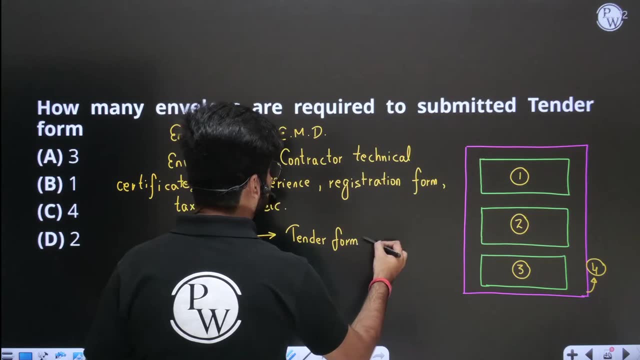 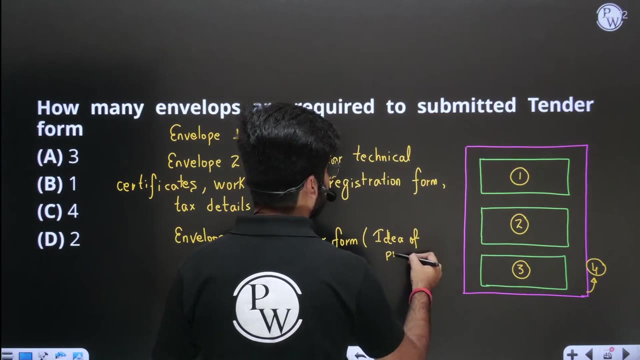 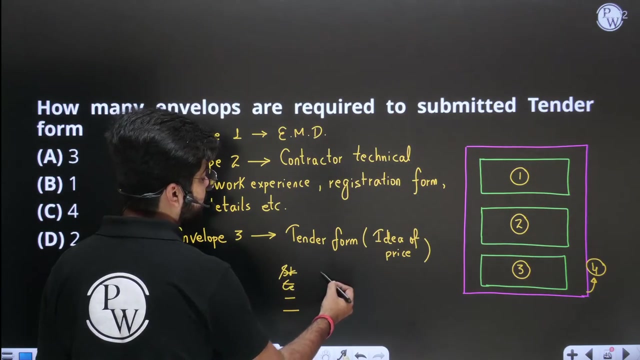 It should be less than or equal to. This is tender form. The tender form is the exact idea of the price. The idea of the price is written in the form. The contract is written in the form. The rate of the contract is written in the form. The rate of the contract is written in the form. 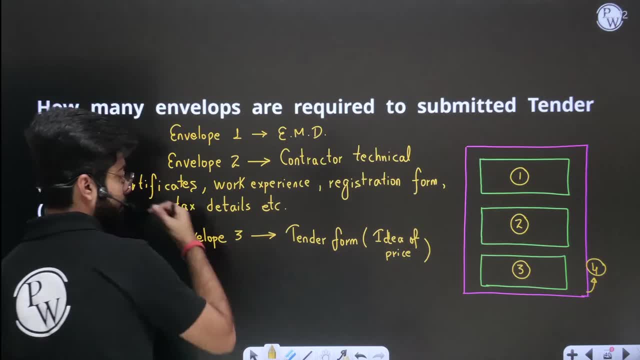 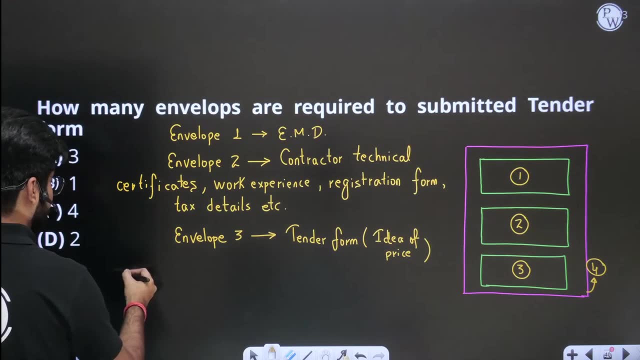 The contract is filled and the form is deposited. When the form is opened, how does it open? If you see the sequence, then tell me What will be the opening sequence If the tender form is opened. What will be the opening sequence? Obviously, the 4th tender form will be opened. 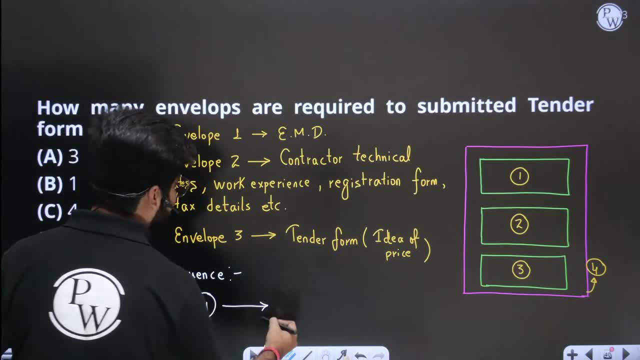 Obviously, the 4th tender form will be opened. What will be the opening sequence? The 4th tender form will be opened. Is it serious or not? Did he deposit the earnest money or not? Is there any seriousness in it? Okay, sir, he also gave the money. 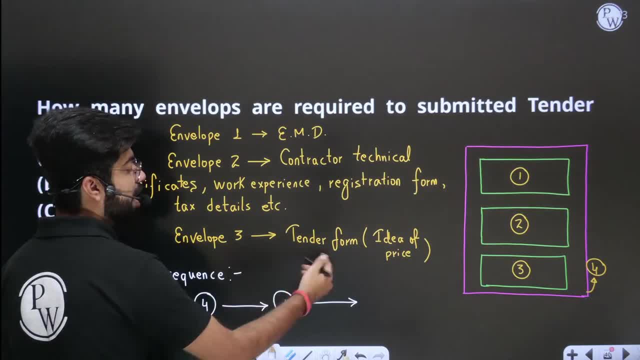 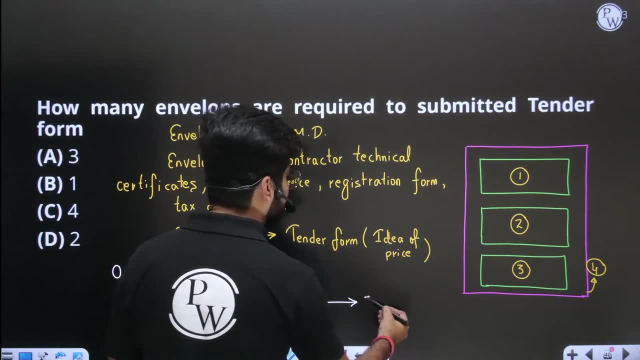 Now when he gave the money, then we will move forward. If this is not there, then we will not move forward. Understand the rules. 10 tender forms have been read. If this is not there, then we will not move forward. If this is there, then we will go to the 2nd. 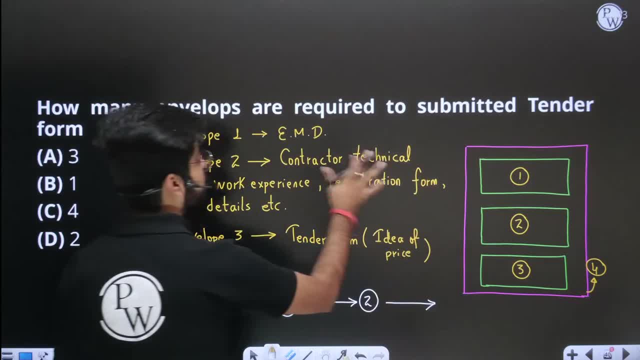 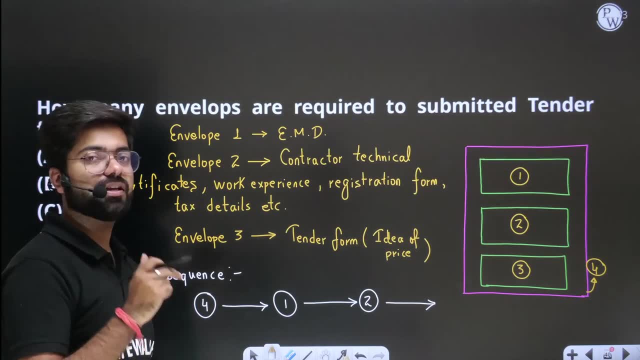 If this is there, then we will check the 2nd, Whether everything is in it or not. Whatever work experience, is there Registration form, tax details, If everything is good in it. If this is in the problem, Registration is not there. If there is any problem. 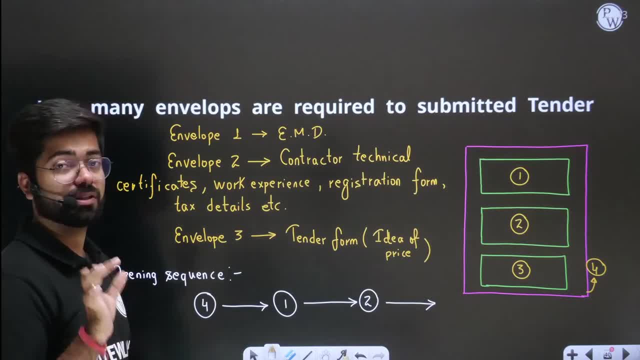 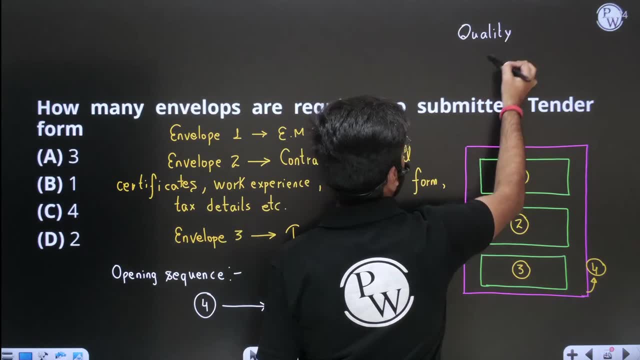 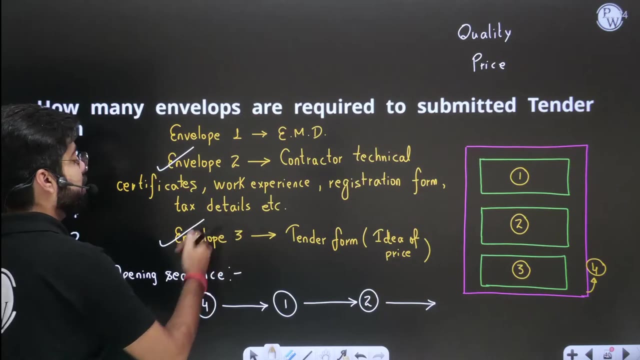 Then we will not move forward, We will not open the tender form. Quality is very important. Understand one thing: Quality plus price. Quality plus price are both. Now the quality is being checked From the second envelope And the price is being checked from the third envelope. How much is the price of that work? 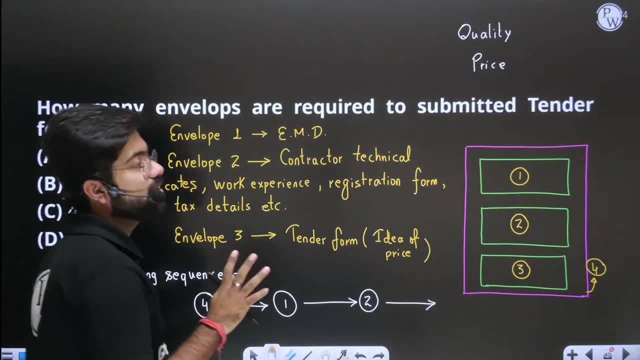 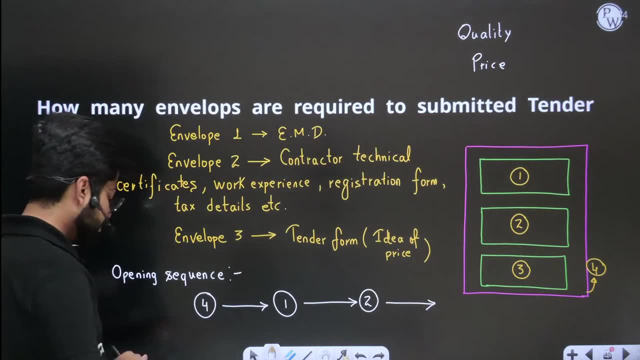 Understand one thing: If there is a problem in 2, If 2 is rejected, Then the third will not be opened. That entire envelope will be removed. Then the next envelope will be opened. Do you understand what I am saying? Is everything clear? What are you commenting? 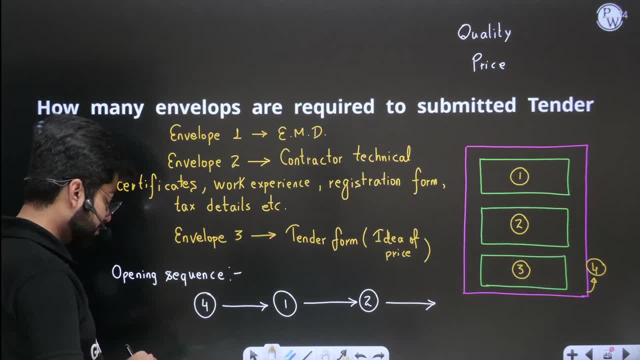 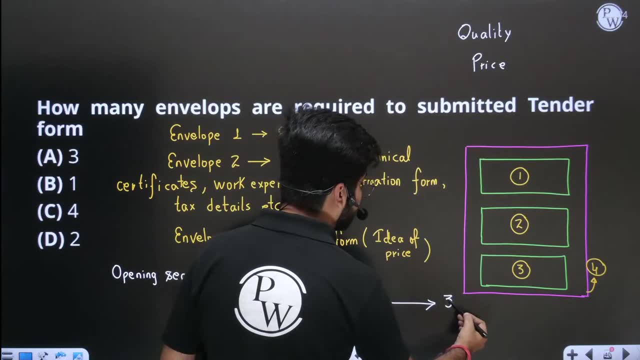 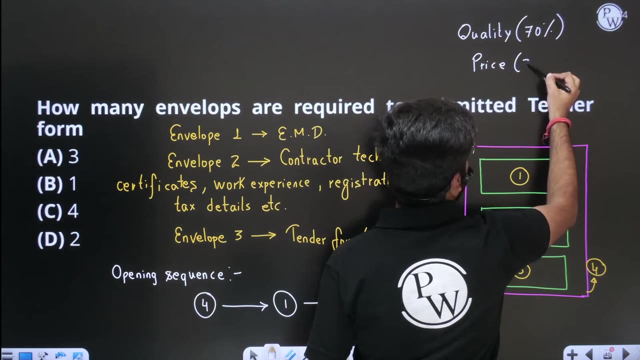 Okay, It's a very simple thing. Where is the comment? Yes, 412. And then what will be opened in the end? Third envelope: So now suppose you gave the quality 70% weightage. Now you are on top. You are a client, You can select it as you want. 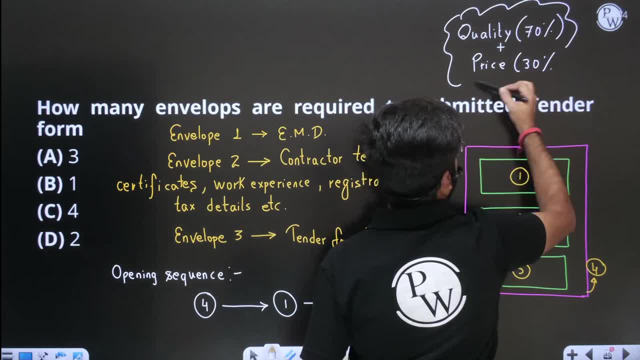 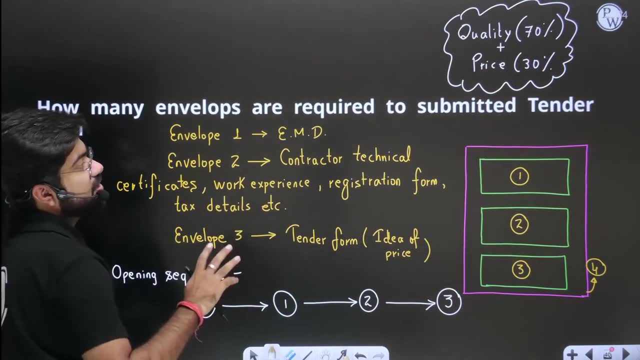 In this way you put your mind here: Weightage wise. You saw the quality 70%, So you gave the quality 70% number. You gave the price 30% number And the number of those who made the most By combining. You have selected that. So in this way, 4 envelopes are opened. 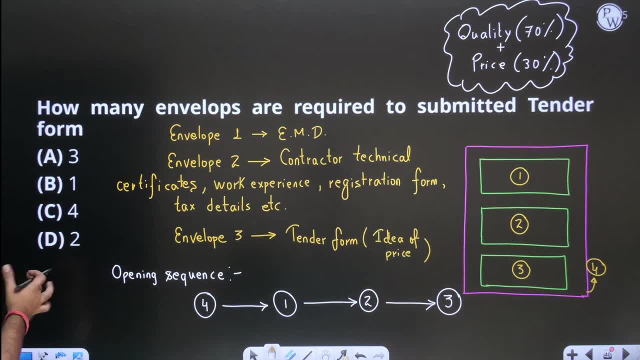 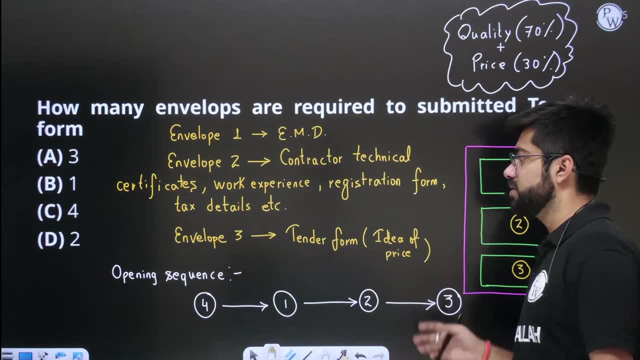 Okay, So I hope you will understand here. Okay, So if you ask a question like this, If 2 envelopes are opened, Right, Then which 2 envelopes will be opened Now, as you have seen here? So in 2 envelopes in the system, One will be of this and the other will be of this. 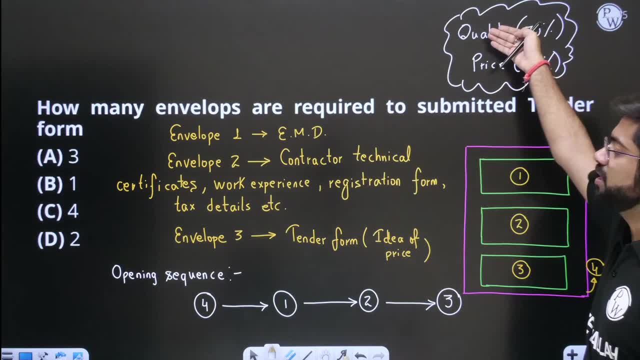 Okay, One will be technical specifications, In which the quality will be visible, And one will be your tender form, In which everything will be written in terms of price, That the rate of each item, Or whatever kind of contract it is. Everything will be mentioned in it. Okay, So what will be the answer? 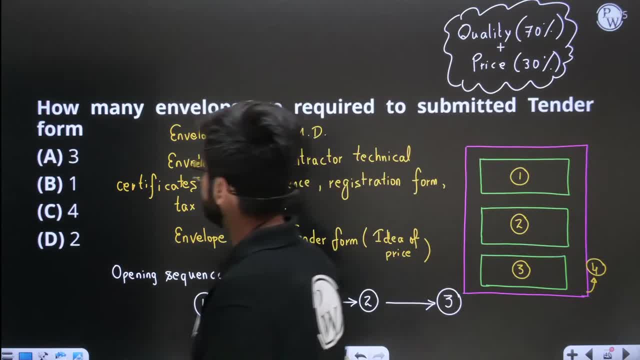 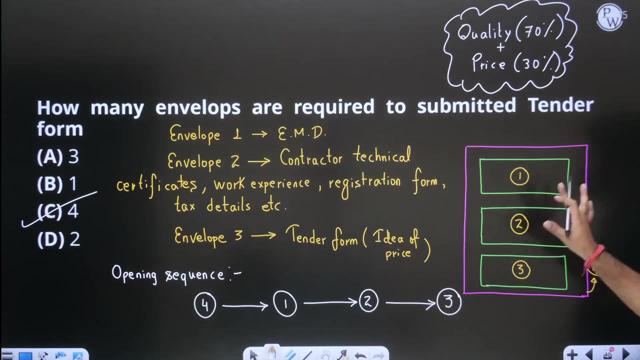 How many envelopes are required to submitted Right During tender. So how many envelopes are there here? 4, Is everyone clear now? Good, So what is the first one? 1, 2, 3, 4, 5, 6, 7, 8, 9. 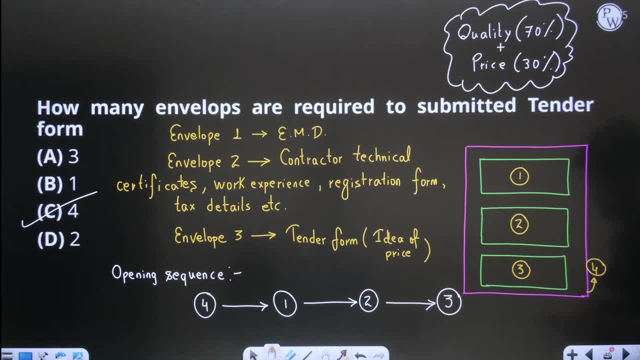 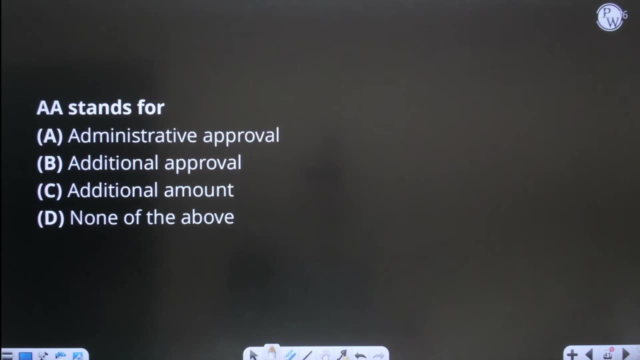 10, 11, 12, 13, 14, 15, 16, 17, 18, 20, 21, 22, 23, 24, 25, 26, 27, 28, 29. What does it mean to take the medicine here? There is an additional amount with C, but this is wrong. 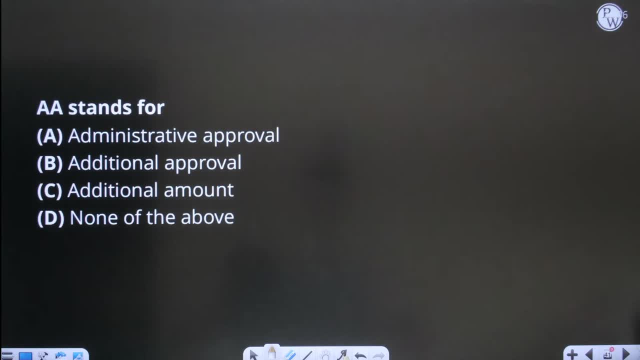 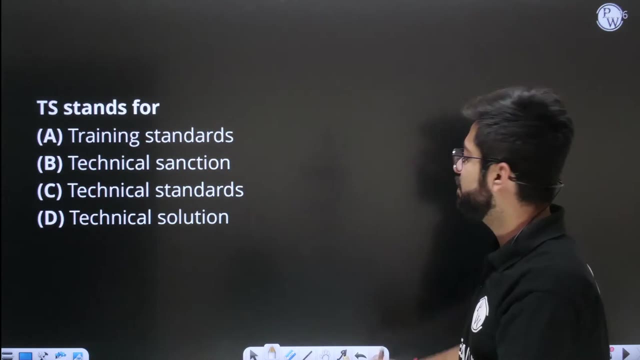 What will be the meaning of double A here? Administrative approval is correct. So first of all, administrative approval is done. Okay, Whenever a department engineer makes any project, then administrative approval is taken. Then what will happen after administrative approval, When administrative approval is obtained? 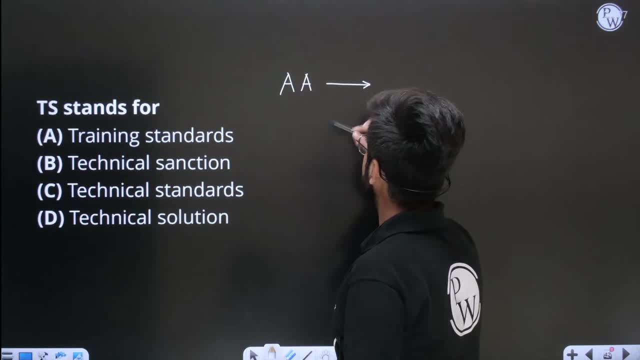 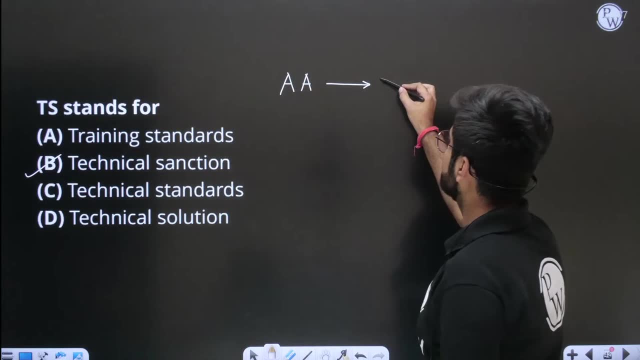 then its technical system will be checked. Technical sanction will be done. here TS means B- Okay, TS will be technical sanction. Then financial sanction will be done. Then financial sanction will be done, And after that, when, all the sanctions will be done. 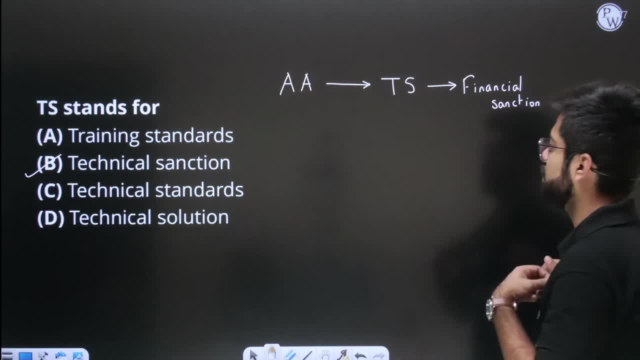 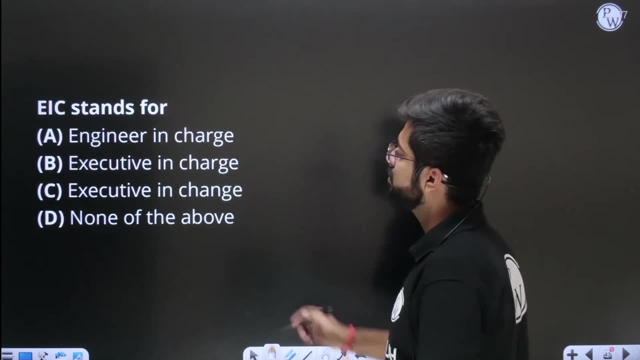 the money will come. Then everything starts to become NIT. So TS stands here for technical sanction. Then who is EIC? EIC means engineering in charge. No Executive in charge. No Executive in charge. Yes, EIC means engineer in charge. 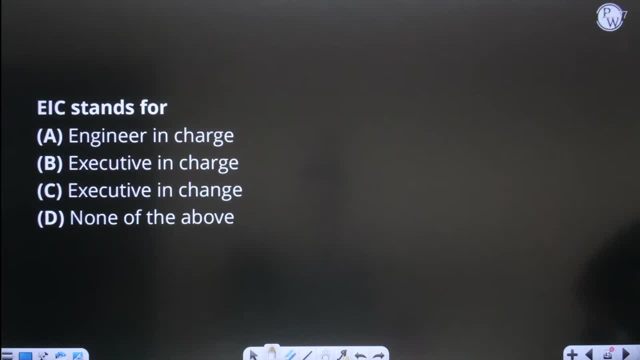 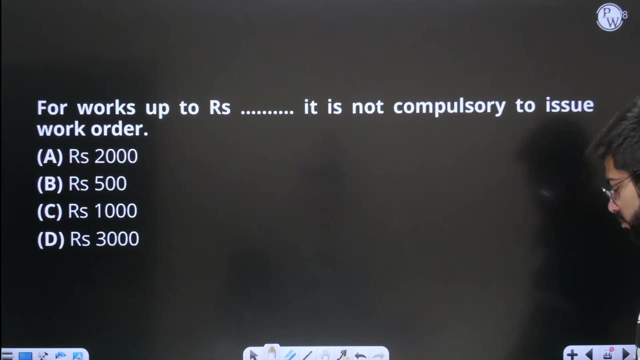 Yes, Correct. EIC means the engineer who is in charge here. This is the option. There is EIC here. Here it is EIC. OK, So EIC means EIC means engineering in charge. All right, Agreed. 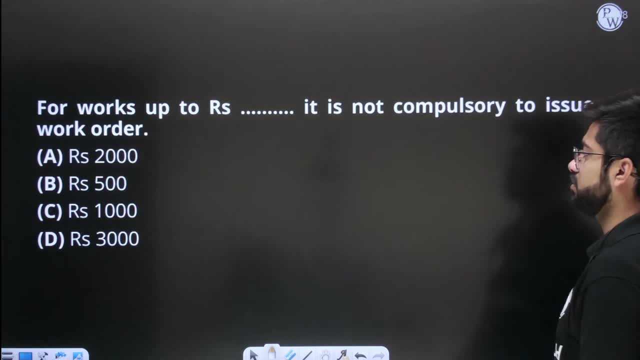 EIC means engineering in charge. Yes, EIC means engineer in charge, Because this is the same engineer who is in charge and the same work will be purch GOT by us. Then the work is up to how many rupees? It is not compulsory to issue a work order. 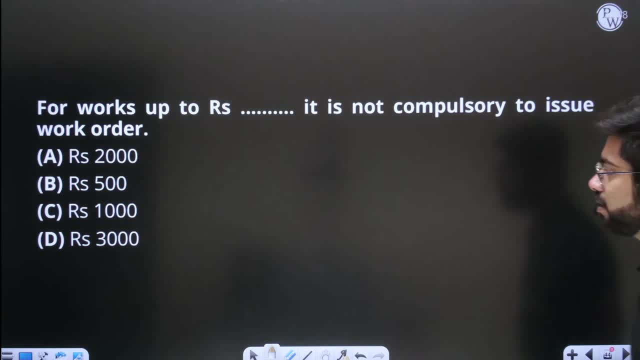 These people usually do work order OK For small works. He works so much that there is no need to do work order. Are many small works? How much work is required to order work from below Rs 1000,, Rs 500, Rs 3000?? 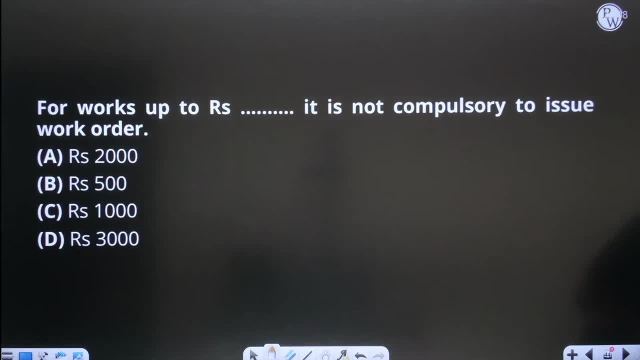 See what you are commenting. How much will be the answer? Absolutely correct. How much is the A in this? No, it will not be A Rs 500.. Obviously, no need to order work from below Rs 500.. 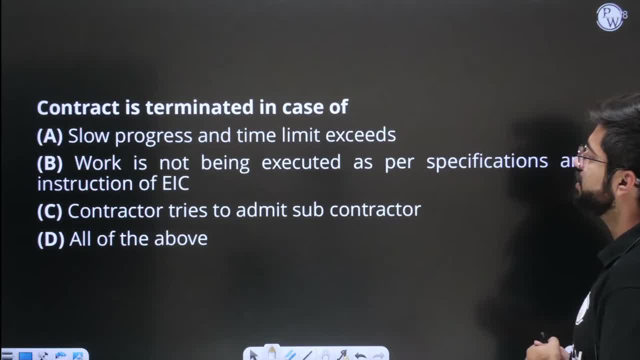 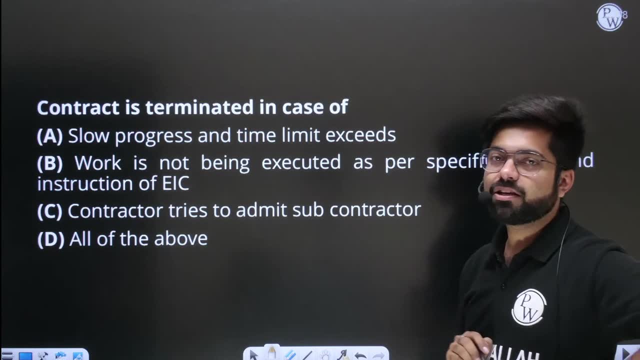 It is a very small work. Then it is said that the contract is terminated in case of The contract will be cancelled when the progress is very slow. The contract will be terminated when the progress is very slow. Work is not being executed as per specifications. 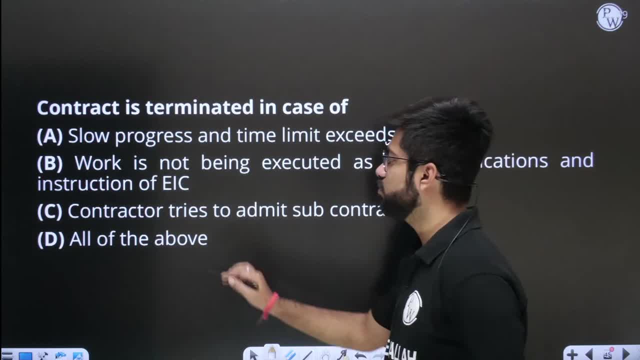 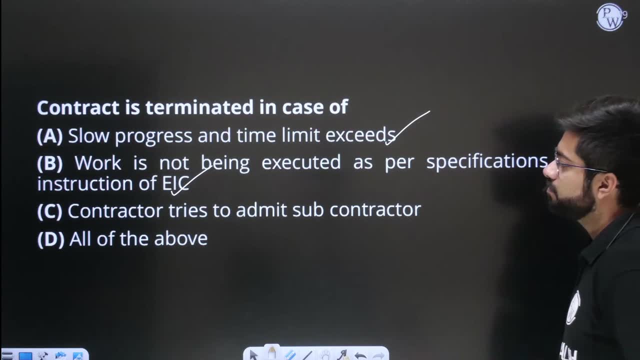 It is not being done as it was told And the engineer in charge is not following the instructions, Even then the contract will be terminated. Okay, Engineers are not listening to them, They are not following the specifications. Then, obviously, the contract will be terminated. 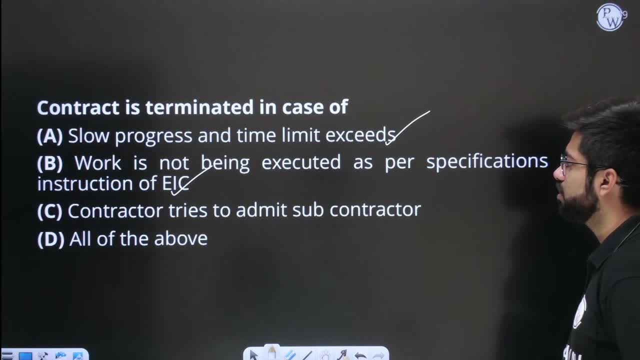 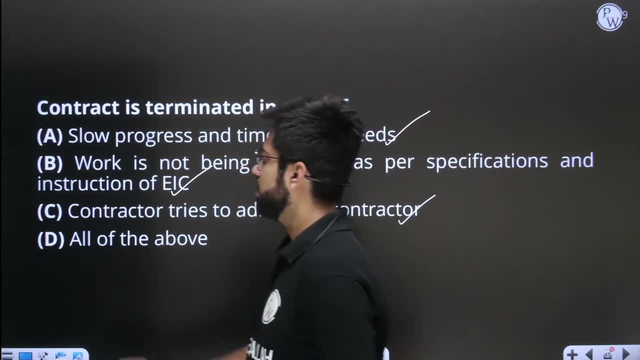 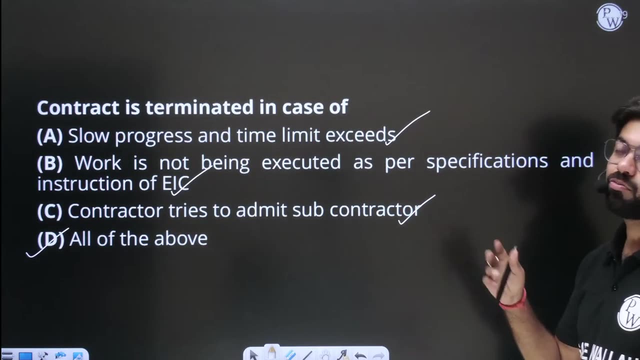 It is written in it. Subcontractor- Absolutely correct. If all these things start happening, Then our contract will be terminated. Okay, Contractor of any thing. Delay anything, Don't listen to anything. Okay, Subcontractor, This contractor will be terminated. 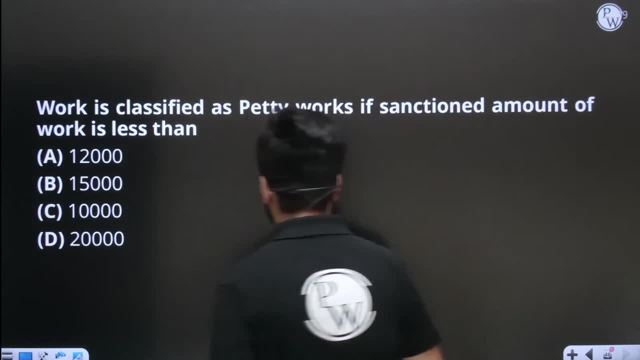 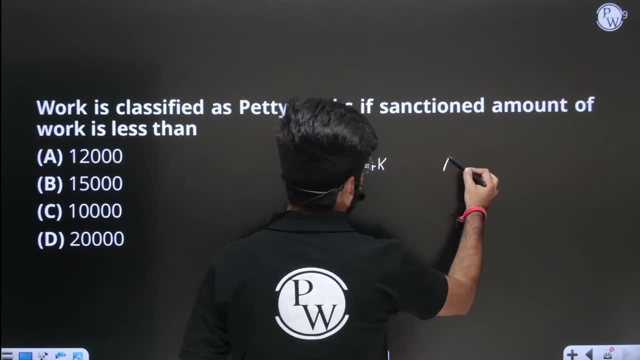 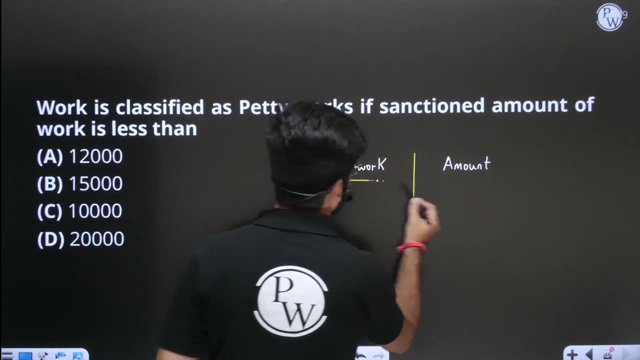 D option is correct. Next, Work is classified as petty work if sanctioned amount of work is less than What are petty works Work? And here we will talk about the amount. Okay, See, If the work, Come on, you guys tell me first. 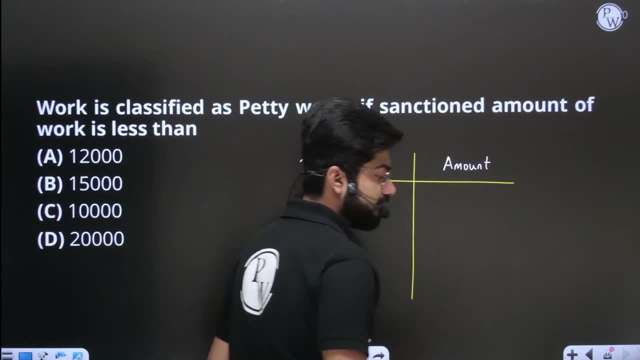 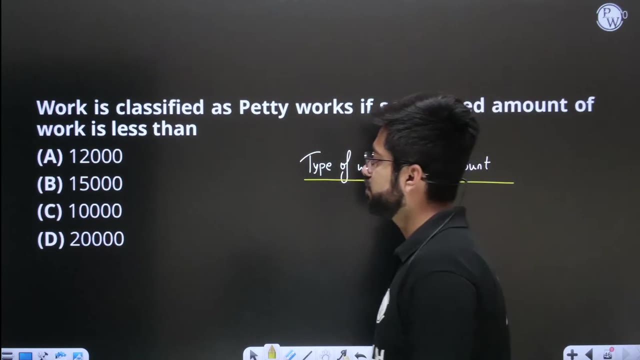 If our amount, What are you telling Petty work? With whom are all going? Hmm, With whom are you going in petty work? Tell me, People are going 10,000.. Yes, 10,000 and 20,000.. 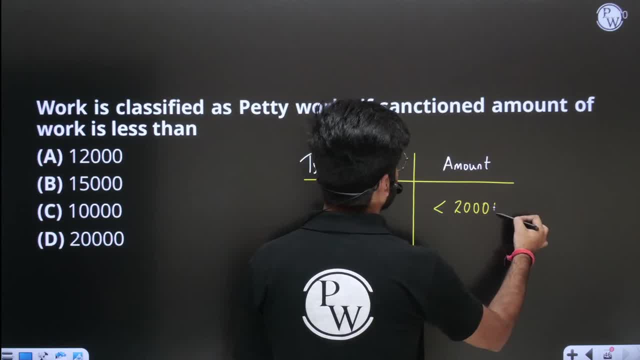 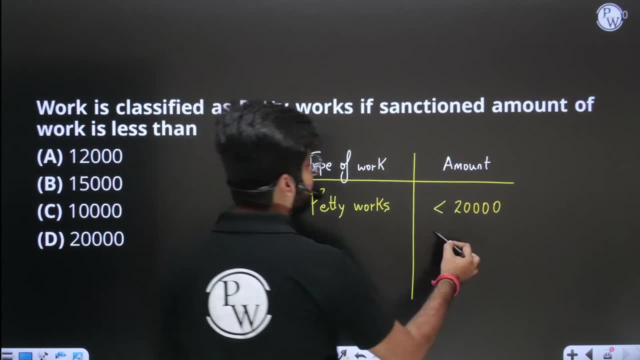 Let's assume 20,000.. Okay, If the amount is less than 20,000.. If the amount is less than 20,000.. Then we will keep it in petty work. Okay, If the same amount is less than 20,000.. 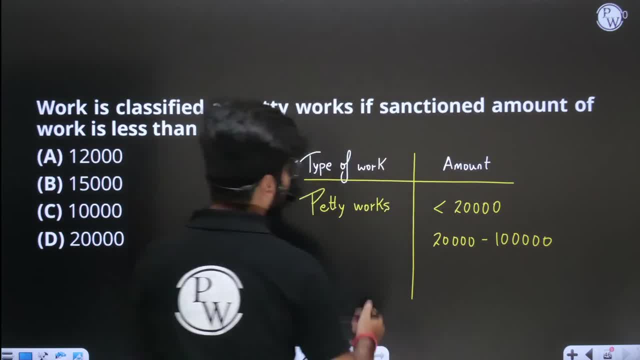 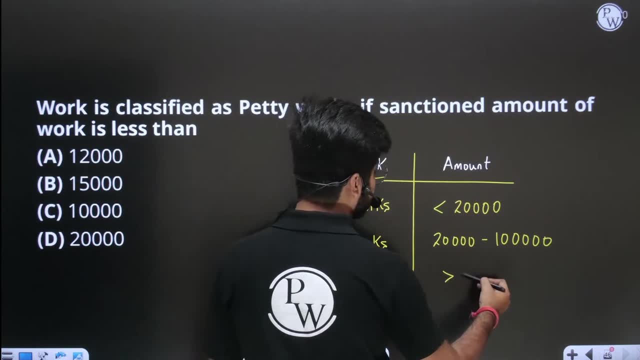 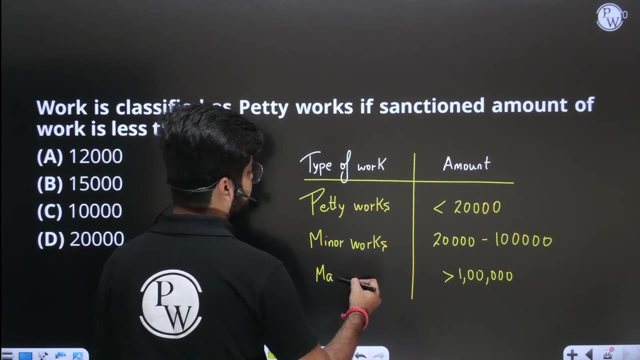 Some small repair, etc. In which 1 lakh is taking 50.. Okay, Then we will keep it in minor works If the work is more than 1 lakh. Okay, If the work is more than 1 lakh, Then we will keep it in major work. 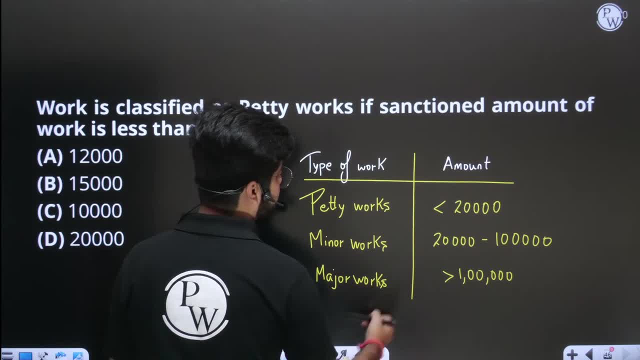 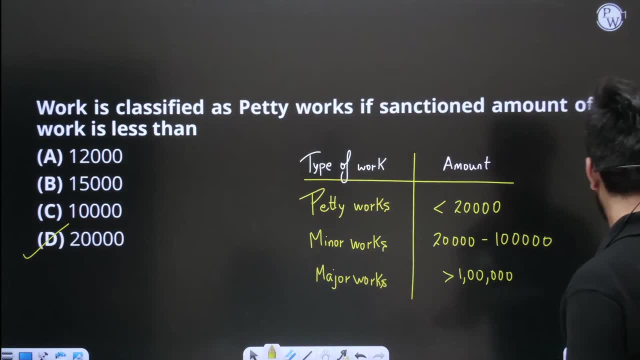 Now what will be the answer? It will be kept in major works. So we will call work petty work When it will be less than 20,000.. Okay, D option is correct. here Is everyone clear. Yes, D is absolutely correct. 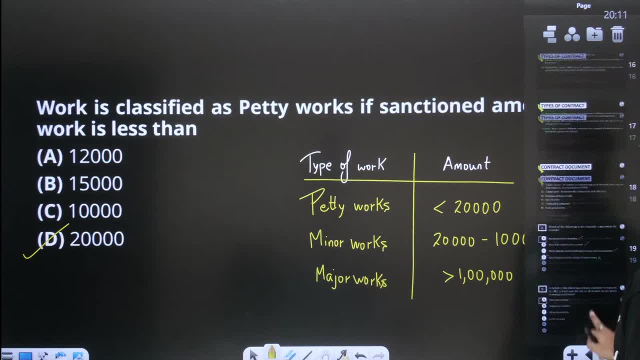 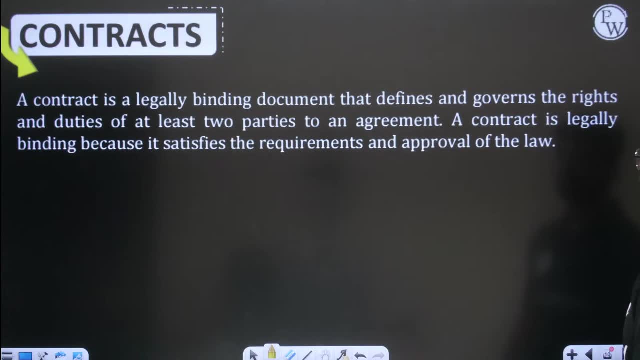 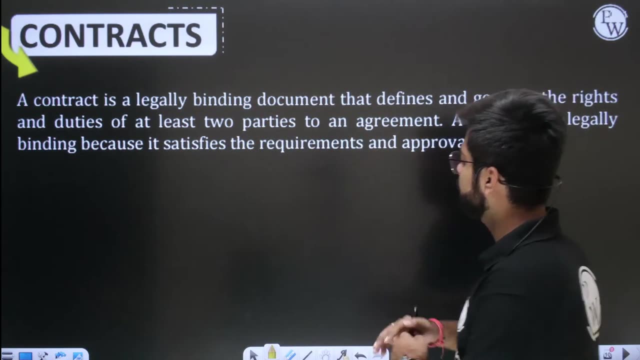 Now our simple work is left, Then our class will end. You will understand everything here. So What is contract? We told you this. We had read it here. So what is contract? It is a legally binding document. If we understand contract vs agreement here. 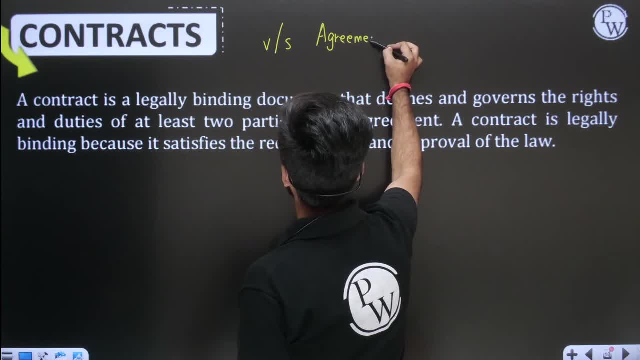 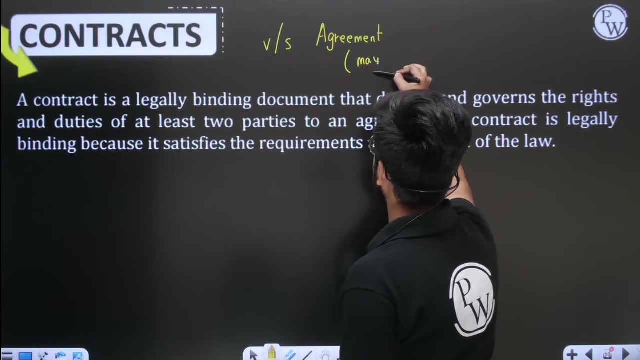 If we understand contract vs agreement here, So agreement and contract have only one difference. In agreement, Enforceable of the law can be May or may not be May, or may not be May or may not be Enforceable by. 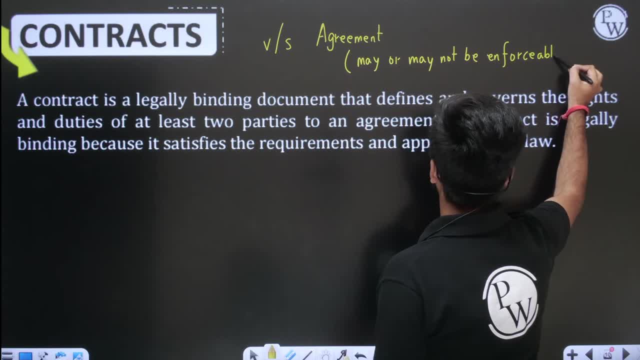 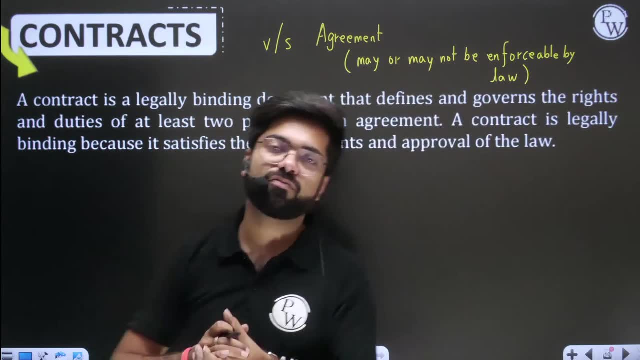 Enforceable by. But if there is a contract, Then I swear to God There is a legal binding in that. Legally, both parties are binding And we have to follow, Otherwise the court case will be in trouble. Contract is a legal binding document. 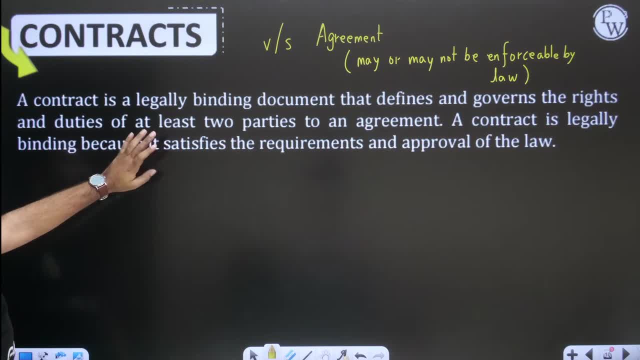 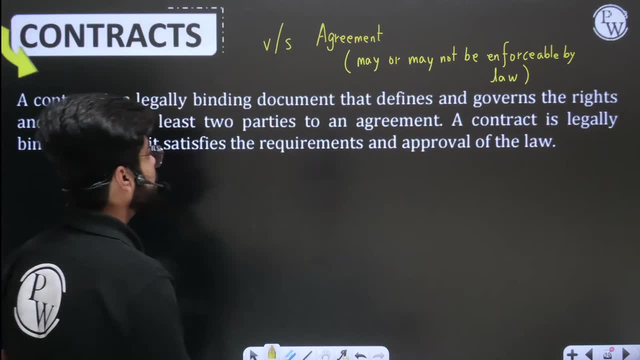 That defines and governs the rights and duties of at least two parties. That defines and governs the rights and duties of at least two parties, And then FIR starts. First information report goes, Then things increase. at one level, Contract is legally binding. 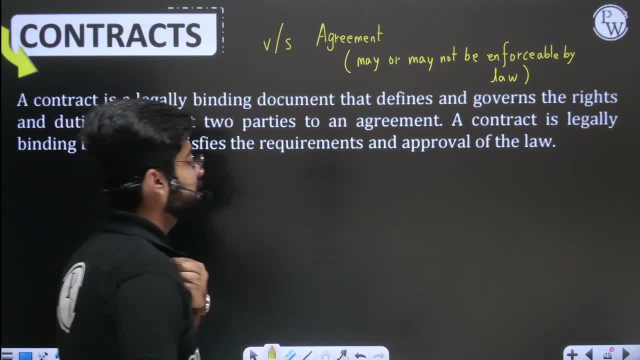 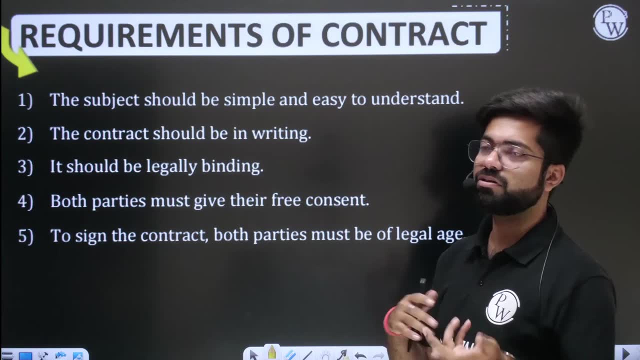 Because it satisfies the requirements and approval of the law. Law comes in between. So this is contract. Well, do this properly. Do what we want. We will do what you want. Pay us and our work is done. Now what are the requirements? 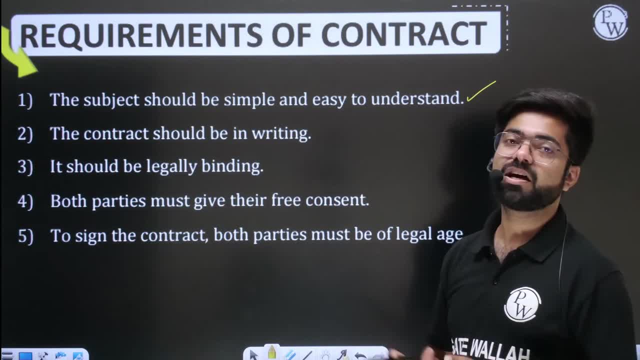 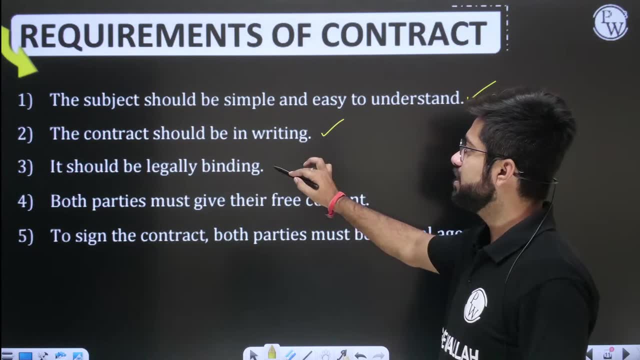 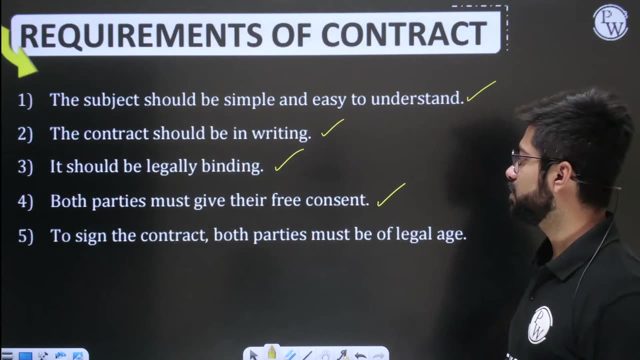 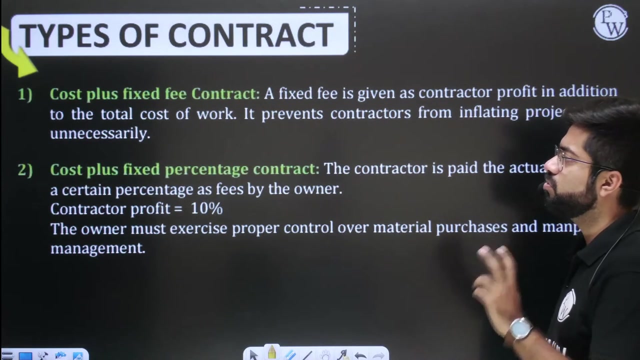 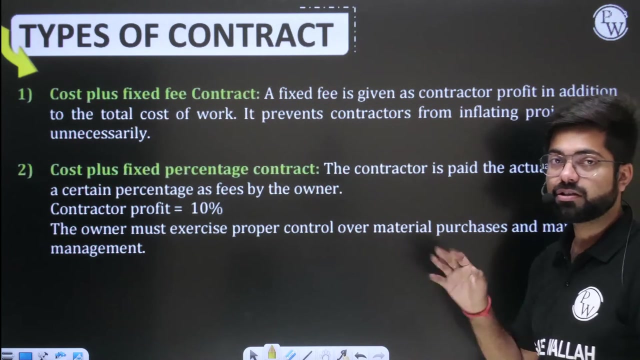 Subject should be simple and easy to understand. Like I said, Contract must be in written form. A written document is very important, In which both parties sign. Legal binding must be there. Both parties must have free consent. it is not that they are being forced to do it, it should not be forced. both should agree. then it should be good work. then both the parties will sign it by staying in the legal domain, ie by staying in the legal domain, by staying in the domain of the age or whatever things are specified. they have to sign it. it is a basic thing. now we have to understand the type of contract of the world. so it is a little important. listen carefully here. first of all, our cost plus fixed fee contract is. 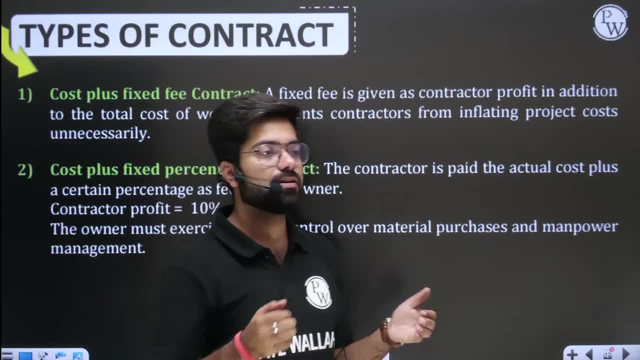 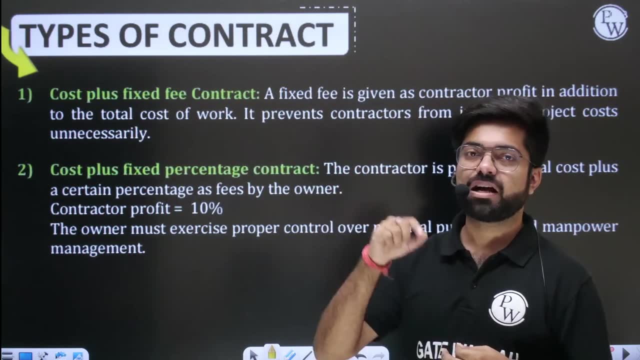 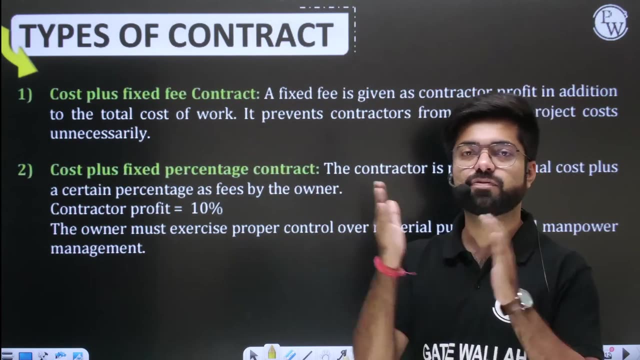 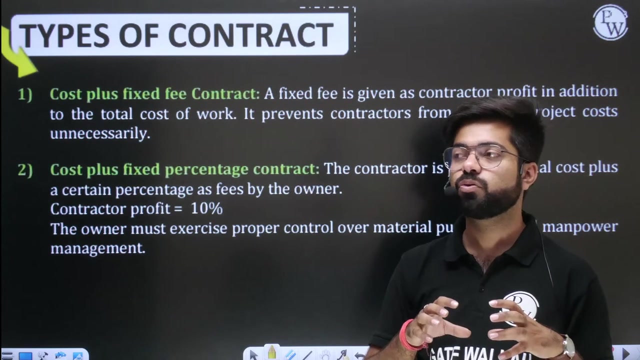 what happened in the cost plus fixed fee, that whatever the cost is, let it be the work that is going on, let it be. apart from that, you will get so much money for this work. it is fixed. it cannot increase or decrease. you will get fixed fee, fixed fee. you understand the name: cost plus fixed fee. let the cost be, let it be plus a fixed amount will be given. now the owner gets a little benefit in this. why? because the contractor will not forcefully try to increase the cost here. when he will forcefully put the bill, then he will increase the cost. 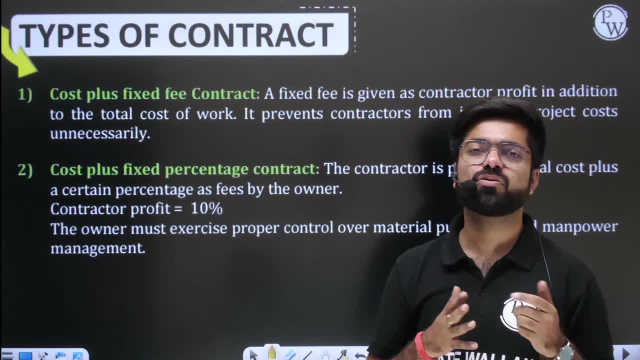 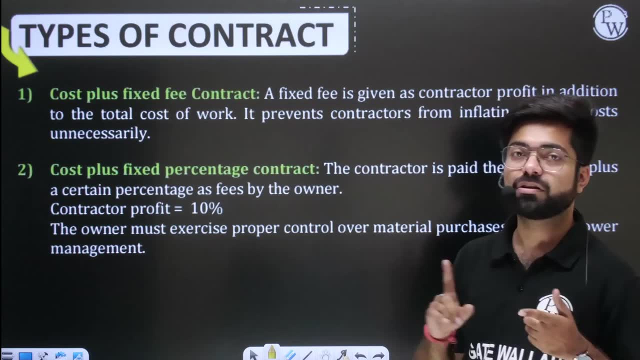 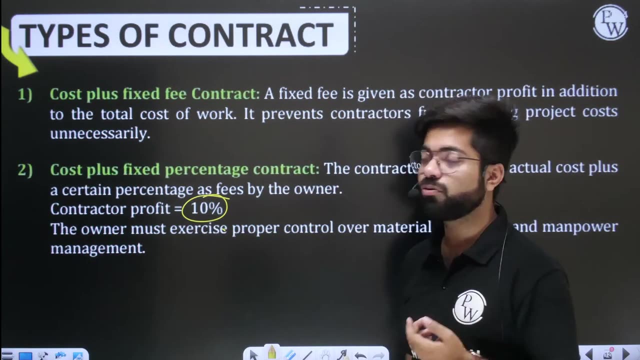 not work but work on the amount, because he has no extra benefit. he'll get his 10,000, he'll get his fixed fee. then why will he increase it? you understand that? then why? but if the- if it happens- your cost plus fixed percentage- let's say the contractor profit is 10% and the work is of a million, then 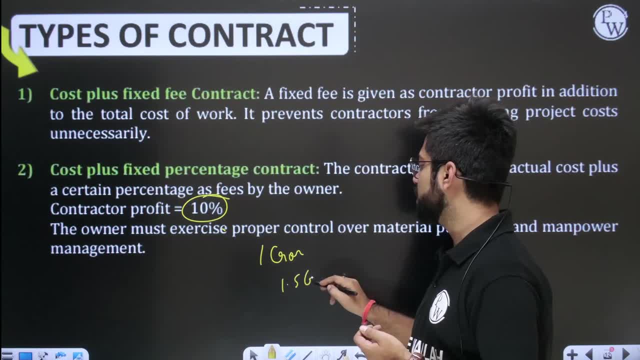 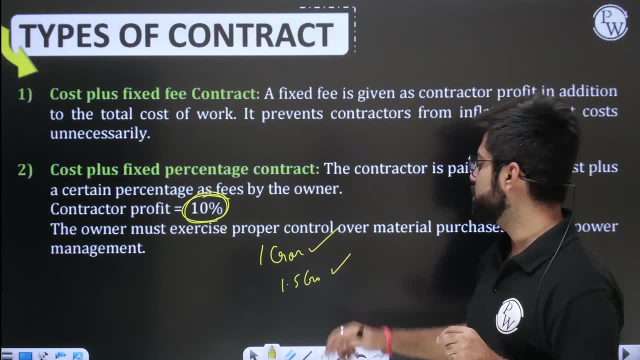 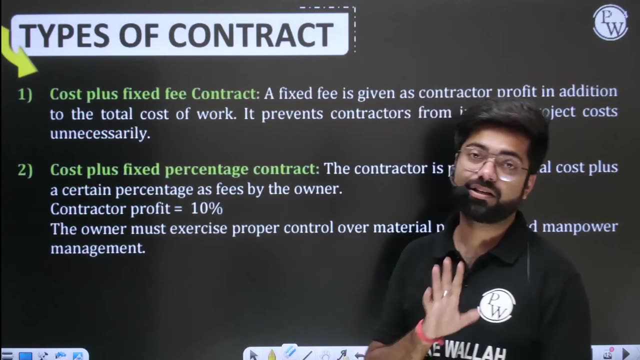 obviously he will not do the work in a million. he will try to do it in a million and a half so that he gets 10%. now, 10% is less of a million and a million is more of a million. then when, When we work on a fixed percentage, then the contractor puts his mind, but the owner has to be very active in it. 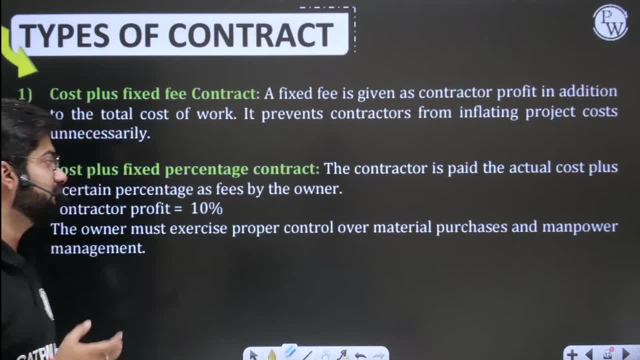 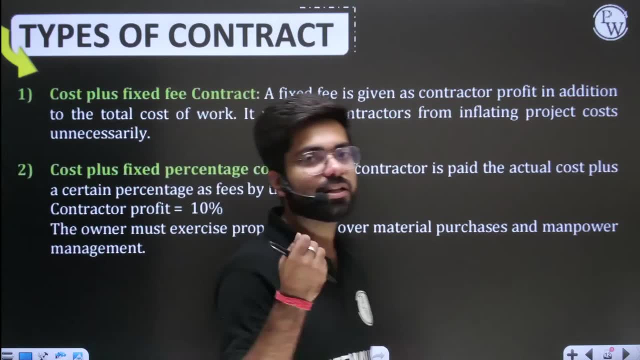 The owner has to see that the stuff is being kept properly or not. When the material is being purchased, then there is no up and down in it. The management of manpower is going on properly or not. I don't know if I have put anything in the bill. 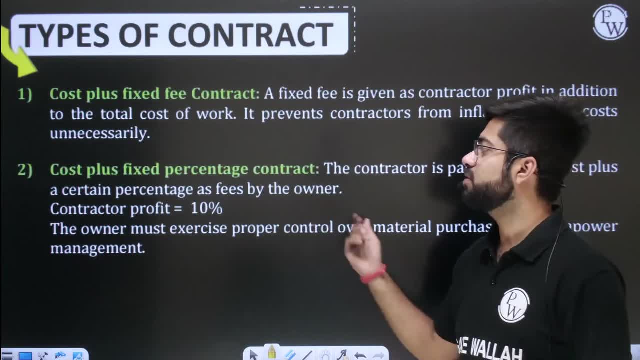 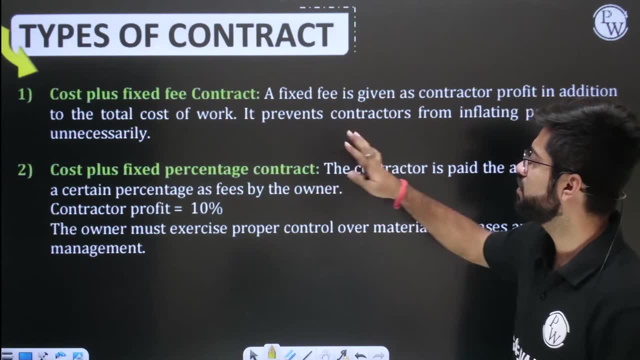 Because the total has to be increased. If the total increases, then the percentage will increase. There is a little load in this, But this generally works in big works. This works in small and big works. This is generally referred in small works. 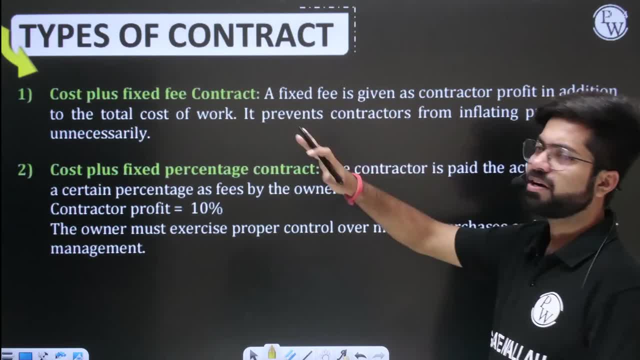 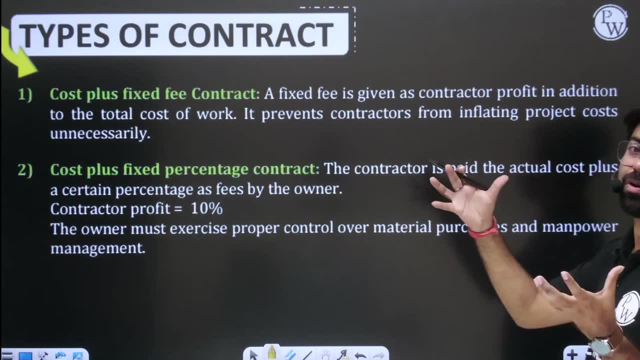 So the total fixed fee is given And in this the contractor does not try to increase the expenses. The contractor prevents from inflating project cost Generally he does not try to increase the project cost in the first one. Did you understand, or not? 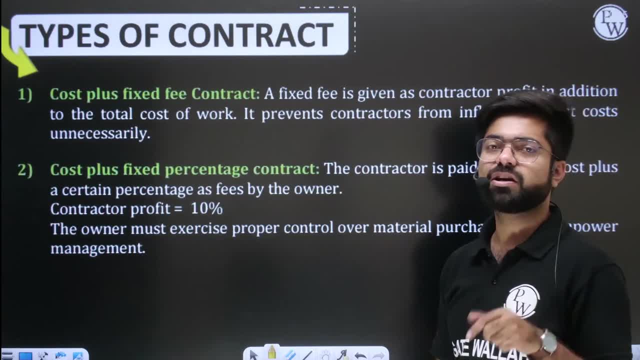 It is very basic. It costs 1 crore rupees. you will get 10,000 rupees. So 1 crore or 1.5 crore, it does not matter. So he is trying to finish it quickly. Right, Take this much money and get out. 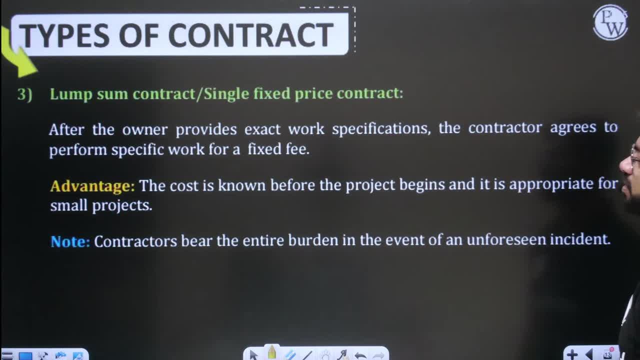 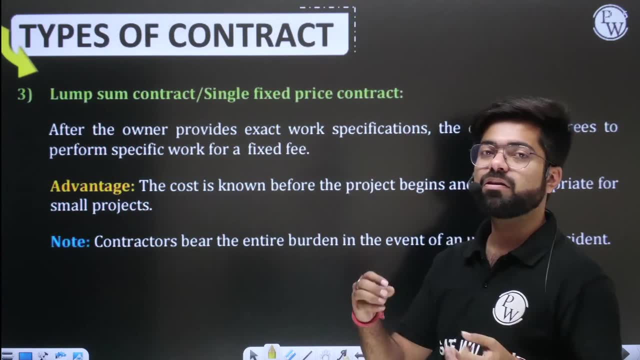 Then comes the lump sum contract, Single fixed price contract. Right, Like you are giving a rent, You must know the rent. You have to make a room or do something You have given the rent. The rent is said to take this much money. 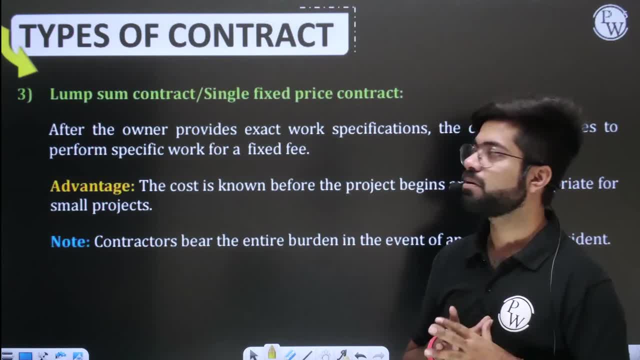 Your headache is with us. We will come to the end. We will see. The matter is over, Right. What did you say? in the lump sum, A single fixed price is given. The owner provides. What does the owner do in the beginning? 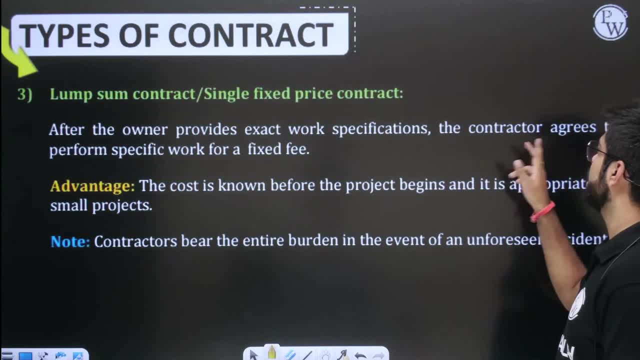 We told you that the work is given to him with such and such exact work specifications, And the contractor agreed that we will do this work. Just give us this much money. How will the material come? How will the labor come? That is our responsibility. 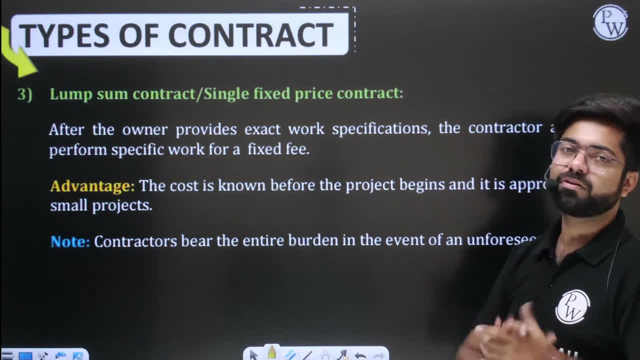 Now you do not take the load, Be happy, We will meet you after 7 days. We will meet you after 7 days. We will show you Okay Quality. I want to go to Biju and see. There is no problem. 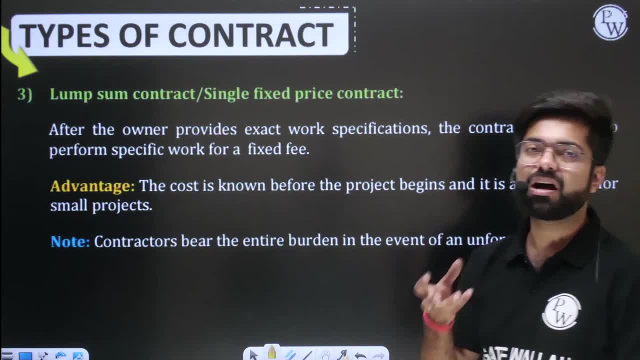 It is not that you have to meet after 7 days. Now what is the advantage? Generally, the small and big work that happens- it is beneficial to give a rent. There are small and big works. It is beneficial to give a rent. 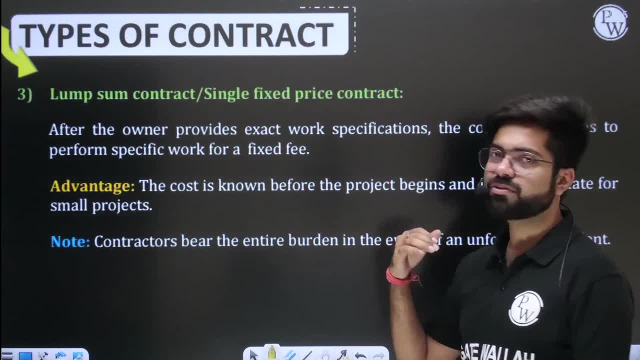 In Hindi it is called to give a rent. This is your lump sum contract. Okay, This is your lump sum contract. So what is the advantage in this? Cost is known before the project. Work is known before the project. We know that this work will be done in 20,000.. 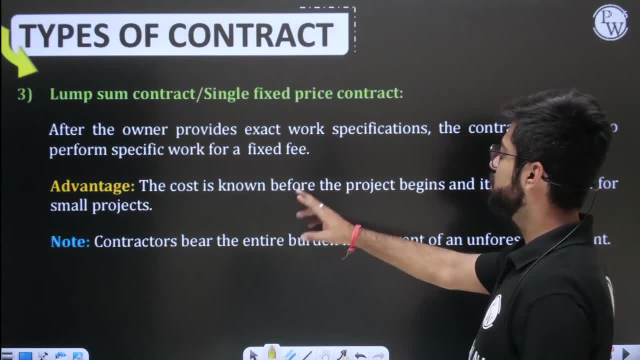 Good, 25,000 will not be able to do this work. It will take a week. Okay, Good, I know everything. We have already gained full knowledge. Okay, Even if we do the end-to-end work in the market, it will still cost more than 1000 rupees. 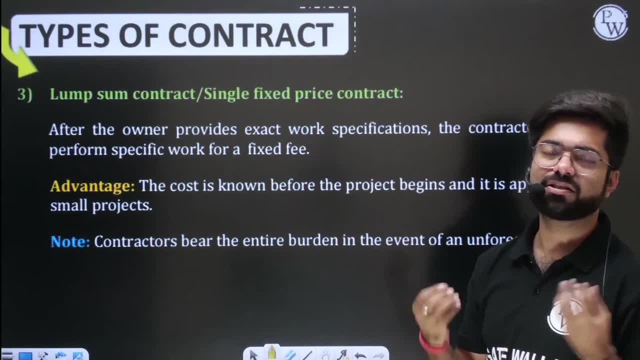 But all the tension is over. All the tension is over. In the middle, the labor is running. this is happening, that is happening. All the responsibility is of him. He will manage, Okay. That's why it will take a little more than 1000 rupees. 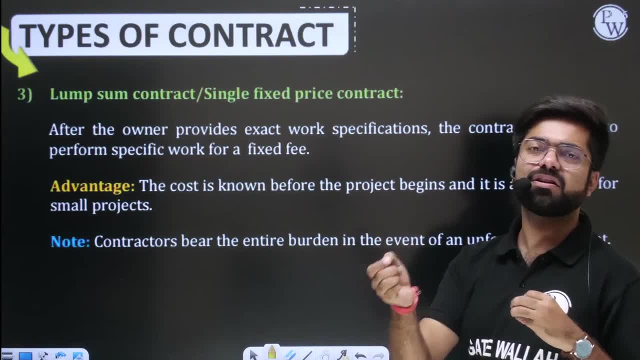 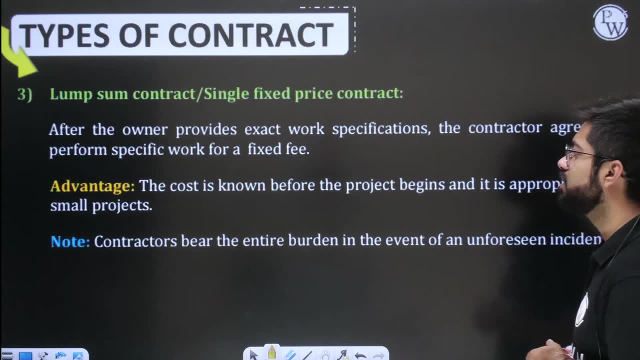 Okay, So this is your lump sum contract. So what is the advantage? Cost is known before the project. We know that this work will be done in 20,000.. It is beneficial to give a rent, So we are aware of the cost in the beginning. 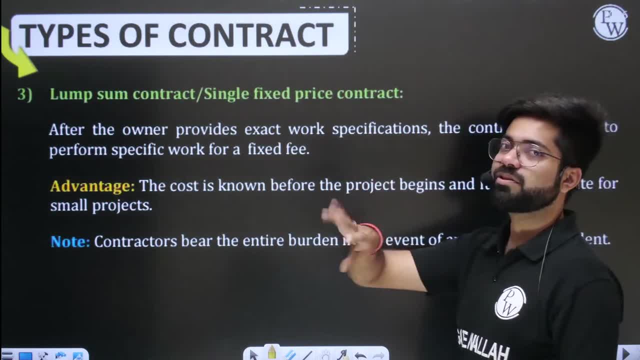 And generally he prefers it for small works. So the special thing here is that the note is written here. The special thing here is that all the responsibility is on the contractor. If there is any high or anything unforeseen, then the entire contract will come on the. 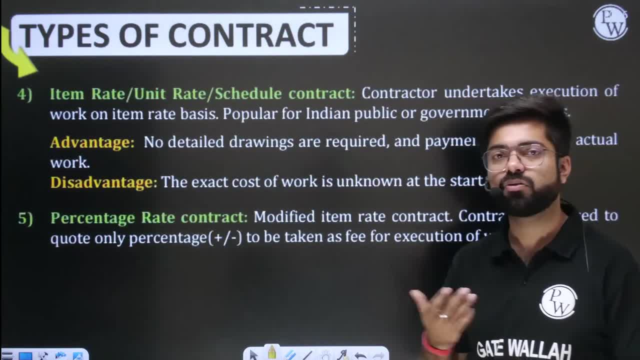 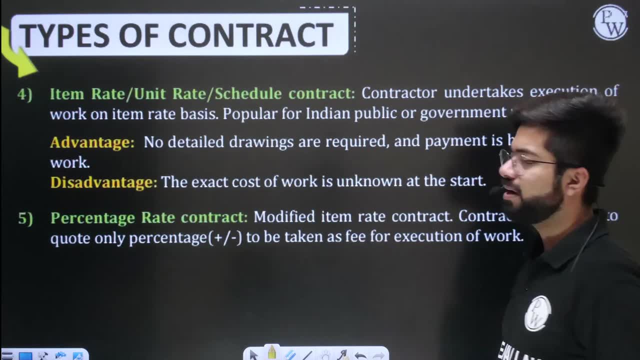 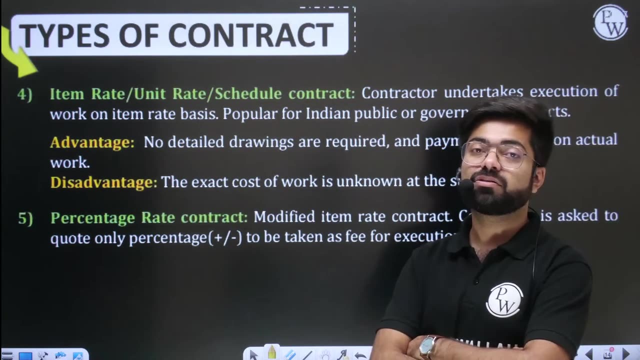 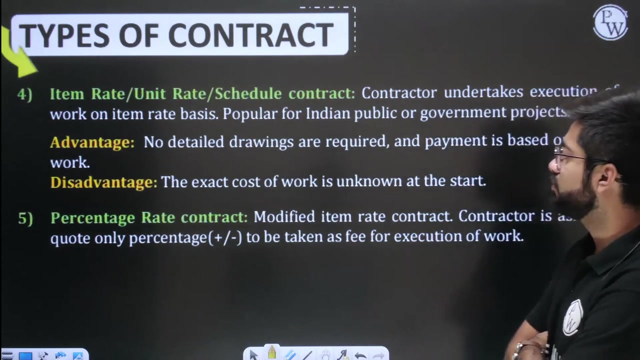 contractor. Okay, Except for the act of god. We cannot do anything in the act of god, But all the responsibility comes on the contractor in the lump sum. So a little bit of money is a little more expensive, A little. Now. if you will make them work on a daily basis, then you will see where the money will go. and if they give you this, then the same work will be done in three days. they will do everything in three days. then it makes a difference. 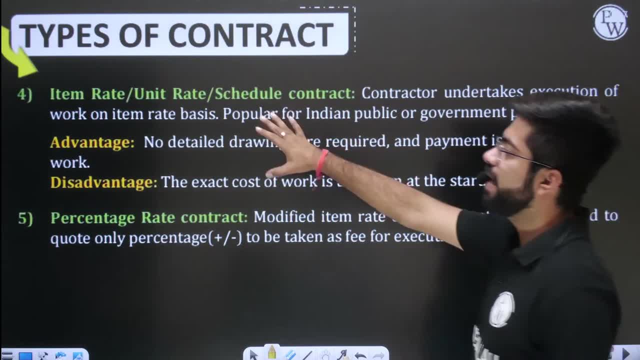 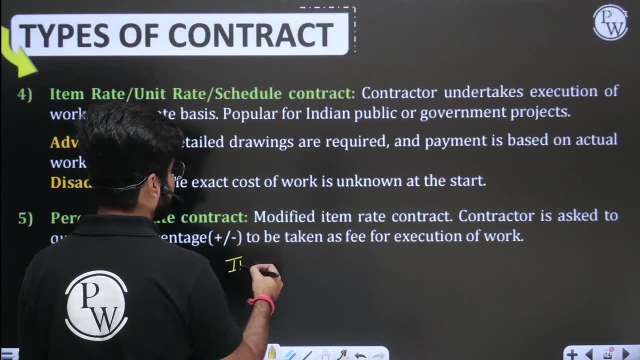 Then there is item rate: unit rate schedule contract. What happens in this? In the tender form, when people download the form and fill it completely, there is an item written in it. What happens in the item rate is that you specify all the items right. 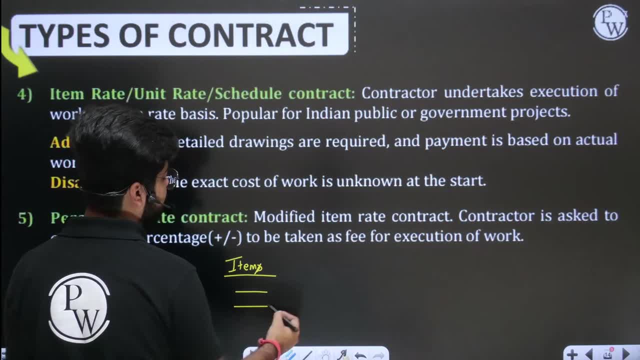 All the items are written here. here it is written that there is earthwork. every work is specified here. Now the rate remains empty in front of it. So how much is this rate At the rate? of all this will be filled by the contractor. all this will be filled by the contractor. 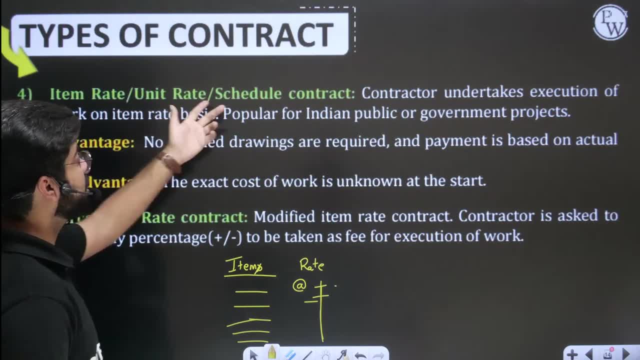 So item rate unit rate is also called unit rate contract or schedule contract. So all this will be filled by the contractor. All this will be filled by the contractor. So all this will be filled by the contractor. All the items are written here. who will fill all their rates? Contractor. 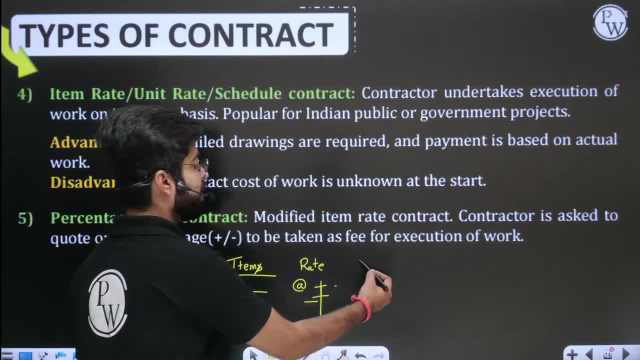 That we will provide this much. Then here the number is written. Now the item is this: this number is suppose it is 5, and one thing is of 10 rupees. then 5 x 10 is 50 rupees. 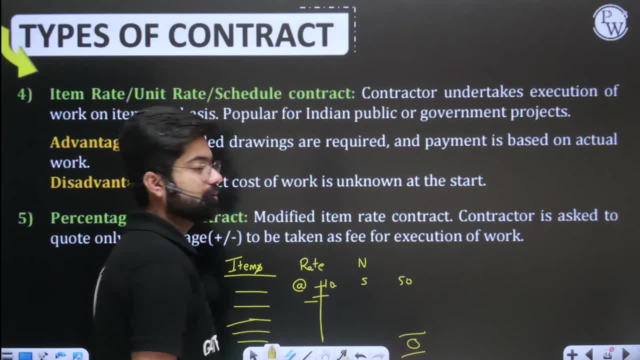 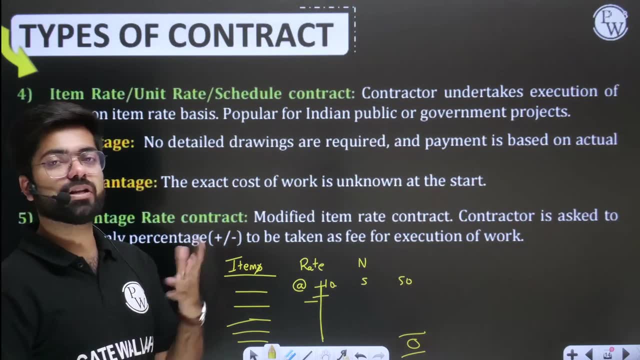 In this way, we get to know the final price. by combining them, We get to know the final price. okay, In this we did not tell any price in the beginning. We did not tell in the form in the beginning that this work should be done in this amount or something, nothing like that. 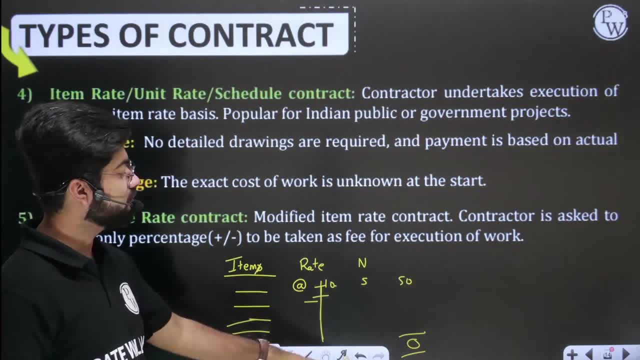 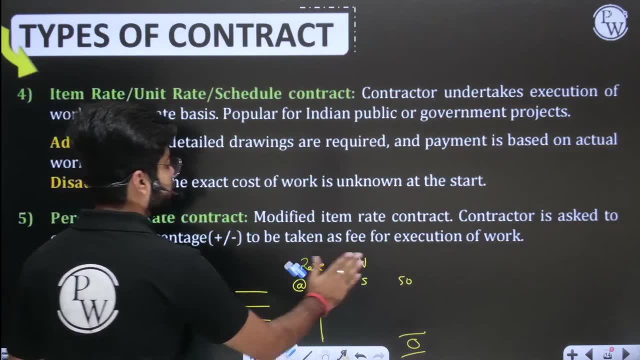 The contractor himself is telling everything, that there is one item. he has filled all the rates. He will fill all the rates with his whole pencil, He will write the number, he will multiply everything and tell the total. okay, And then, if we like it, okay. 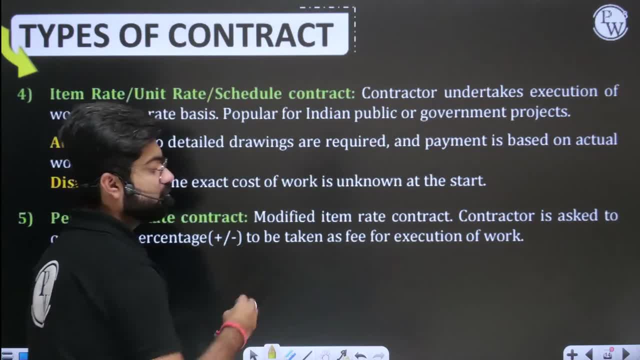 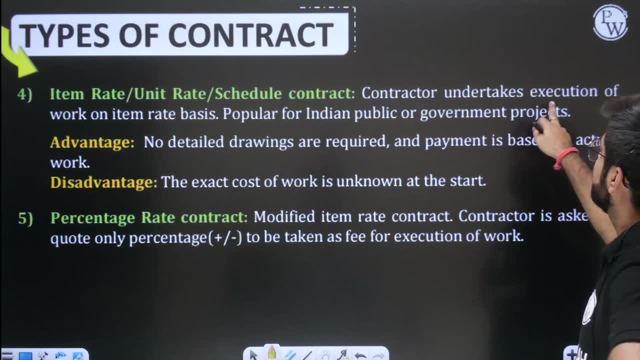 Suppose the total price that came out here. suppose the total price that came out here. we like it. okay, We will tell him to come, come from tomorrow, meet okay. So what is in this? Contractor undertakes execution of work on item rate basis. 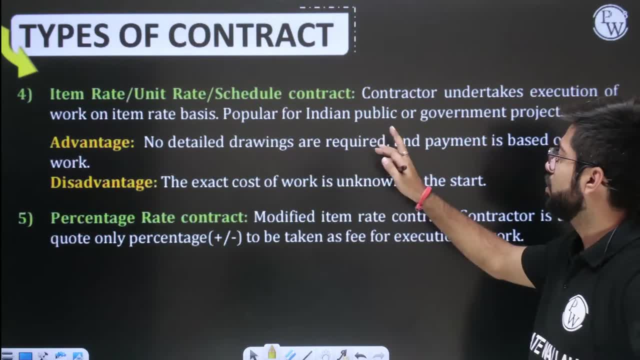 He writes the rate of each item himself. okay And popular. for Indian yes means the government projects in which the item rate contract is done. It is generally done okay. So now the client, who is our engineer: he completes all the calculations and estimations with JEE. 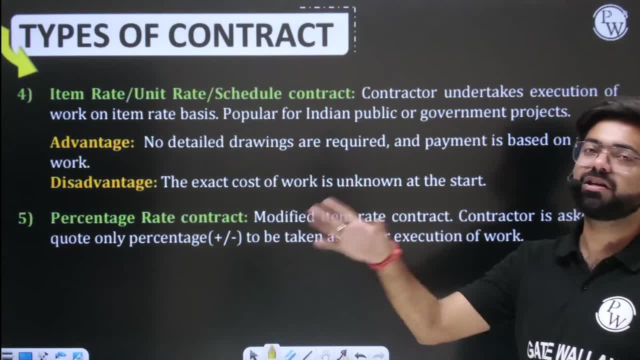 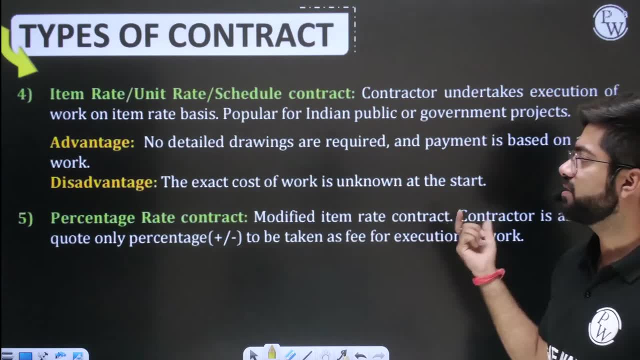 He completes the entire estimation with JEE That in this canal there is so much soil, so much soil and this and that That is whatever work is there. there is so much profit in it. So the whole list is ready And how much work is to be done for each item, a complete estimate is ready. 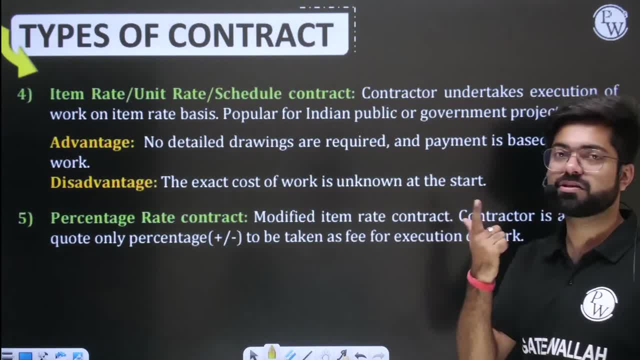 It just has to be filled in all places And the contractor who will fill it cheaply will tell him to come, Okay, Okay, what is the advantage in this? There is no detailed drawing and all these things are necessary. Payment is simple. 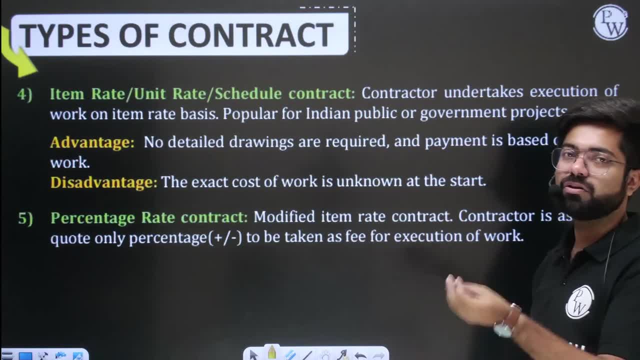 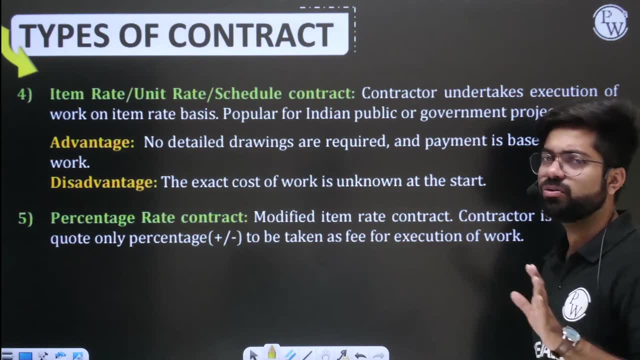 It is based on actual work, That these things have been written, these items, This work has to be done and how much money they have to take. That's it, Okay, but the exact cost of work is unknown in the beginning. Okay, we have an estimate. 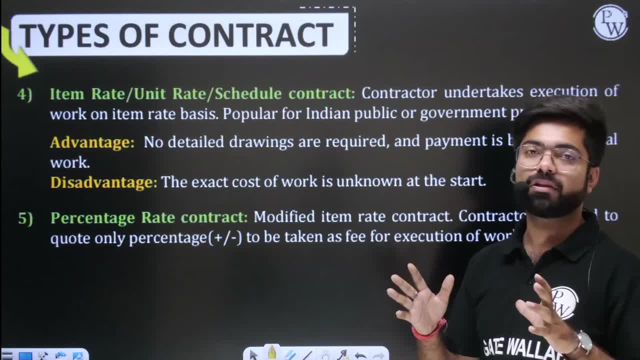 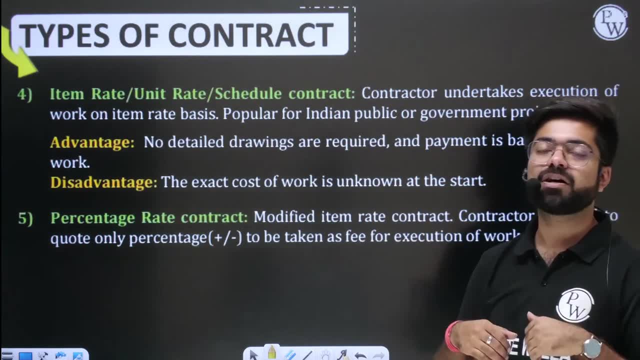 Obviously we have an estimate Now. look, we don't know, In the starting we just filled the form empty. Now, if they fill it, then it will come to us. When it will come to us, there will be changes in it as well. 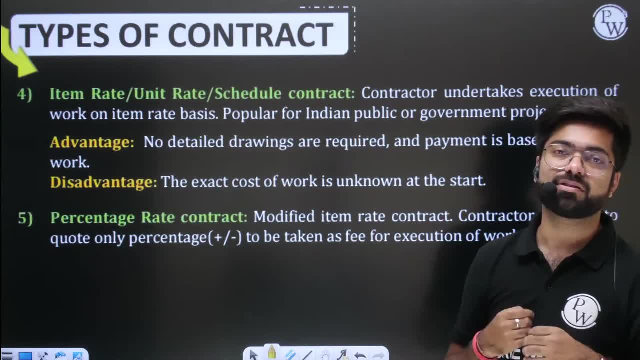 So in the starting, we don't know what they will fill. Someone can fill more, someone can fill less. Okay, Although we have an idea, That's a different thing, But the exact cost is not known in the starting, Because they will fill the form. 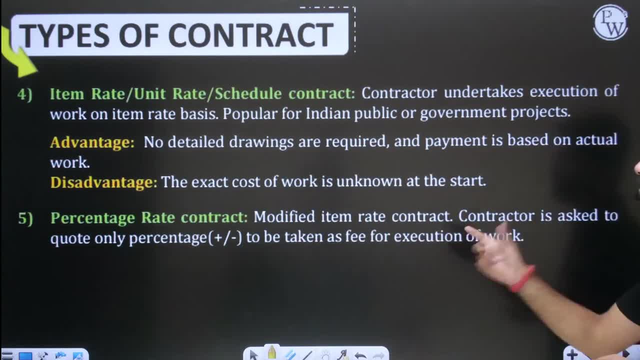 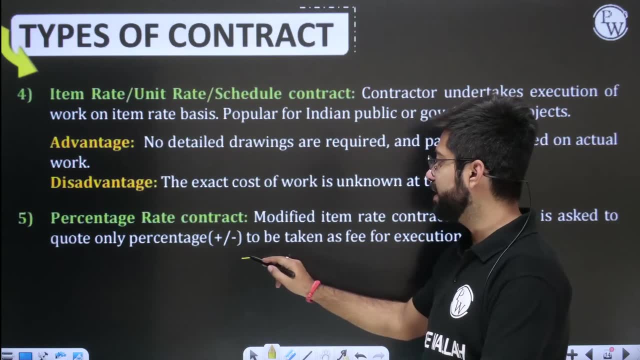 When they open the tender. then things will be known. Okay. Then comes the percentage rate contract. This is your item rate In that. only it has a modified version. Now what happens in the percentage rate contract? That every item that is written. 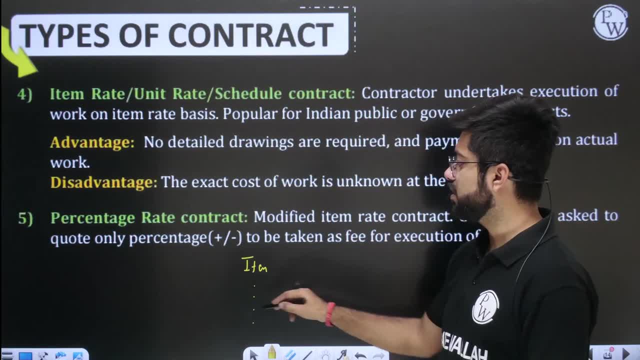 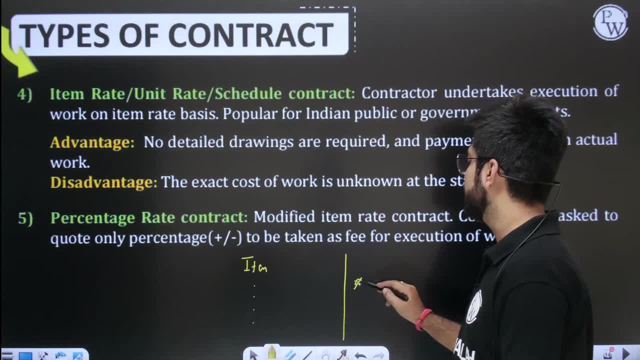 This work has to be done. This work has to be done In this north port. we will take 10 percent At the rate of 10 percent profit In this work. we will take 5 percent profit. So in every individual work, 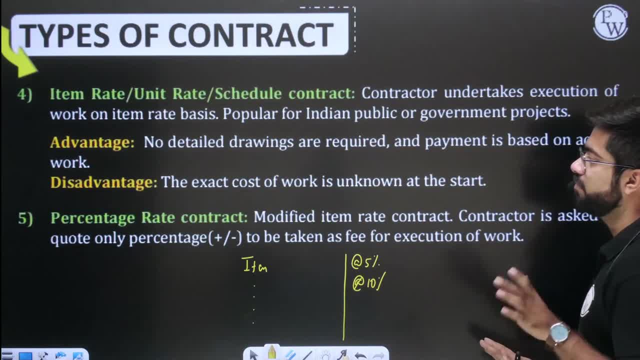 It writes its own profit here. Okay, Just understand. It's written here that modified item 나도 under contract, Only percentage to be taken for execution of work. Write your percentage forward in each work, What you want in this. This is called a percentage rate contract. 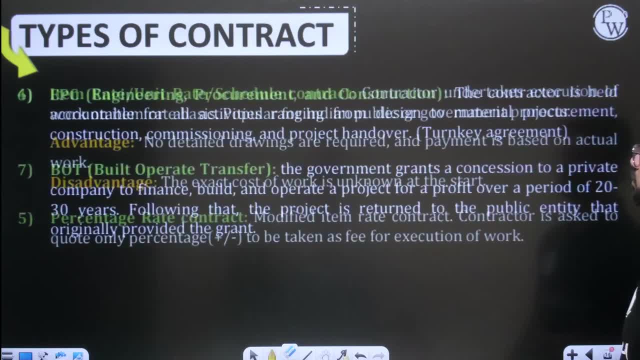 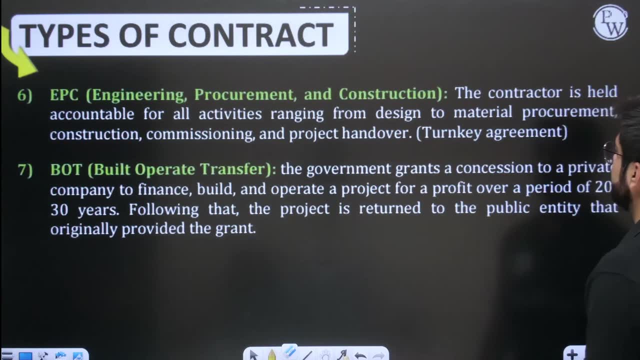 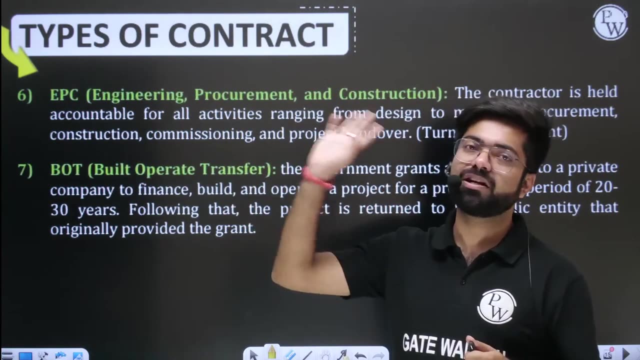 Okay, De chilly orang pegar. Modified version: demand rate Correct Engineering Procurement and Construction. Contractor is held accountable for all activities, ranging from design to material procurement. construction Means: in total, everything has to be done by the contractor. If you get the work done, you tell the contractor to build the building. we will come and see after 3-4 months how the building will be built. 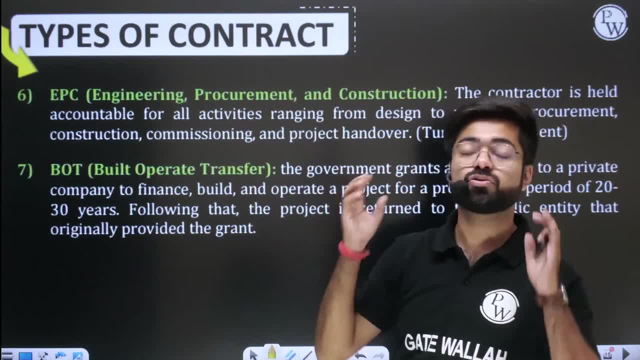 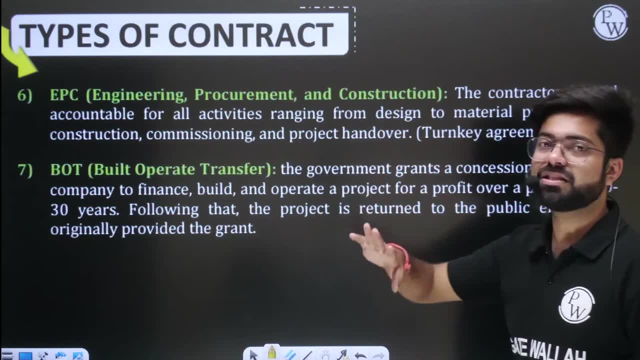 So whatever engineering, design, new thinking or procurement has to be done in this, material has to be procured, land has to be taken, anything has to be done. You do construction. when everything is done, then we will come to cut peat. 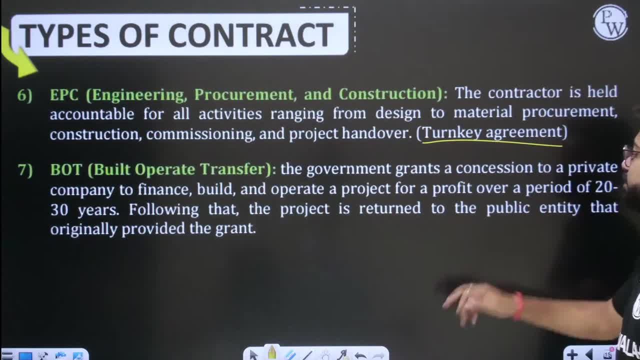 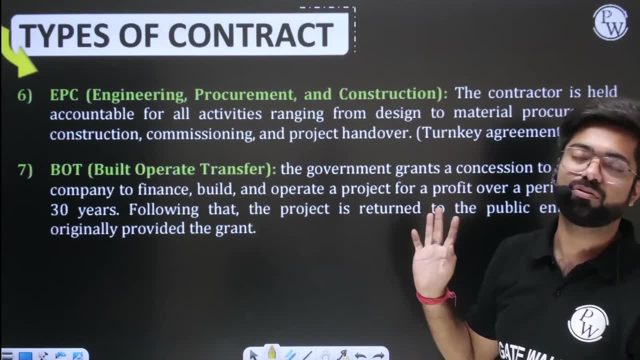 We will come to cut peat. then it is called turnkey agreement. Turnkey means when the building is completely ready, then we will come to turn the key. in the end. We will come to turn the key in the end. you will see the whole work yourself. 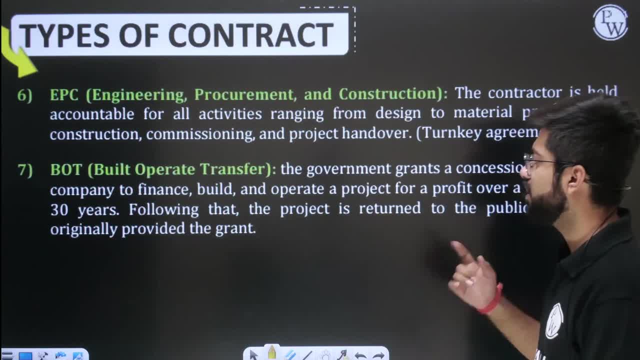 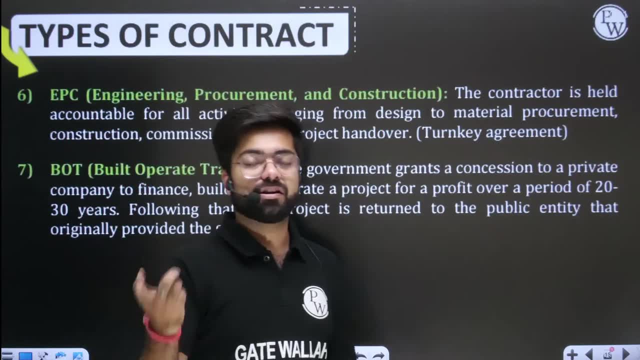 So this is the EPC contract. It is very famous. it should also be known. Rest BOT is going on a lot these days. What is happening these days is that you must have heard of Triple P, Public Private Partnership. These days, as you have seen, the airport of Lucknow has been given to Adani ji. 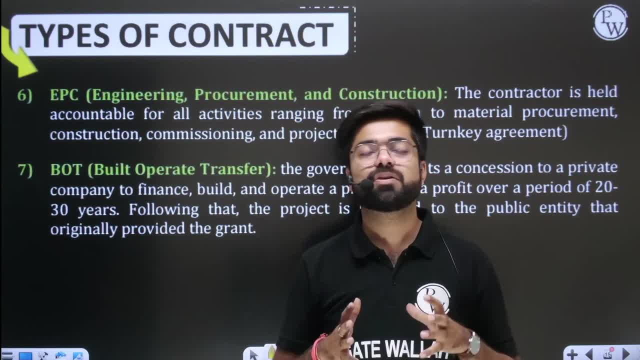 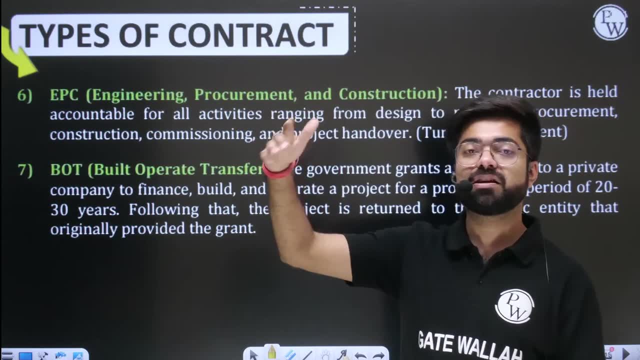 Do you know or not? So what is in the public-private partnership? suppose a road is being built. So suppose the government- the government has to see the development of the country- And the private players, Adani, Ambani, all these people are seeing the benefits. 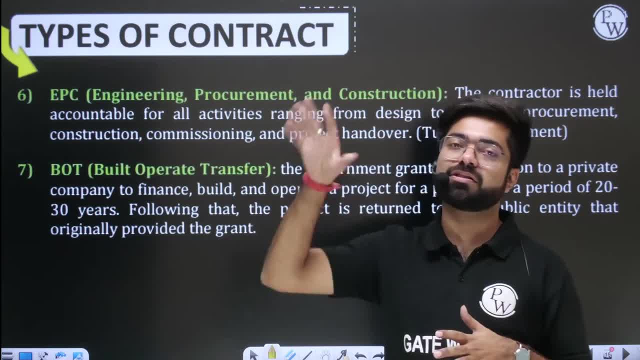 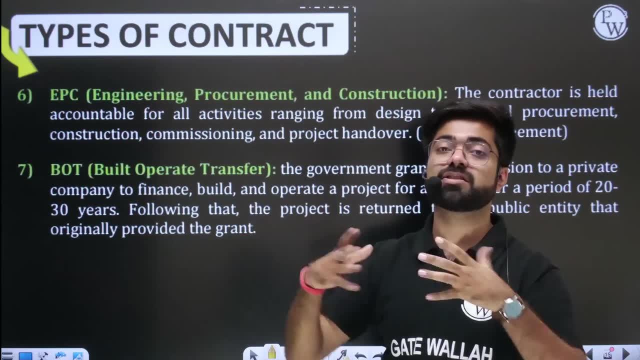 So tell Adani Ambani to do this. you make a road with your money. do everything yourself. Then make a good road. you are the owner of it. we will give you the land on lease. We will give you the land on lease. the government is saying: we will give you on lease. 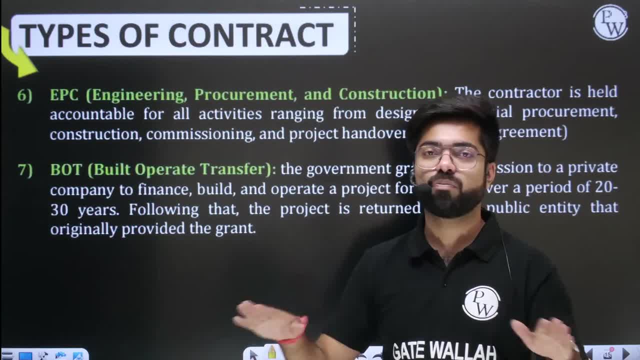 How many years will you say? 30 years, 40 years? You make a road, put toll tax there And a lot of money. You make a lot of money. There is no problem, Just go take out your money. 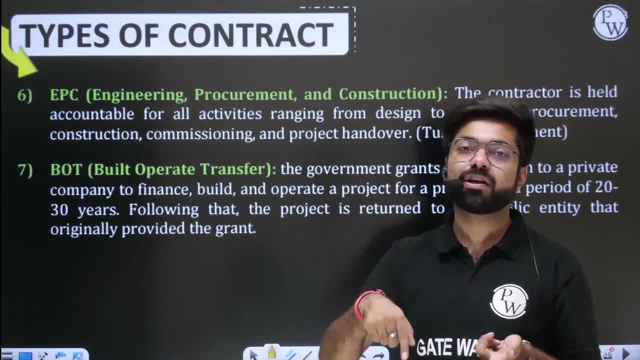 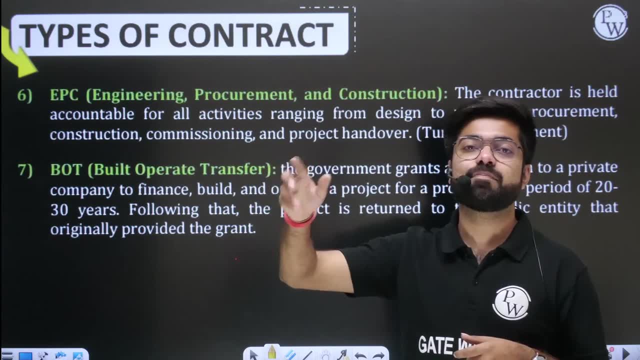 So what is the benefit? The public is happy because the road has been built. they are getting speed. the expressway has been built, As it is happening in UP Now. our airport is being built very well Now, but since Adani ji has come here, the parking is going very high. 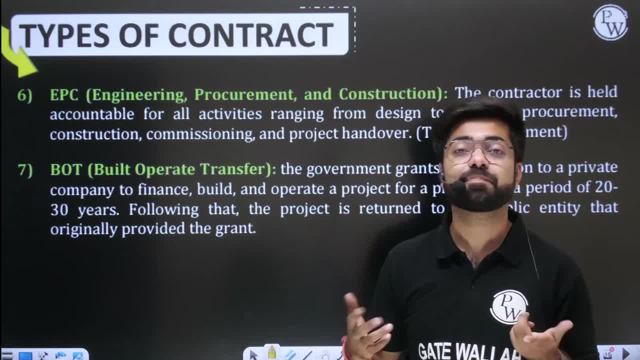 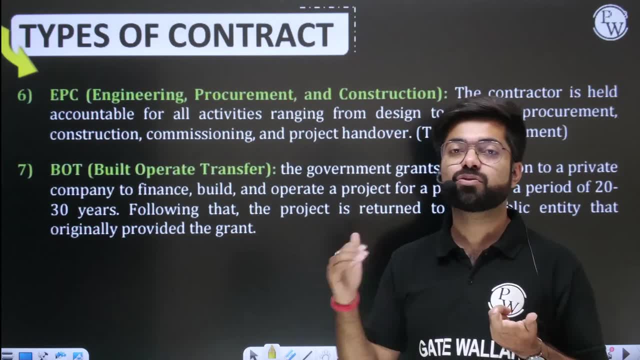 Because they can make money from their own mind. Why are they doing toll tax? Why are they investing money in parking? Because when they are developing it, they will collect the money that they have invested. They will collect. take a little profit. 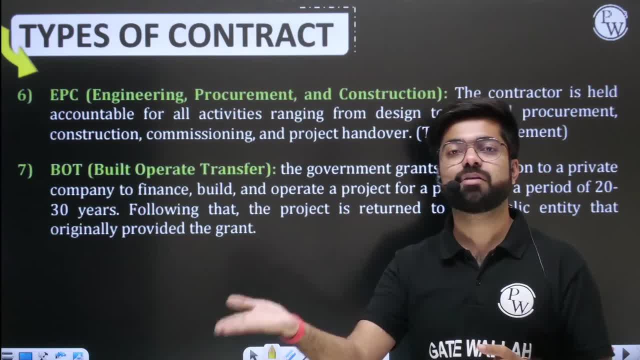 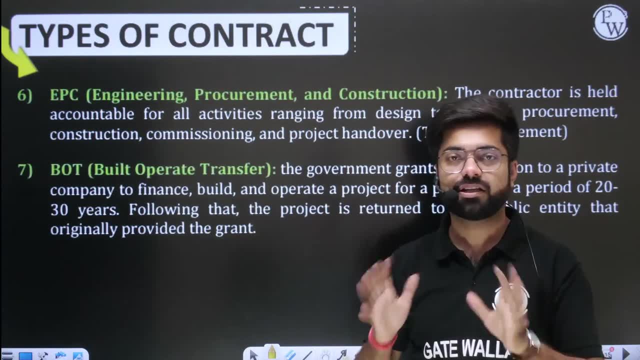 After that, when their cost will come out, then they will give the airport or road back to the government. So they built first. First, they built first, they prepared the infrastructure, Road, airport. they can do anything. They are big people, they have millions of rupees. 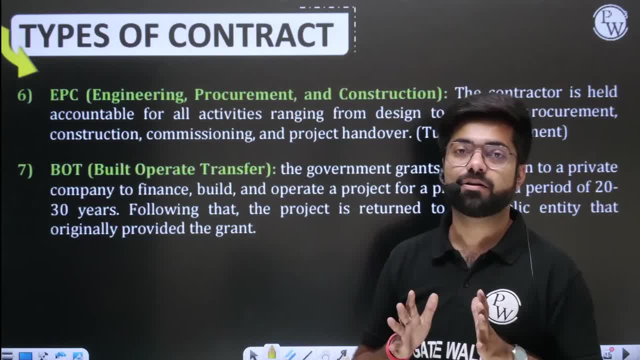 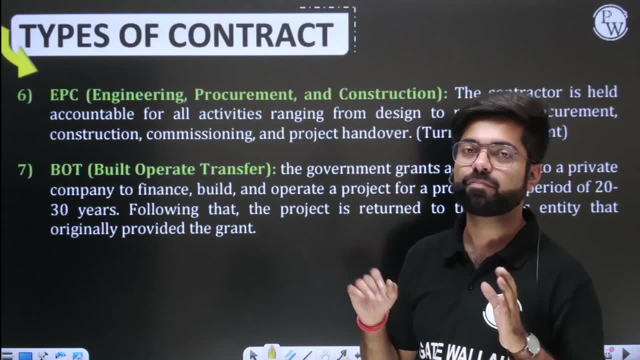 They have built it. After that. they drove it, operated it, maintained it, collected toll tax. The money started to be collected. They are operating. They took all the money And when they collected toll tax for 20 years, 30 years, 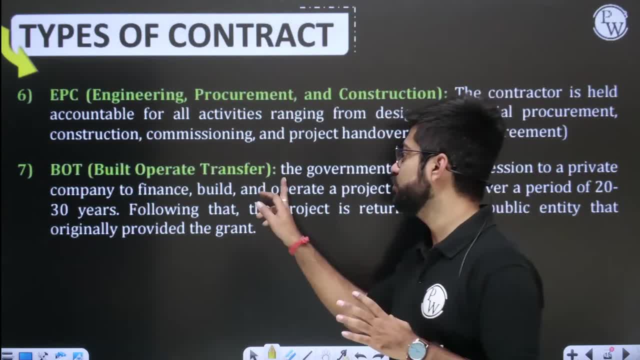 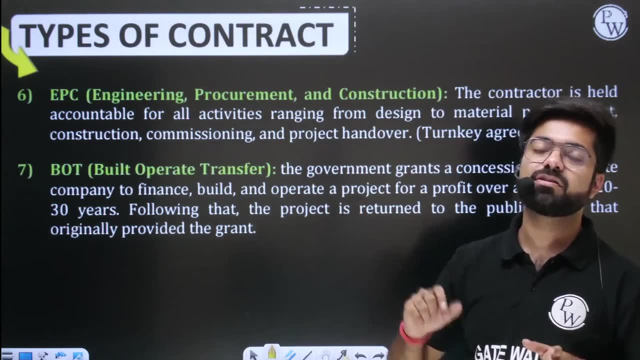 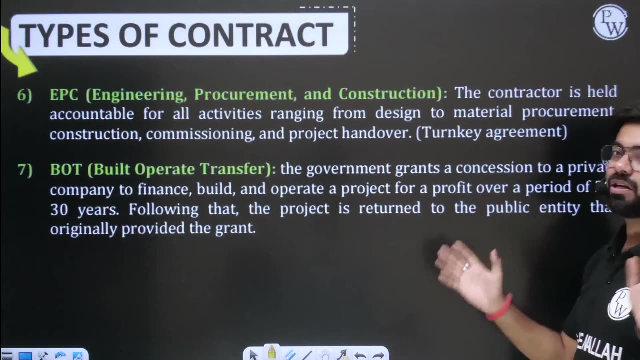 And they came out with a profit of a whole crore rupees. Then that whole property will be transferred to the government. This is called working in public-private partnership. Private individuals, private financial institutions and our public work together here. So first operate the build, run it and transfer it at the end. 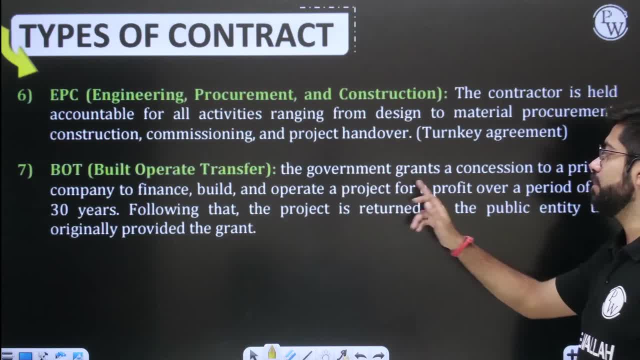 So government grants a concession to a private company to finance, build, operate a project for a profit over a period of 20 or 30 years. Take out your profit for 20 years and then return it. Okay, Return the project to the public entity. 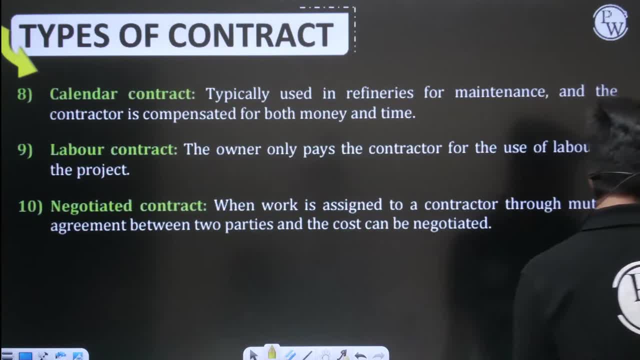 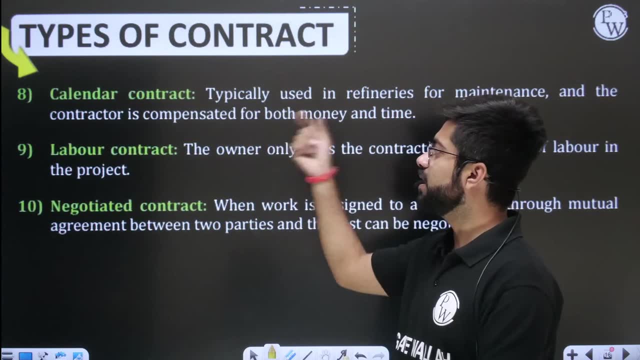 Got it, Return it to the government. It is a very basic thing. It is also very popular these days. You must have seen it. Okay, It is clear. It is very simple, Very basic. Then comes the calendar contract, Typically used in refineries. 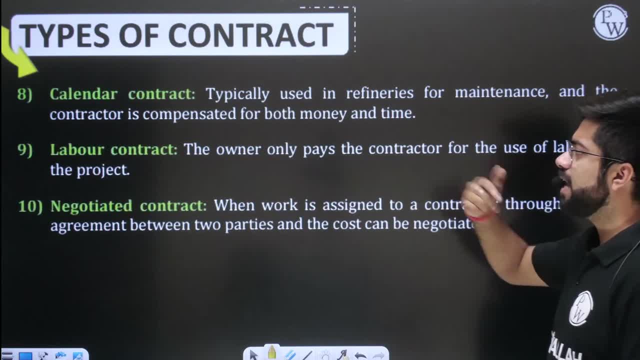 Now, what is the calendar contract? It should be done from time to time Maintenance, like annual repairs Maintenance. So this is a maintenance type contract. Okay, On the basis of calendar, that it has to be cleaned every 6 months, Whatever that kind of thing is. 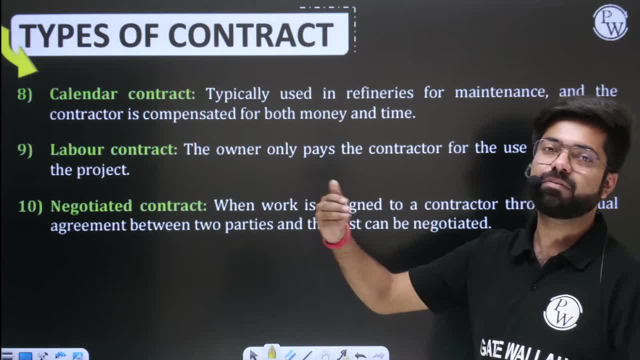 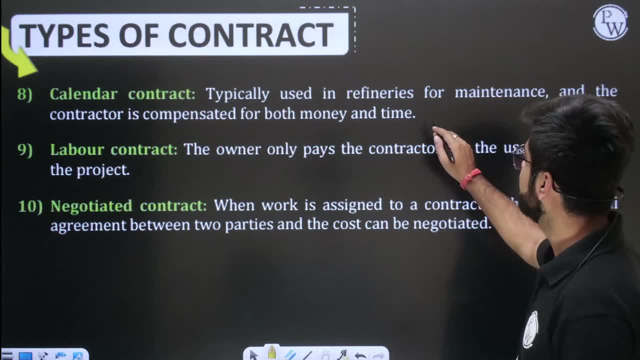 Not money. Like refineries, have a lot of maintenance. You know that refineries are oil refineries, So there is a lot of maintenance work in it. So the contractor, Whatever material is being applied to, the contractor, Not money. Money is obviously to be obtained at the end. 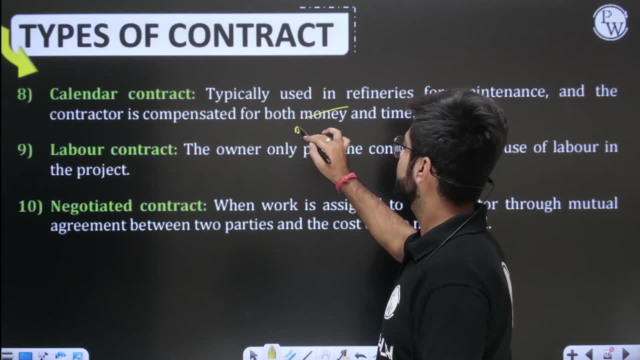 So whatever material and time it takes, it is compensated for. that It is done. Calendar contract: that every 6 months come here and work, Do maintenance, Clean the refinery- Okay, Because dirt gets stuck here and everything Blockage. So it is done. 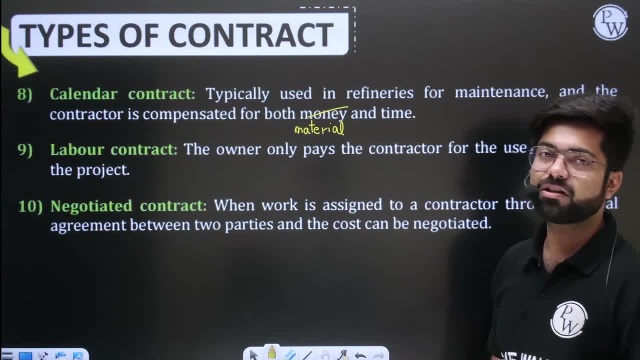 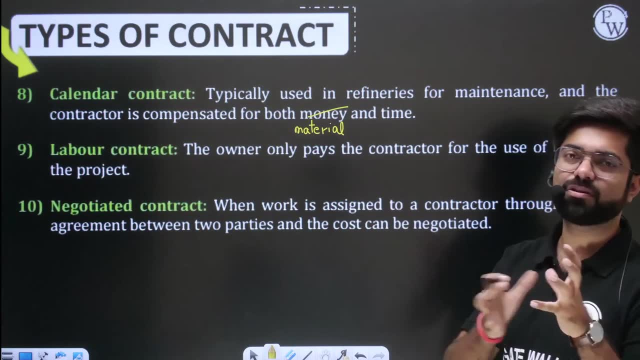 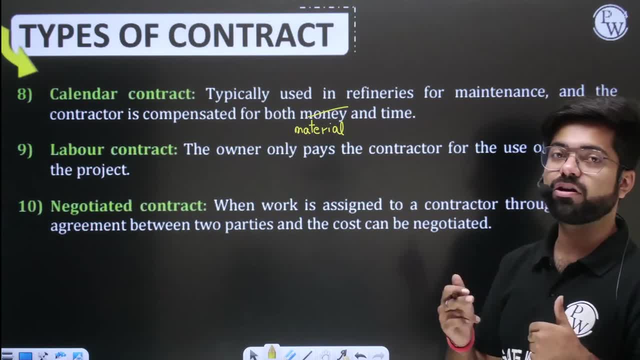 Okay, Because dirt gets stuck here and everything Blockage is done, So you have to fix it time to time. So it is called a calendar contract In which you don't have to do any work continuously. You have to come at every moment. 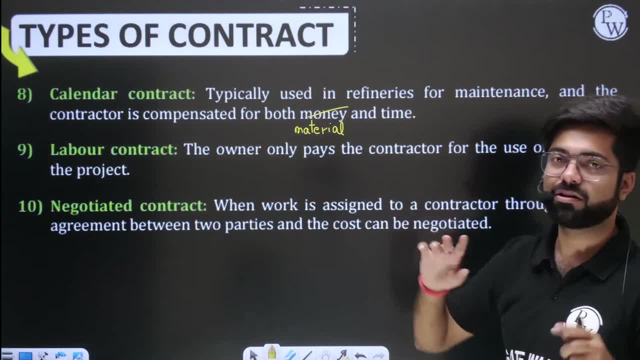 Repair the grant. You have to come at every moment and maintain. This is called a calendar contract. Okay, So we will do the setting with an contractor. Like we have a house in the room, What happens in it? The work, like every 6 months in one year, repairs it. 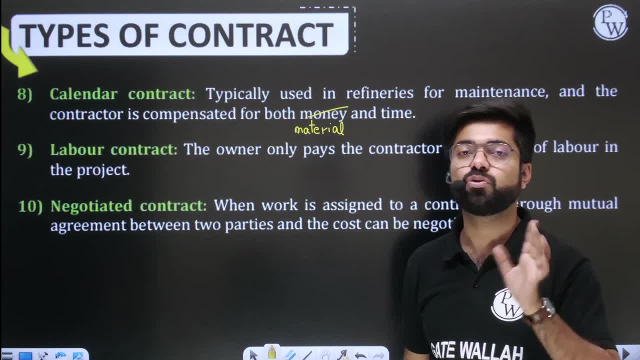 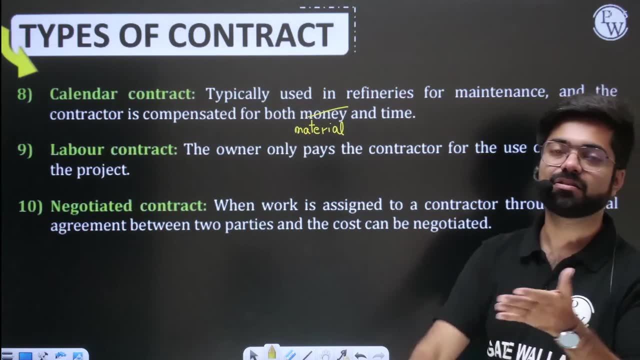 That happened. The work like every 6 months in one year. The work like every 6 months in one year. It is done. Service does not happen. We have a calendar contract. We have signed an agreement with RO. You keep coming here and clean the filter in 4-4 months. 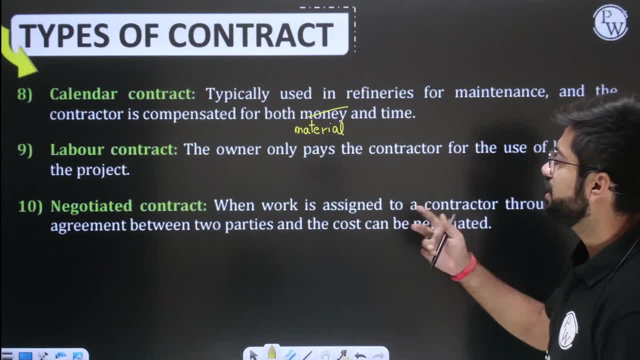 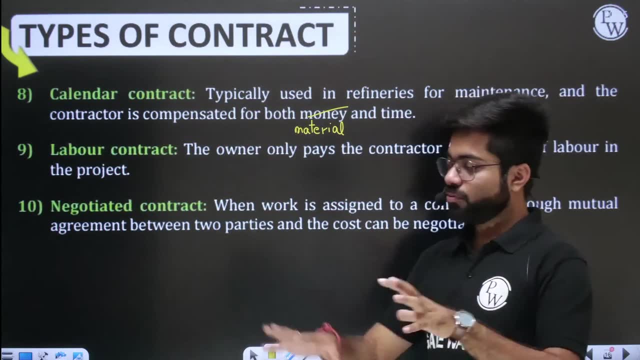 Then labor contract. Now you can understand by name: Owner only pays the contractor for the use of labor in the project. If you have everything in the house, you have kept everything in the house. you have called only labor. like you have ordered paint and everything and said that: 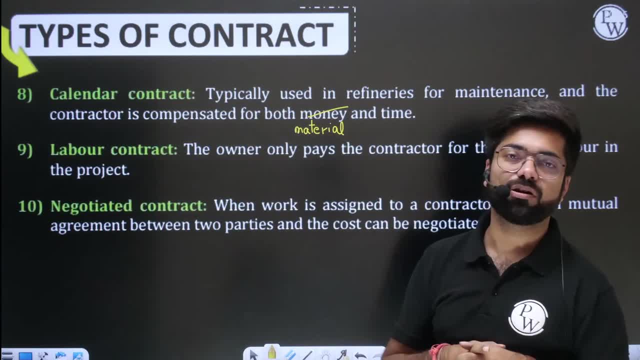 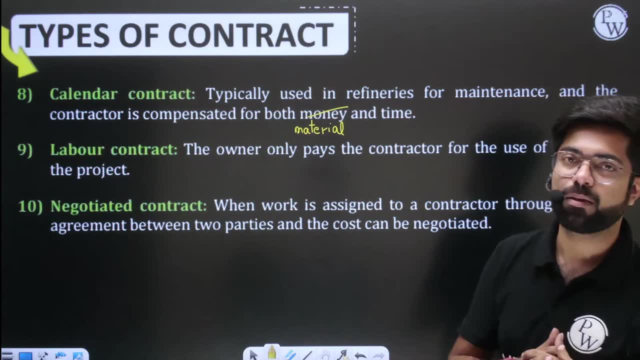 you take 500 rupees and quickly paint the whole room in a day. So which contract is this? Labor contract In which only the work of manpower is being used. the money is being given. We already have the rest of the materials. 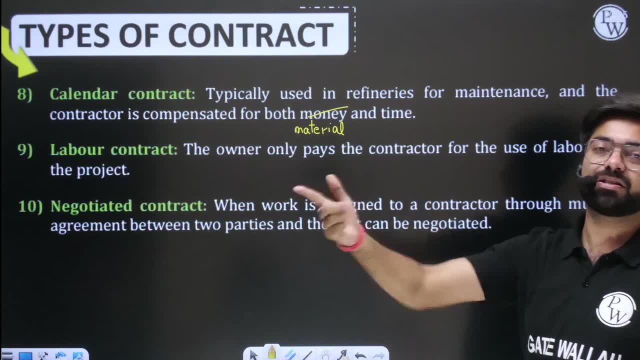 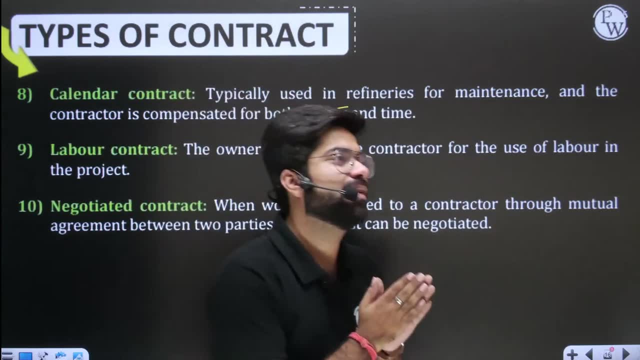 So the owner, the client, only gives labor money. Okay, This is what we have told you. Negotiated contract. is such a contract, Brother? please agree. Please agree for 100 rupees. Why are you taking 105 rupees? 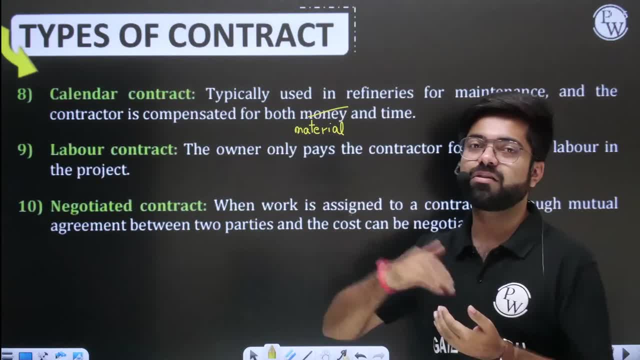 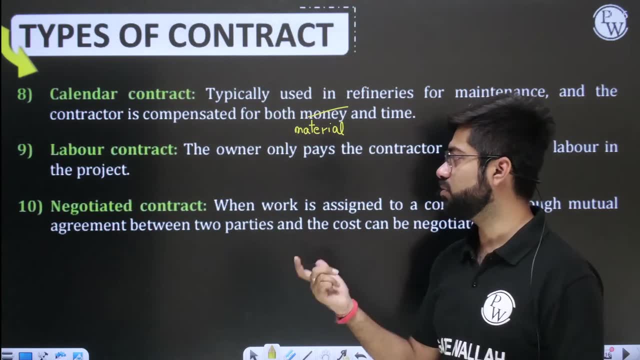 This is negotiated, Negotiated means between the owner and the contractor. negotiation is going on. Assume that you make it cheaper. He says no, we will take only this much. So this negotiation is done When work is assigned to a contractor through mutual agreement. 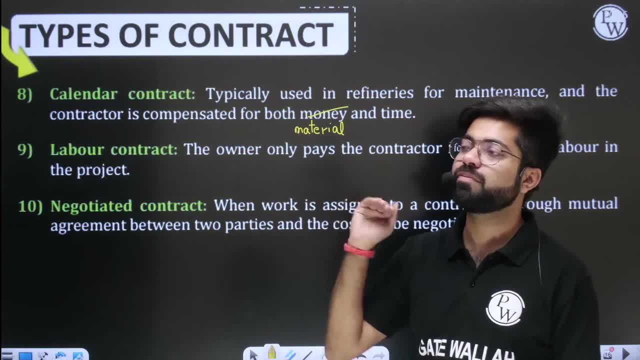 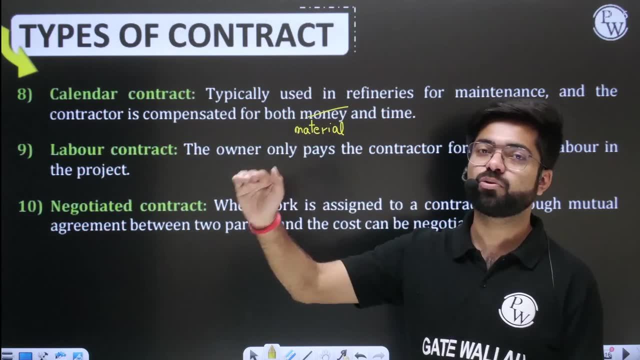 Negotiation is mainly done when the price or the budget we had allocated in our mind is getting all the contractors above that. Every man is working more expensively than him, So we have to negotiate with the cheapest one. Okay, Then we negotiate and negotiate the cost. 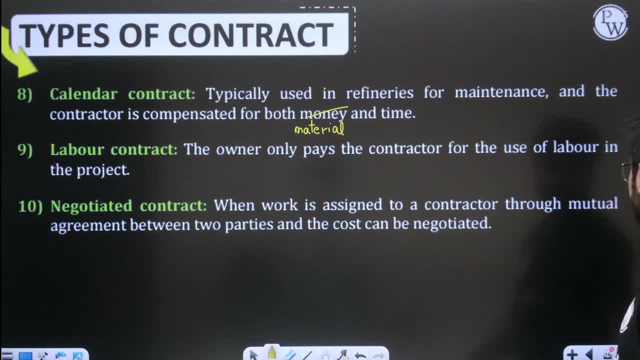 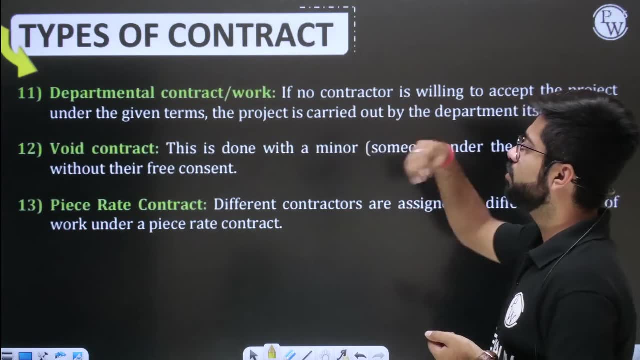 and set it in mutual understanding. Okay, So this is your negotiated contract, Very simple. Then departmental contract. Assume that there is no contractor And the department is working, Then it is a departmental contract Because the work is going on inside the house. 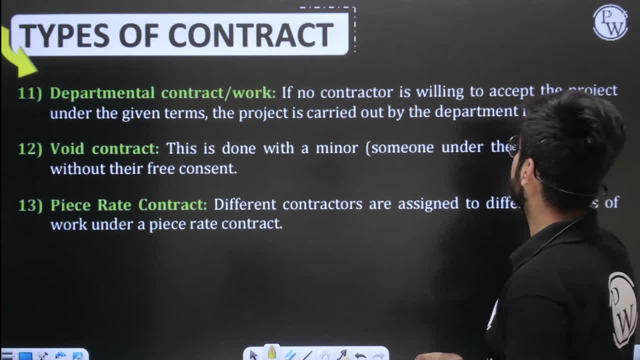 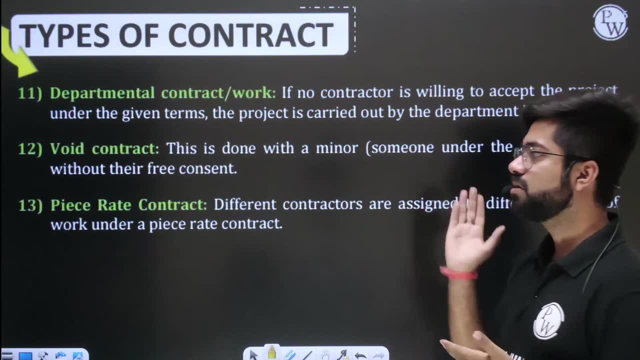 Very simple. It is a departmental contract. If no contractor agrees, then the department does the project itself. The department does it itself, Whichever department it is, whether it is a local department, local department- whoever it is, Then void contract. 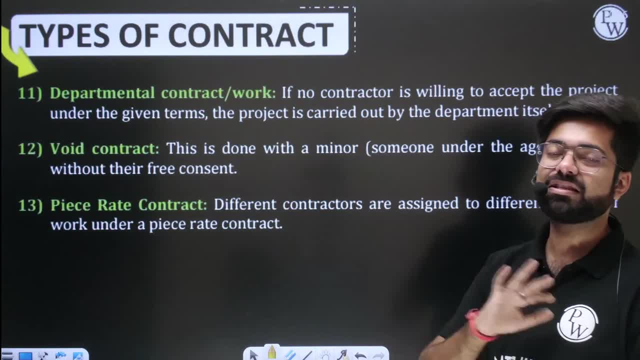 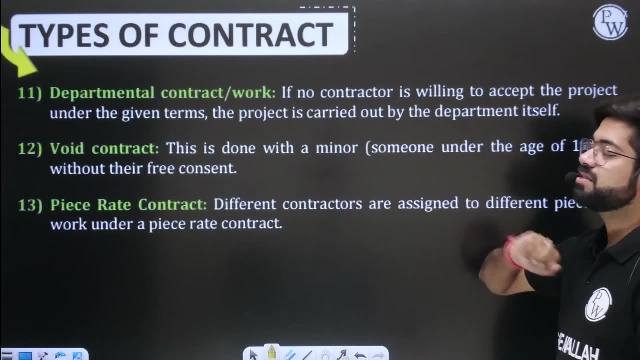 Now, what does void contract mean? That this contract is not worthy of anyone? If you have contracted with someone under the age of 18 years of age, Or you did not give him free consent, You got him to work on a gun. So if such contracts are caught later, 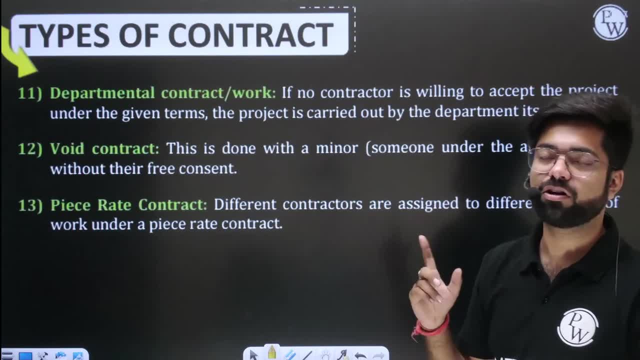 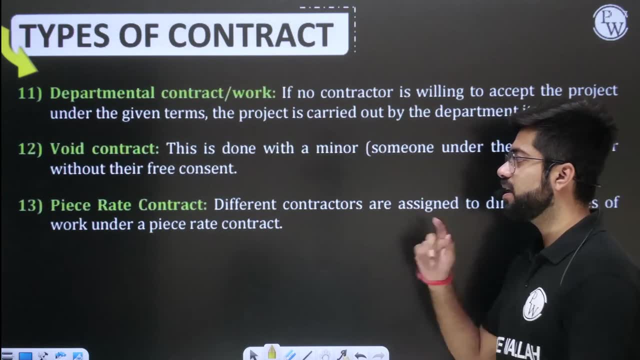 then that contract will be void anyway. So it is called void contract. It is null and void. No law will apply on it. It is all over from there. Okay, Then there is a peace rate contract. What is in it? This is the last one. 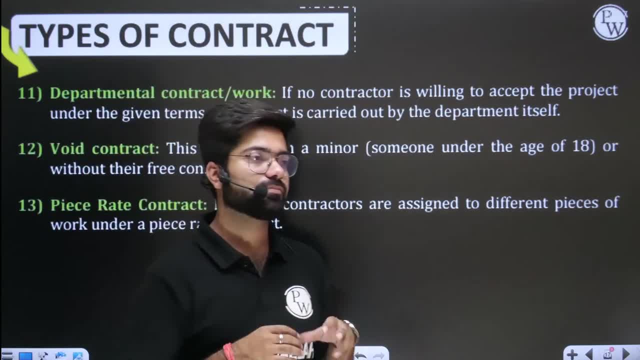 What is in a peace rate contract? What is in a peace rate contract, For example, you have to become a metro. Okay, You have to become a metro. Now there was a private company. Let's take the example of L&T. 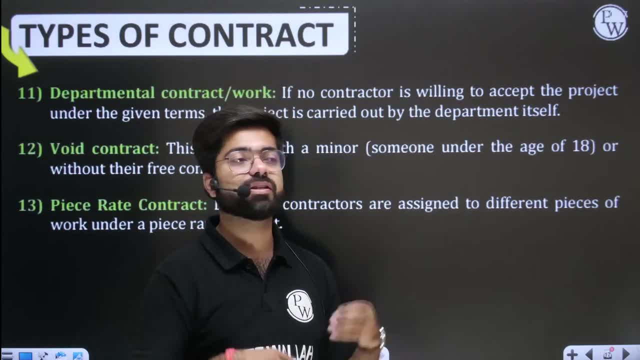 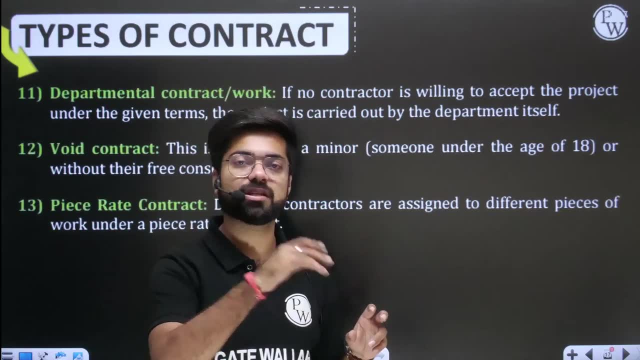 In that he caught a lot of small jobs for different contractors. He said it is like this: You go and make a foundation, Then you get out of here You come, You make a pillar, You make a pier, You move. 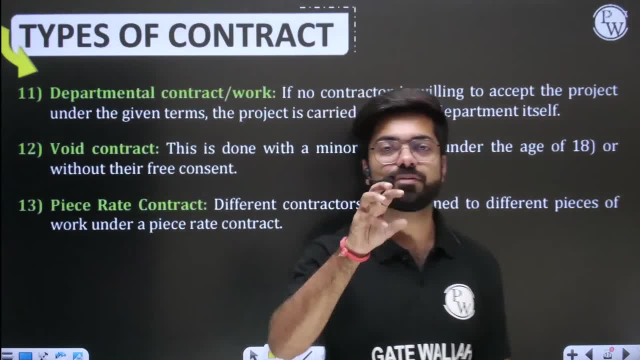 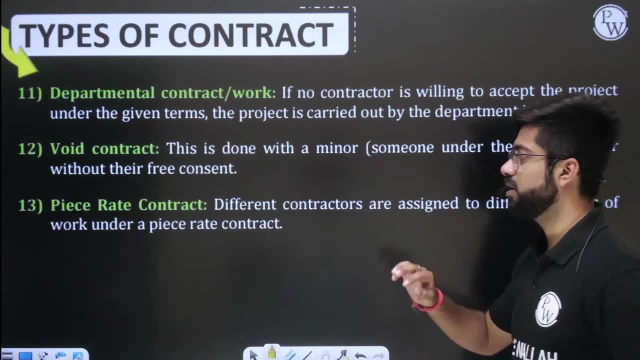 You put a wire, Put a rail. In this way, the work is divided into different parts, That is, different pieces. different pieces of work are given to different contractors. Different pieces of work are given to different contractors. Peace rate contract. 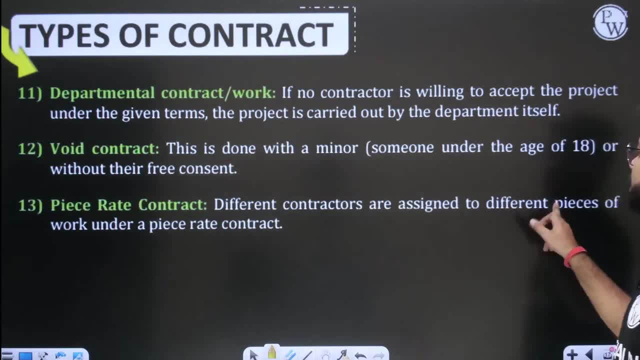 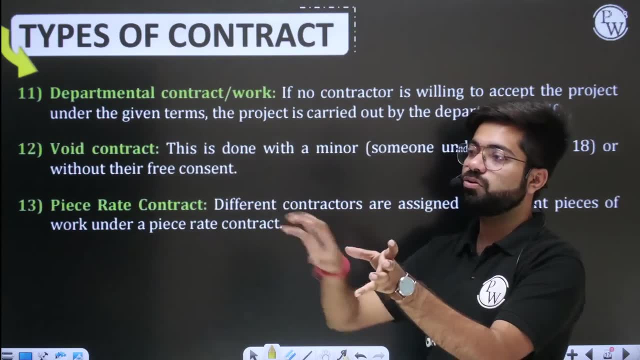 Okay, That is. different contractors are assigned to different pieces of work. in a big job, In a big job, small pieces are made And every contractor is told to do this, You do that, You do this, You do that. So 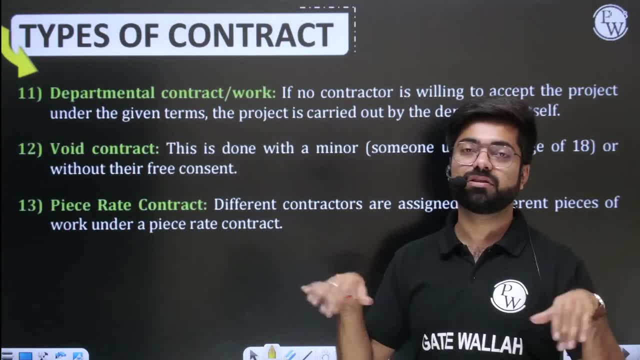 different jobs are given. For example, the house is built, So one is given the work of the wall, One is given the work of the foundation. One is told you go and put the electricity line. One is told you do the work of plumbing. 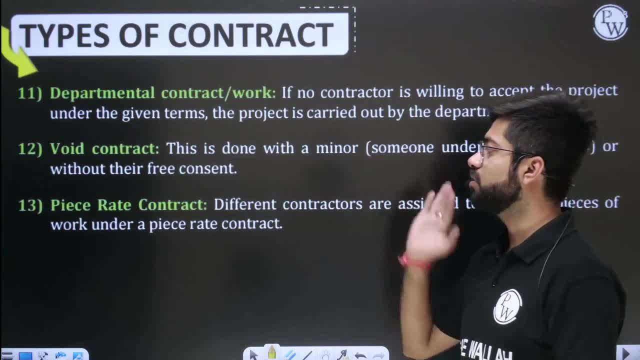 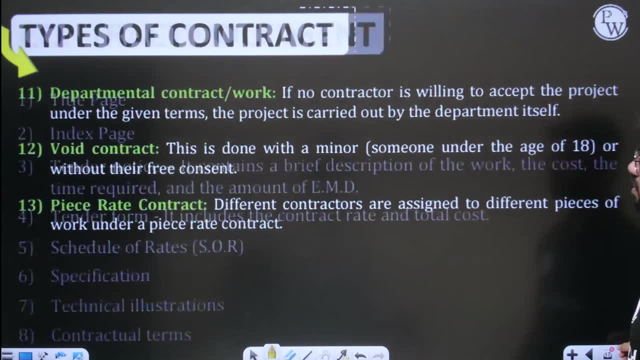 Plumbing the pipes that are used. So in this way different contractors are called and different contracts are made. This is called peace rate contract, So peace rate work is also called. So you must have understood that these are the different types. 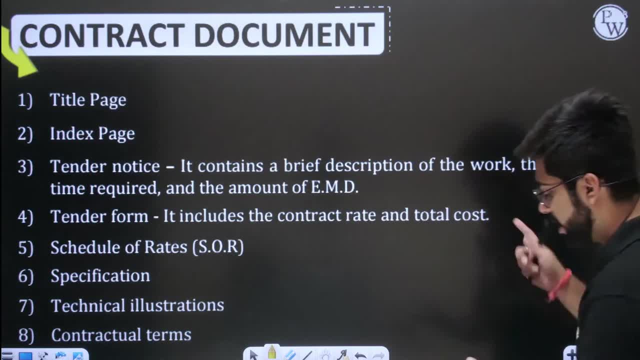 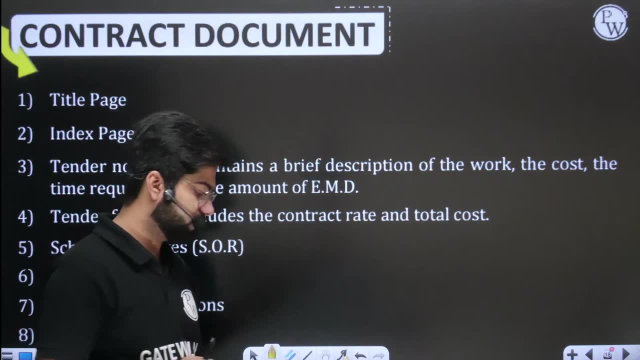 of contracts that are made. Okay, This is the last slide of today, Sir. the orientation of the CE course, which will start tomorrow. its orientation: Okay, The orientation of the CE course, which will start tomorrow. its orientation: See in the first class. 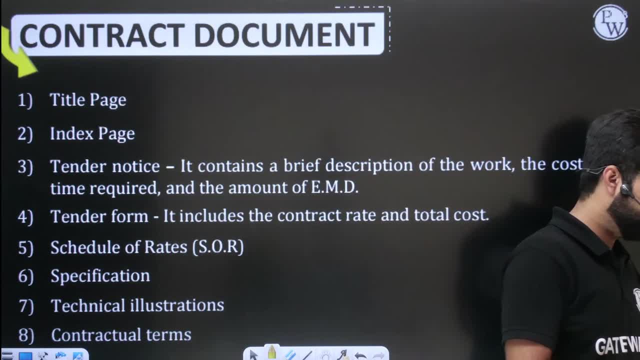 Otherwise, if the orientation is different, then the orientation of the CE course, which is starting from tomorrow, is different Otherwise. Otherwise, whatever is starting to look in the app, otherwise we will finish here tomorrow. then here the survey is starting from 12 o'clock in the evening in the crash course. 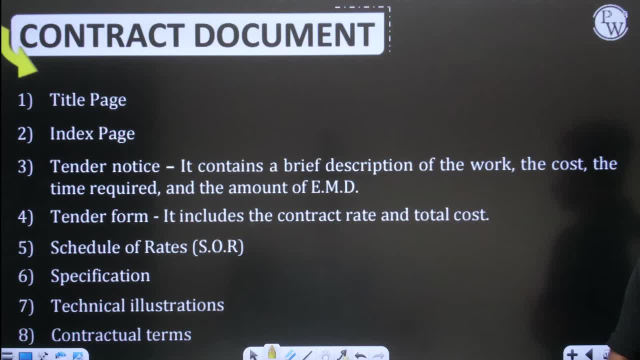 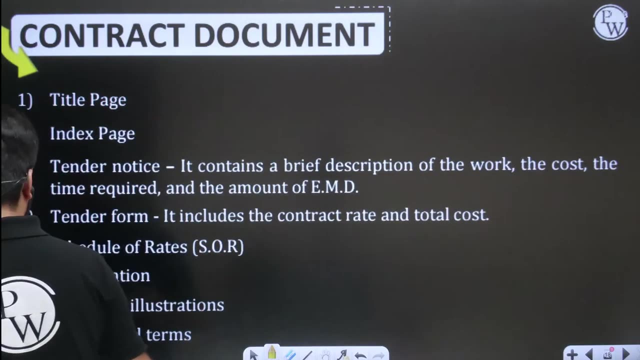 Okay, now let's talk about which contracts have documents. right, Let's talk a little bit about the documents that are there in the contract. So what are the documents in the contract? First of all, what is the title page? The title page will obviously be the name of the work: what to do if it is the work of flood fighting, or if it is to make a canal, or if it is maintenance or whatever work, is mainly written on the first page. then there is a little description. 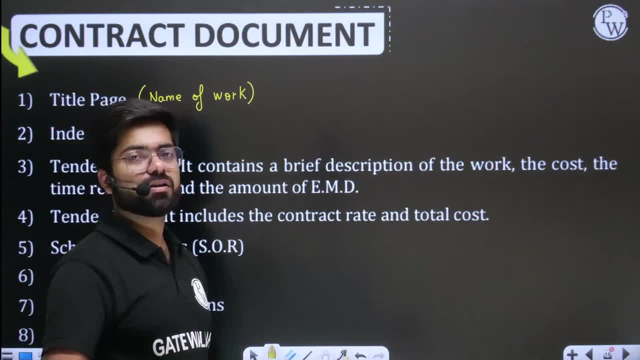 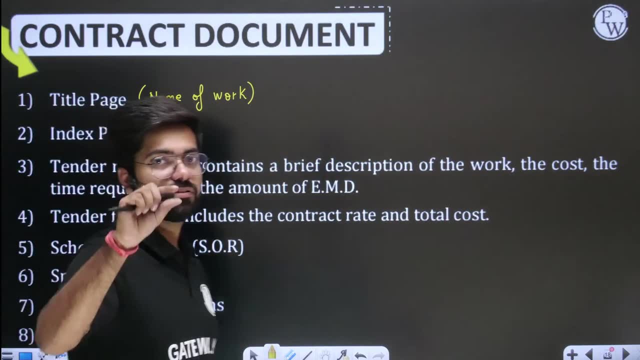 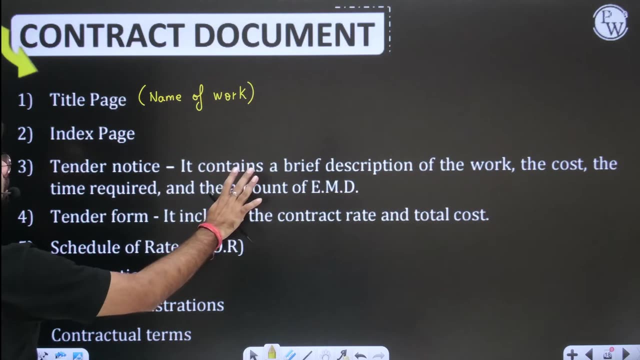 Then there is an index page. there are different pages in the index page that it will cost so much money. so many things are written separately. Okay, Sometimes there is a contract. there are very expensive contracts, very expensive contracts are made. then there will be an index page. then there will be a tender notice. there will be a brief description given in it that how much cost, how much time and how much earnest money to deposit that tender notice is done. 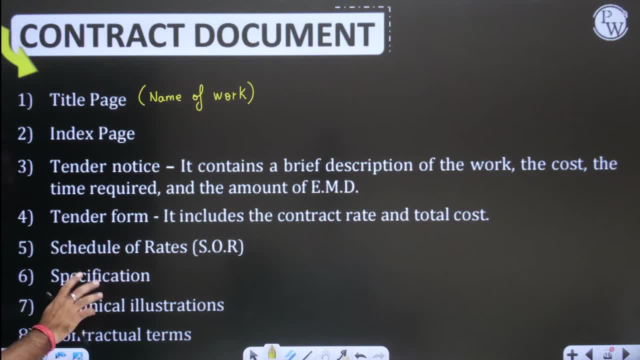 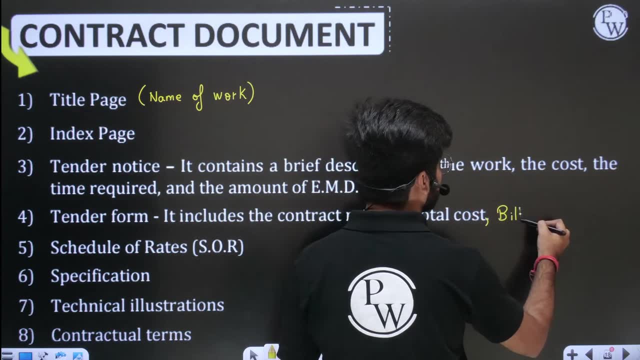 Then there will be your tender form- tender forms have been told to you, in which your contract rate will be, total cost will be. there are bill of quantities- okay, bill of quantities, which are called BOQs. You will have to fill all these bills in the tender form. 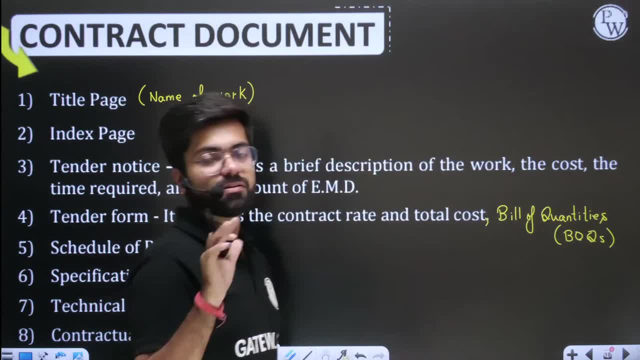 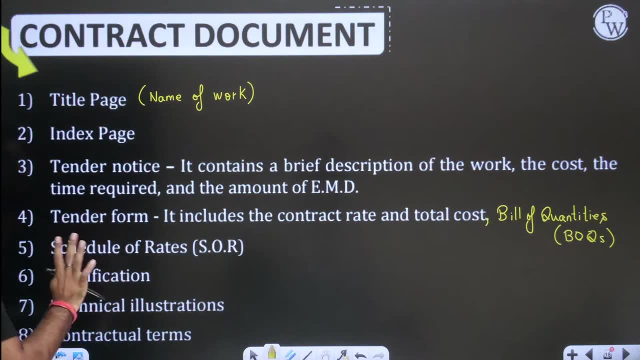 In that see the contractor's money. as the contractor's money is less or more, how will this be decided? is the contractor working less or more? we get to know all that only from this tender form. In it, its rate, cost, total bill of quantities are all found in it. 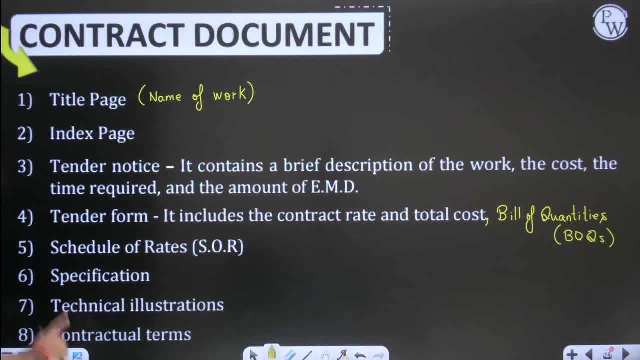 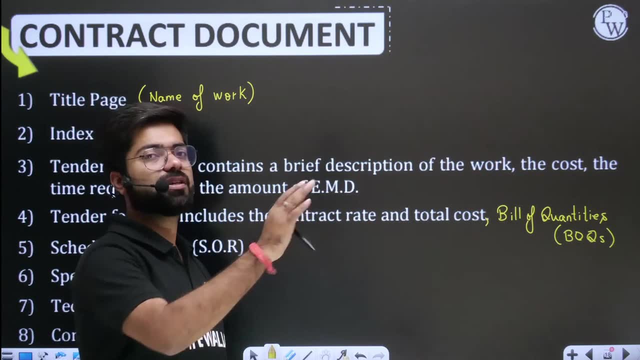 Okay, everything will be known from here. Then there is the schedule of rates. right, the schedule of rates. Now what happens in the schedule of rates generally? Peter Woddy has his own schedule of rates. This much, this much, you have to provide this much. 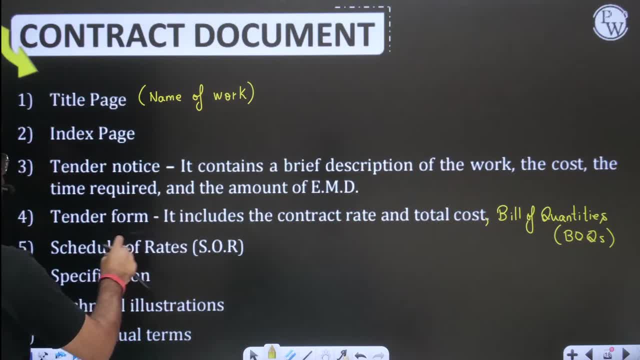 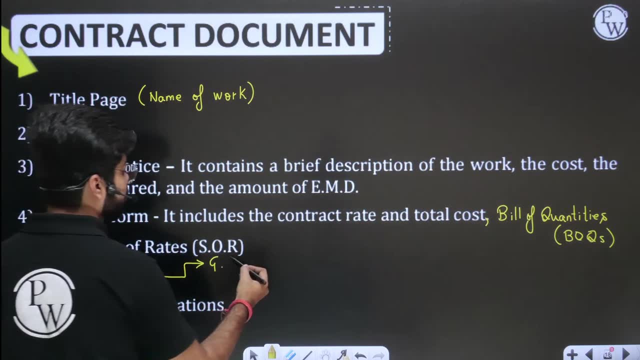 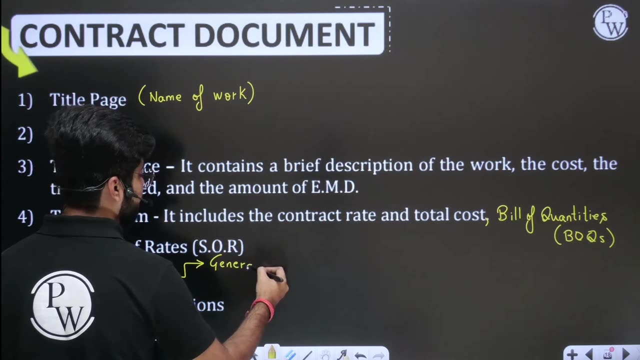 you have to provide this much, So that schedule of rates, that, whatever things will happen, you will have to provide around this price. Then there are specifications. there are two specifications. one is called General GCC, General Contract Conditions. General Conditions are done that these things should be like this. we need this, we need our canal in this way. 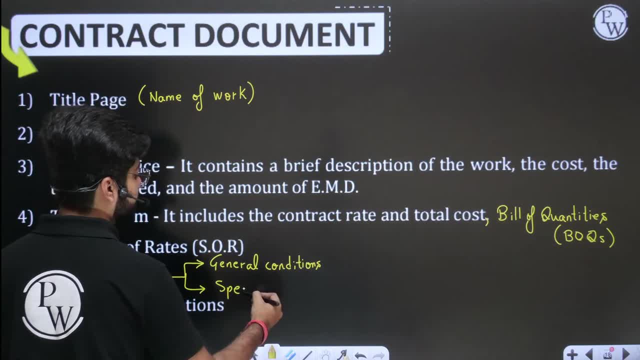 two or three trees should also be planted next to it. and then there are special conditions. you have to tell something special separately: that our house is being built, put a swimming pool in it, make a small one at the back. so these are all special conditions. 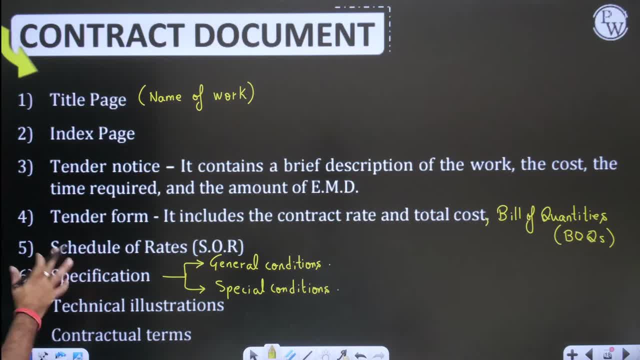 whatever the specifications are, the conditions of the contract are told here. then there are technical drawings etc. there are technical drawings, etc. that there will be a lot of drawings, that there will be a map, there will be elevation, whatever will be applied in it, then all those technical stations are in it and in the end there are contractual terms. 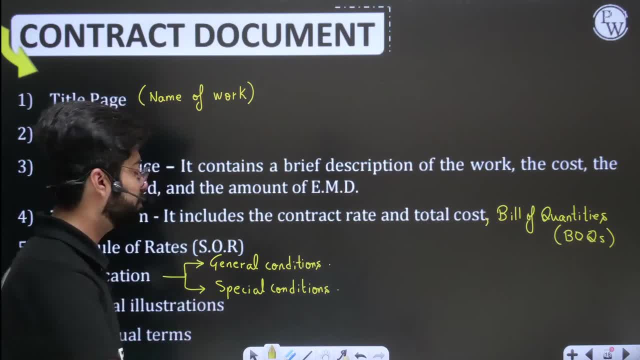 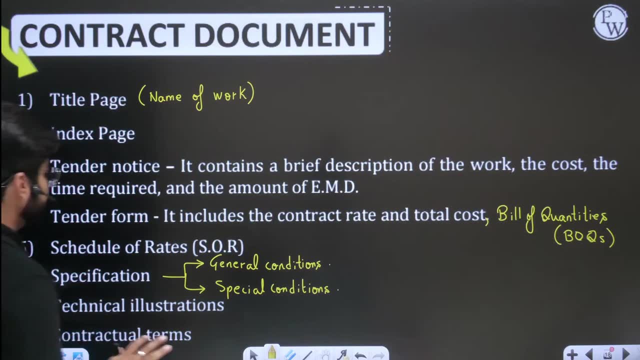 that if this happens, then we will do this. if that happens, then whatever contractual conditions are, they are all written here in it. Okay, I hope you understood this very well in a very simple way. okay, but the contract is after the tender. 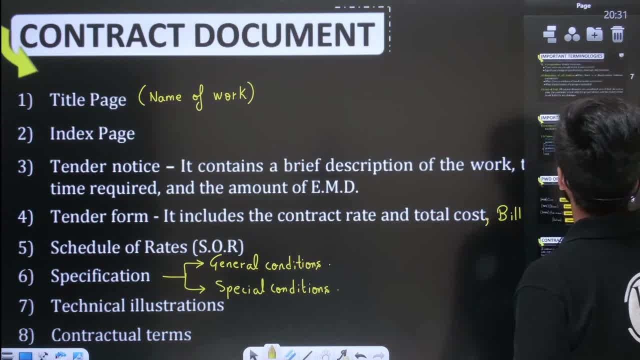 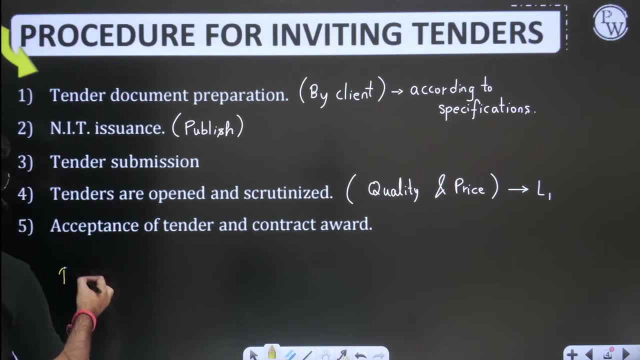 if we tell you a little: tender, tender was also here, so tender. I told you in the beginning that tender document is written. okay, which are these documents? we give you an idea. okay, if we talk about documents, then one is in it. 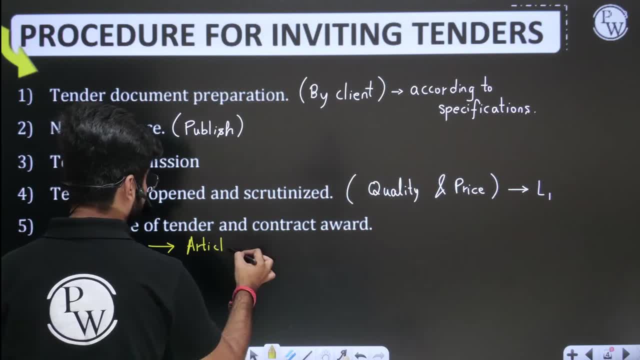 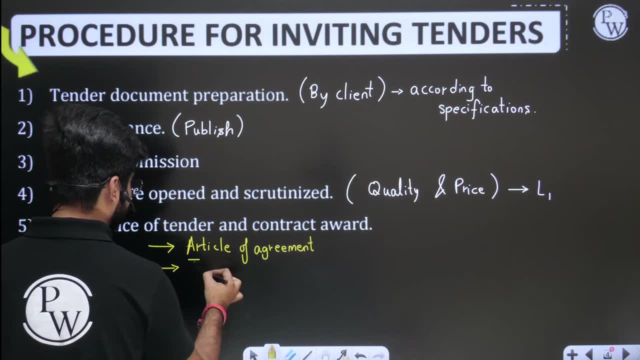 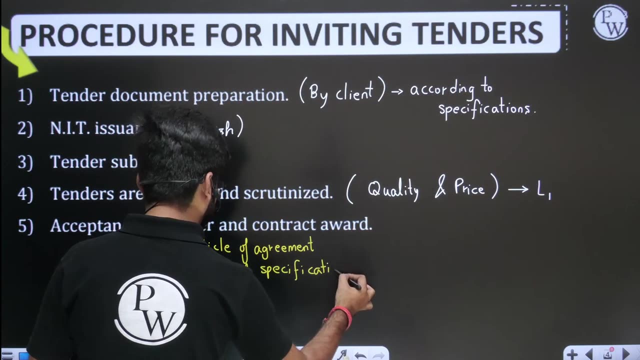 Article of Agreement, that how will both the parties agree? here It is written about because it is there. then, after that, all technical engagements are said: Ion, this thing we need Today, this much size is told. then all this thing is said, technical specifications are all brought about and some drawings are also put in it. 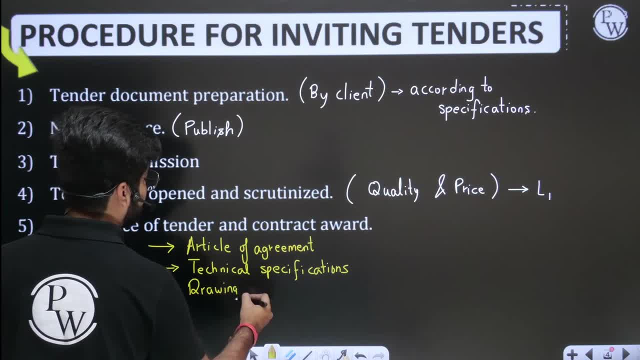 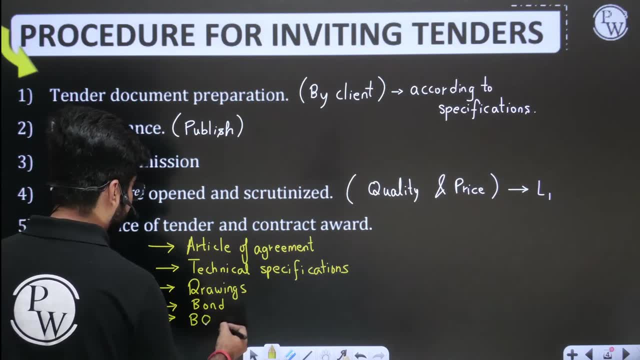 okay, these are the works of Jограф Yipur. Still some work is shown by the Spanish board. Then, whatever the bond will be okay, the wi-fi после testesremo will remain. it will be told then on the basis of this, there is another Southwest in管, Maine tomorrow. 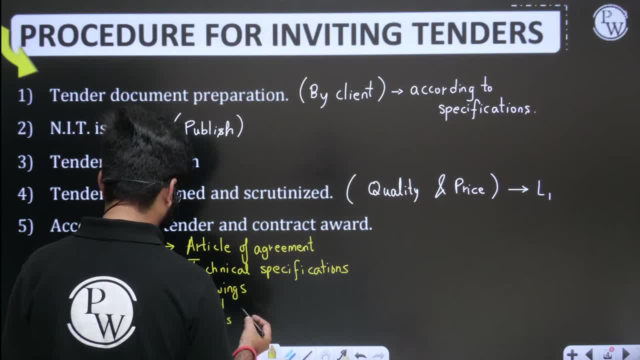 The rest will be what will be the rest, that is, whether the rating for the entire university data will be down or anything. According you, If it is material or not, then we will take care of it here as well. list of makes. but you will list with. sorry, I think you can, I can, I have. 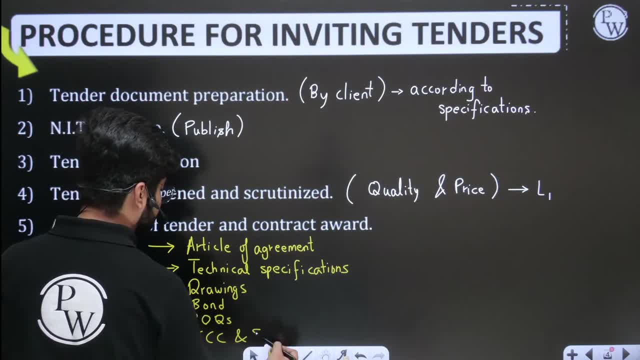 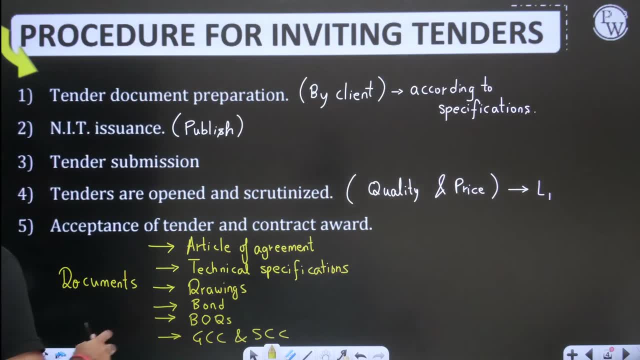 escape my general contract conditions only or, which is, special contract conditions only. generally I'm a basic startup. I'm especially good with a lecture so I thought I have to go. such is ready. I think I was care. I'll tell you a key process: site become good. so my health could not be handed over to health. 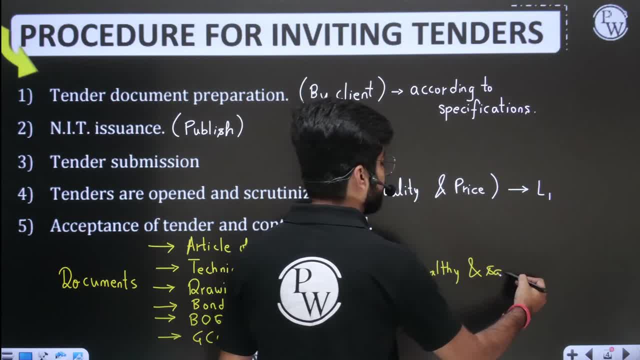 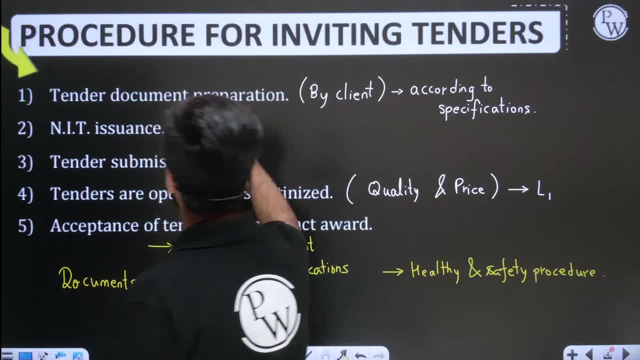 or safety procedure can follow, can I contractor co health or safety procedure can follow, can I? so what's up? TV tender form may ready and I starting my this are a document. when they always feel it's called publish credit, we use of the SS, SS, SS, a honey to you. okay about health and safety procedure. well, 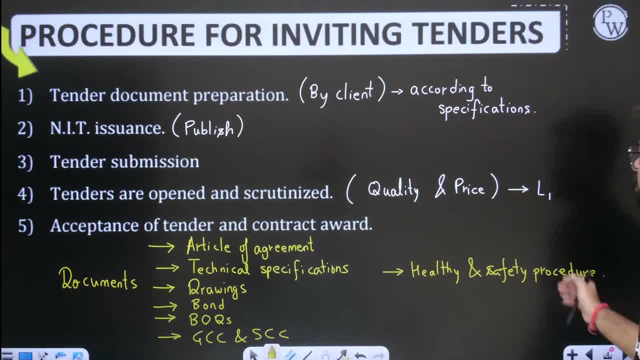 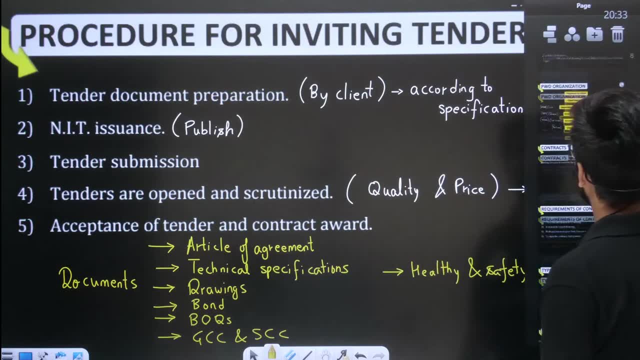 about the follow. look at the name. you could take a licking contactor. okay, this is health and safety procedure. follow can achieve the key sub-team in particular case. a challenge: smooth, very good speaker I hope key you are. some may be so I'm look poor aku samaj again. sorry time contact with a question, so 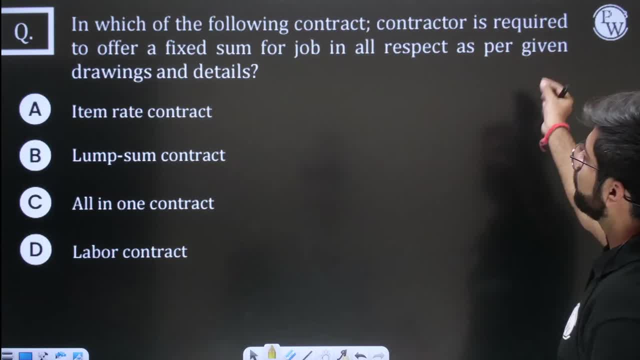 they can have low in which of the following contract: contractor is required to offer a fixed sum for a job. a fixed sum. but also comment, go, because some kiss me dengue. comment to you bottom how I fix. some kiss me the agar. obviously, boss, implement big dissonant is managerica, so don't you do jar goes too fast i'm. 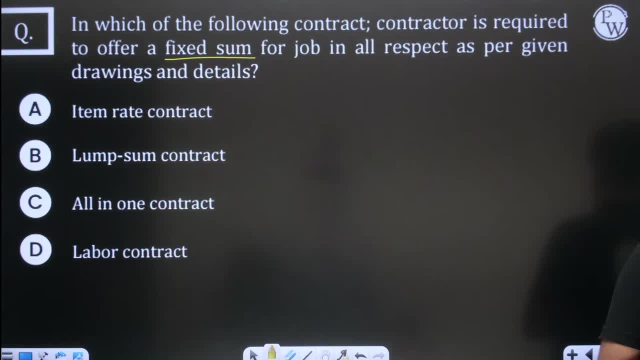 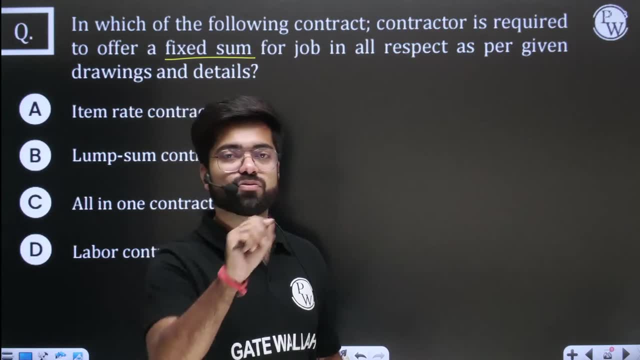 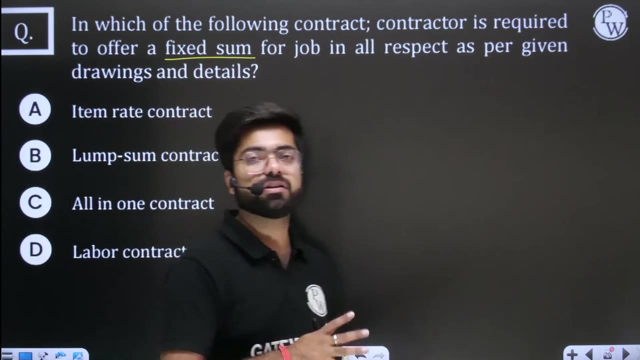 gonna take a quick attention to comment at all better. I'll be simple: breach. come at love with a kid to many bottom and a contractor about eliquid team, not just go preach clear here. his name, which I said was not enough, reach, come below to You- didn't agree with the contract. you had signed the contract but you refused it. this is called breach of contract. 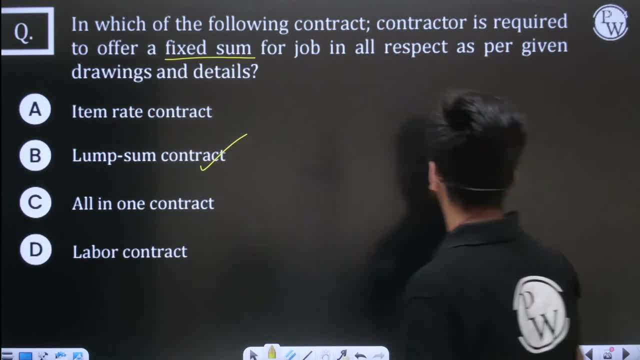 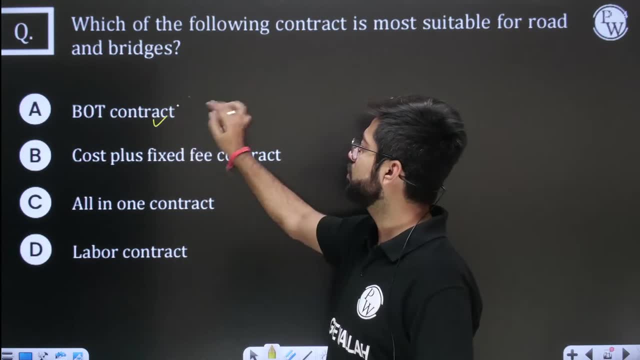 So what is fixed sum and what is lump sum? It is very basic. Then, which of the following contract is most suitable for road and bridges? I have told you about road and bridges, toll tax, one BOT contract, BOT built, operate, transfer. 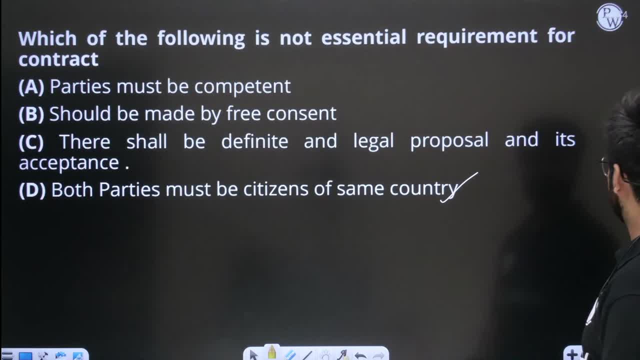 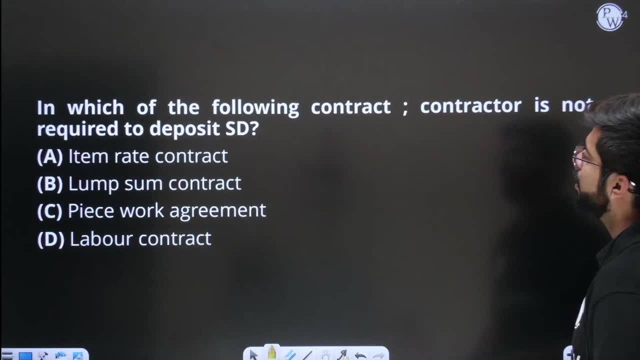 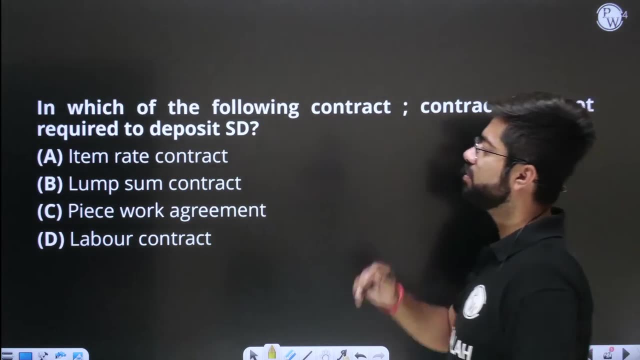 This was already a question. This is also done. This is also done. Fixed sum: this is the same question. Let's remove it. In which of the following contract contractor is not required to deposit security deposit In which he doesn't have to give security deposit? 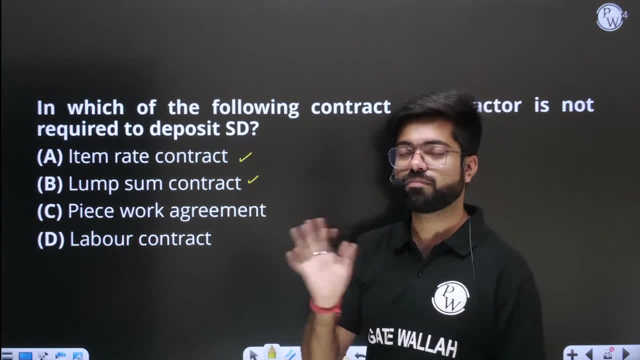 See, you have to give in item rate, in lump sum, in sum. you have to give security deposit In sum match you do anything. Don't give in piece work. You don't have to give in piece work because in piece work many different contractors come. 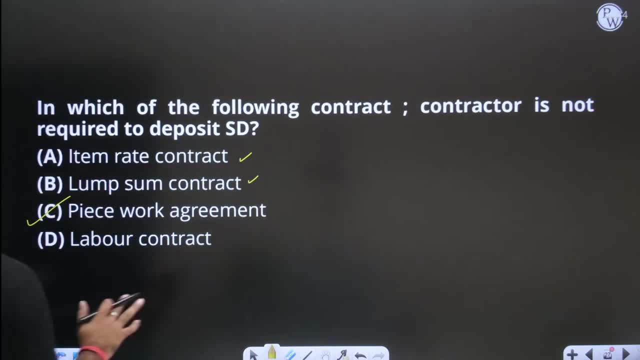 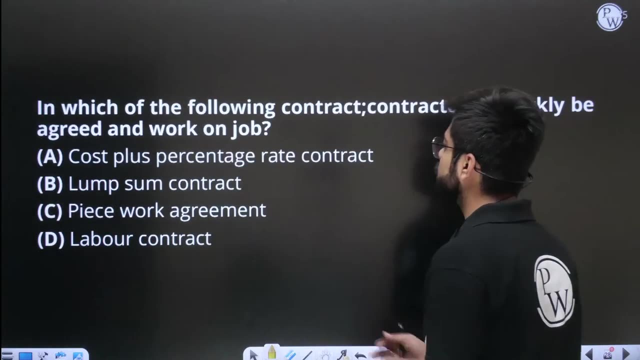 Everyone gets small work. There is no provision of security deposit in this- Okay. There is no loss of security deposit in this. All this has been corrected to piece In which of the following contract: contractor is quickly agreed and work on job- Okay. in which contractor consists a lot of enthusiasm to work on job. 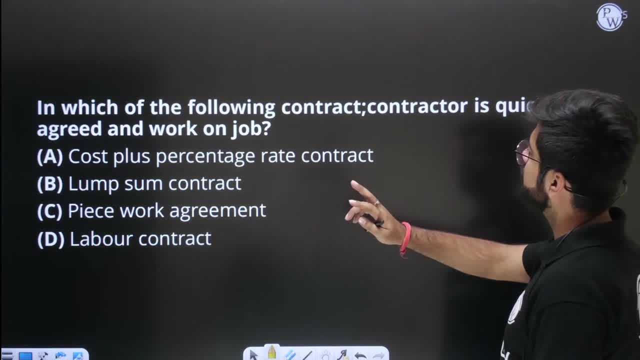 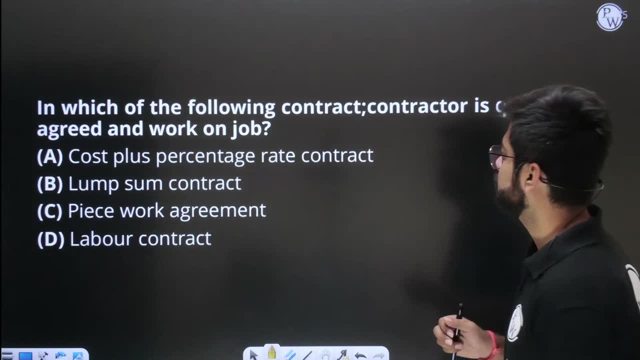 Okay, this is what he is asking. The English of D- norm is a little different. in here, Contractor is quickly agreed to work on job. Obviously there is a benefit in this, as he is coming to the job at the end of the once date. 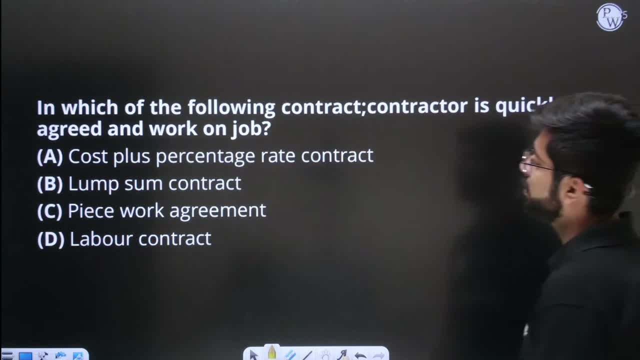 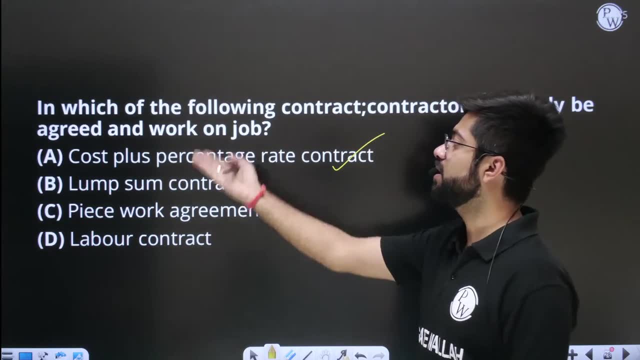 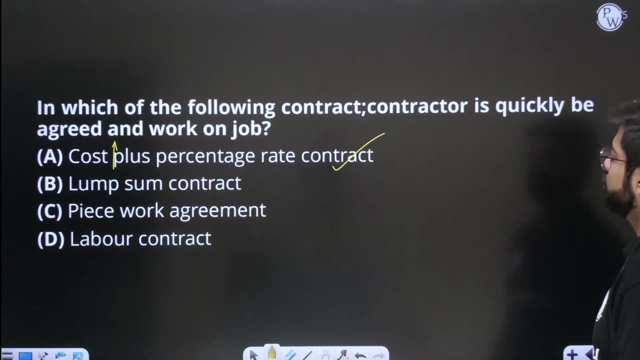 So yes, there is an agreement here. Okay, When the percentage is 10%, then he will try to increase the cost so that he can get a big percentage. then in the cost plus percentage, he will agree immediately. Then in which of the following contract the contractor tries to complete the job quickly? 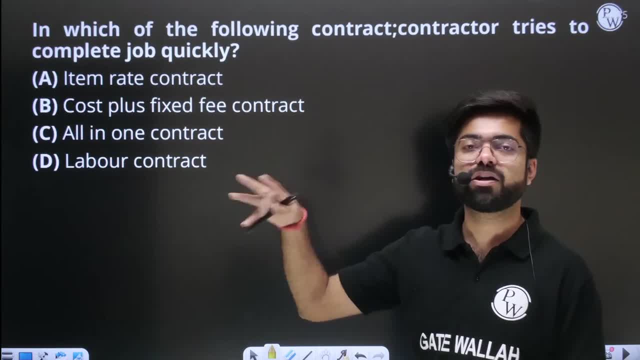 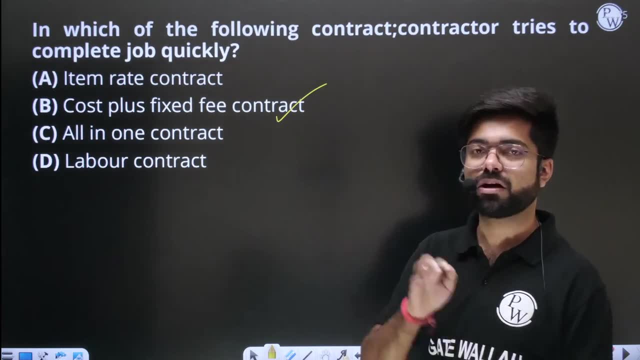 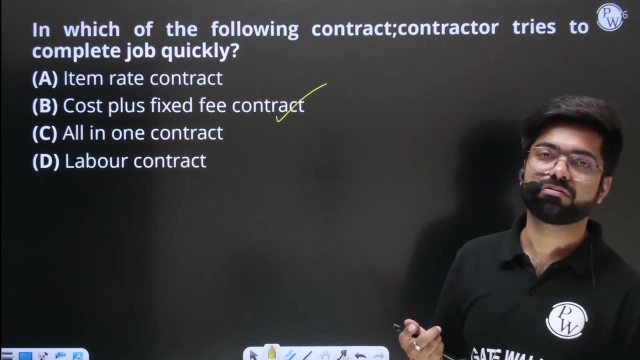 He will work quickly, he will not pull long, he will not try to increase the cost. he will do it quickly when, When he will get a fixed fee right, When he will get a fixed fee. I have told you that if he wants to get 10,000, and he knows that he will get 10,000 fixed, then finish that work quickly. 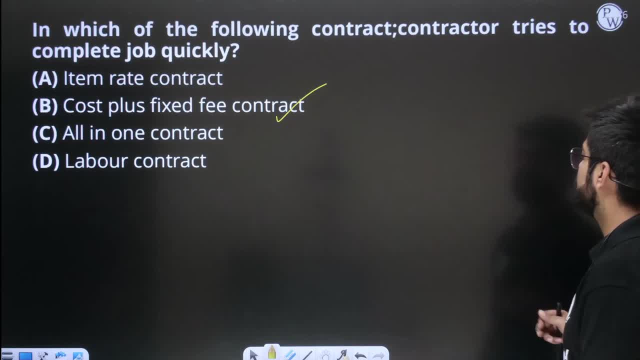 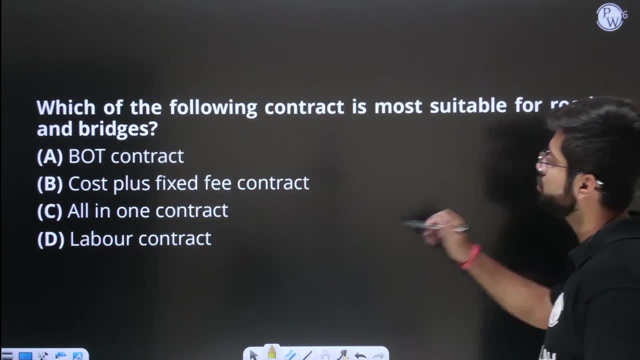 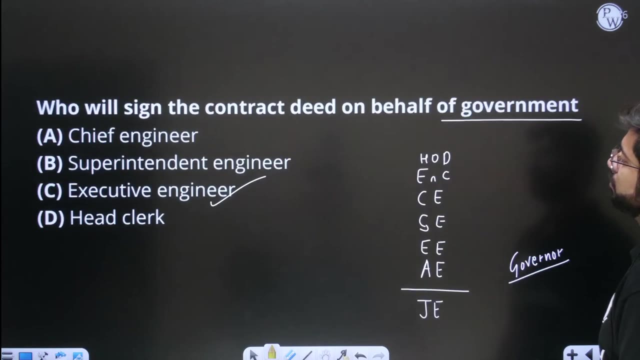 Finish that work quickly, okay, So this is your cost plus fixed fee contract. Okay, Simple, Simple, simple. simple. Then road, and for this there is a BOT contract. We have understood the contract. we have told you this, Okay, so I think all these questions are over. 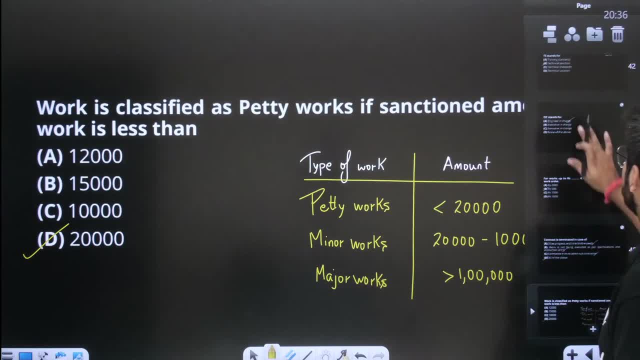 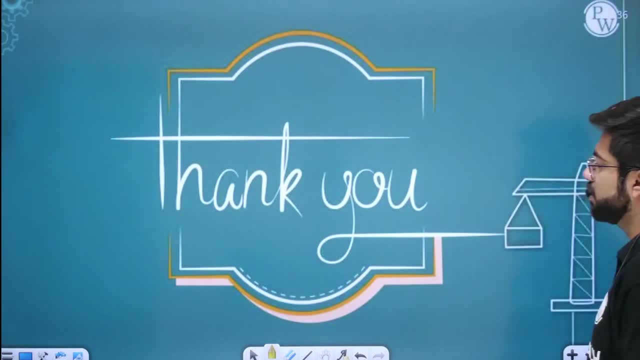 All the questions are over, So let's just end here, Okay, So I hope that you have understood the tender well. If there is any problem, you will not have any problem, So let's end. What else did we teach in BMC?